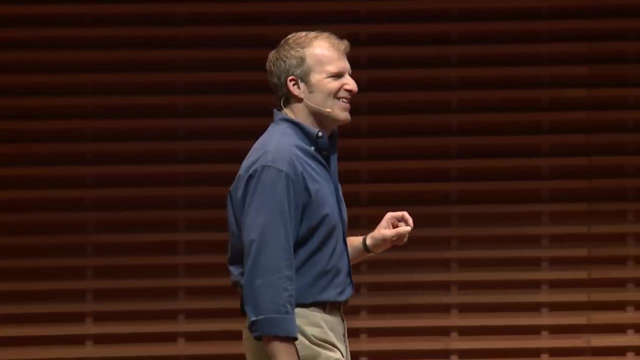 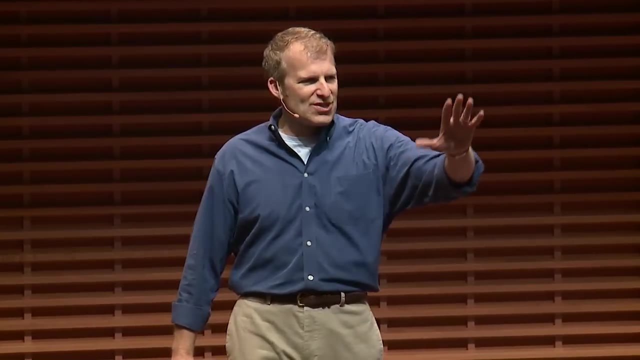 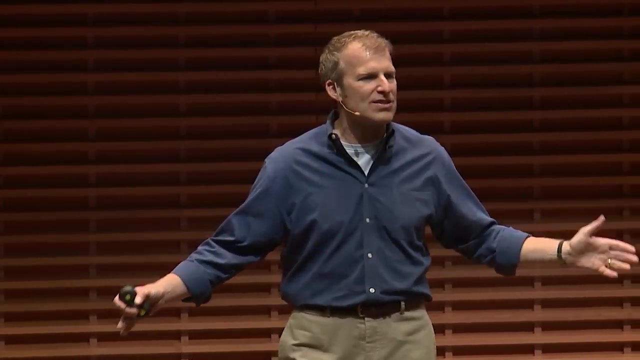 of us miss Of. We'll make sure to get this to you so you can torment your friends and family at a later date. When I first was exposed to this over 12 years ago, I only found three And I felt really stupid. So I like to start every workshop, every class I teach, with this. 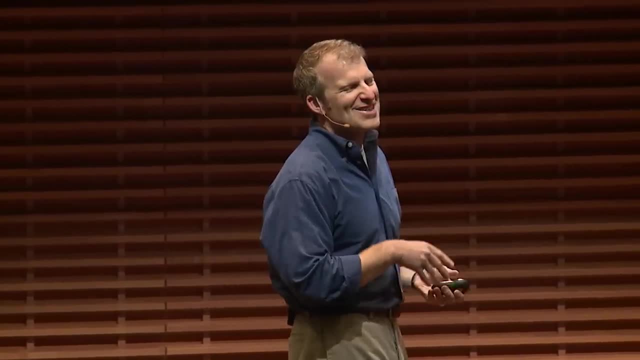 to pass that feeling along. No, no, that's not. that's not why I want to get this, And with that, here's my answer. I'm sure, if I could pass this to you, I think you could've why I do this. I do this because this is a perfect analogy for what we're going to be talking about. 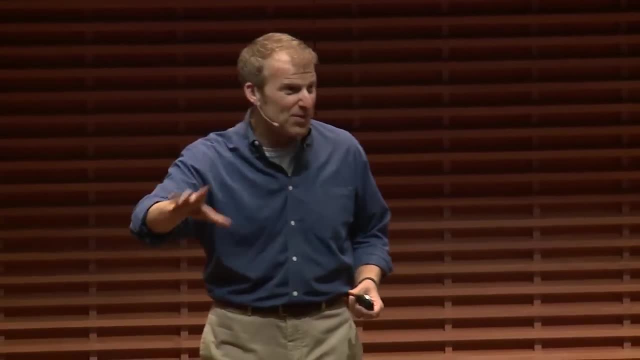 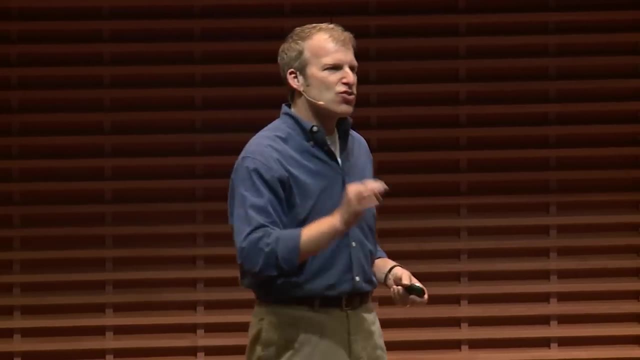 today. The vast majority of us in this room- very smart people in this room- were not as effective as we could have been in this activity. We didn't get it right, And the same is true when it comes to speaking in public, particularly when spontaneous speaking. It's little things that. 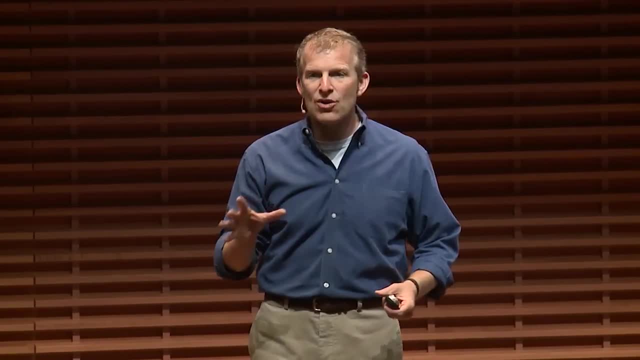 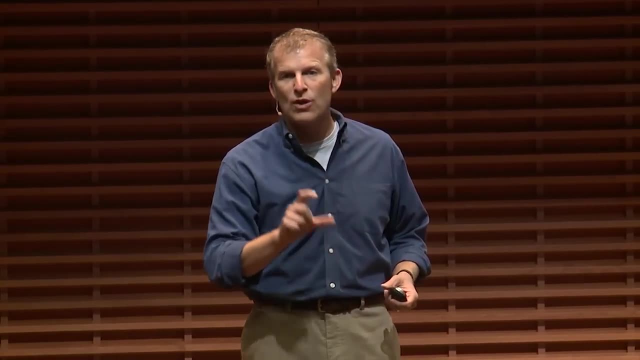 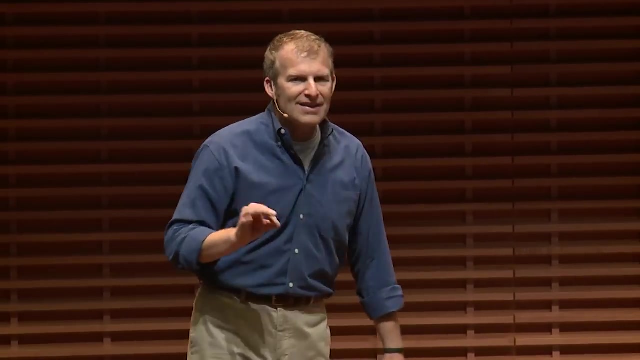 make a big difference in being effective. So today we're going to talk about little things in terms of your approach, your attitude, your practice that can change how you feel when you speak in public, And we're going to be talking primarily about one type of public speaking, not the type, 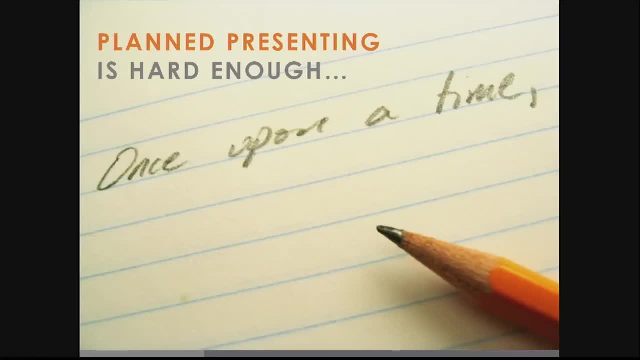 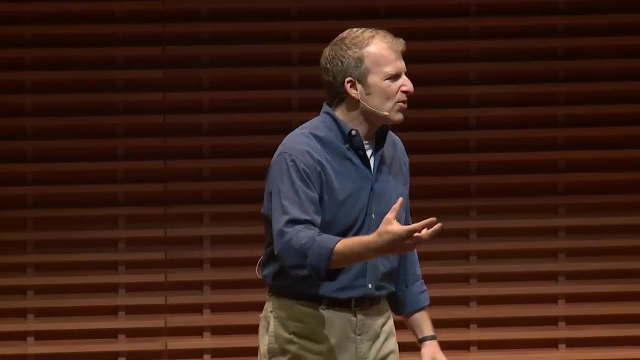 that you plan for in advance, the type that you actually spend time thinking about. you might even create slides for These are the keynotes, the conference presentation, the formal toasts. That's not what we're talking about today. We're talking about spontaneous speaking. 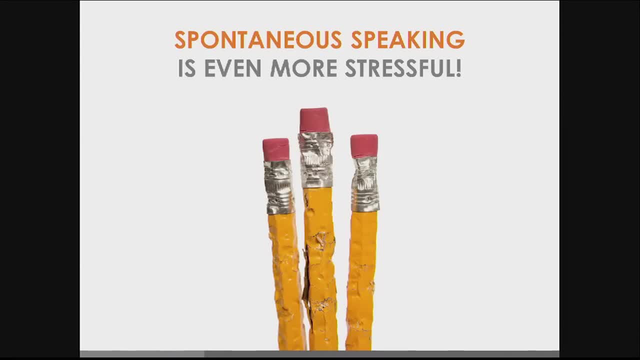 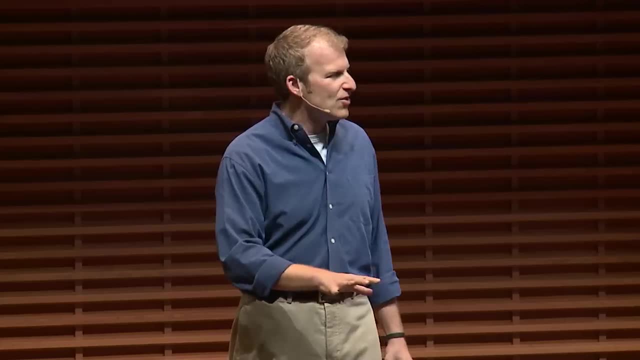 When you're in a situation that you're asked to speak off the cuff and in the moment. What we're going through today is actually the result of a workshop I created here for the business school Several years ago. a survey was taken among the students and they said: what are things we could do to help? 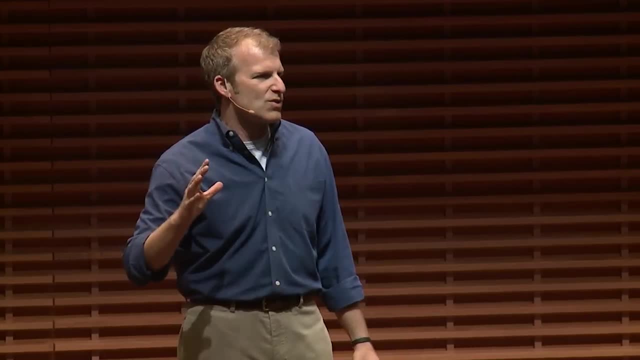 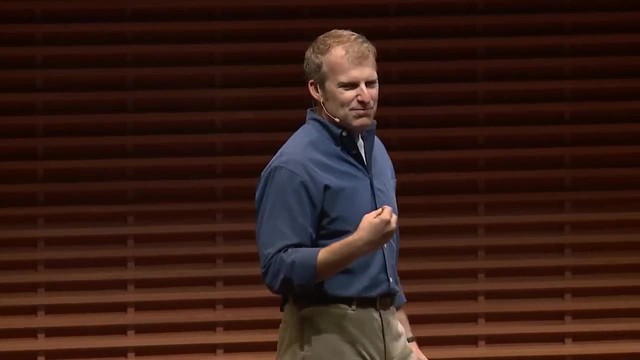 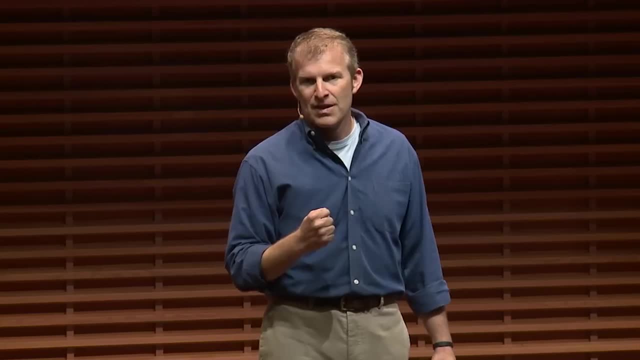 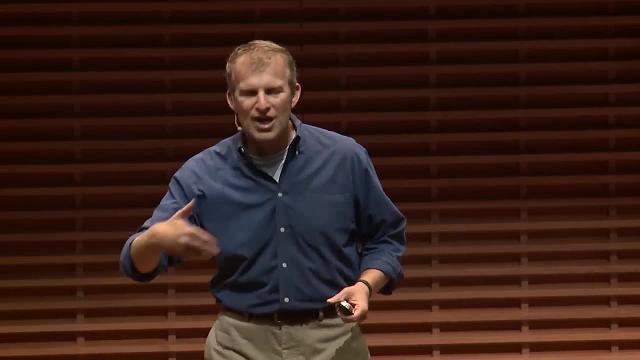 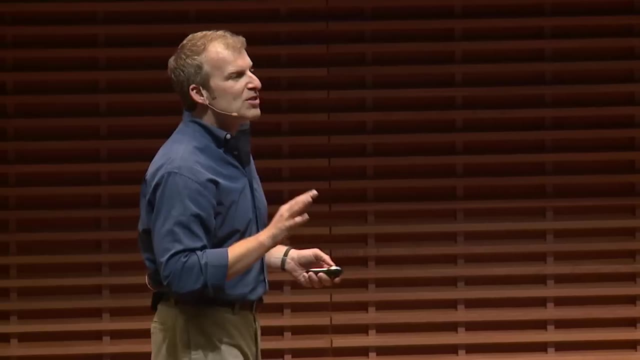 So today we're going to talk about little things in terms of your approach, your attitude, your practice that can change how you feel when you speak in public, And we're going to be talking primarily about one type of public speaking, not the type that you plan. 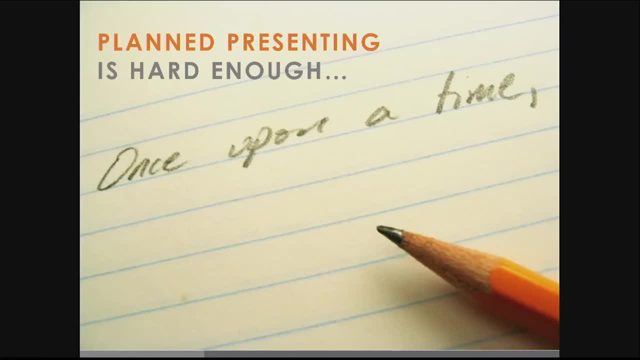 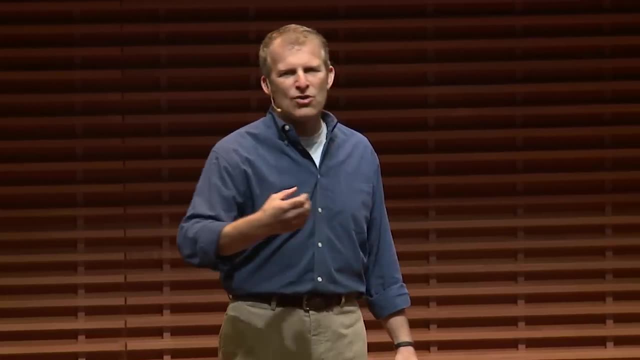 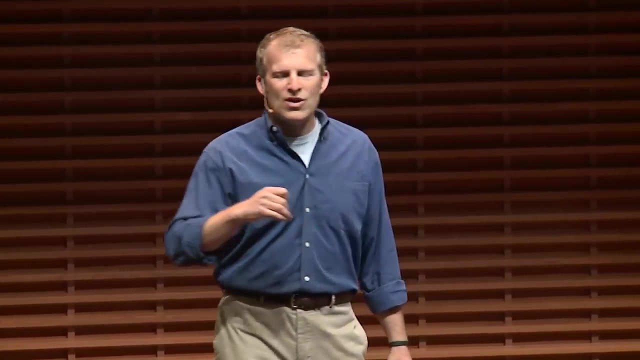 for in advance, the type that you actually spend time thinking about. you might even create slides for These are the keynotes, the conference presentation, the formal toasts. That's not what we're talking about today. We're talking about spontaneous speaking. 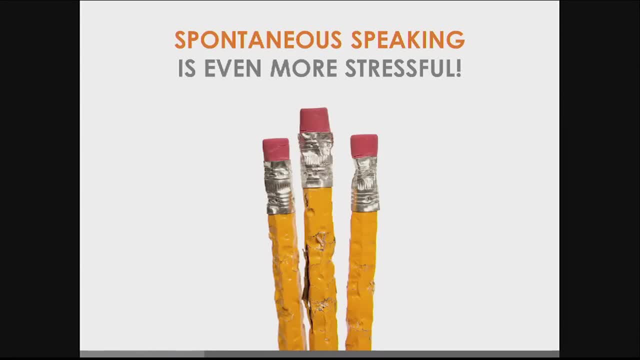 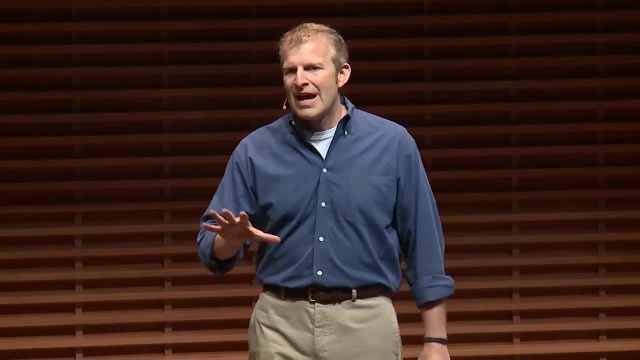 We're talking about a conversation that you're asked to speak off the cuff and in the moment. What we're going through today is actually the result of a workshop I created here for the business school Several years ago. a survey was taken among the students and they 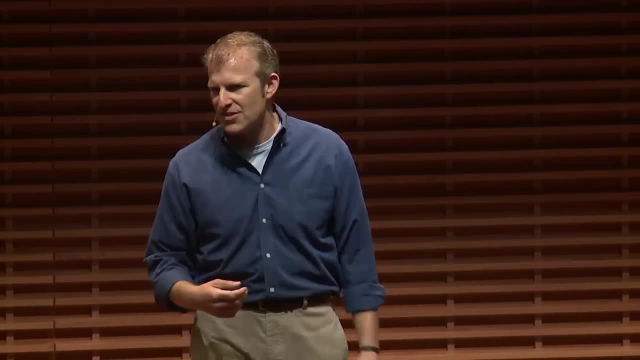 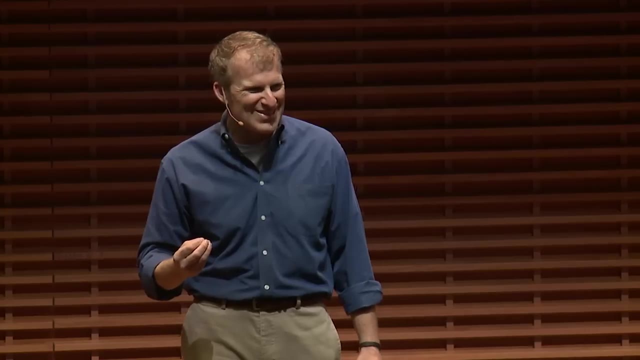 said: what are things we could do to help make you more successful here. And at the top of that list was this notion of responding to cold calls. Does everybody know what a cold call is? It's where the mean professor like me looks at some students and says, what do? 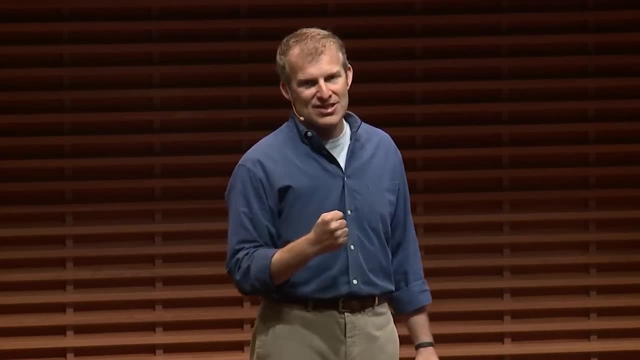 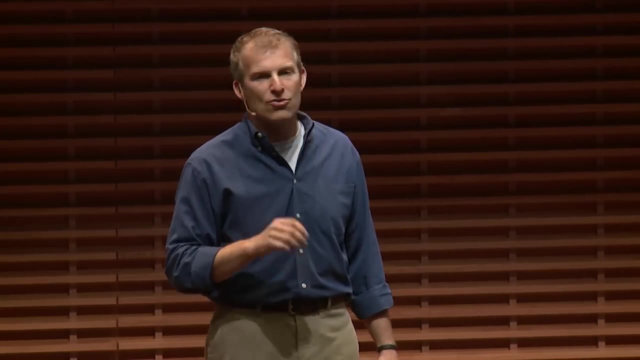 you think, And there was a lot of panic And a lot of silence. So as a result of that, this workshop was created and a vast majority of first year students here at the GSB go through this workshop. So I'm going to walk. 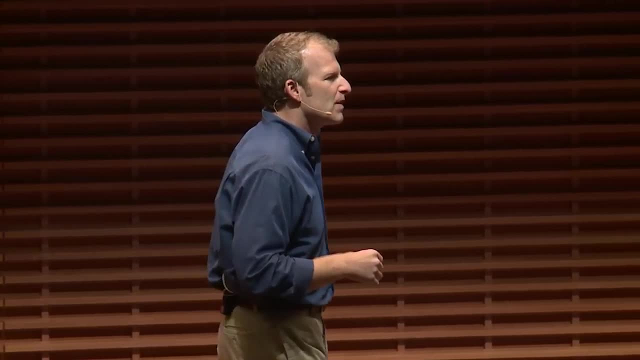 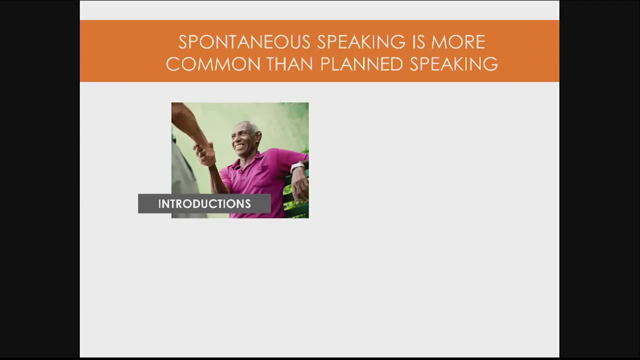 you through sort of a hybrid version of what they do. The reality is that spontaneous speaking is actually more prevalent than planned speaking. Perhaps it's giving introductions. You're at a dinner and somebody says: you know so, and so would you mind introducing them Maybe. 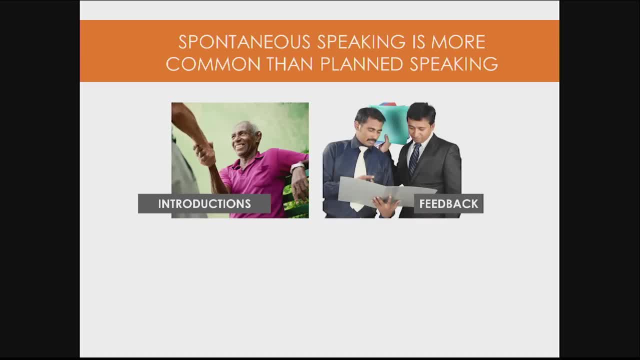 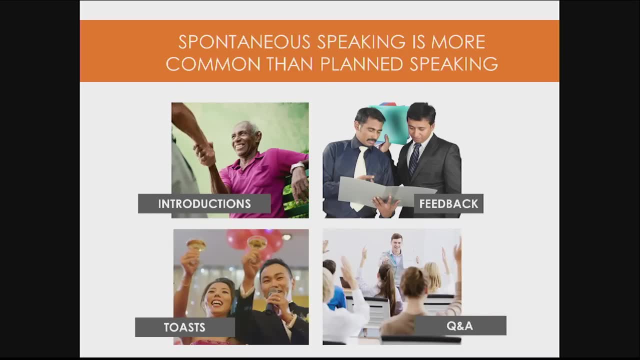 it's giving feedback. in the moment Your boss turns to you and says: would you tell me what you think? It could be a surprise toast Or, finally, it could be during the Q&A session And, by the way, we will leave plenty of time at the end of our day today for Q&A. I'd love to 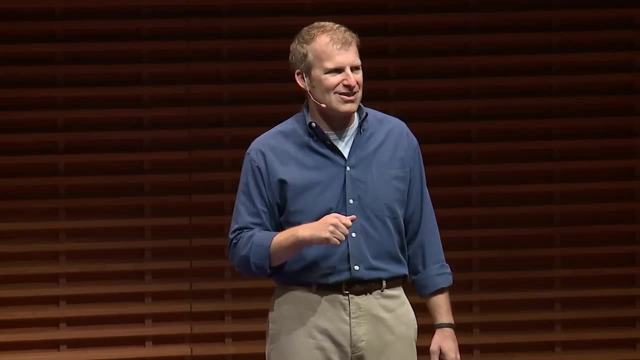 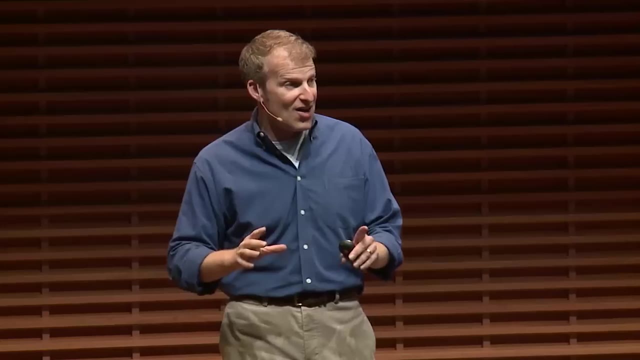 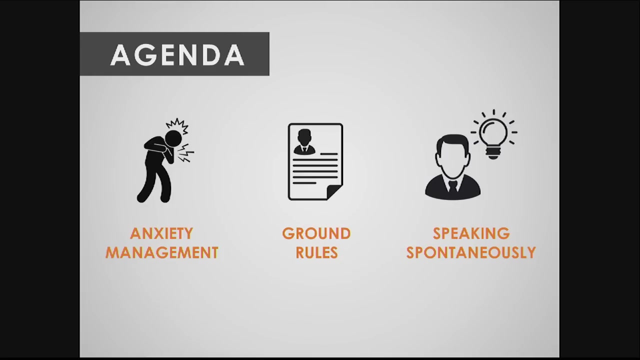 hear the questions you have about this topic or other topics related to communicating. So our agenda is simple: In order to be an effective communicator- regardless of if it's planned or spontaneous- you need to have your anxiety under control. So we'll start there. 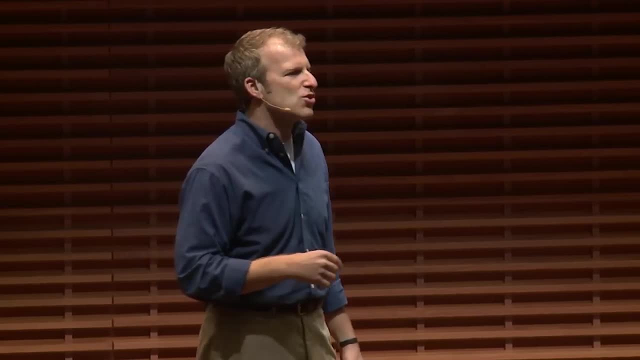 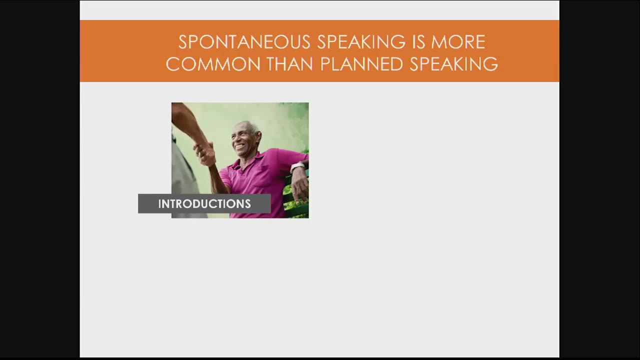 workshop, So I'm going to walk you through sort of a hybrid version of what they do. The reality is that spontaneous speaking is actually more prevalent than planned speaking. Perhaps it's giving introductions. You're at a dinner and somebody says you know so and so. 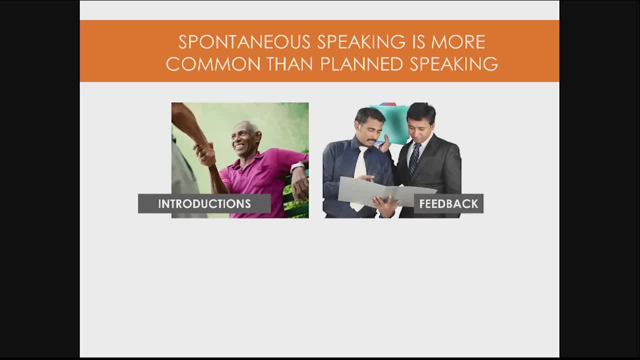 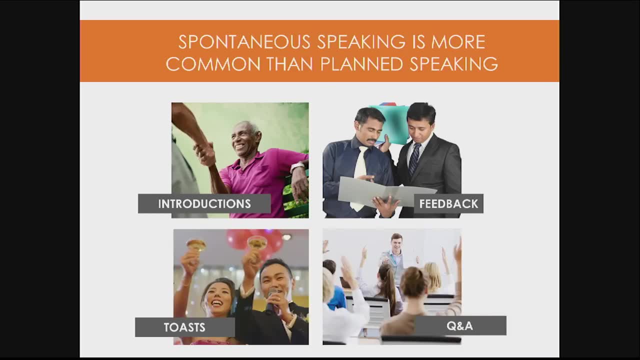 would you mind introducing them? Maybe it's giving feedback In the moment your boss turns to you in says: would you tell me what you think? It could be a surprise toast Or, finally, it could be during the Q&A session And, by the way, we will leave plenty of time at the end of our day today for 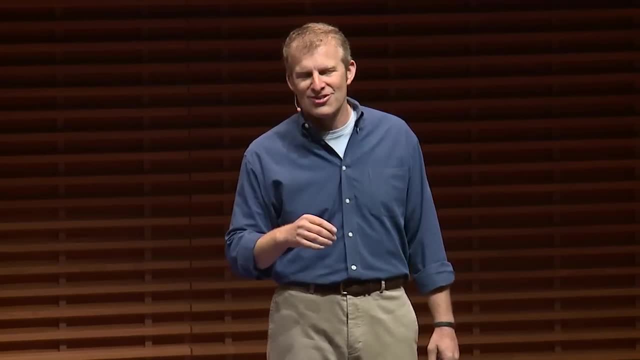 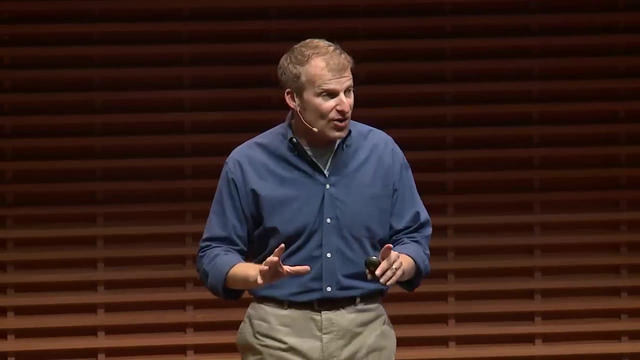 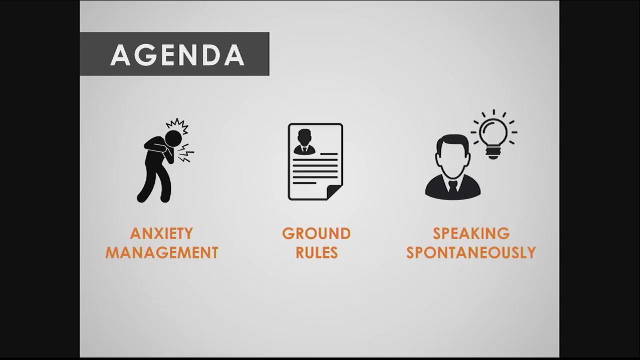 Q&A. I'd love to hear the questions you have about this topic or other topics related to communicating. So our agenda is simple: In order to be an effective communicator- regardless of if it's planned or spontaneous- you need to have your anxiety under control. So we'll start there. 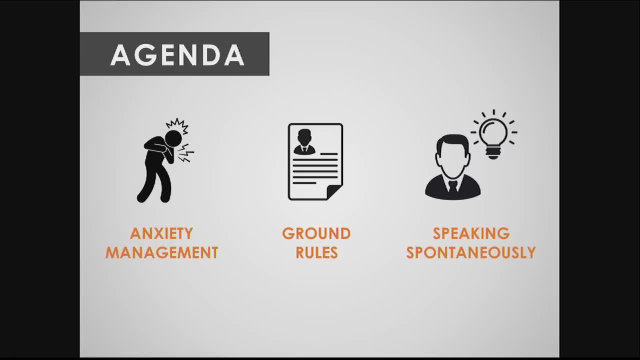 Second, what we're going to talk about is some ground rules for the interactivity we'll have today, And then, finally, we're going to get into the heart of what we will be covering And again, as I said, lots of activity, and I invite you to participate. So let's get started with anxiety. 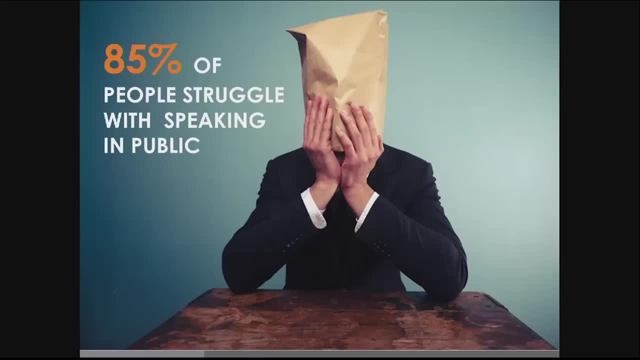 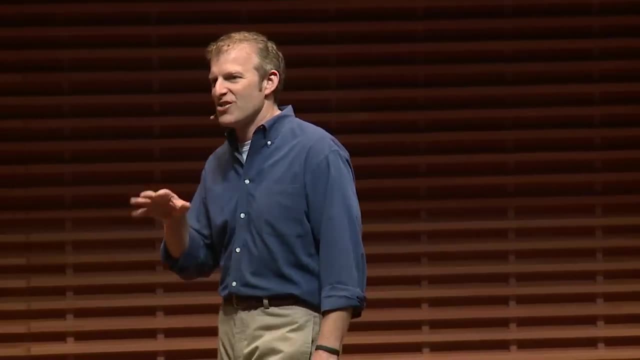 management. 85% of people tell us that they're nervous when speaking in public, And I think the other 15% are lying. We could create a situation where we could make them nervous too. In fact, just this past week, we've had a lot of people tell us that they're nervous when speaking in. public, And I think the other 15% are lying. We could create a situation where we could make them nervous too. And again, as I said, lots of activity, and I think the other 15% are lying. We could create a situation where we could make them nervous too. And again, just this past week, a study from 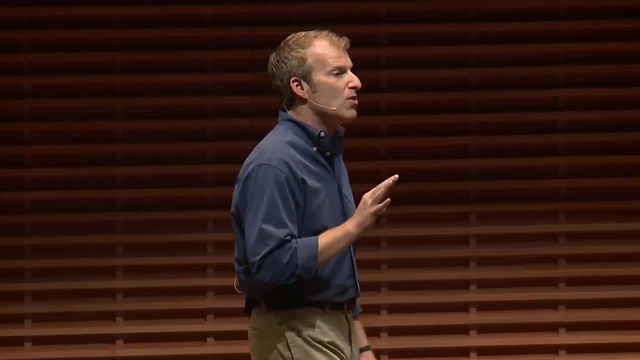 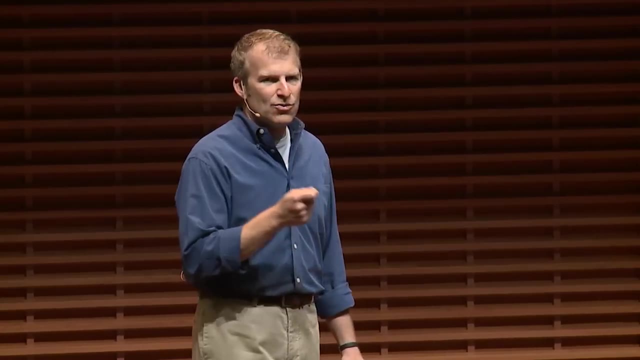 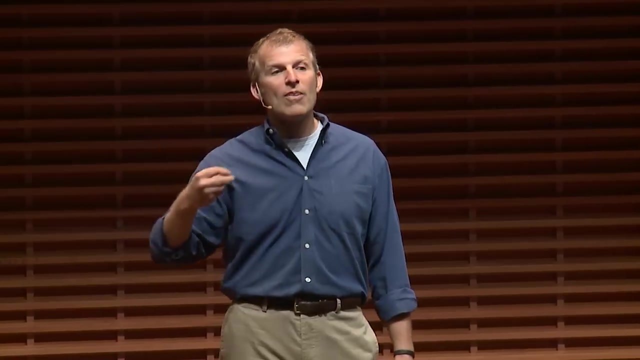 Chapman University asked Americans what are the things you fear most? And among being caught in a surprise terrorist attack, having your identity stolen, was public speaking Among the top five, was speaking in front of others. This is a ubiquitous fear and one that I believe we can. 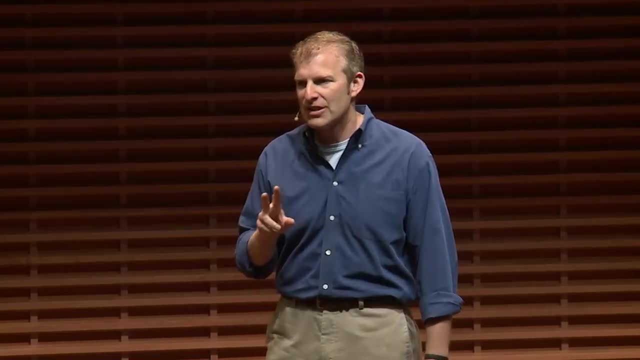 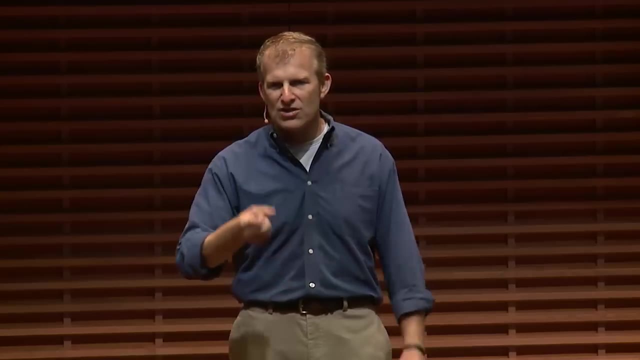 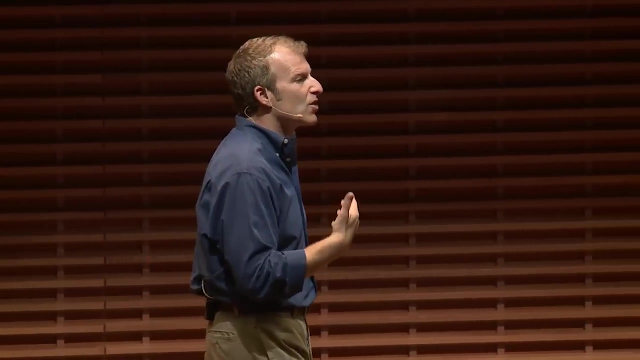 learn to manage- And I use that word manage very carefully, because I don't think we ever want to do it. It gives us energy, helps us focus, tells us what we're doing is important, but we want to learn to manage it. So I'd like to introduce you to a few techniques that can work, And all of these 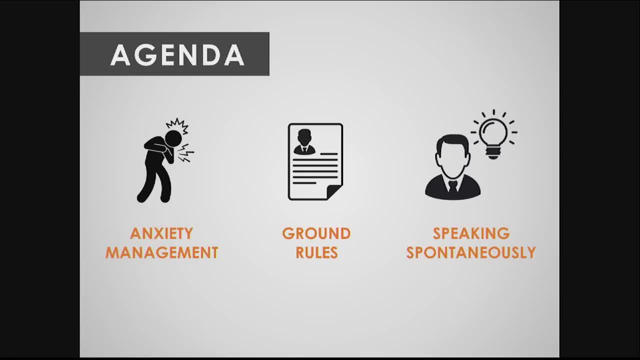 Second, what we're going to talk about is some ground rules for the interactivity we'll have today, And then, finally, we're going to get into the heart of what we will be covering And again, as I said, lots of activity, and I invite you to participate. 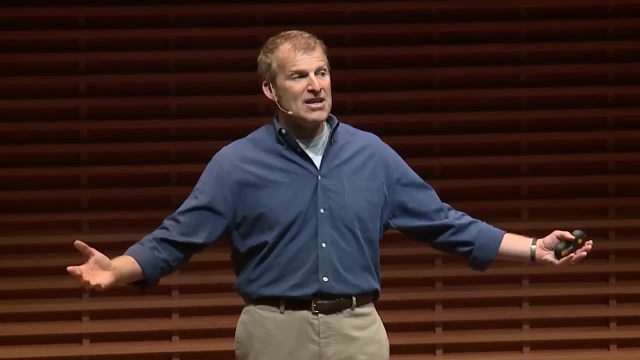 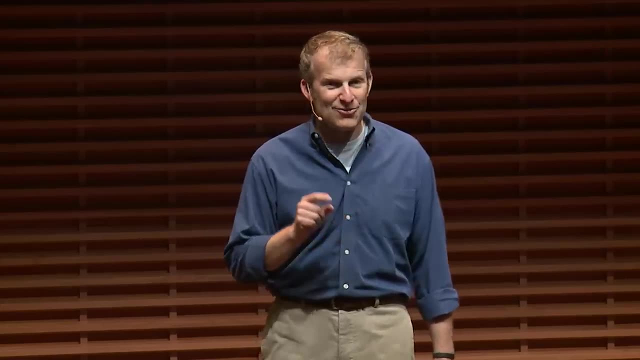 So let's get started with anxiety management. Eighty-five percent of people tell us that they're nervous when speaking in public, And I think the other 15 percent are lying. We could create a situation where we could make them nervous too, In fact, just this past. 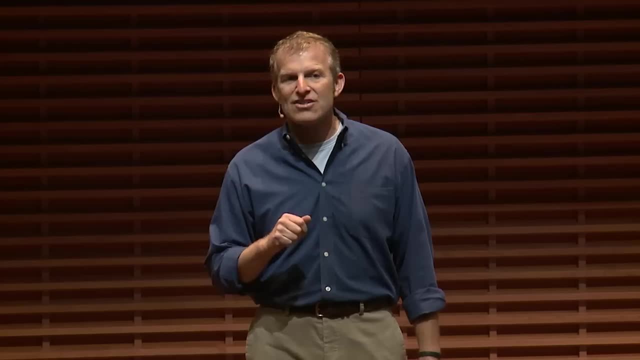 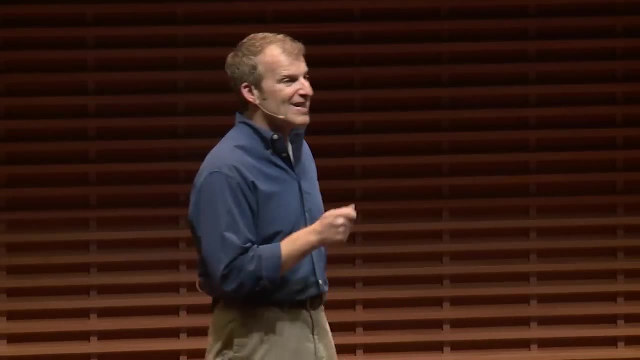 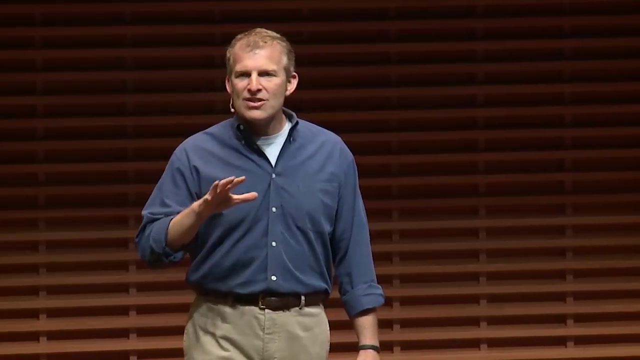 week, a study from Chapman University asked Americans what are the things you fear most, And among being caught in a surprise terrorist attack, having your identity stolen, was public speaking Among the top five was speaking in front of others. This is a ubiquitous fear. 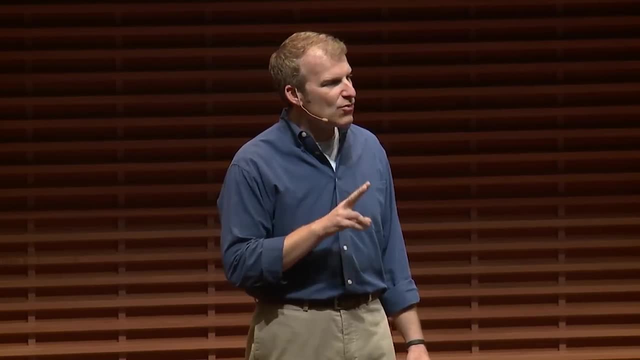 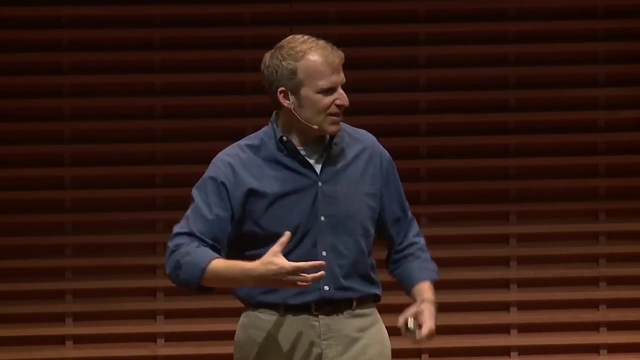 and one that I believe we can learn to manage- And I use that word manage very carefully, because I don't think we ever want to overcome it. Anxiety actually helps us. It gives us energy, helps us focus, tells us what we're doing is important, but we want to learn to. 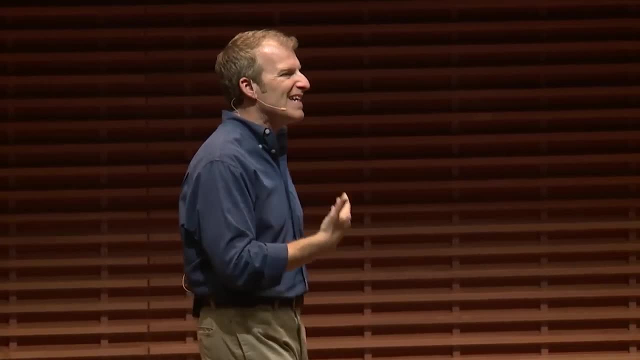 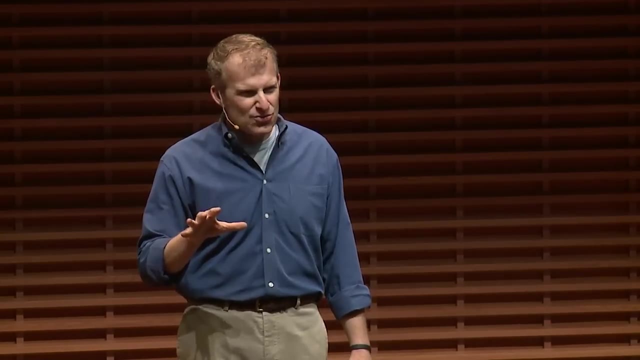 manage it. So I'd like to introduce you to a few techniques that can work, And all of these techniques are based on academic research. But before we get there, I'd love to ask you what does it feel like when you're sitting in the audience watching a nervous speaker present? How do 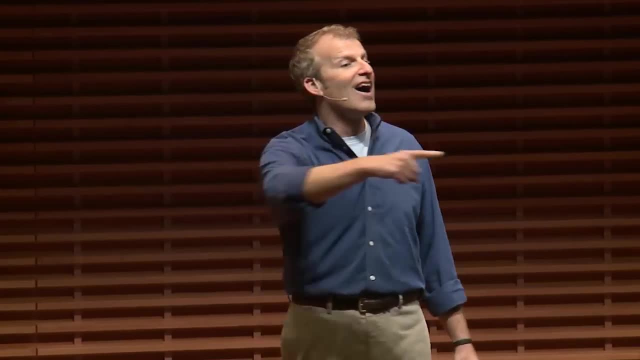 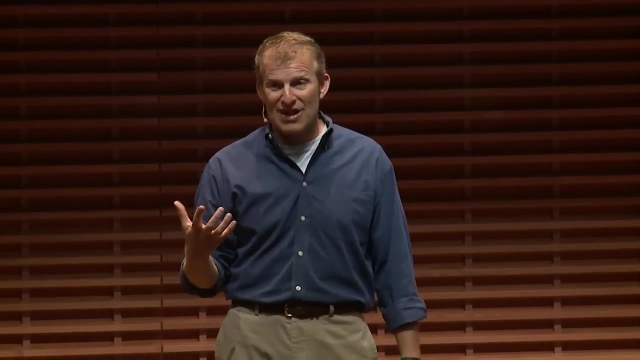 you feel. Just shout out a few things. How do you feel? Uncomfortable, Uncomfortable. I heard many of you going, yes, uncomfortable. It feels very awkward, doesn't it? What do we do Now? a couple of you probably like watching somebody suffer, but most of us don't. 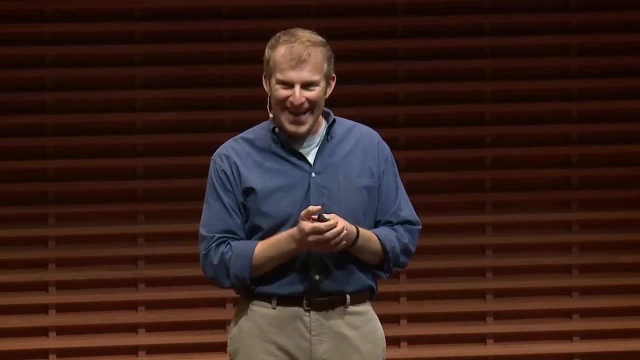 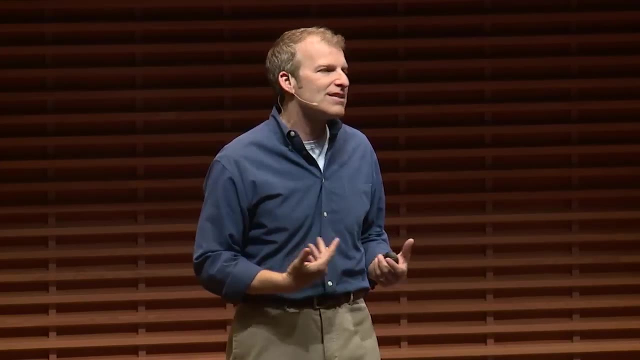 So what do we do? We sit there and we nod and we smile or we disengage. And to the nervous speaker looking out at his or her audience seeing a bunch of people nodding or disengaging, that does not help. So we need to learn to manage our anxiety because fundamentally, your job as a communicator. 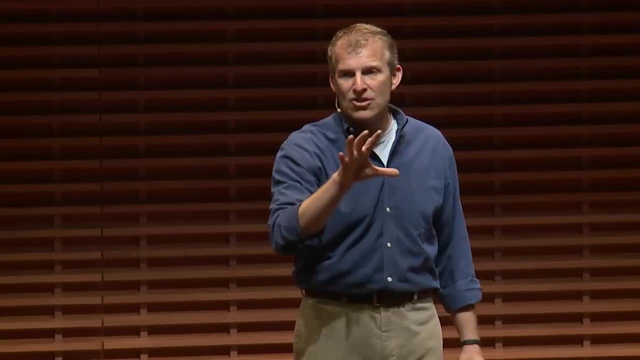 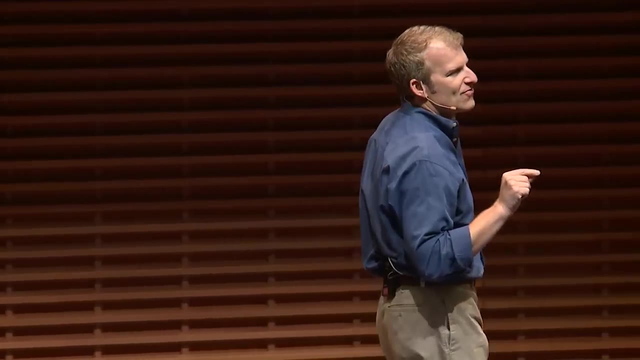 regardless of if it's planned or spontaneous- is to make your audience comfortable, Because if they're comfortable they can receive your message. And when I say comfortable, I am not referring to the fact that your message has to be sugar-coated and nice for them to hear. 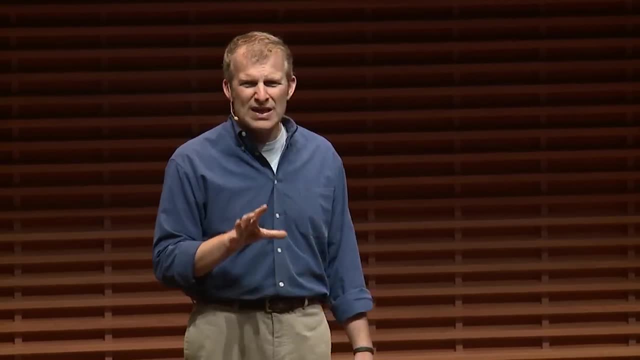 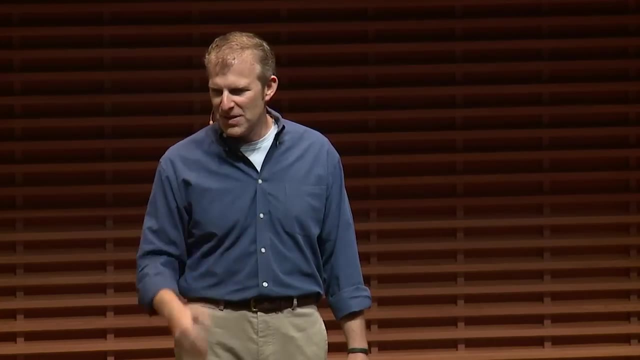 techniques are based on academic research. But before we get there, I'd love to ask you what does it feel like when you're sitting in the audience watching a nervous speaker present. How do you feel? Just shout out a few things. How do you feel Uncomfortable? I heard many of you going. 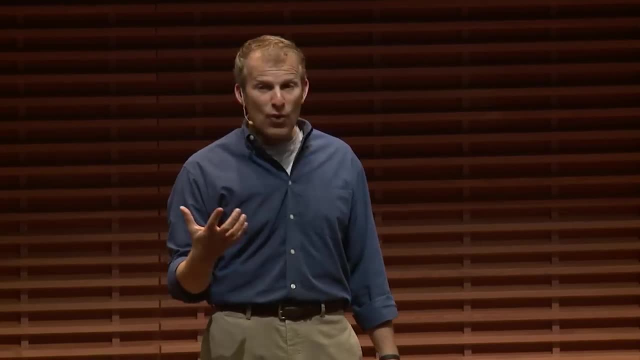 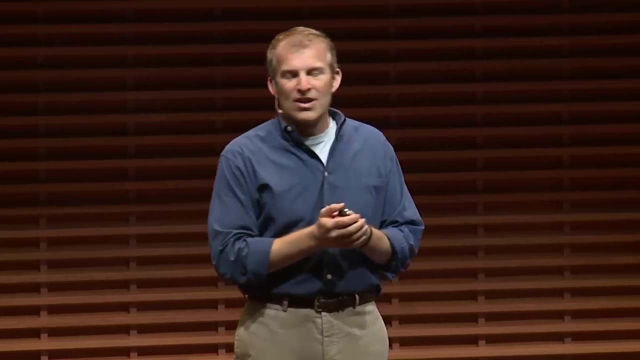 yes, uncomfortable. It feels very awkward, doesn't it? So what do we do? Now, a couple of you probably like watching somebody suffer, okay, But most of us don't. So what do we do? We sit there and we nod and we smile, or we disengage. 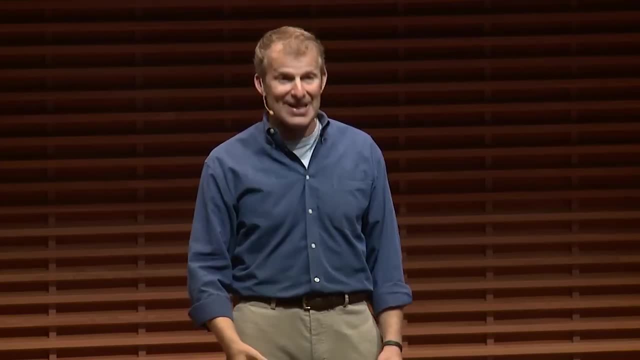 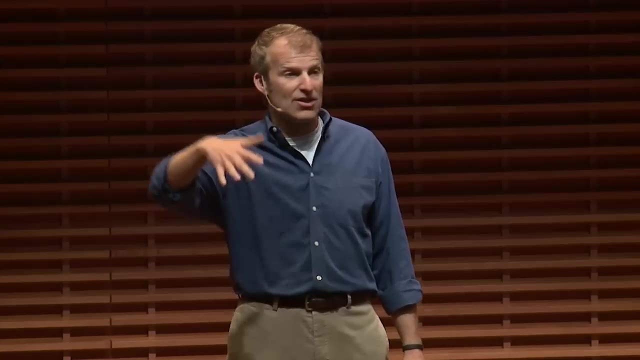 And to the nervous speaker looking out at his or her audience, seeing a bunch of people nodding or disengaged. that does not help, okay. So we need to learn to manage our anxiety, because fundamentally, your job as a communicator- rather, regardless of if it's planned or spontaneous- 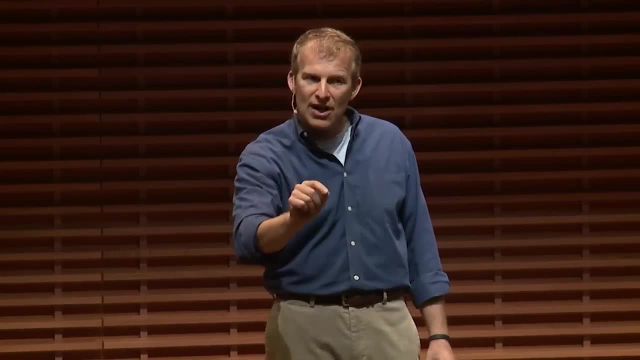 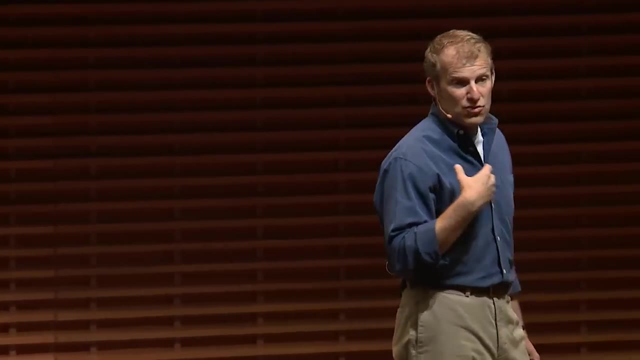 is to make your audience comfortable, Because if they're comfortable, it's actually about making you comfortable, Okay, So that's kind of what it's like watching someone suffer in a nervous situation余 Think up, Then we take the wrongsupport right. Have you ever thought about that? 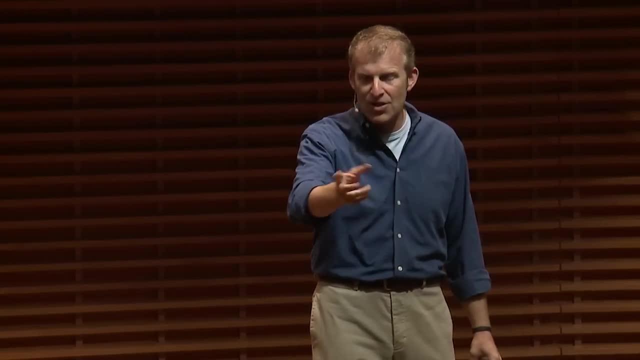 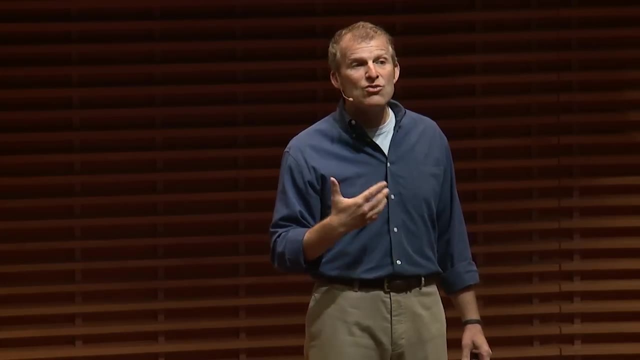 After you message somebody how you're feeling about him: R scared, S scared, I don't, I don't either, I don't either. Okay, So that's nice. What do we do, by the way? First off, you start by imagining where Ng is. 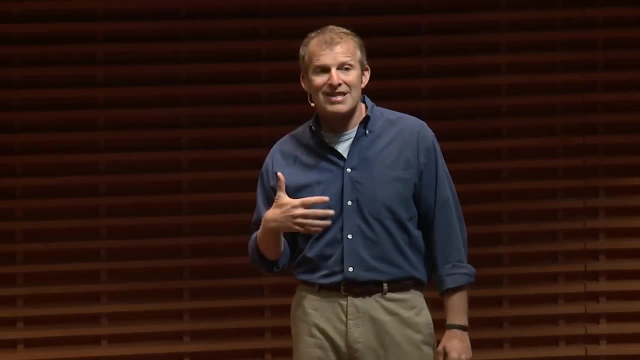 He's on the same page as the next speaker. I see Ng We policy show. We explain to the audience this. I see Ng This is me. We think Ng Where were you? No, Where's Ng? He's behind me. 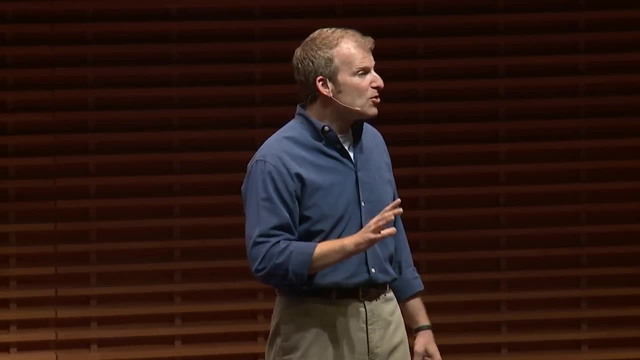 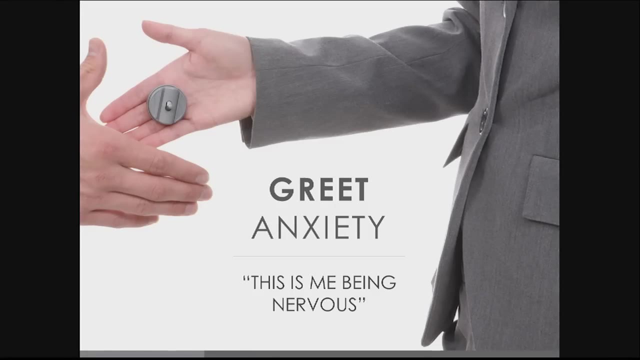 I see, Ng. Where are you begin to feel those anxiety symptoms? For most people, this happens in the initial minutes prior to speaking. In this situation, what happens is many of us begin to feel, whatever it is that happens to you. Maybe your stomach gets a little gurgly, Maybe your legs begin to shake, Maybe you 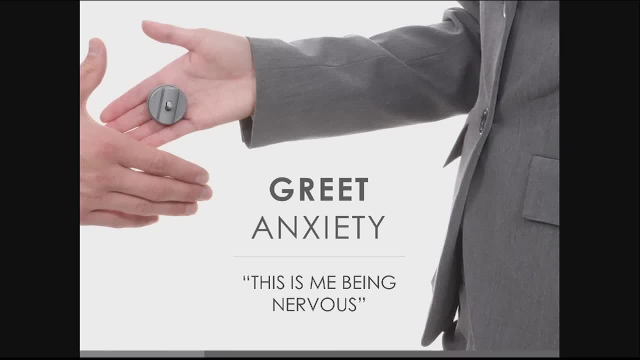 begin to perspire And then we start to say to ourselves: oh my goodness, I'm nervous. Uh-oh, they're going to tell I'm nervous, This is not going to go well, And we start spiraling out of control. So research on mindful attention tells us that if, when we begin to feel those anxiety, 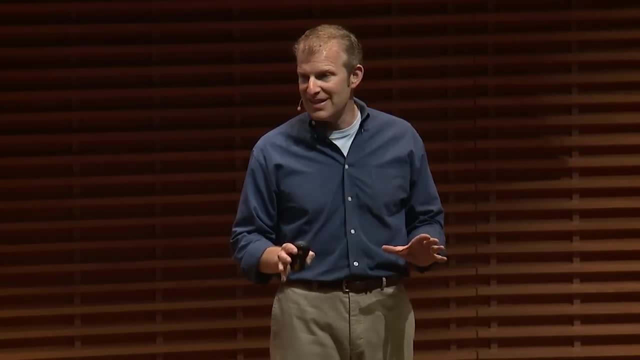 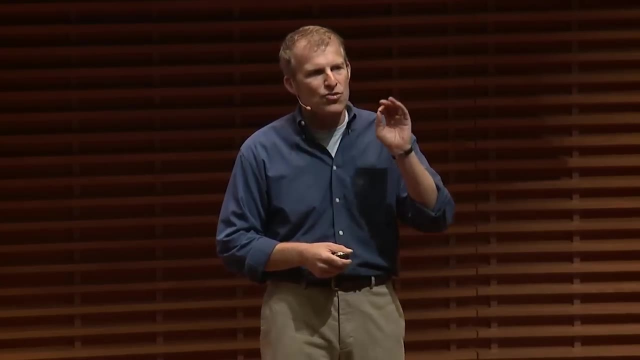 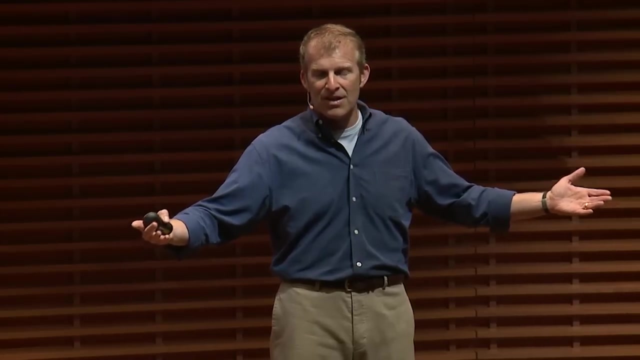 symptoms. we simply greet our anxiety and say, hey, this is me feeling nervous, I'm about to do something of consequence. And simply by greeting your anxiety and acknowledging it, that it's normal and natural- Heck, 85% of people tell us they have it- You actually can stem the tide of 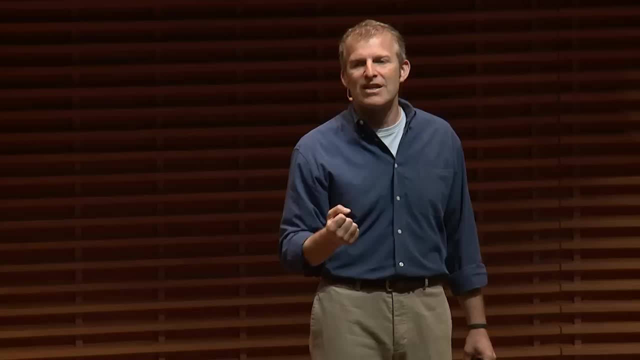 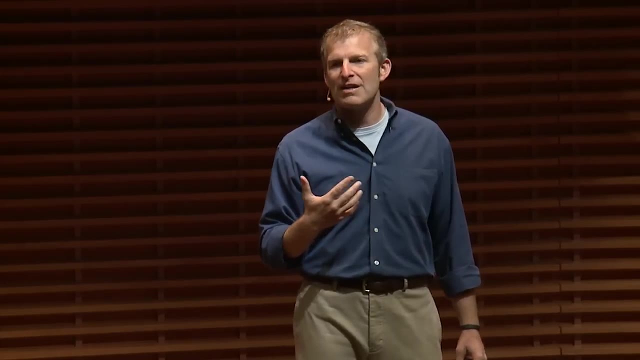 It can be a harsh message, but they have to be in a place where they can receive it. So it's incumbent on you, as a communicator, to help your audience feel comfortable, and we do that by managing our anxiety. So let me introduce you to a few techniques that I think you can use right away to help. 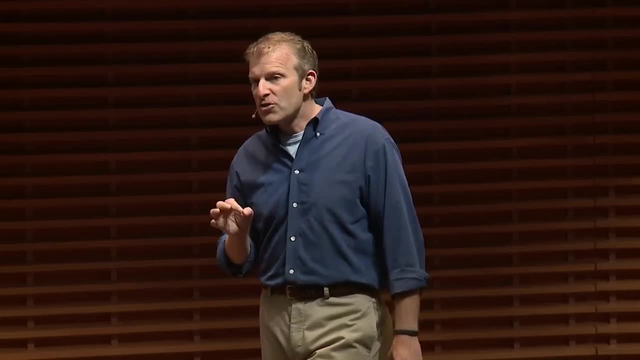 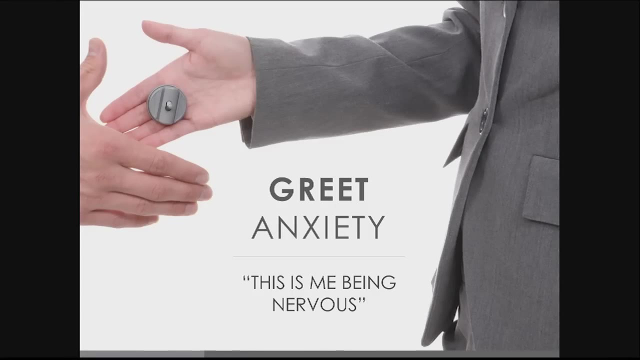 you feel more comfortable. The first has to do with when you begin to feel those anxiety symptoms. For most people, this happens in the initial minutes prior to speaking. In this situation, what happens is many of us begin to feel. whatever it is that happens. 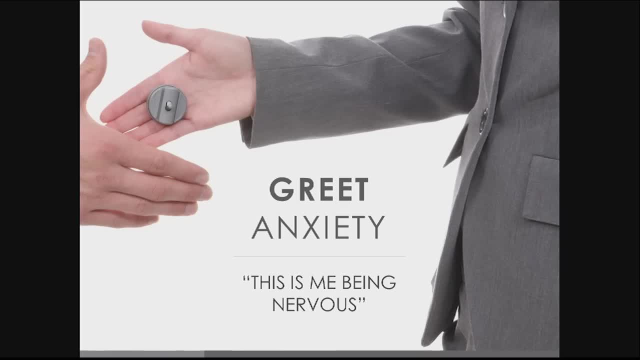 to you. Maybe your stomach gets a little gurgly, maybe your legs begin to shake, maybe you begin to perspire. And then we start to say to ourselves: oh my goodness, I'm nervous, uh-oh, they're going. 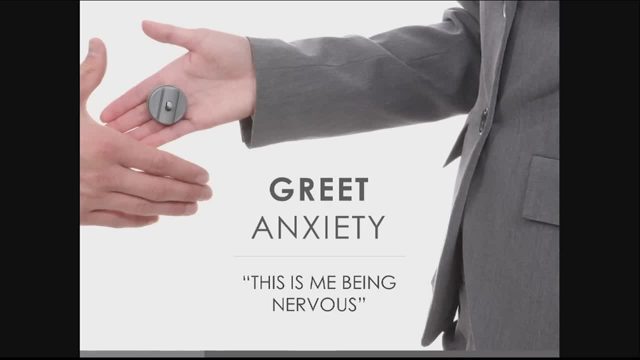 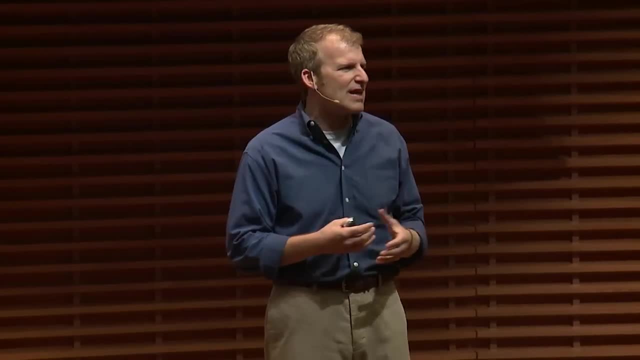 to tell: I'm nervous, this is not going to go well, and we start spiraling out of control. So research on mindful attention tells us that when we begin to feel those anxiety symptoms, we simply greet our anxiety and say, hey, this is me feeling nervous. 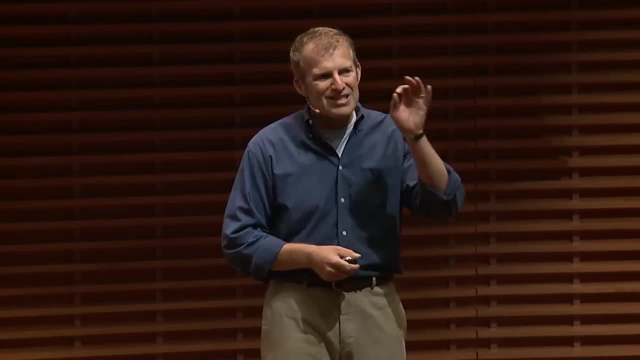 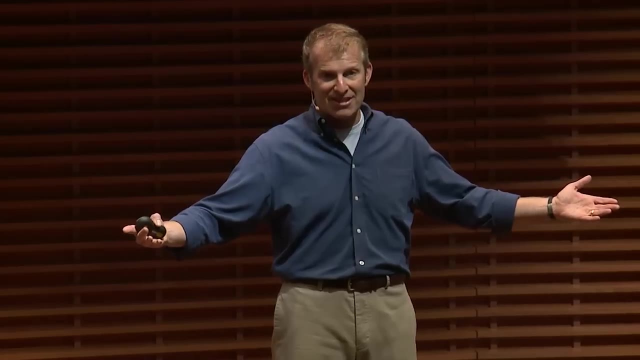 I'm about to do something of consequence, And simply by greeting your anxiety and acknowledging it that it's normal and natural- heck, 85% of people tell us they have it- you actually can stem the tide of that anxiety spiraling out of control. 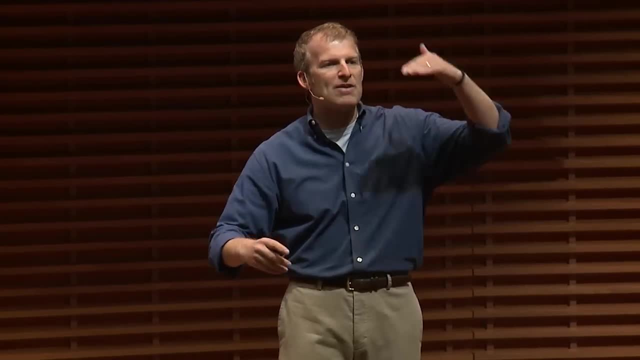 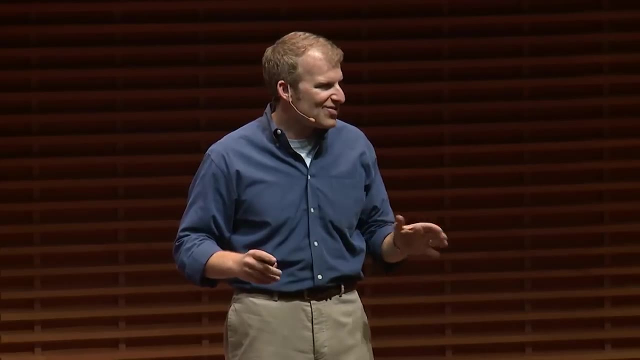 It's not necessarily going to reduce the anxiety, But it will stop it from spinning up. So the next time you begin to feel those anxiety signs, take a deep breath and say: this is me feeling anxious. I notice a few of you taking some notes. 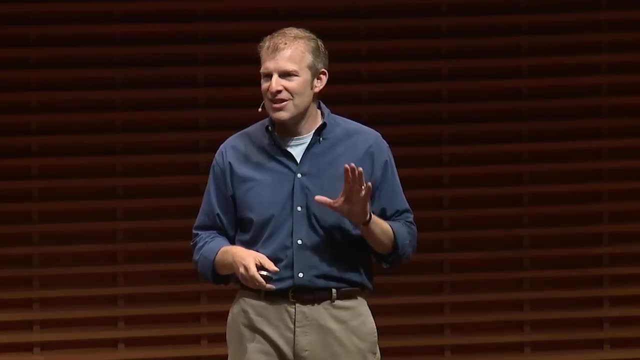 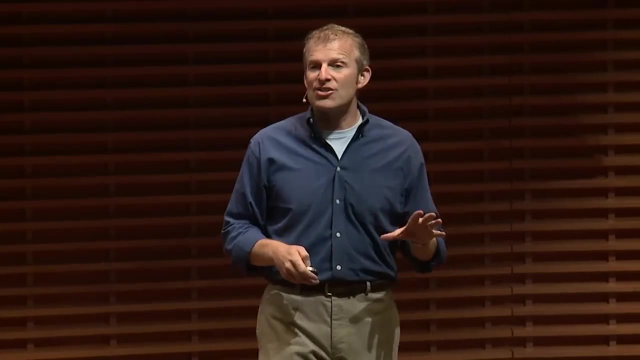 There's a handout that will come at the end that has everything that I'm supposed to say. Okay, I can't guarantee I'm going to say it, but you'll have it there In addition to this approach, a technique that works very well, and this is a technique. 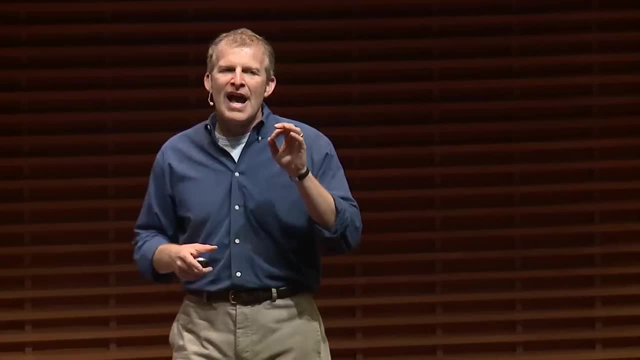 that I helped do some research on way back when I was in graduate school. Okay, This is a technique that works very well and this is a technique that I helped do some research on way back when I was in graduate school. Has to do with reframing how you see the speaking situation. 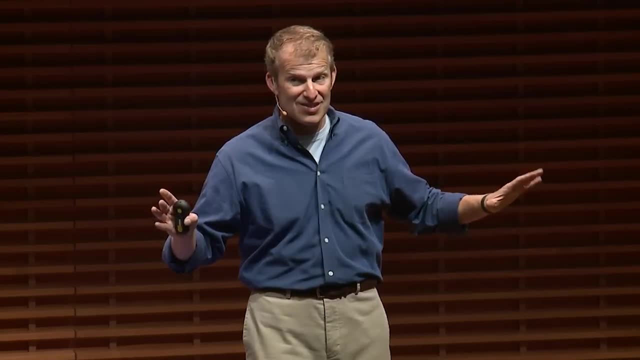 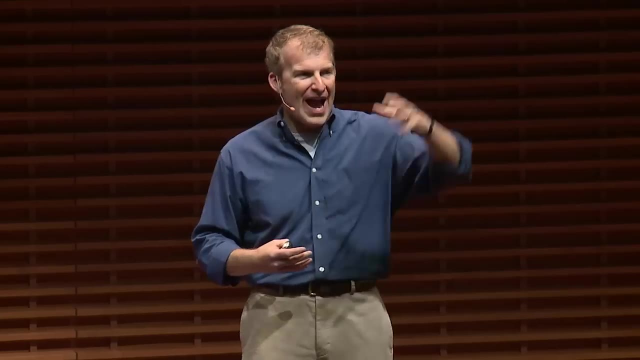 Most of us, when we are up presenting- planned or spontaneous- we feel that we have to do it right And we feel like we are performing. How many of you have ever acted, done singing or dancing? I'm not going to ask for performances now. 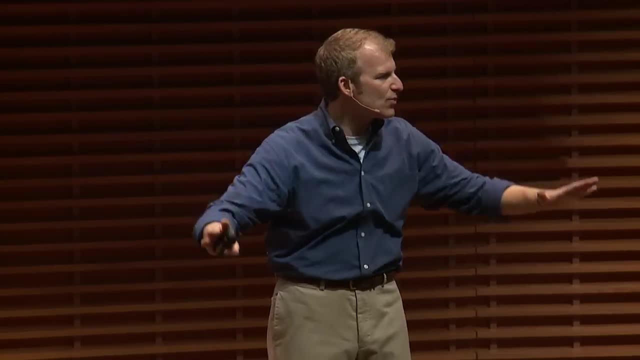 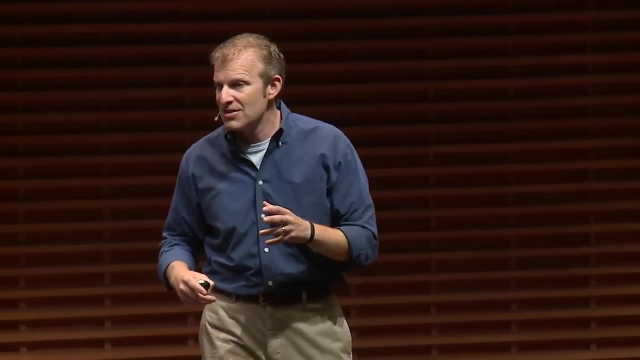 that anxiety spiraling out of control. It's not necessarily the case that you're not feeling nervous. It's not necessarily going to reduce the anxiety, but it will stop it from spinning up. So the next time you begin to feel those anxiety signs, take a deep breath and say: this is me. 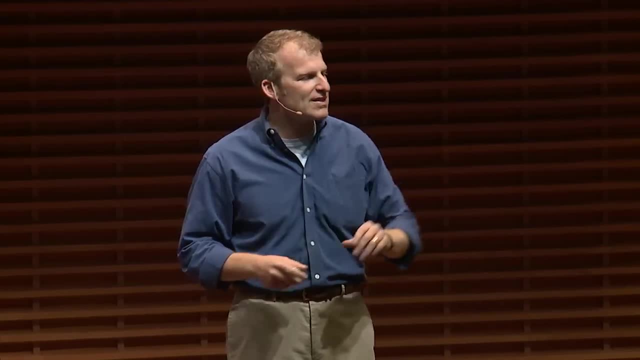 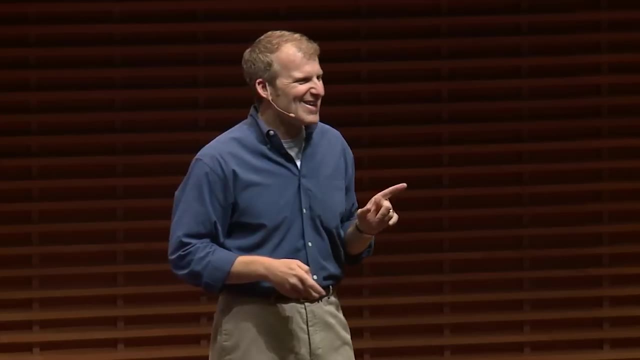 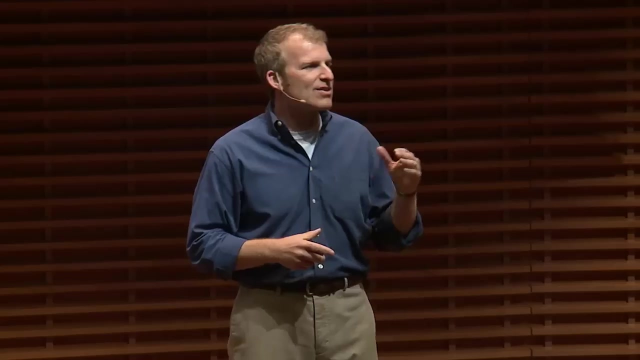 feeling anxious. I notice a few of you taking some notes. There's a handout that will come at the end that has everything that I'm supposed to say. Okay, Can't guarantee I'm going to say it, but you'll have it there. In addition to this approach, a technique that works very well, and this is a 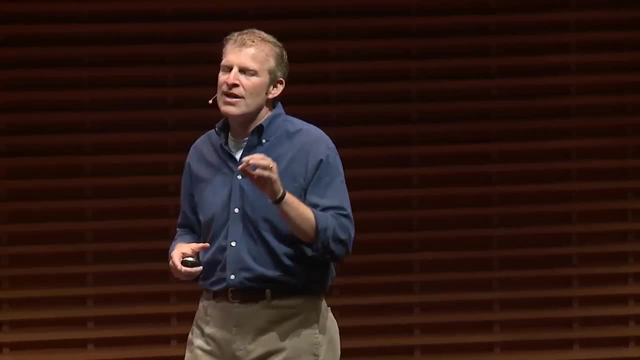 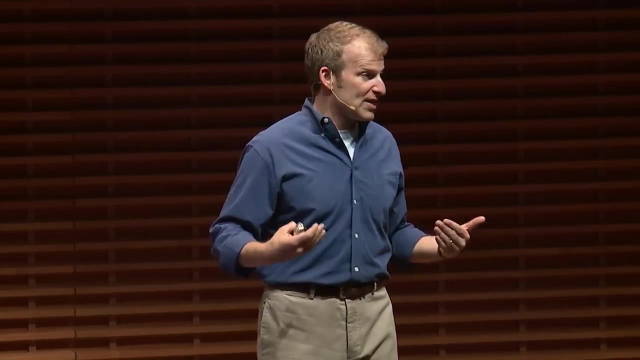 technique that I helped do some research on is the technique that I use to help people feel better, And it's a technique that I used to do research on way back when I was in graduate school. Has to do with reframing how you see the speaking situation Most of us when we are up. 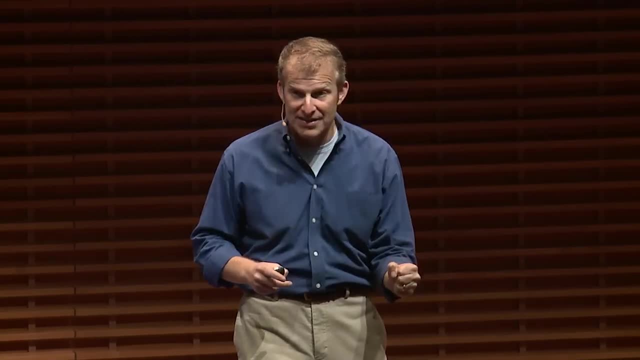 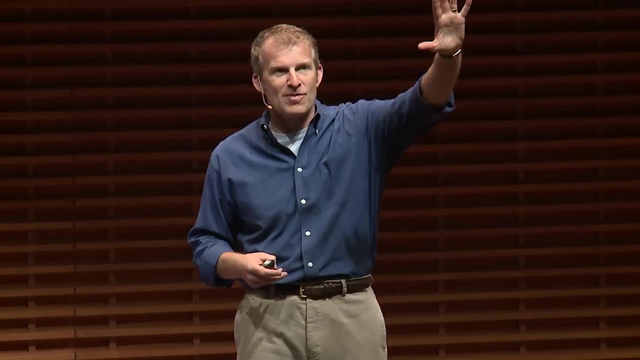 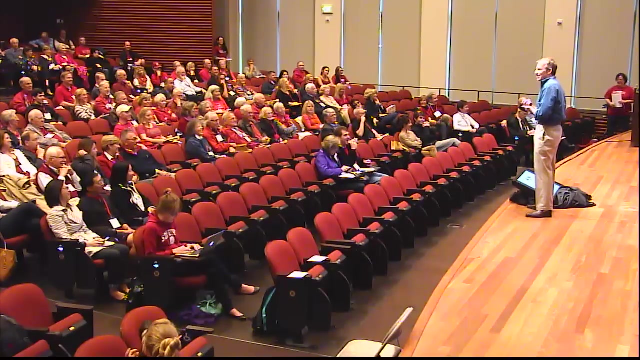 presenting, planned or spontaneous. we feel that we have to do it right And we feel like we are performing. How many of you have ever acted, done singing or dancing? I'm not going to ask for performances now. Okay, Many of you have. We should note that we could do next year. maybe a talent. 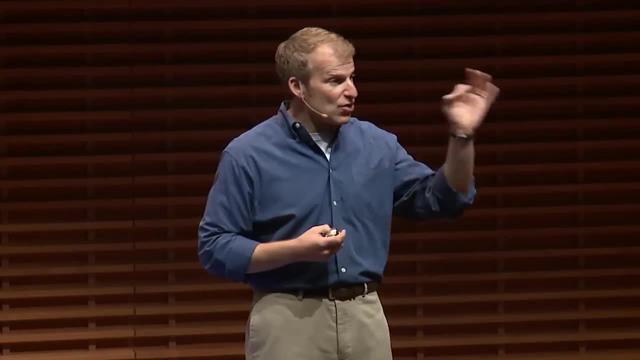 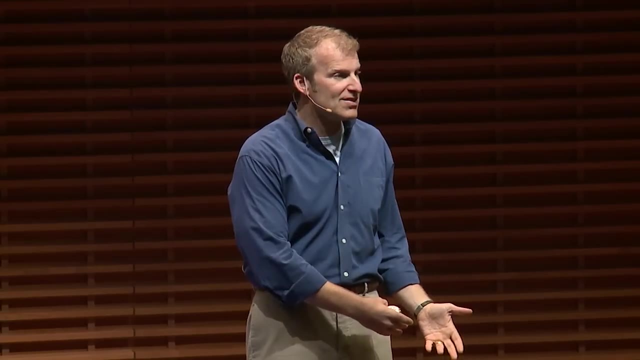 show of alums. It looks like we got the talent there. That's great. So when you perform, you know that there's a right way and a wrong way to do it. If you don't hit the right note or your right line at the right time at the right place, you've made a mistake. It messes. 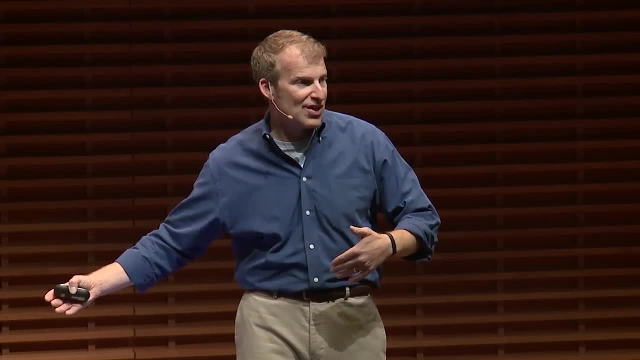 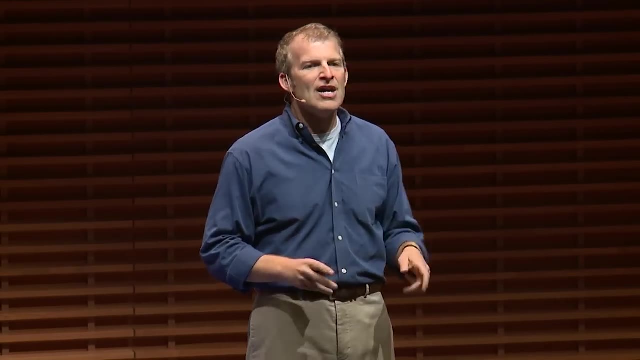 up the audience. It messes up the people on stage, But when you present, there is no right way. There's certainly better and worse ways, but there is no one right way. So we need to look at presenting as something other than performance, And what I'd like to suggest is what we need to. 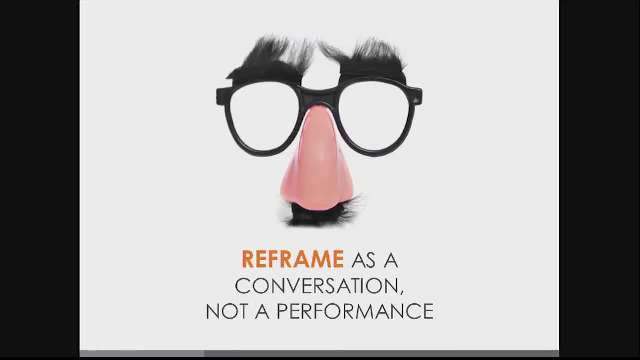 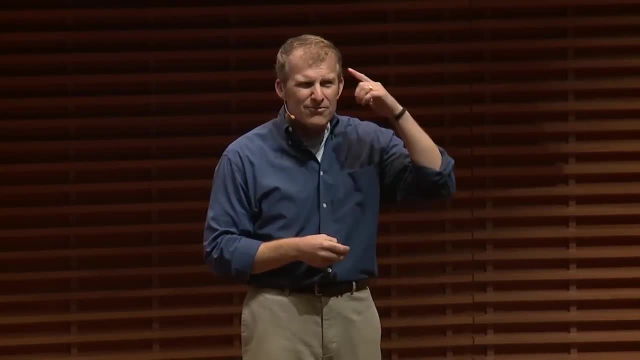 see this as is a conversation. We need to see this as a conversation. We need to see this as a conversation. Right now, I'm having a conversation with 100 plus people, rather than saying I'm performing for you. But it's not enough just to say this is a conversation. I want to give you some. 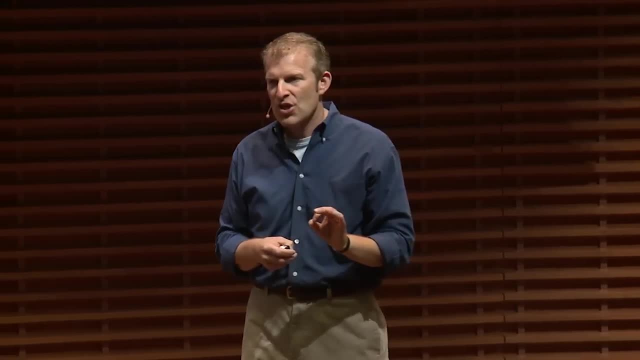 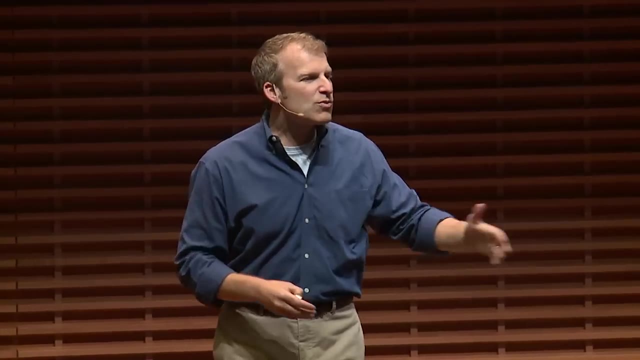 concrete things you can do. First, start with questions. Questions, by their very nature, are dialogic. They're two-way. What was one of the very first things I did here for you? I had you count the number of Fs and raise your hands. I asked you a question. 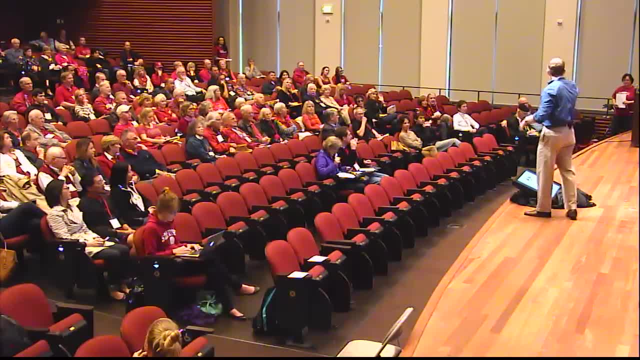 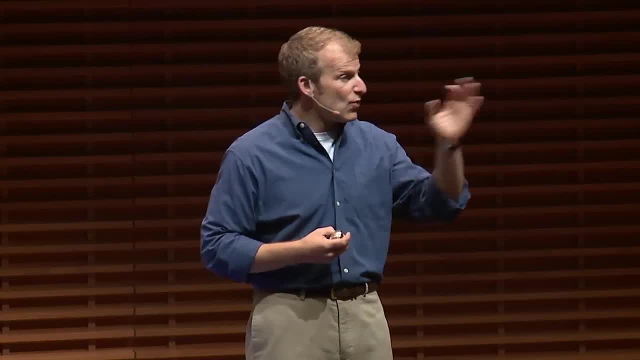 Okay, Many of you have. We should note that we could do next year maybe a talent show of alums. It looks like we got the talent there. That's great. So when you perform, You know that there's a right way and a wrong way to do it. 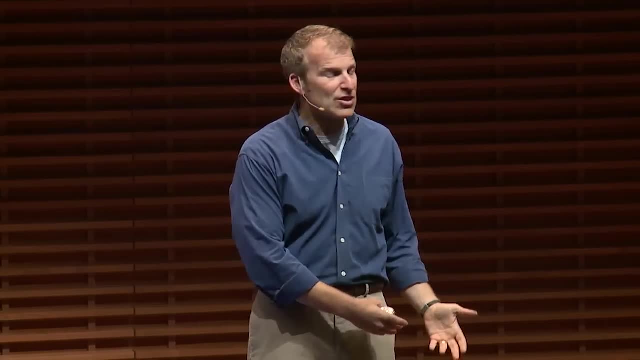 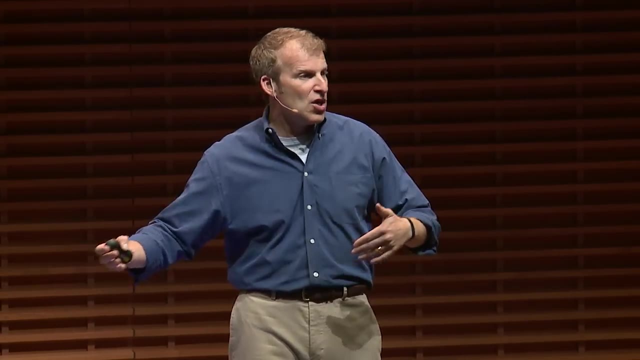 If you don't hit the right note or your right line at the right time at the right place, you've made a mistake. It messes up the audience, It messes up the people on stage, But when you present, there is no right way. 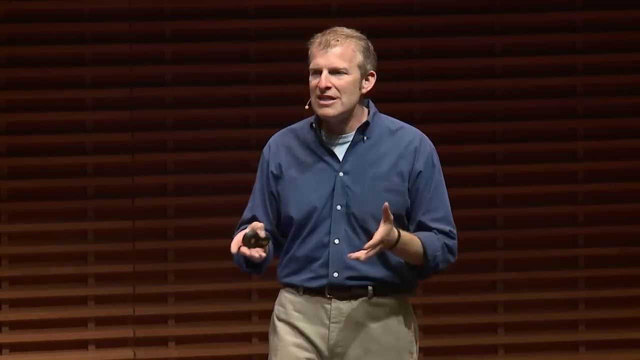 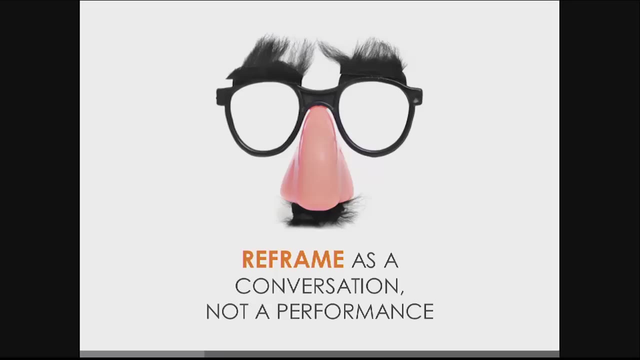 There's certainly better and worse ways, but there is no one right way, So we need to look at presenting as something other than performance, And what I'd like to suggest is what we need to see this as is a conversation. Right Right now, I'm having a conversation with a hundred plus people, rather than saying I'm 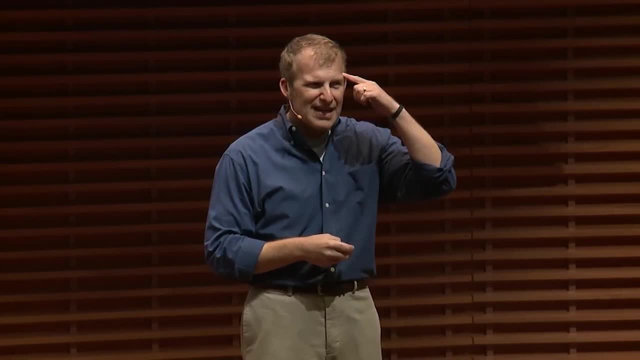 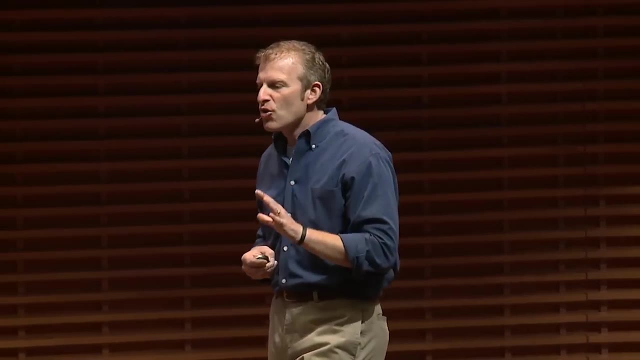 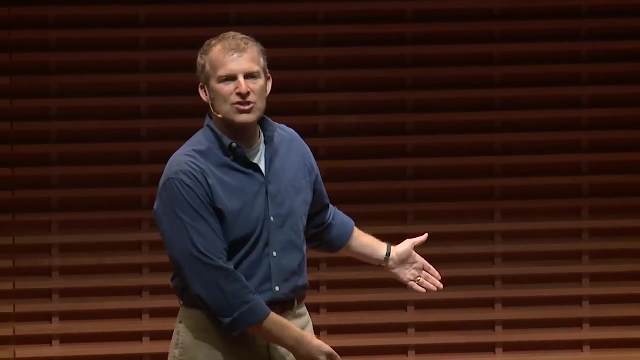 performing for you. But it's not enough just to say this is a conversation. I want to give you some concrete things you can do. First, start with questions. Questions, by their very nature, are dialogic. They're two way. What was one of the very first things I did here for you? 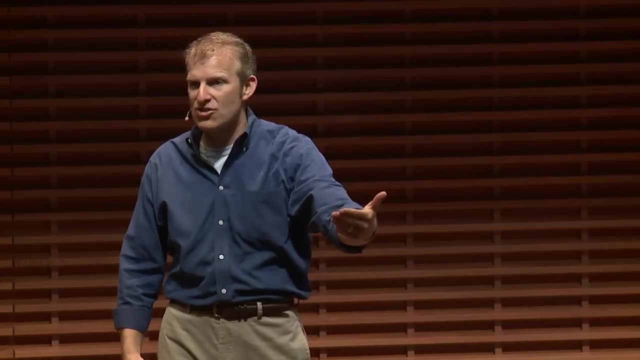 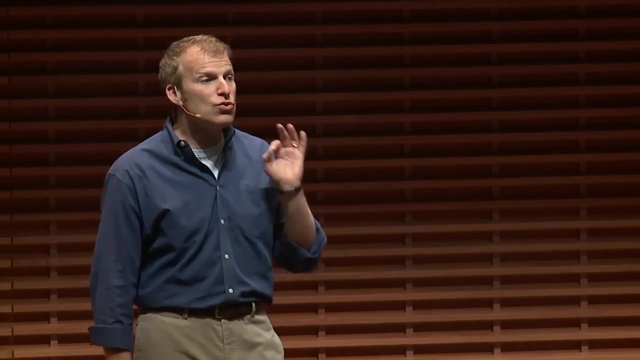 I had you count the number of Fs and raise your hands. I asked you a question That gets your audience involved. It makes it feel to me, as the presenter, as if we are in conversation. So use questions. They can be rhetorical, They can be polling. 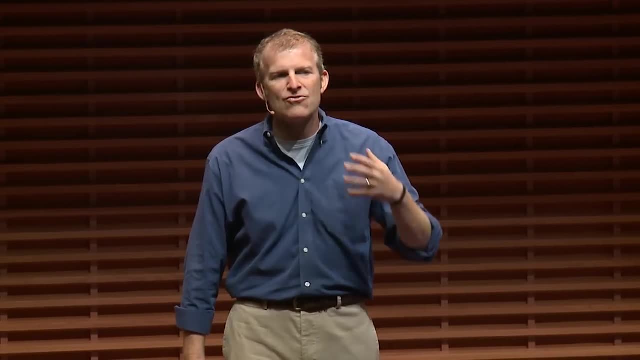 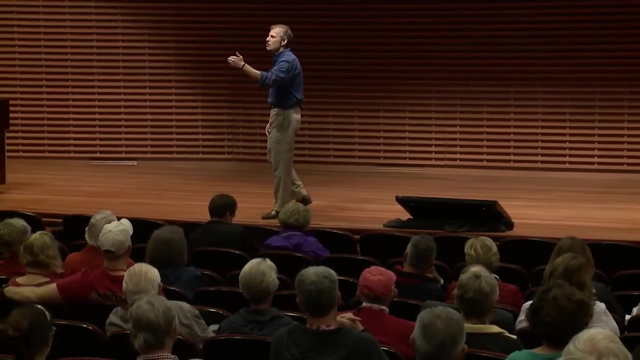 Perhaps I actually want to hear information from you. In fact, I use questions when I create an outline for my presentations, Rather than writing bullet points. I list questions that I'm going to answer And that puts me in that conversational mode. 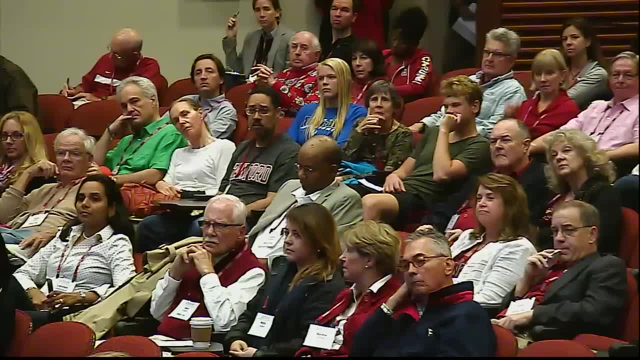 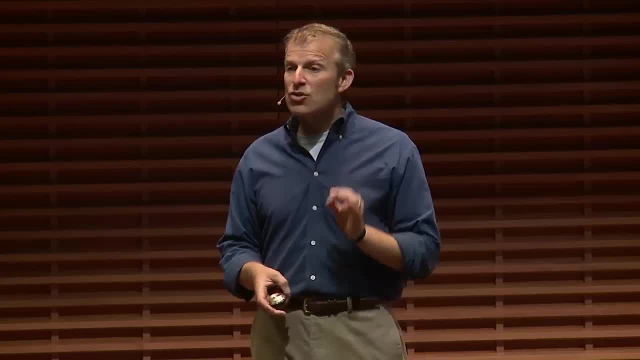 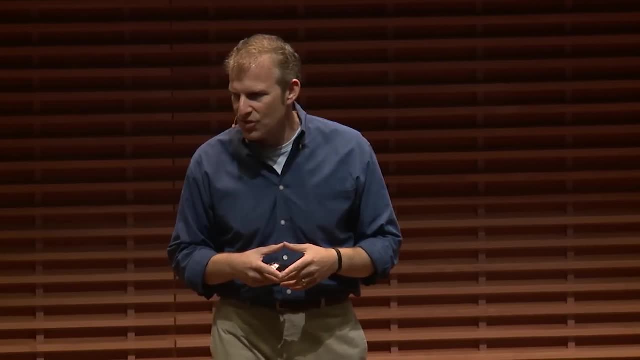 If you were to look at my notes for today's talk, you'll see it's just a series of questions. Right now I'm answering the question: How do we manage our anxiety? Beyond questions, another very useful technique for making us conversational is to use conversational language. 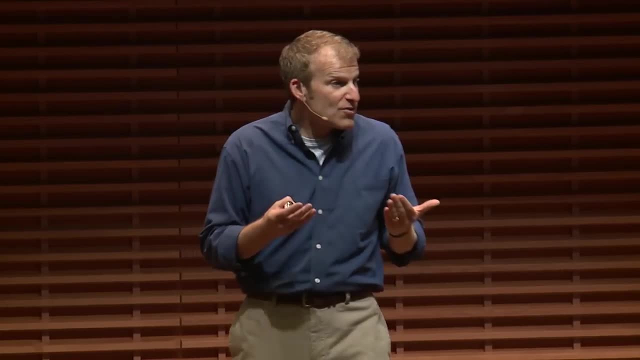 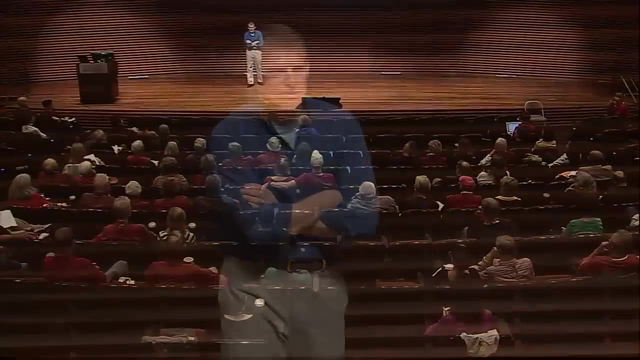 Many nervous speakers distance themselves physically. If you've ever seen a nervous speaker present, he or she will say something like this: Welcome, I am really excited to be here with you. They pull as far away from you as possible because you threaten us speakers. 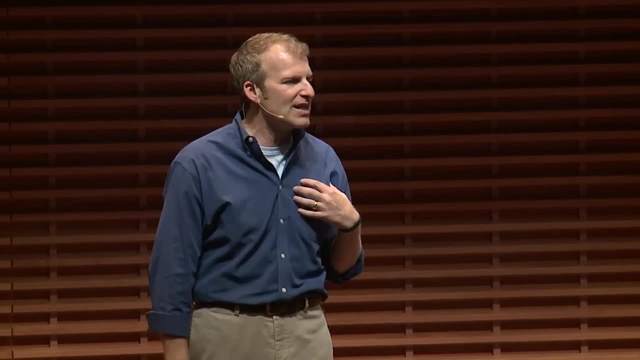 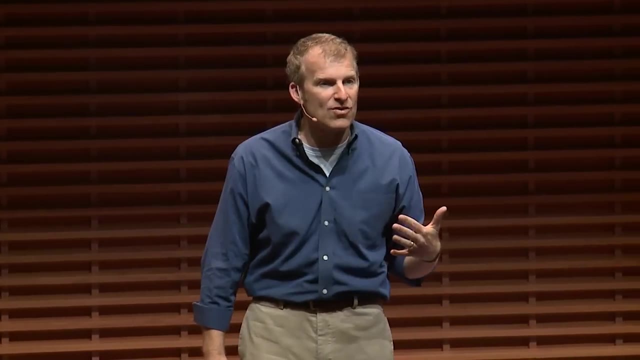 That gets your audience involved. It makes it feel to me, as the presenter, as if we are in conversation. So use questions. They can be rhetorical, They can be polling. Perhaps I actually want to hear information from you. In fact, I use questions when I create an. 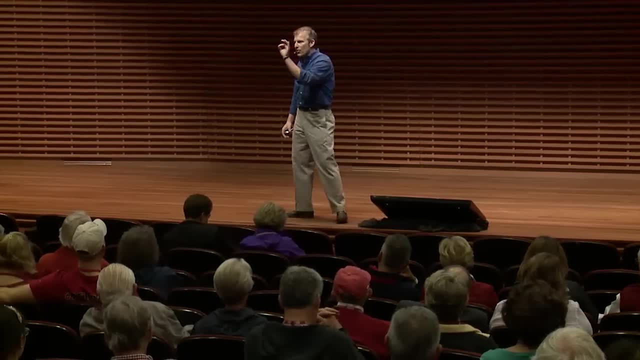 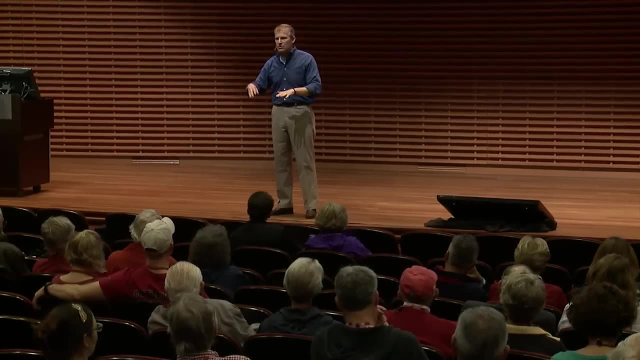 outline for my presentations, Rather than writing bullet points. I list questions that I'm going to answer And that puts me in that conversational mode. If you were to look at my notes for today's talk, you'll see it's just a series of questions. Right now I'm answering the 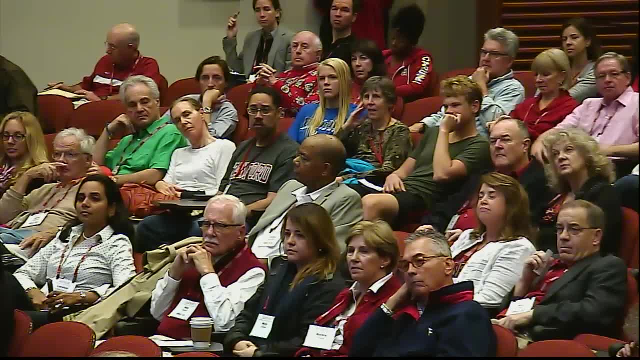 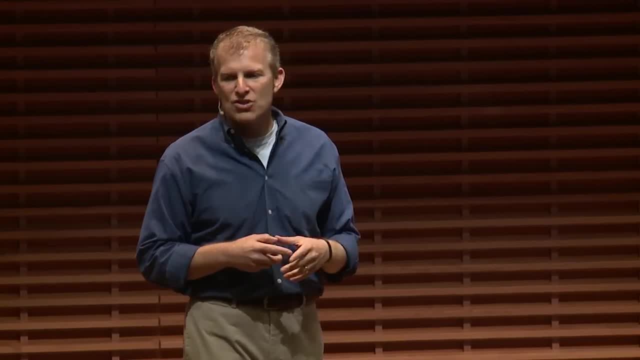 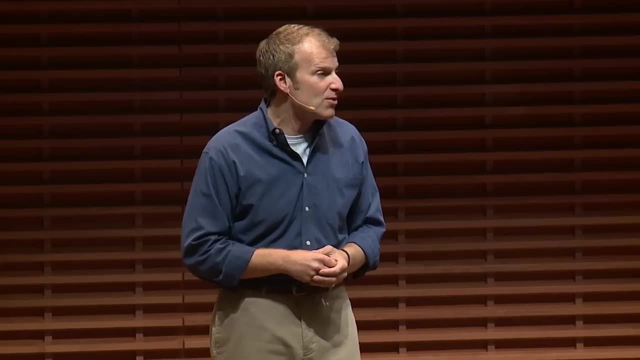 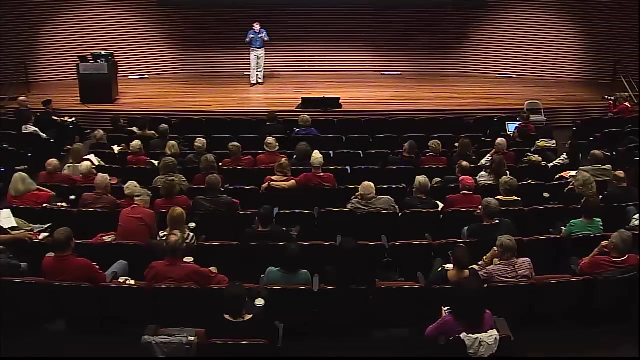 question: how do we manage our anxiety? Beyond questions, another very useful technique for making us conversational is to use conversational language. Many nervous speakers distance themselves physically. If you've ever seen a nervous speaker present, he or she will say something like this: Welcome, I am really excited to be here with you. They pull as far away from. 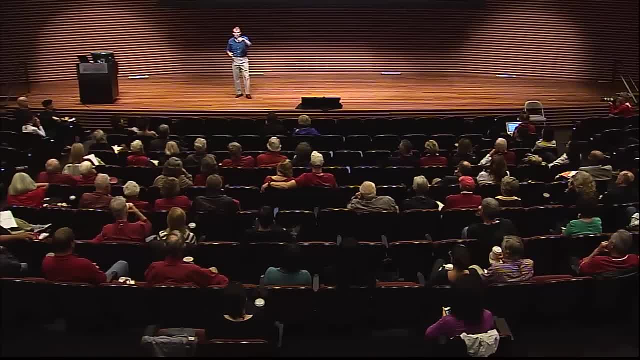 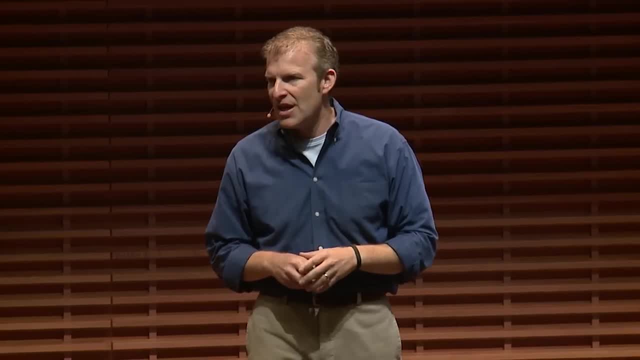 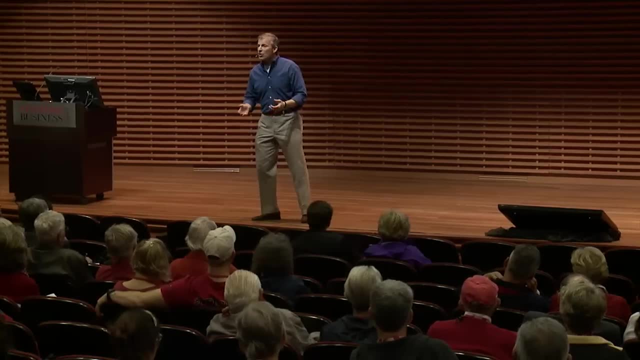 you as possible, because you threaten us speakers, You make us nervous, so we want to be here with you. We do the same thing linguistically. We use language that distances ourselves. It's not unusual to hear a nervous speaker say something like: one must consider the ramifications, or today we're 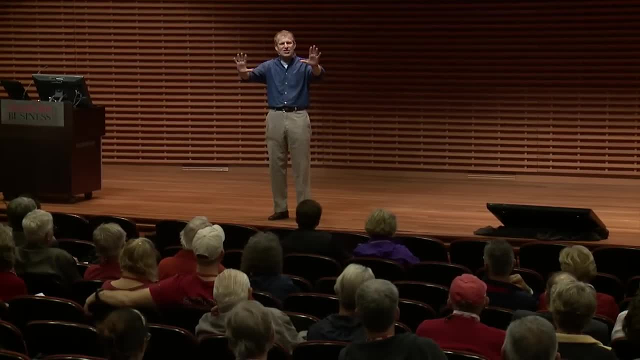 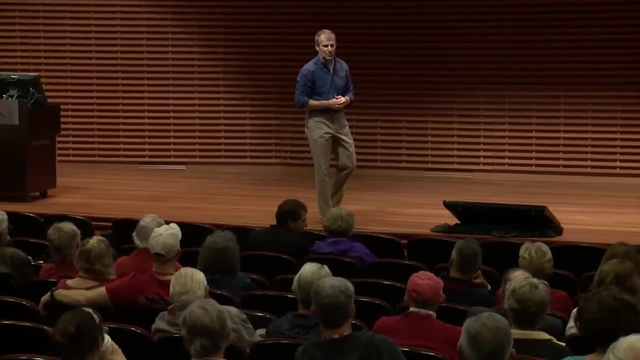 going to cover step one, step two, step three. That's very distancing language. To be more conversational, use conversational language Instead of one must consider: say: this is important to you We all need to be concerned with. do you hear that? inclusive conversational language? It has to. 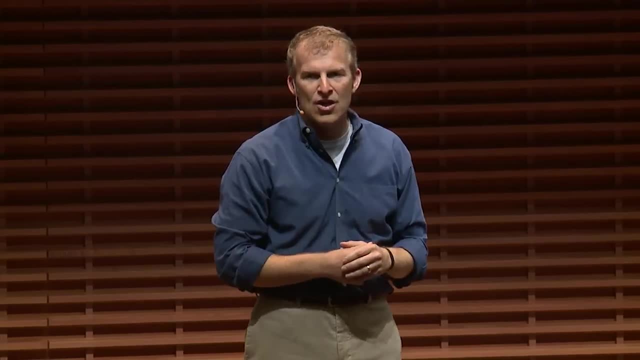 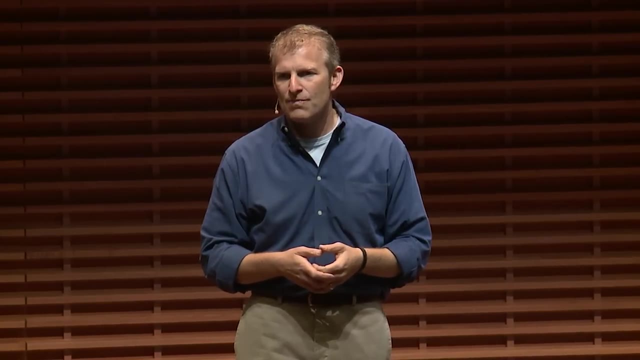 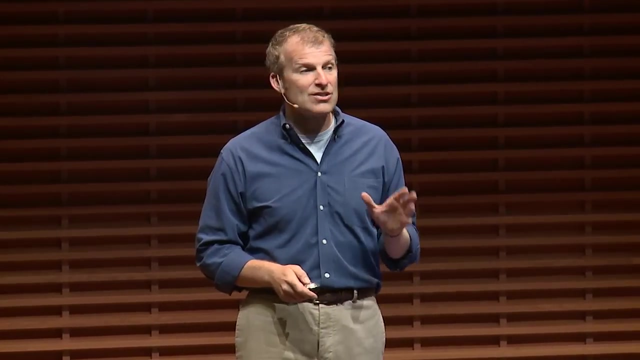 be in our pronouns Instead of step one, step two, step three. First, what we need to do is this. The second thing you should consider is here: Use conversational language, So being conversational can also help you manage your anxiety. The third technique I'd like to share is research that I 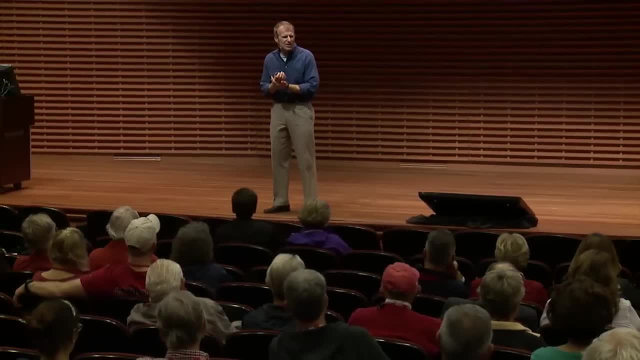 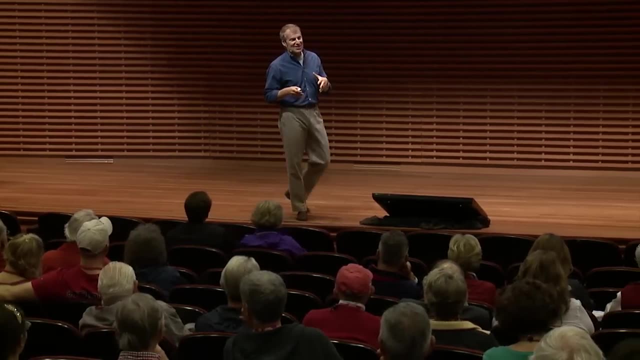 actually started. when I was an undergraduate here I was very fortunate to study with Phil Zimbardo of the Stanford Prison Experiment fame. Many people don't know that Zim actually was instrumental in the development of the Stanford Prison Experiment. He was the first person to 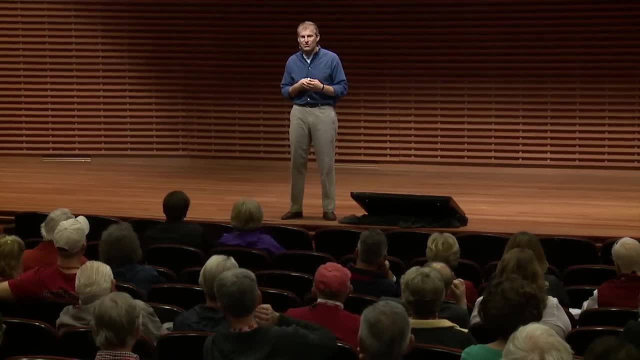 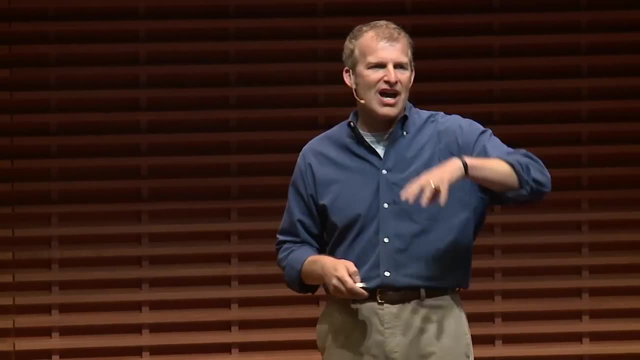 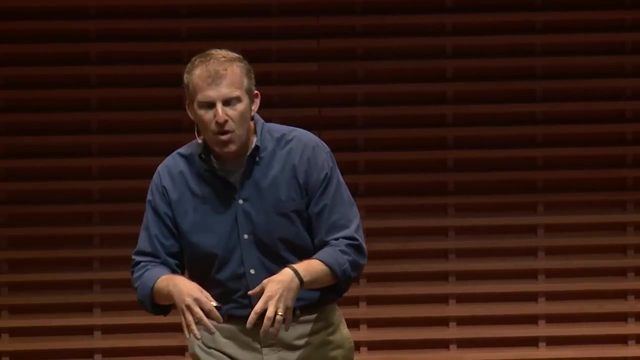 be instrumental in starting one of the very first shyness institutes in the world, and especially in the country, And I did some research with him that looked at how your orientation to time influences how you react, And what we learned is if you can bring yourself into the present moment rather than 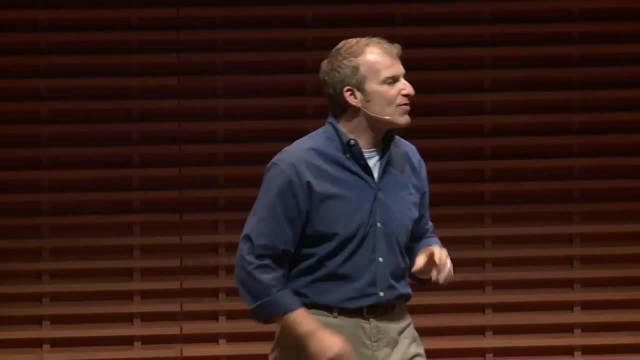 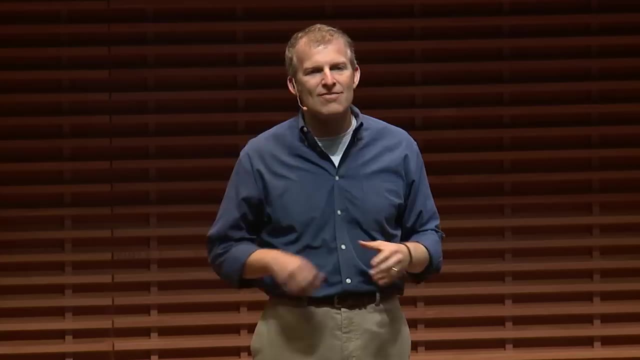 You make us nervous, So we want to get away from you. All right, Let's get away from you. We do the same thing linguistically. We use language that distances ourselves. It's not unusual to hear a nervous speaker say something like: one must consider the 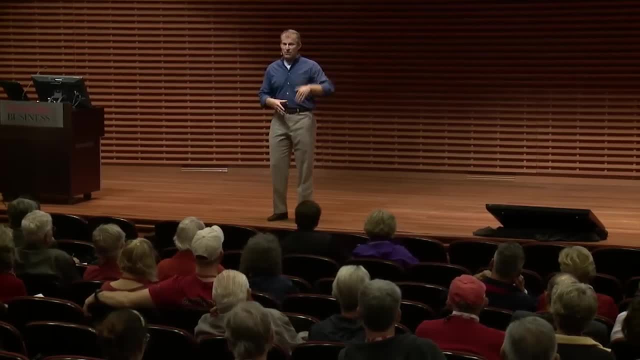 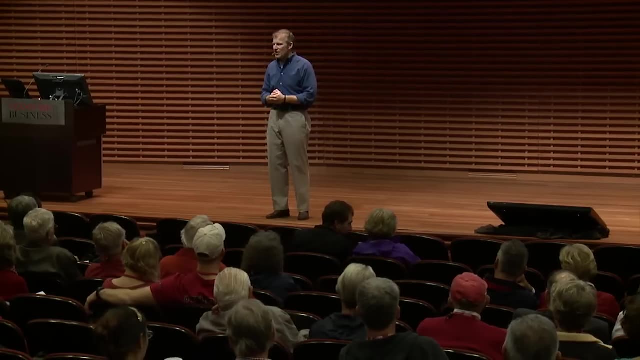 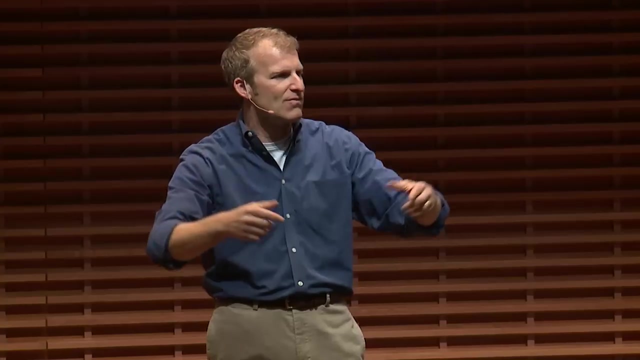 ramifications, or today we're going to cover step one, step two, step three. That's very distancing language. To be more conversational, use conversational language Instead of one must consider, say: this is important to you We all need to be concerned with. do you hear that inclusive conversational language. 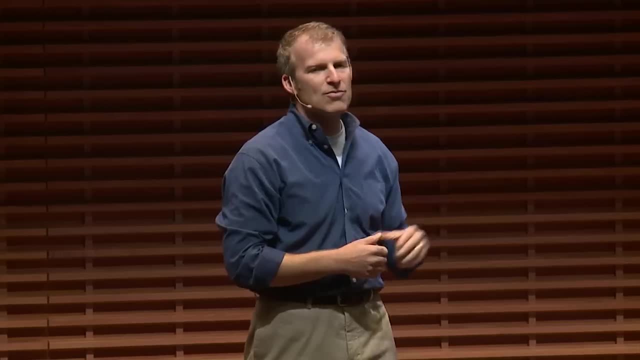 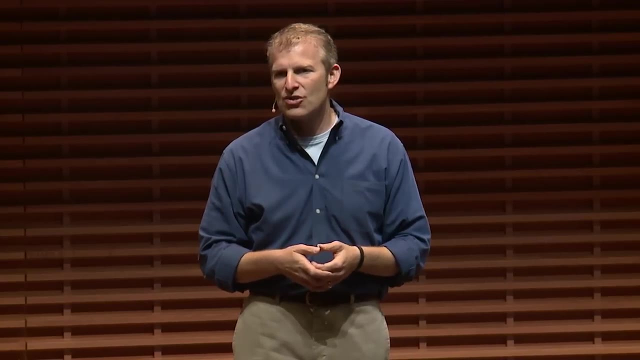 Has to do with the pronouns. Instead of step one, step two, step three. First, what we need to do is this. The second thing you should consider is here: Use conversational language, So being conversational can also help you manage your anxiety. 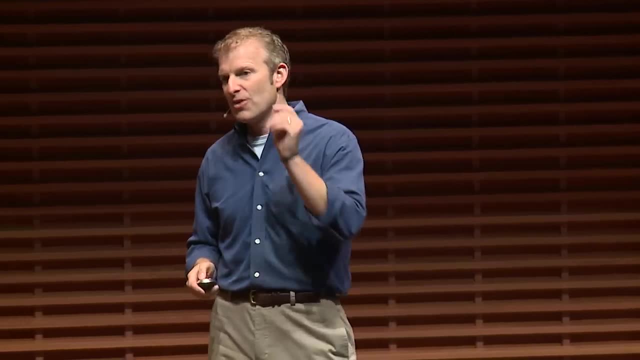 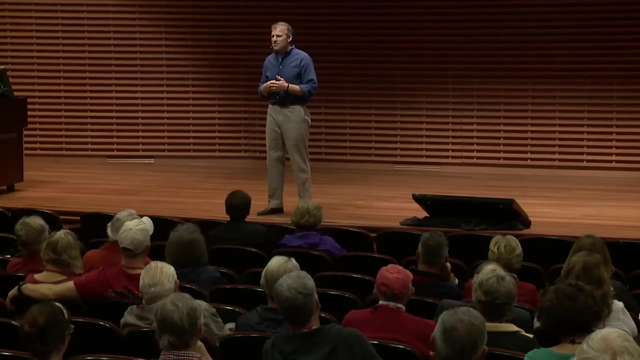 The third technique I'd like to share is research that I actually started when I was an undergraduate here. I was very fortunate to study with Phil Zimbardo of the Stanford Prison Experiment fame. Many people don't know that Zim actually was instrumental in the development of the Stanford Prison Experiment. 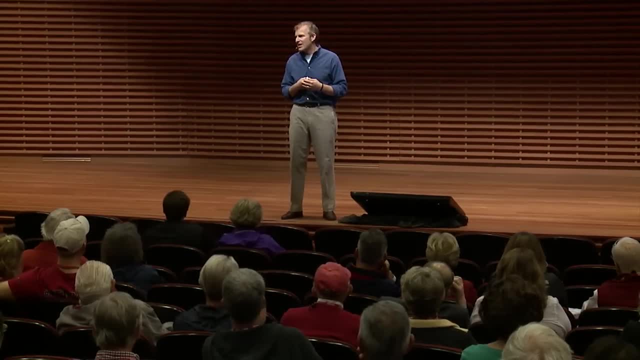 I was very fortunate to study with Phil Zimbardo of the Stanford Prison Experiment fame. Many people don't know that Zim actually was instrumental in the development of the Stanford Prison Experiment and starting one of the very first shyness institutes in the world. 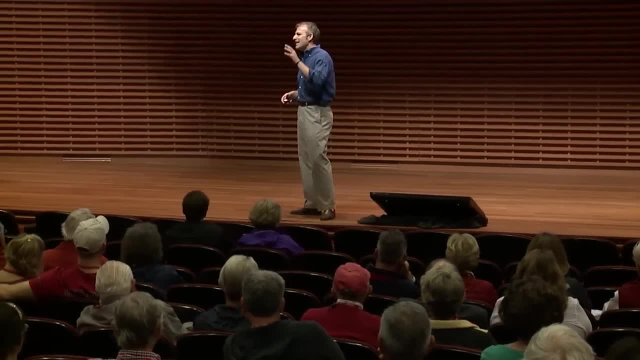 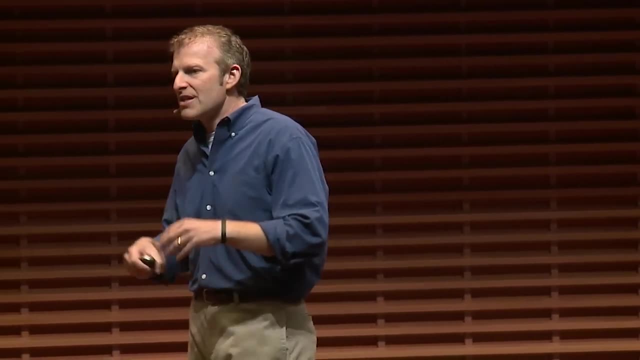 and especially in the country, And I did some research with him that looked at how your orientation to time influences how you react, And what we learned is if you can bring yourself into the present moment rather than being worried about the future consequences. 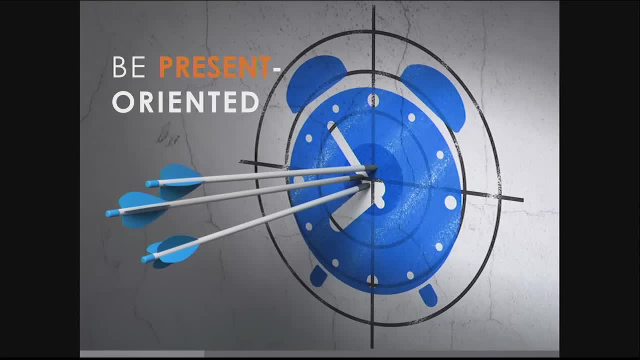 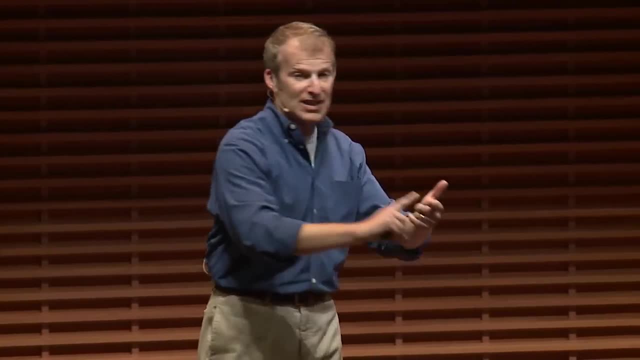 you can actually be less nervous. Most of us, when we present, are worried about the future consequences. My students are worried they're not going to get the right grade. Some of you are worried you might not get the funding, you might not get the support. 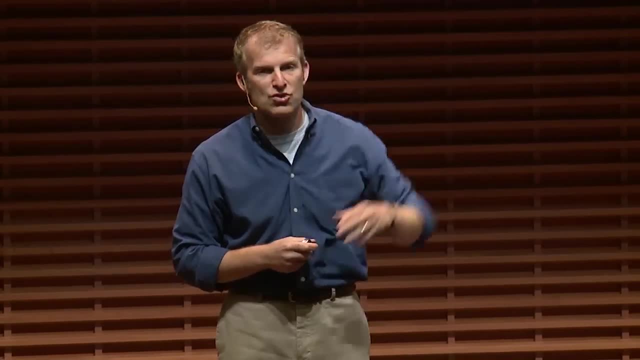 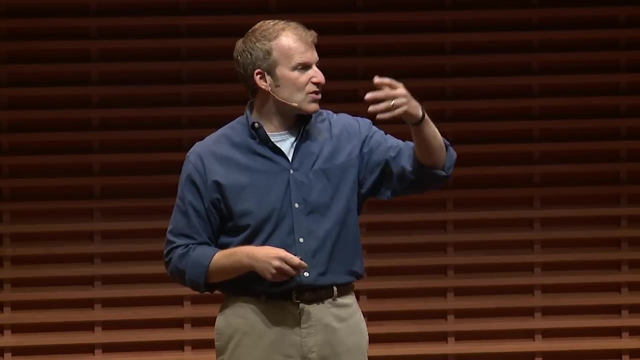 you might not get the laughs that you want. All of those are future states. So if we can bring ourselves into the present moment, we're not going to be as concerned about those future states and therefore we'll be less nervous. There are lots of ways to become present-oriented. 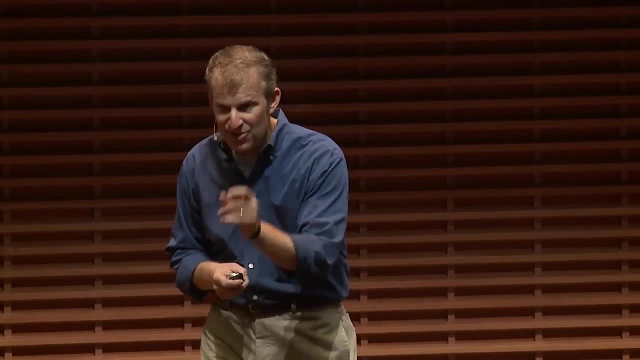 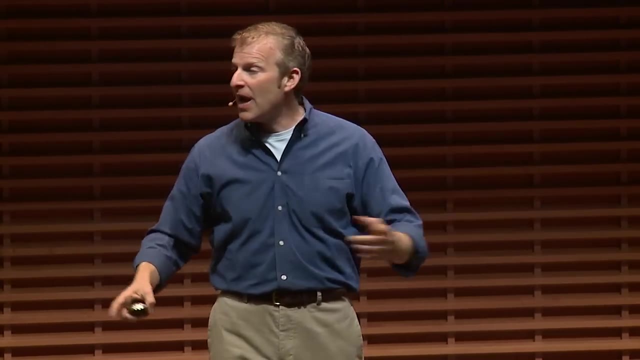 I know a professional speaker. He's paid $10,000 an hour to speak. It's a good gig. He gets very nervous. He's up in front of crowds of thousands. Behind the stage, what he does is a hundred push-ups. 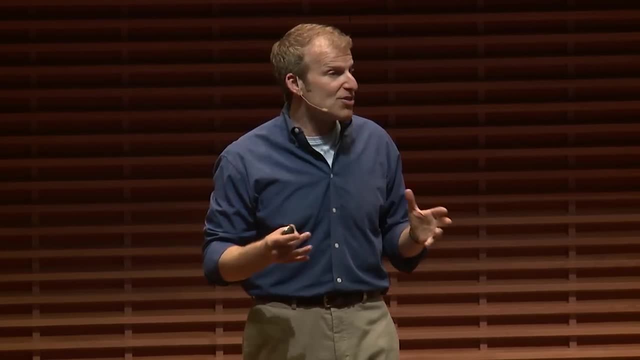 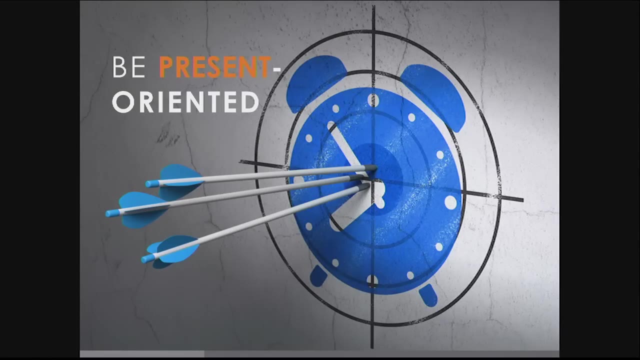 being worried about the future consequences, you can actually be less nervous. Most of us, when we present, are worried about the future consequences. My students are worried they're not going to get the right grade. Some of us are worried they're not going to get the right grade. Some of us are. 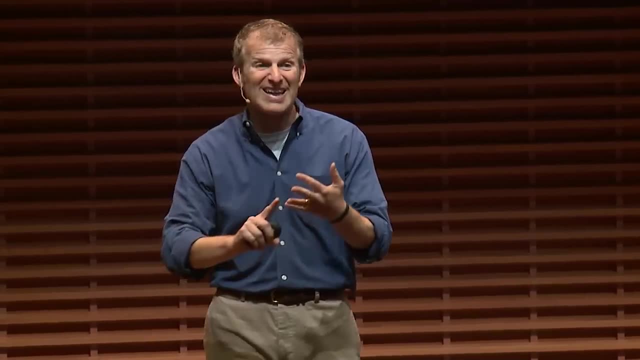 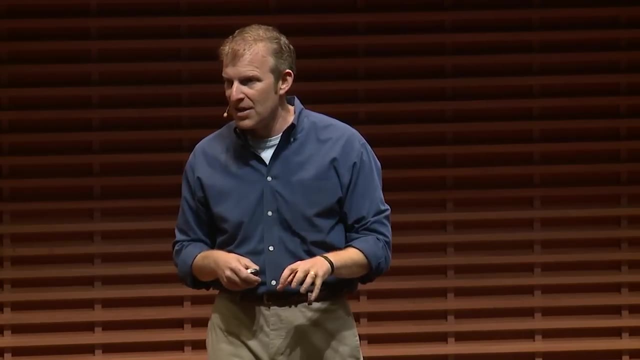 worried they're not going to get the right grade. So if you are worried, you might not get the funding, you might not get the support, you might not get the laughs that you want. All of those are future states. So if we can bring ourselves into the present moment, we're not going to be as 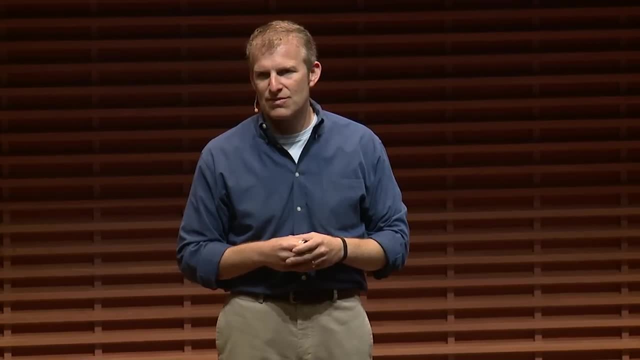 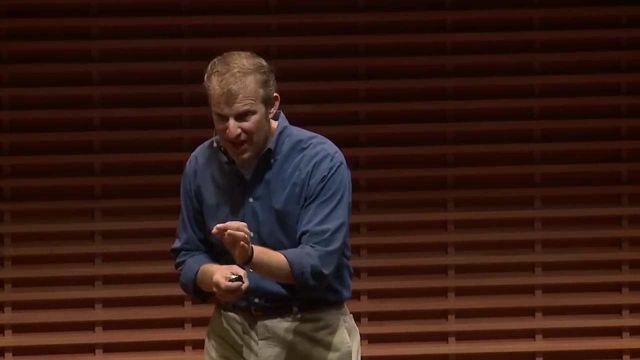 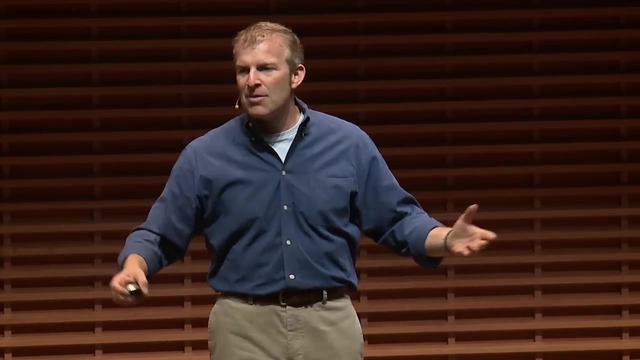 concerned about those future states and therefore we'll be less nervous. There are lots of ways to become present-oriented. I know a professional speaker. He's paid $10,000 an hour to speak. It's a good gig. He gets very nervous. He's up in front of crowds of thousands Behind the 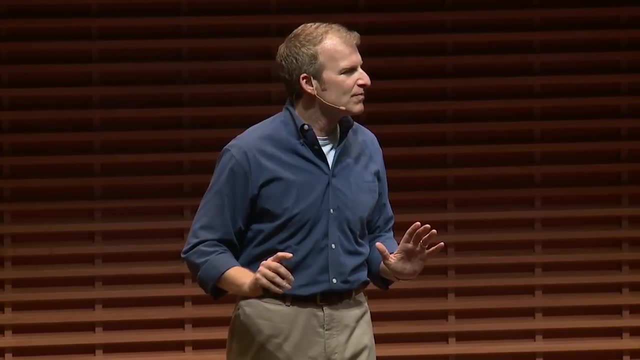 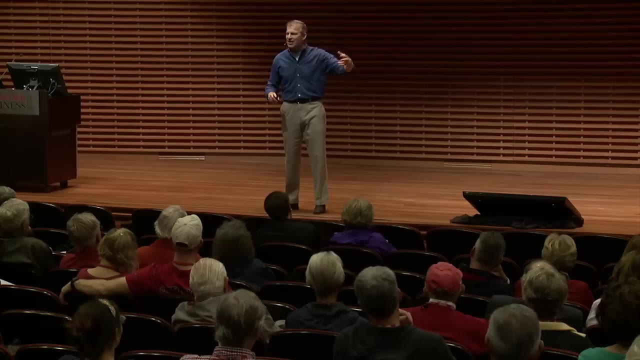 what he does is a hundred push-ups right before he comes out. You can't be that physically active and not be in the present moment. Now I'm not recommending all of us go to that level of exertion, because he starts out of breath and sweaty right. 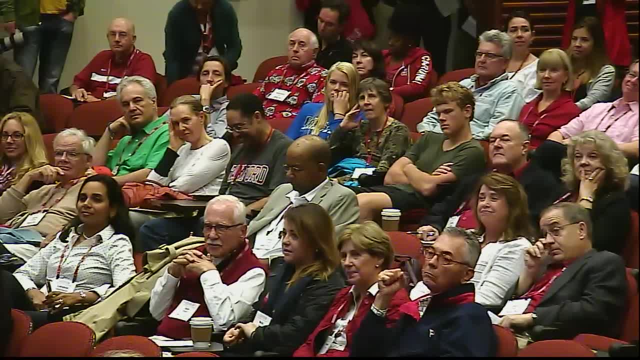 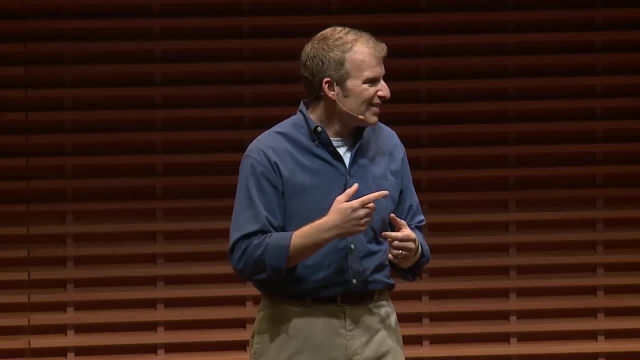 But a walk around the building before you speak, that can do it. There are other ways. If you've ever watched athletes perform and get ready to do their event, they listen to music. They focus on a song or a playlist that helps get them in the moment. 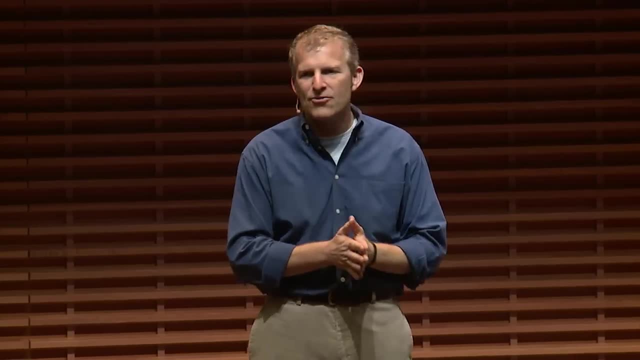 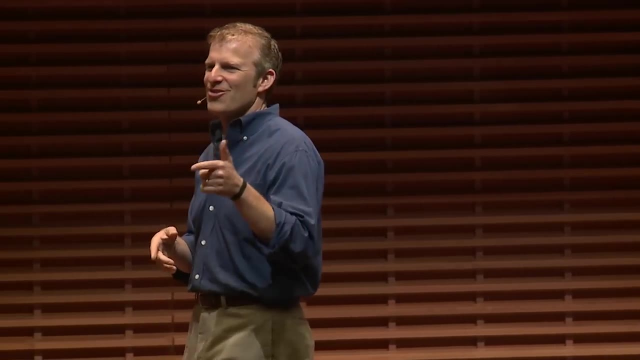 You can do things as simple as counting backwards from 100 by tough numbers like 17.. I'm going to pause because I know people in the room are trying. yeah, Gets hard. after that third or fourth one, I know My favorite way to get present-oriented is to say tongue twisters. 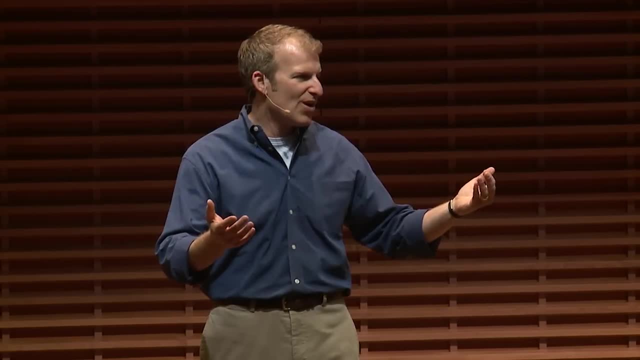 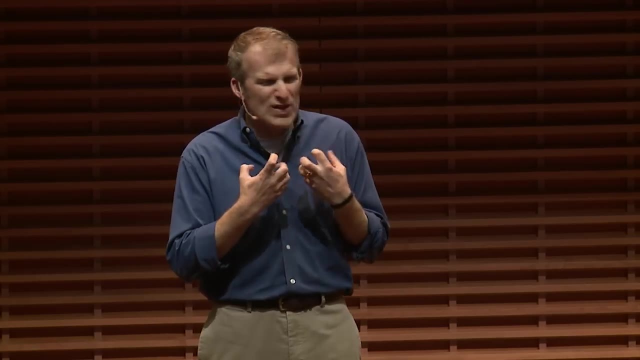 Saying a tongue twister forces you to be in the moment, otherwise you'll say it wrong, And it has the added benefit of warming up your voice. Most nervous speakers don't warm up their voice. They retreat inside themselves and start saying all these bad things to themselves. 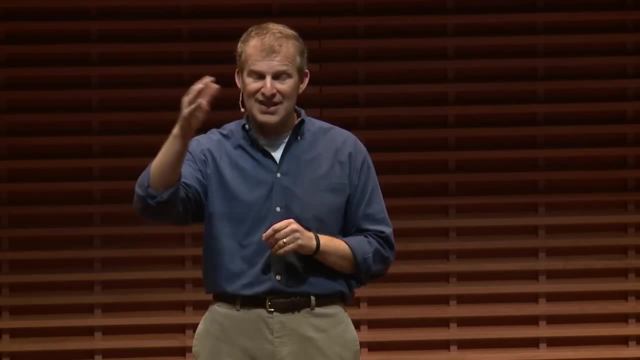 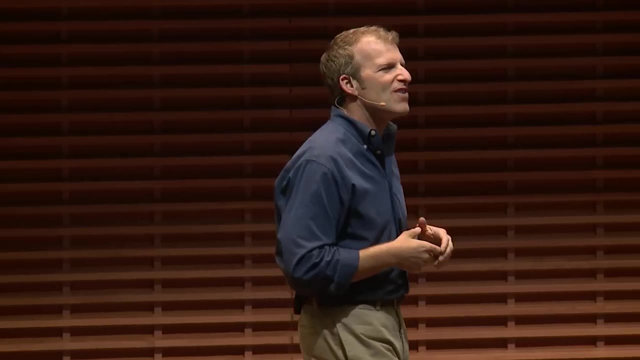 So saying a tongue twister can help you be both present-oriented and warm up your voice. Remember I said today we're going to have a lot of participation. I'm going to ask you to repeat after me my favorite tongue twister. And I like this tongue twister because if you say it wrong, 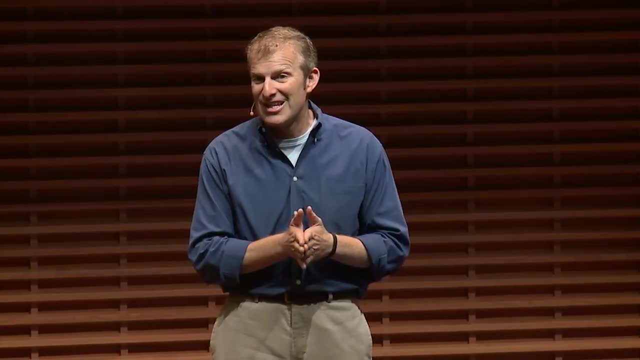 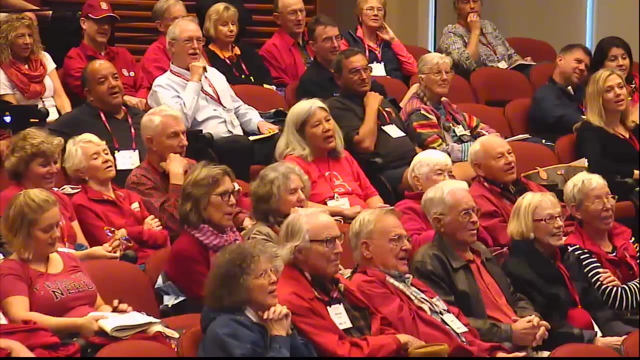 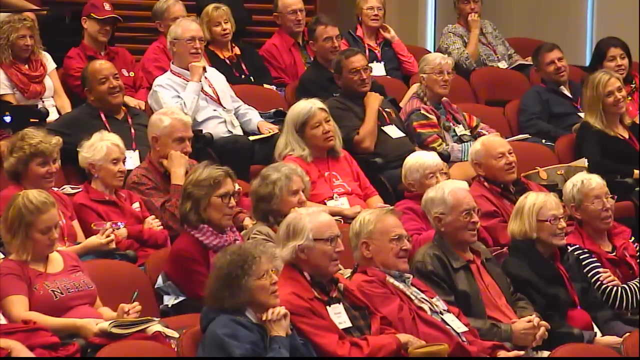 you say a naughty word And I'm going to be listening to see if I hear any naughty words this morning. Repeat after me. It's only three phrases. I slit a sheet, A sheet I slit, And on that slitted sheet I sit. 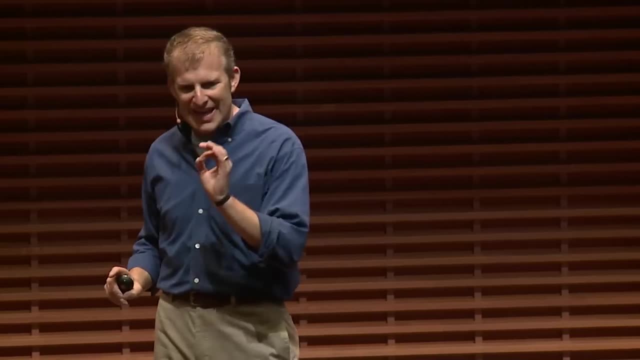 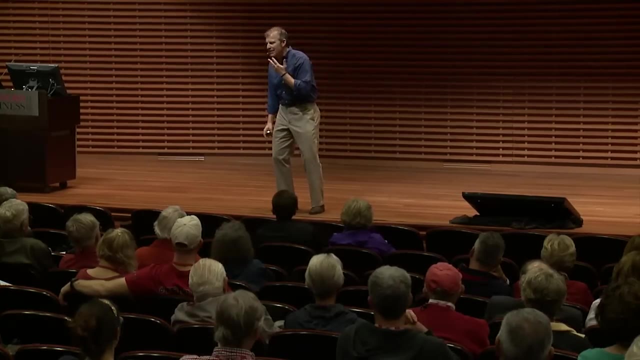 right before he comes out. You can't be that physically active and not be in the present moment. Now I'm not recommending all of us go to that level of exertion because he starts out of breath and sweaty right. But a walk around the building before you speak. 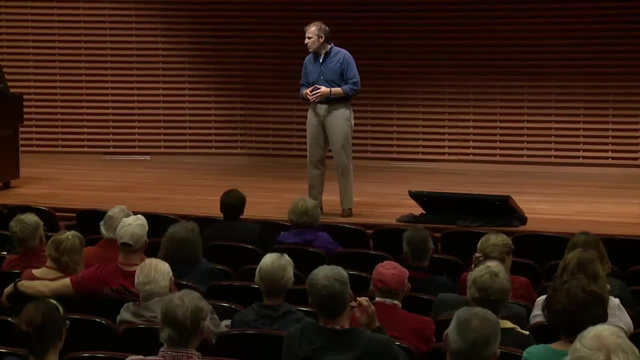 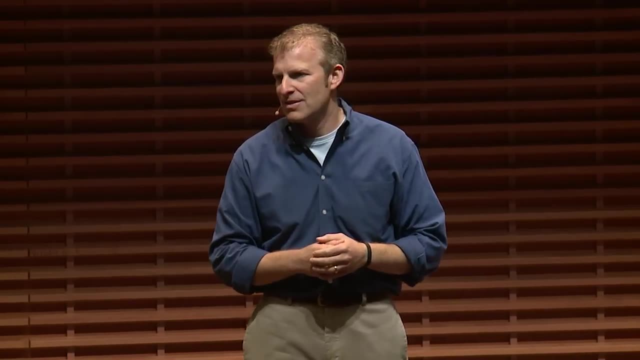 that can do it. There are other ways. If you've ever watched athletes perform and get ready to do their event, they listen to music. They focus on a song or a playlist that helps get them in the moment. You can do things as simple as. 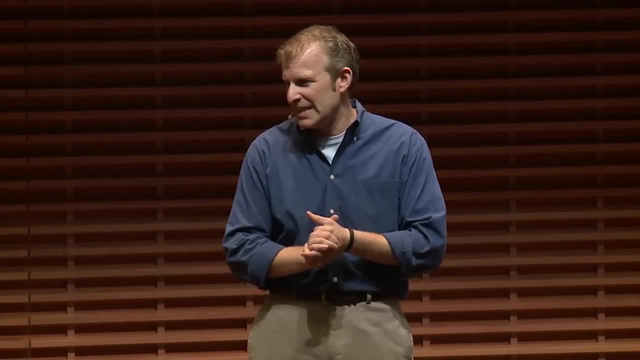 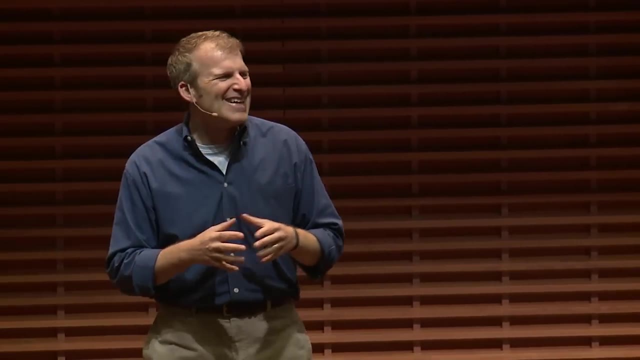 counting backwards from a hundred by tough numbers like 17.. I'm going to pause because I know people in the room are trying: yeah, Gets hard. after that third or fourth one, I know My favorite way to get present-oriented is to say tongue twisters. 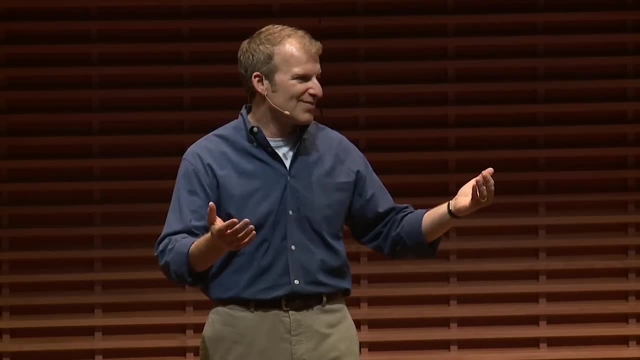 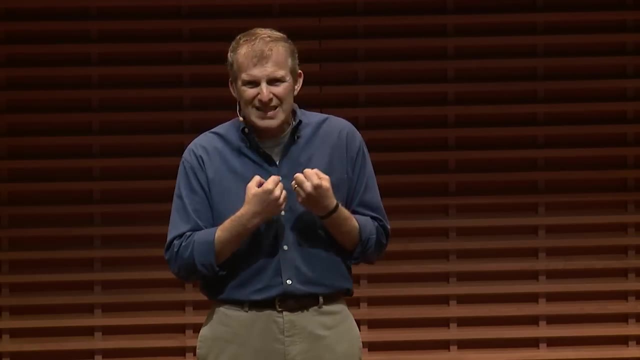 Saying a tongue twister forces you to be in the moment, otherwise you'll say it wrong, And it has the added benefit of warming up your voice. Most nervous speakers don't warm up their voice. They retreat inside themselves and start saying all these bad things to themselves. 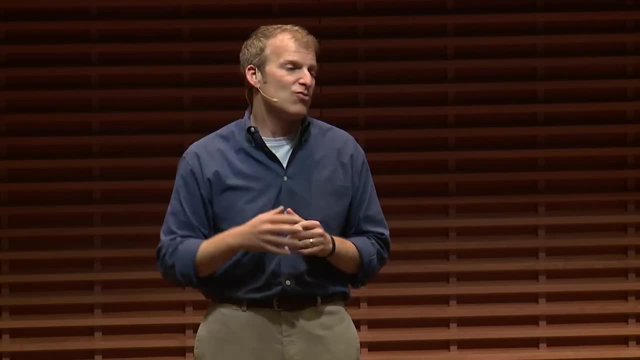 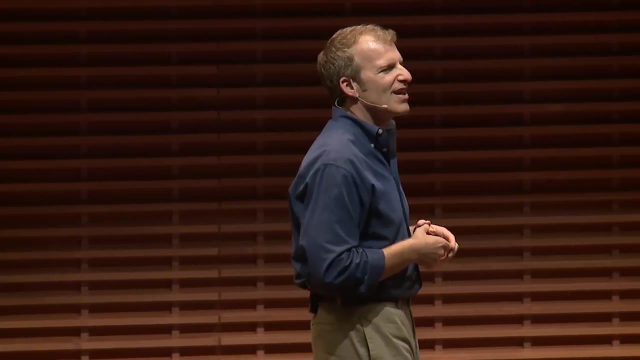 So saying a tongue twister can help you be both present-oriented and warm up your voice. Remember I said today we're going to have a lot of participation. I'm going to ask you to repeat after me my favorite tongue twister: 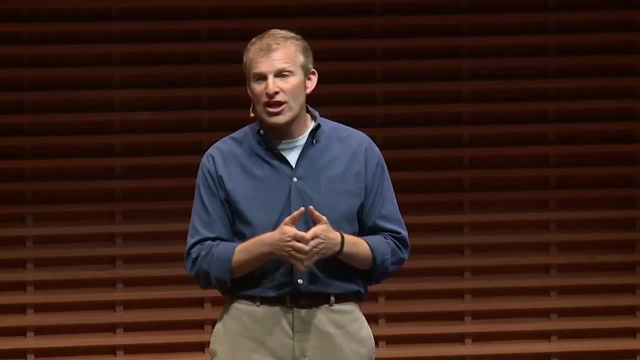 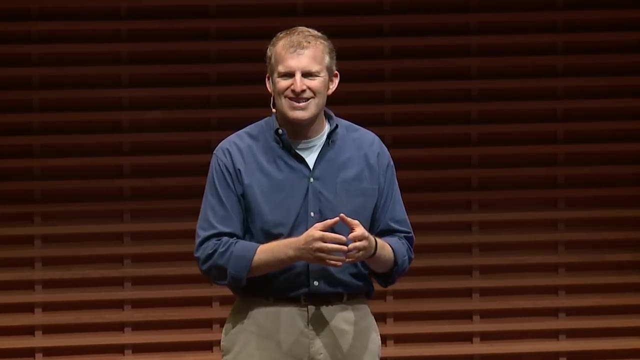 And I like this tongue twister because if you say it wrong, you say a naughty word And I'm going to be listening to see if I hear any naughty words this morning Repeat after me. It's only three phrases. I slit a sheet. 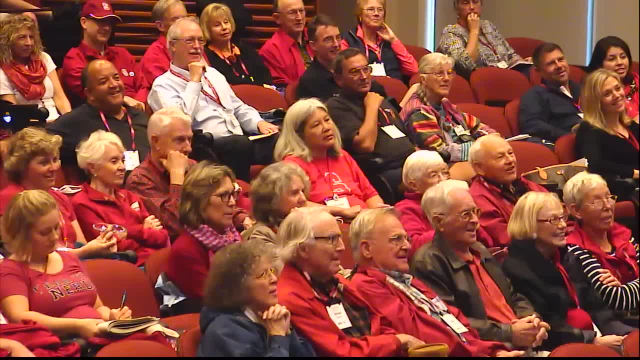 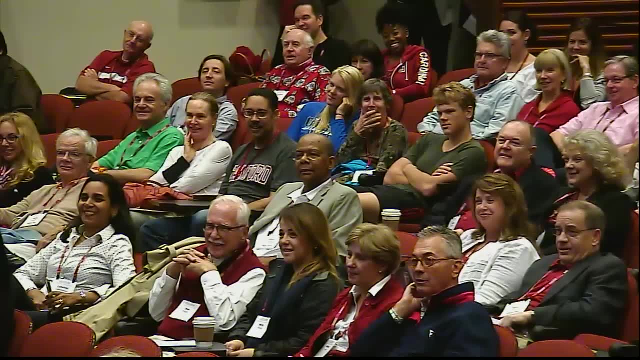 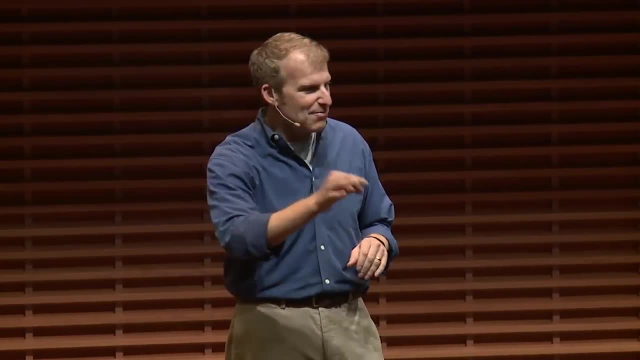 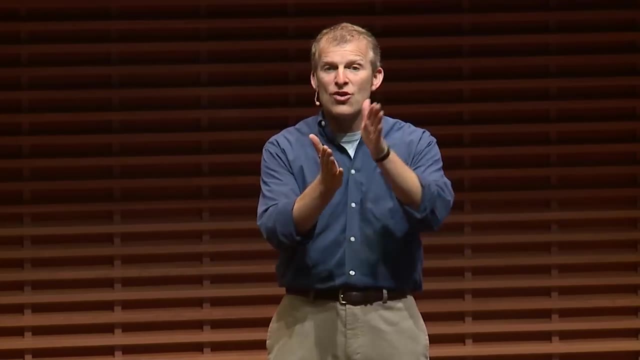 Excellent, Very good. Now, in that moment, in that moment you weren't worried about I'm in front of all these people. this is weird. this guy's having me do this. You were so focused on saying it right and trying to figure out what the naughty word was. 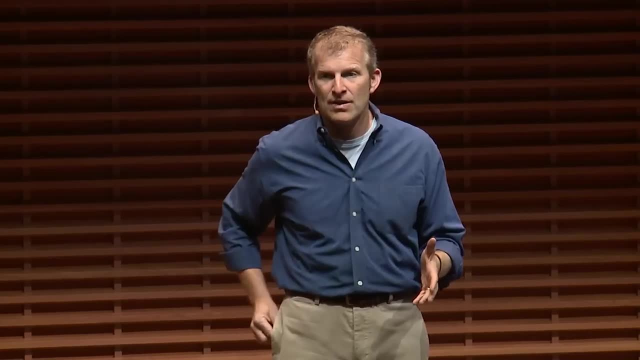 that you were in the present moment. That's how easy it is. So it's very possible for us to manage that. So it's very possible for us to manage that. So it's very possible for us to manage our anxiety. 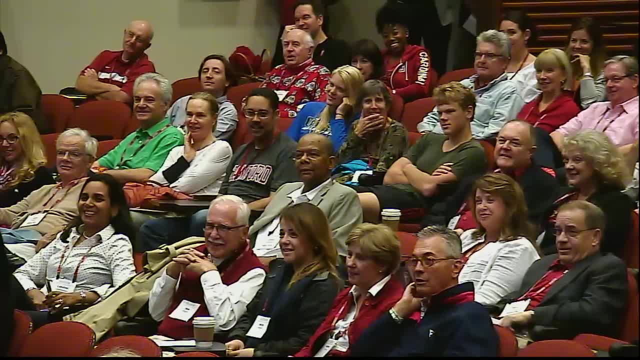 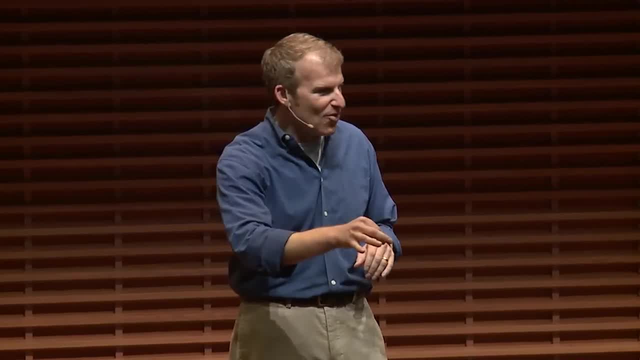 And on that slitted sheet I sit. Oh, very good, No shits, Excellent, Very good. Now, in that moment, in that moment you weren't worried about, I'm in front of all these people. this is weird. this guy is having me do this. 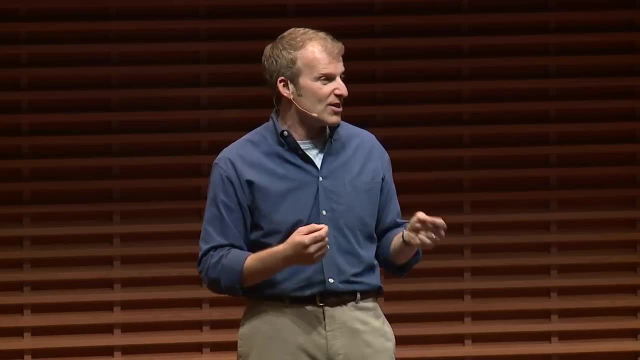 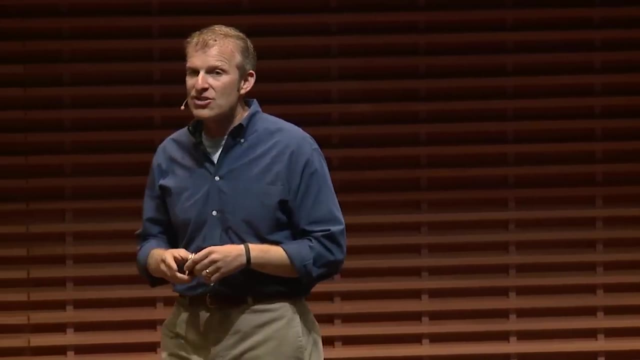 You were so focused on saying it right and trying to figure out what the naughty word was that you were in the present moment. That's how easy it is, So it's very positive, And then, on that slide, I'm going to get back to you. 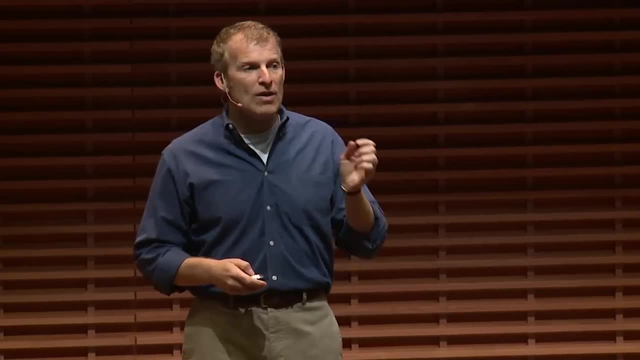 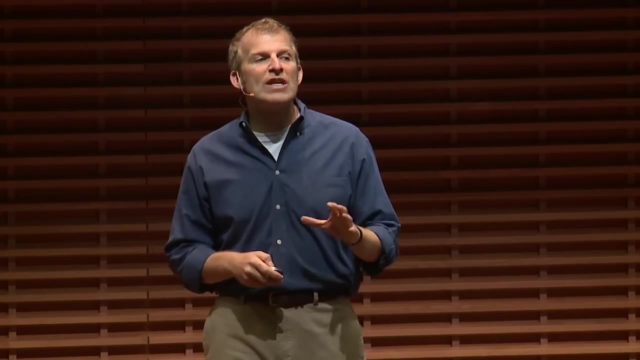 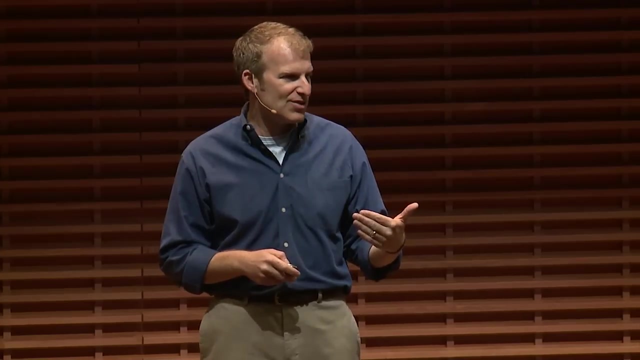 When we think about this, you guys are really excited. You feel like you have to say something about this at the moment. So, as I've said, get out of this, Get out of the way, Get out of the way, And then at the end of the conversation, we're not going. 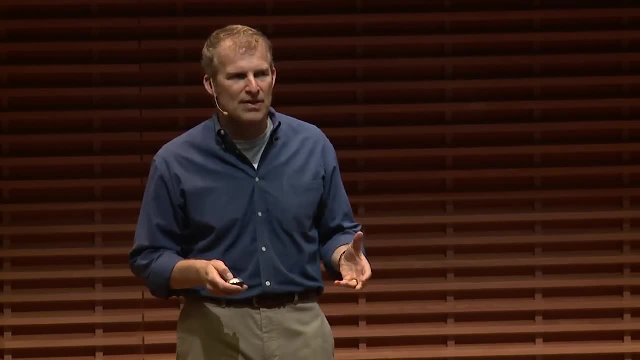 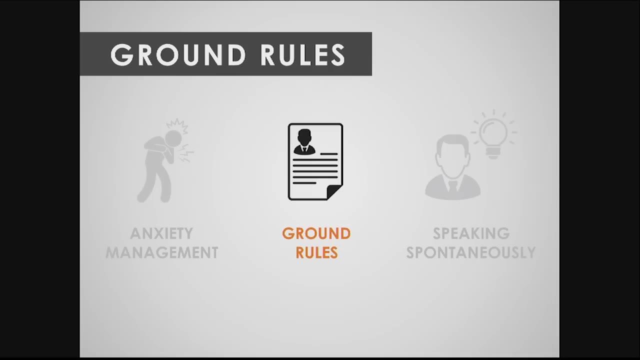 to go back and do it again. We're not going to do that. sources for you. So let's get started on the core part of what we're doing today, which is how to feel more comfortable speaking in spontaneous situations. Some very simple ground. 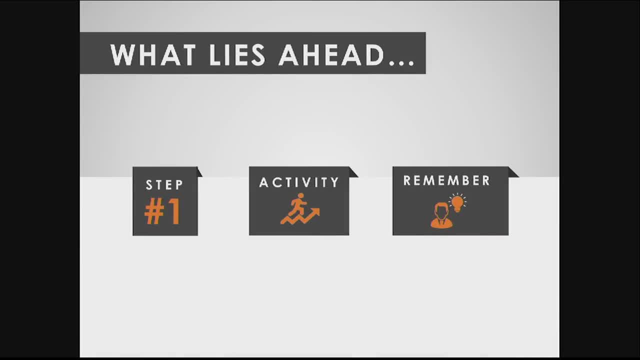 rules for you. First, I'm going to identify four steps that I believe are critical to becoming effective at speaking in a spontaneous situation. With each of those steps, I'm going to ask you to participate in an activity. None of them are more painful than saying: 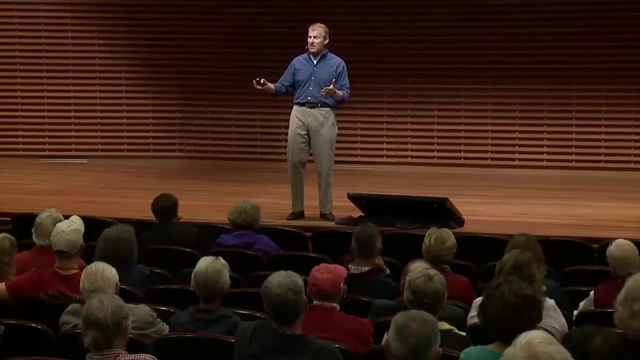 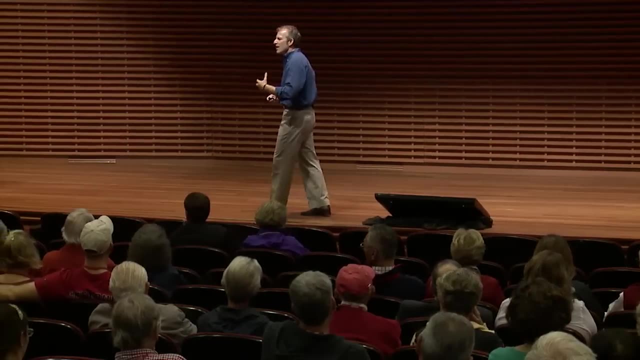 the tongue twister out loud. They may require you to stand up, They might require you to talk to the person next to you, but none of them are painful. And then, finally, I'm going to conclude with a phrase or saying that comes from the wonderful world of improvisation. 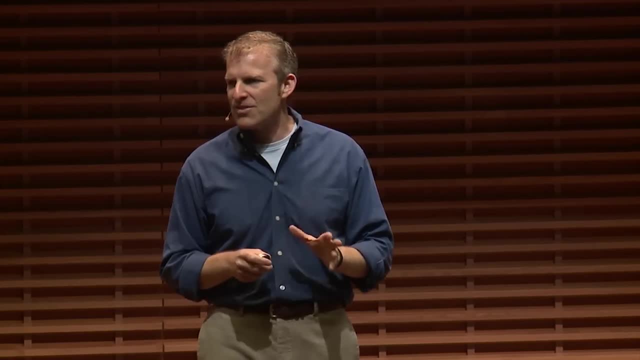 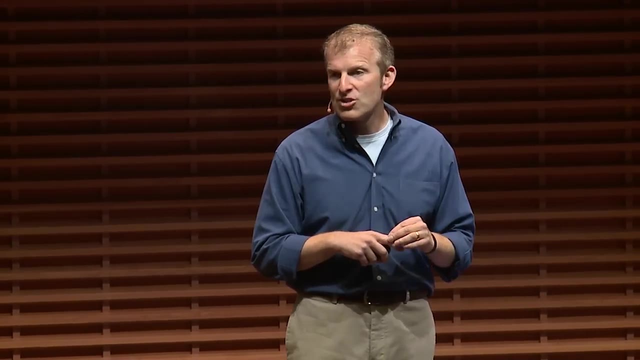 Through the continuing studies program here at Stanford. for the past five years I have co-taught a class with Adam Tobin. He is a lecturer in the creative arts department. He teaches film and new media and he's an expert at improv. 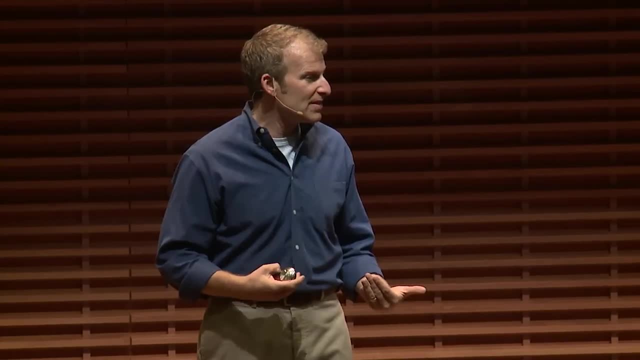 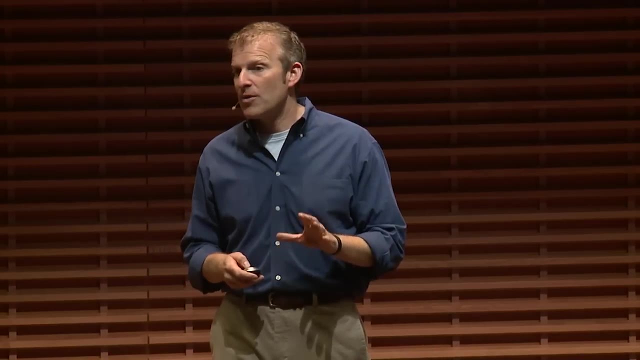 We can do it initially by greeting the anxiety when we begin to feel those signs. We can do it when we reframe the situation as a conversation And we do it when we become present-oriented. Those are three of many tools that exist to help you manage your anxiety. 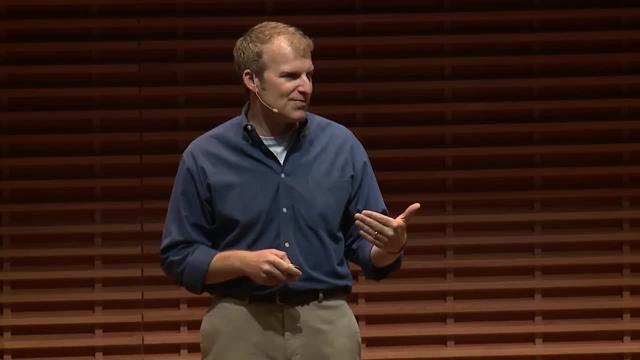 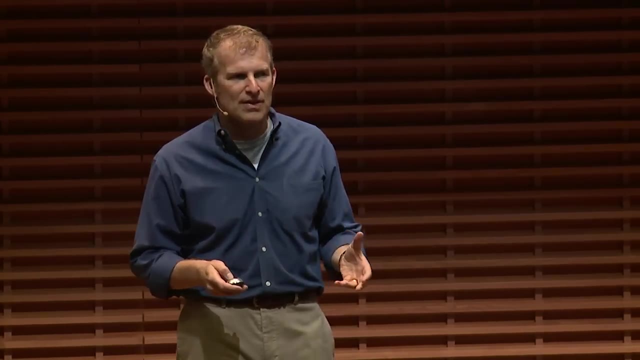 If you have questions about other ways, I'm happy to chat with you, And at the end I'm going to point you to some resources that you can refer to to help you find additional sources for you. So let's get started on the core part. 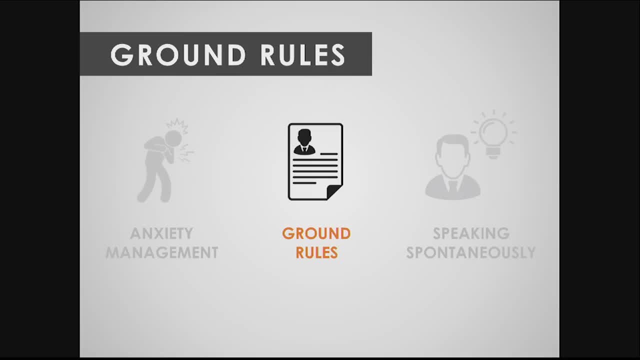 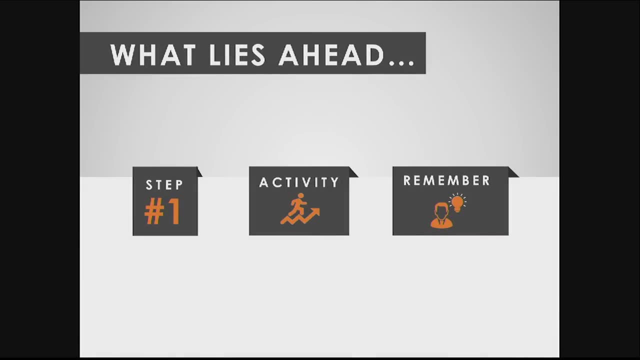 of what we're doing today, which is how to feel more comfortable speaking in spontaneous situations. Some very simple ground rules for you. First, I'm going to identify four steps that I believe are critical to becoming effective at speaking in a spontaneous situation. 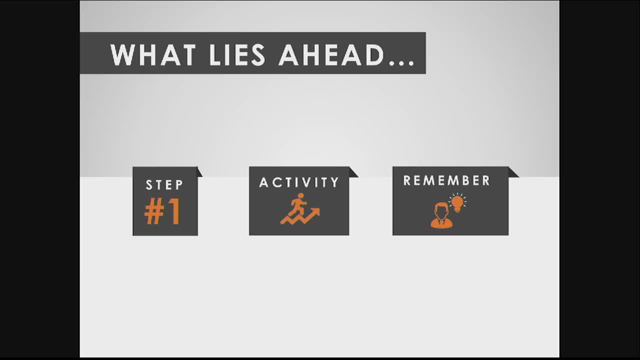 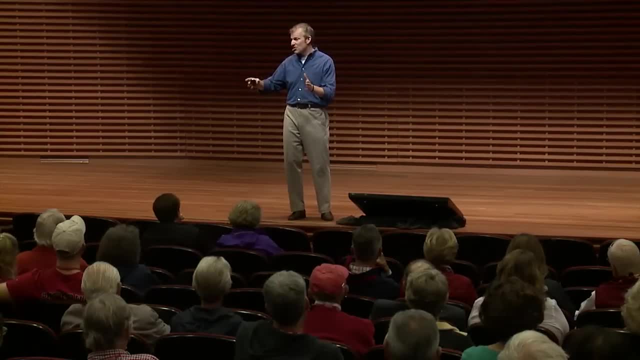 With each of those steps, I'm going to ask you to participate in an activity. None of them are more painful than saying the tongue twister out loud. They may require you to stand up. They might require you to talk to the person next to you. 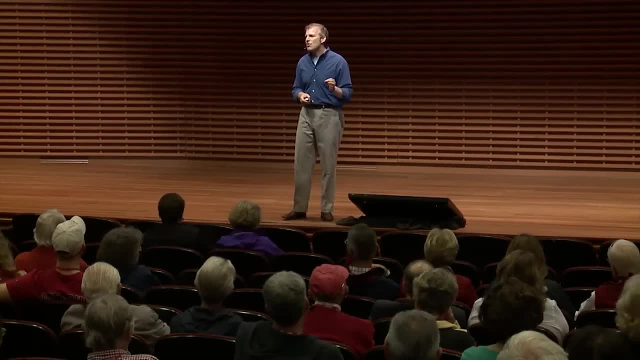 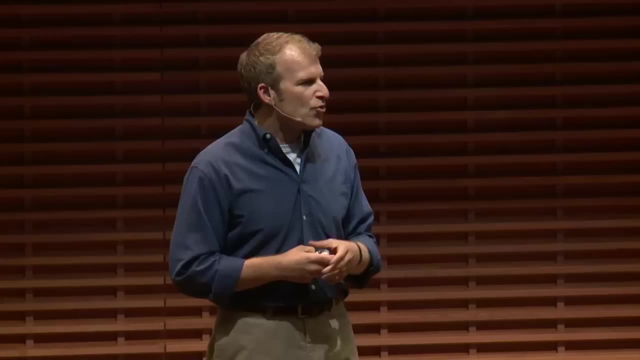 But none of them are painful. And then, finally, I'm going to conclude with a phrase or saying that comes from the wonderful world of improvisation. Through the continuing studies program here at Stanford for the past five years I have co-taught a class with Adam Tobin. 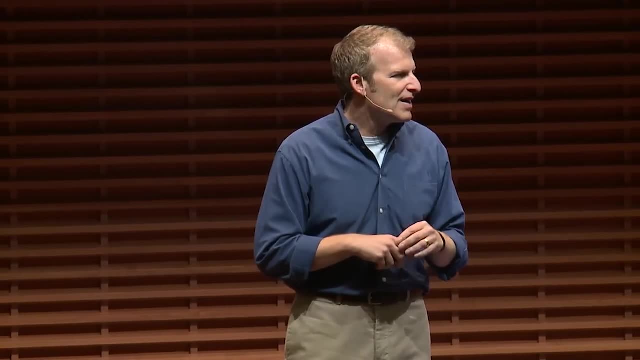 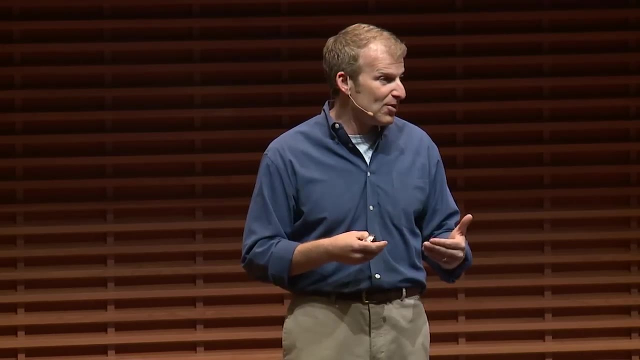 He is a lecturer in the creative arts department. He teaches film and new media And he's an expert at improv And we've partnered together to help people learn how to speak more spontaneously. We call it improvisationally speaking, And Adam has taught me wonderful phrases. 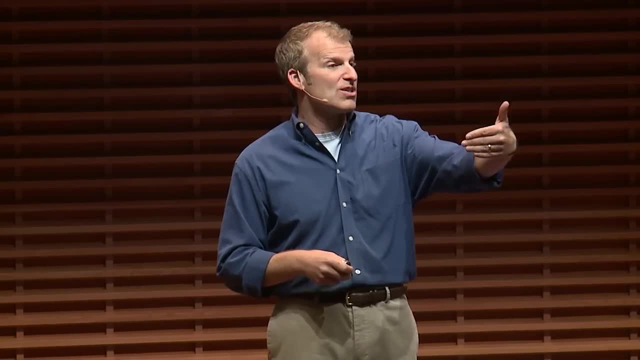 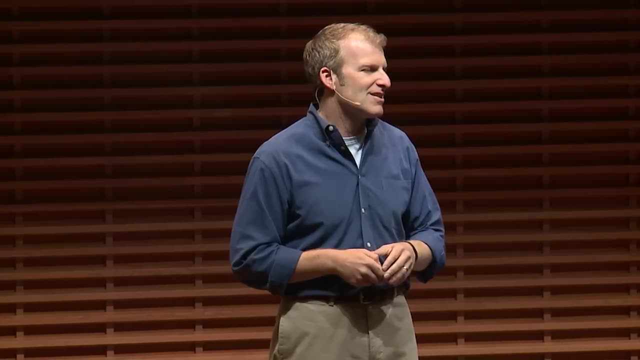 and ideas from improv that I want to impart to you that really stick. That's why I'm sharing them with you, to help you remember these techniques. And again, at the end of all this, you'll get a handout that has this listed. 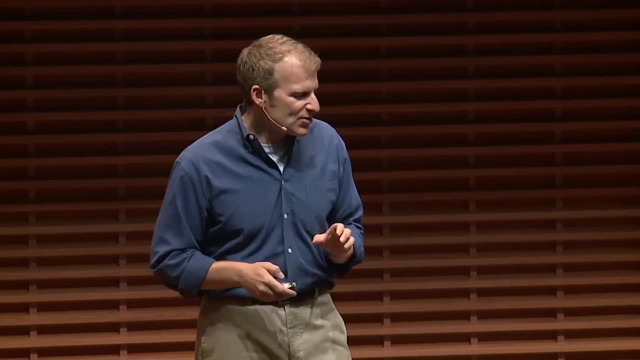 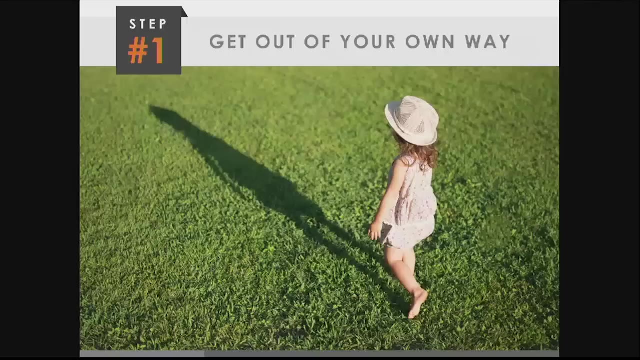 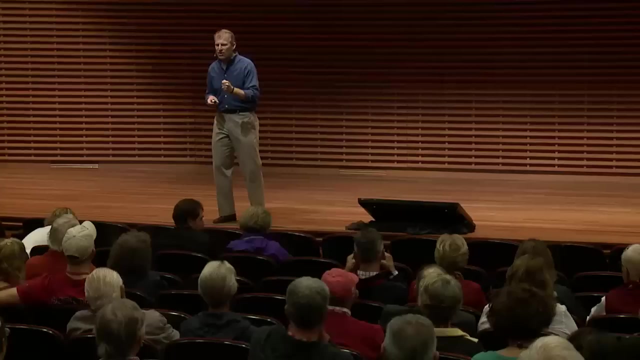 So let's get started. The very first thing that gets in people's way when it comes to spontaneous speaking is themselves. We get in our own way. We want to be perfect, We want to give the right answer. We want our toast to be incredibly memorable. 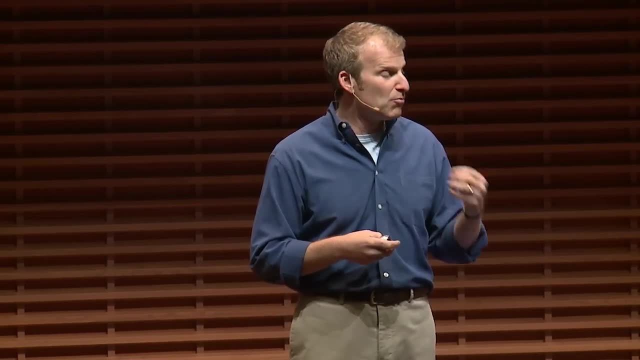 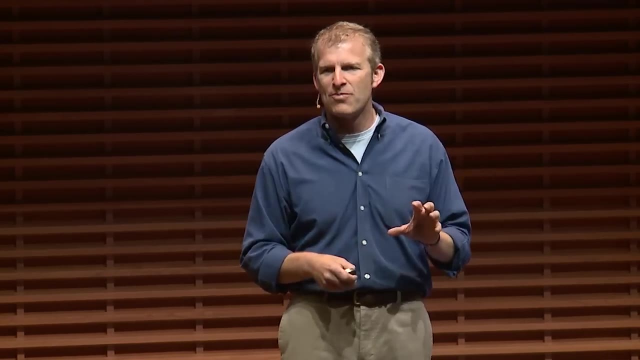 And we've We've partnered together to help people learn how to speak more spontaneously. We call it improvisationally speaking, And Adam has taught me wonderful phrases and ideas from improv that I want to impart to you that really stick. That's why I'm sharing them with you to help. 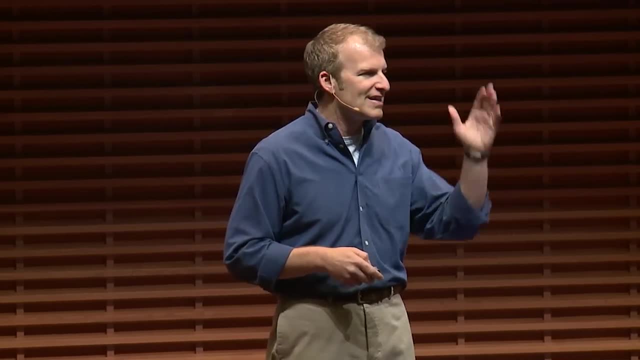 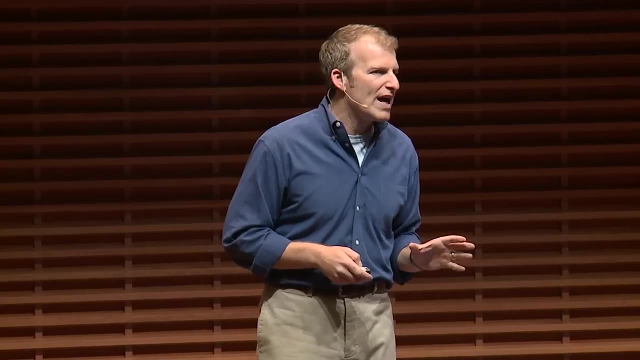 you remember these techniques And again, at the end of all this, you'll get a handout that has this listed. So let's get started. The very first thing that gets in people's way when it comes to spontaneous speaking is themselves. We get. 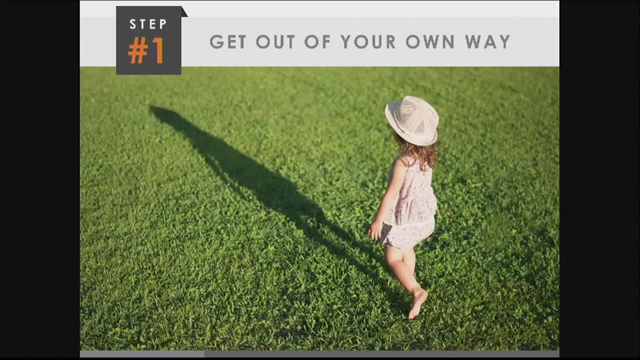 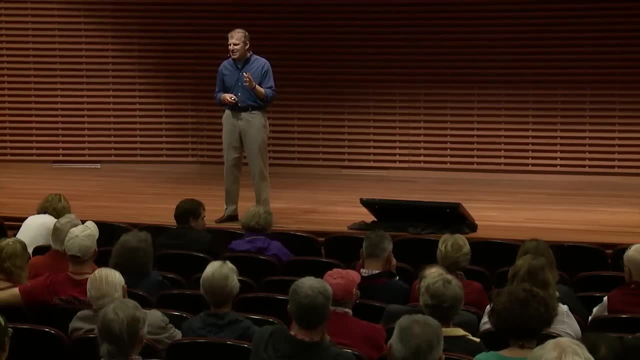 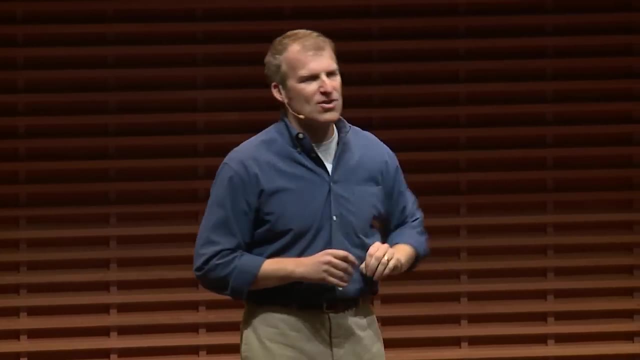 in our own way. We want to be perfect, We want to give the right answer, We want our toasts to be incredibly memorable. These things are burdened by our effort, by our trying, The best thing we can do. the first step in our process is to get ourselves out. 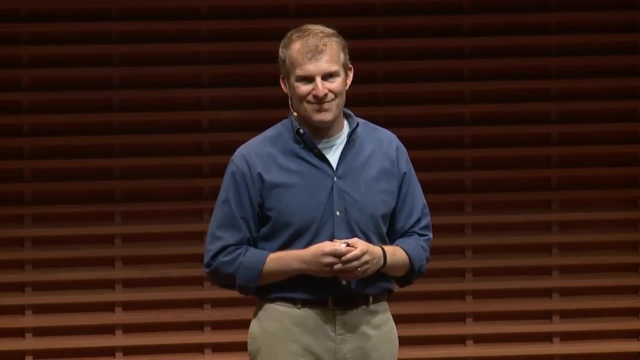 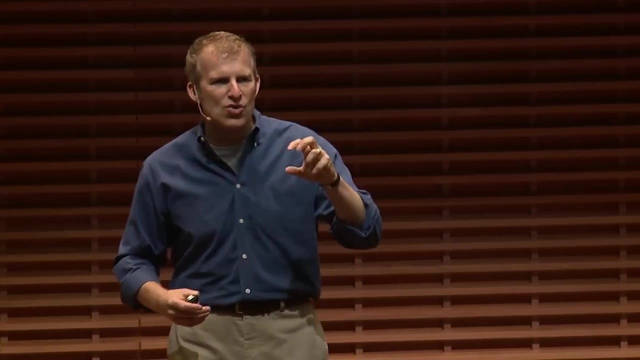 of the way, Easier said than done. Most of us in this room are in this room because we are type A personalities: We work hard, We think fast, We make sure that we get things right. But that can actually serve as a disservice as we try. 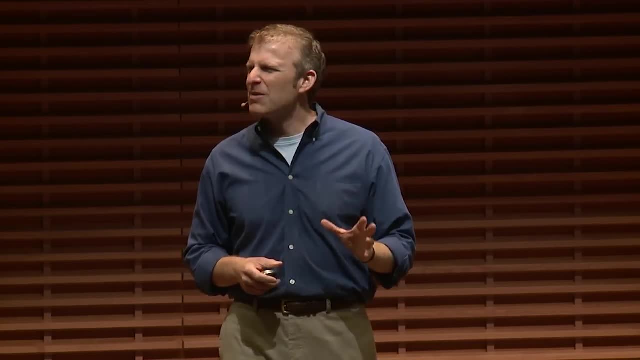 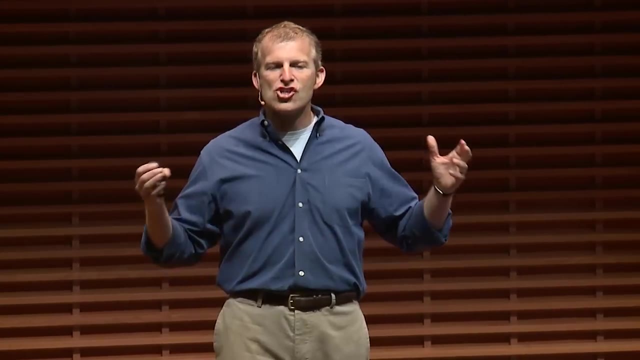 to speak in the moment. I'd like to demonstrate a little of this for you, and I need your help to do that. So we're going to do our first activity. We are going to do an activity that's called Shout the Wrong Name. In a moment, if you are able and willing, I'm going to. 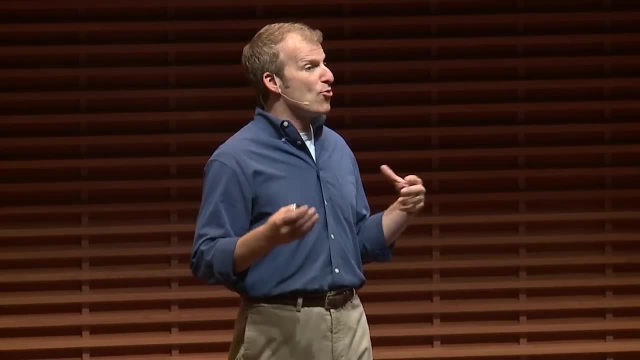 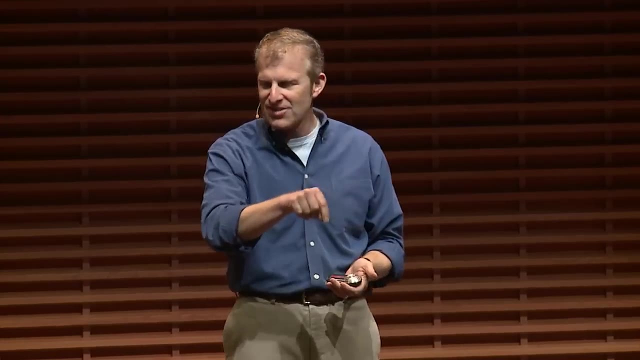 ask you to stand And I am going to ask you for about 30 seconds to look all around you in this environment And you are going to point at different things And I know it's rude to point, but for this exercise, please point. I want you to point to things and you are going to call the things. 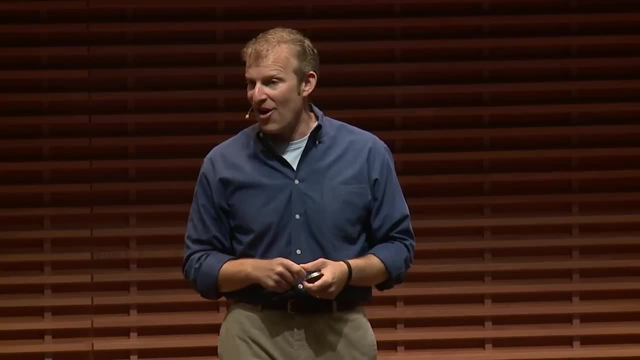 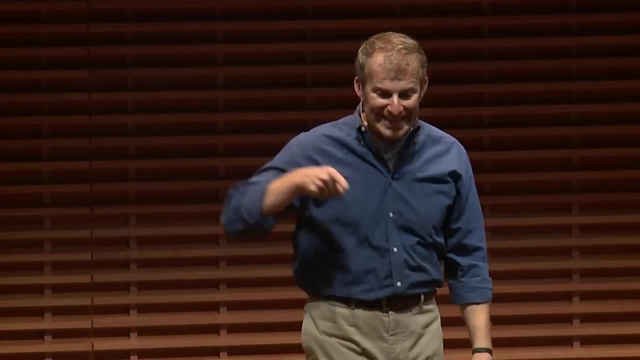 you are pointing to out loud anything but what they really are. So I might point to this and say refrigerator. I might point to this and say cat, I am pointing to anything in your environment, around you. It can be the person sitting next to you, standing next. 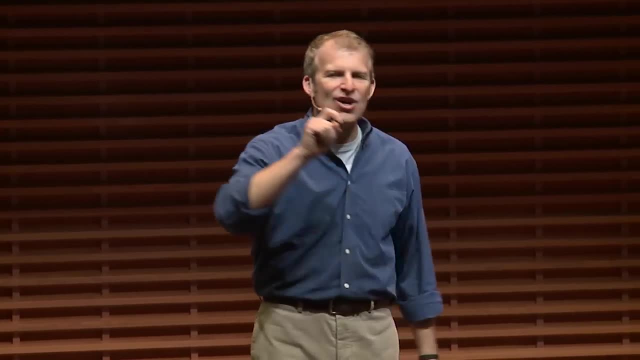 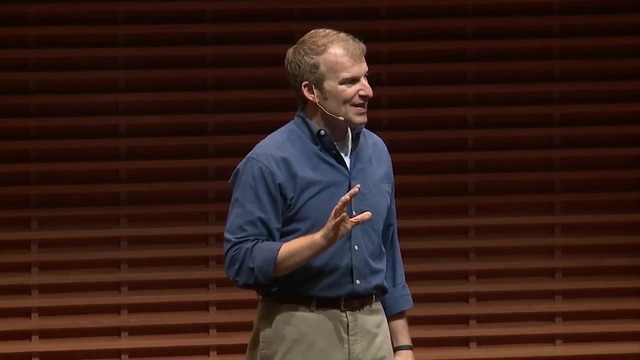 to you. You will just shout and shouting is important- the wrong name. So in a moment I'm going to ask you to stand and do that. Please raise your hand if you already have the first five or six things you are going to call out. 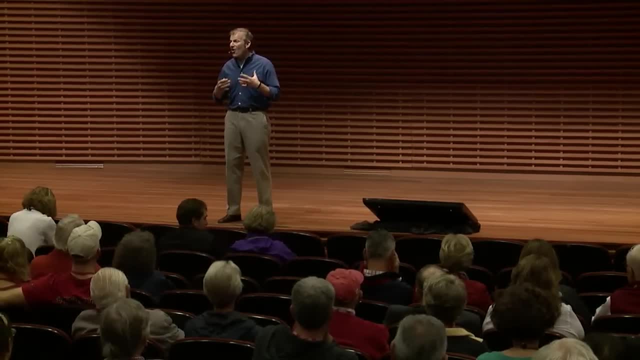 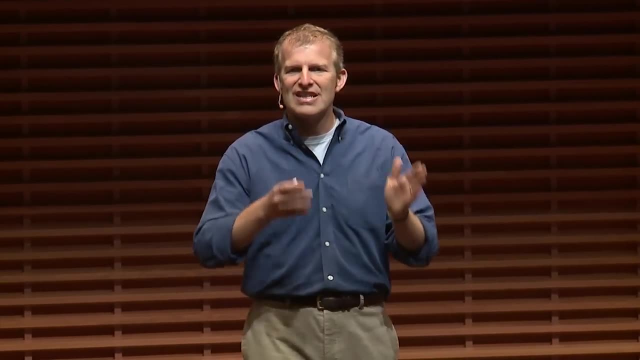 These things are burdened by our effort, by our trying The best thing we can do. the first step in our process is to get ourselves out of the way. Easier said than done. Most of us in this room are in this room. 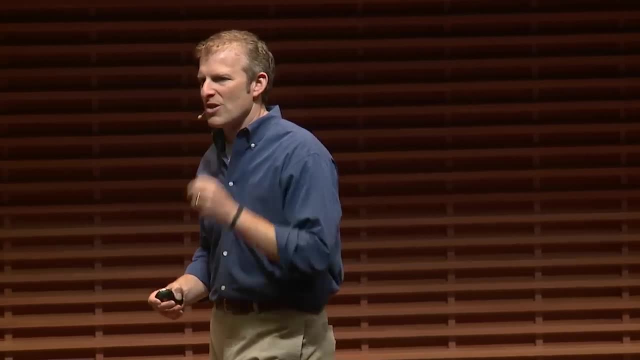 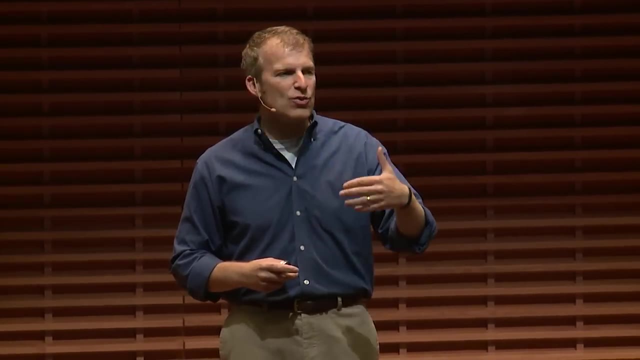 because we are type A personalities: We work hard, We think fast, We make sure that we get things right- But that can actually serve as a disservice as we try to speak in the moment. I'd like to demonstrate a little of this for you. 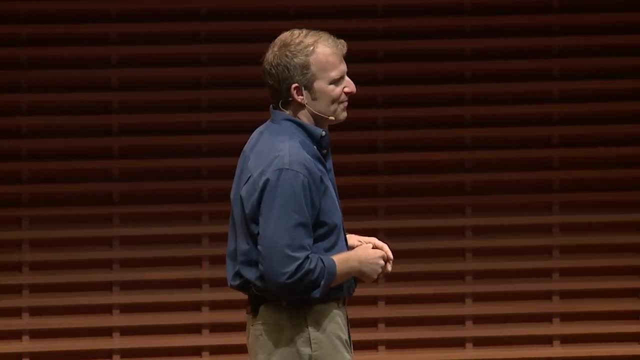 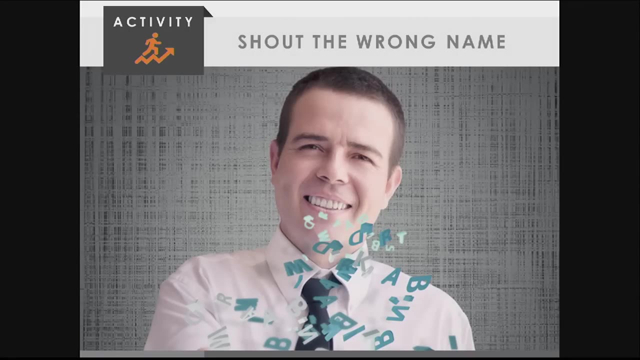 and I need your help to do that. So we're going to do our first activity. We are going to do an activity that's called Shout the Wrong Name. In a moment, if you are able and willing, I'm going to ask you to stand. 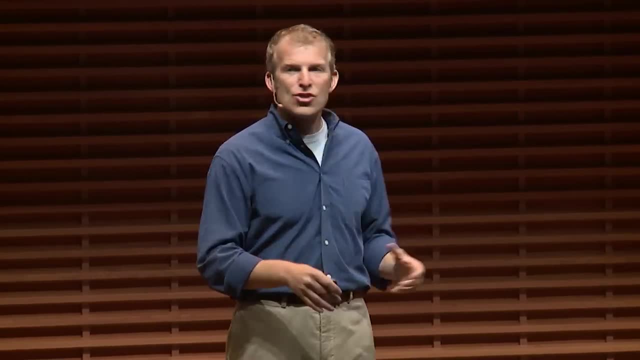 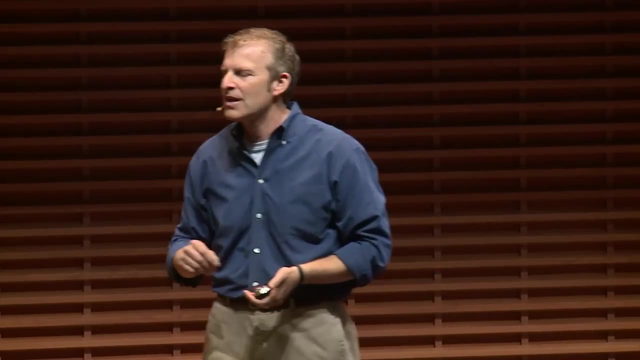 And I am going to ask you for about 30 seconds to look all around you in this environment and you are going to point at different things And I know it's rude to point, but for this exercise, please point. I want you to point to things. 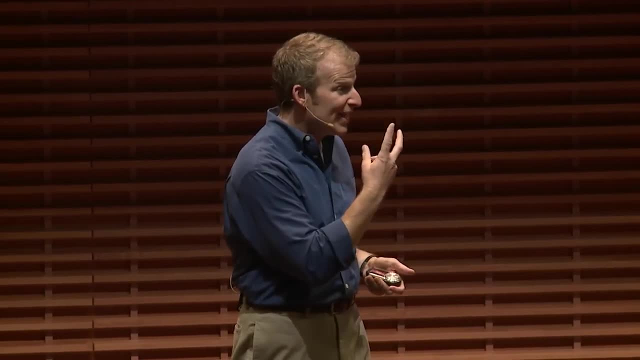 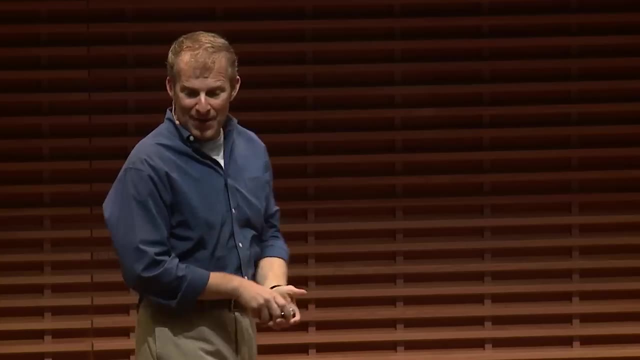 and you are going to call the things you are pointing to out loud anything but what they really are. So I might point to this and say refrigerator. I might point to this and say cat. I am pointing to anything in your environment around you. 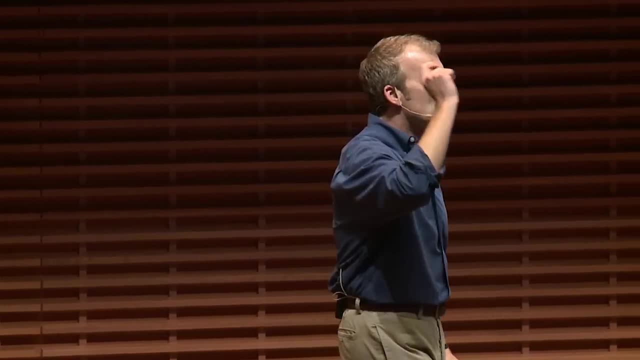 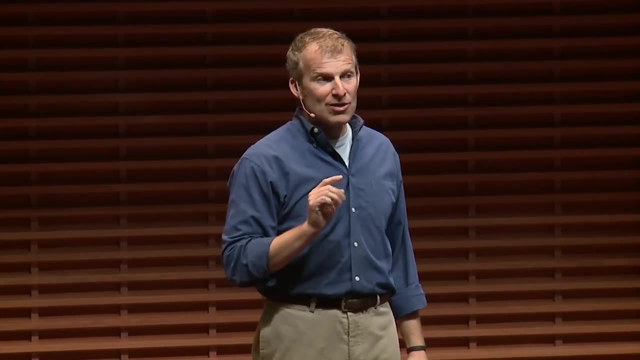 It can be the person sitting next to you. standing next to you. You will just shout and shouting is important, the wrong name. So in a moment I am going to ask you to stand and do that. Please raise your hand if you already have the first five or six things. 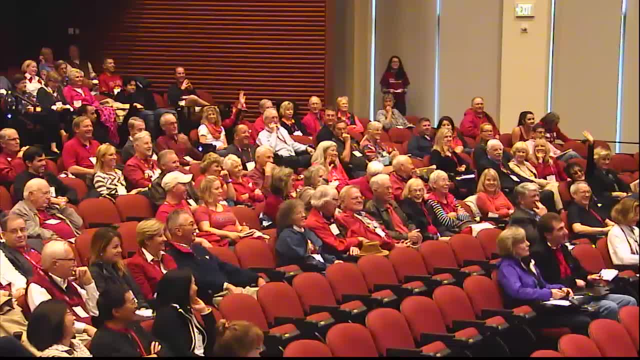 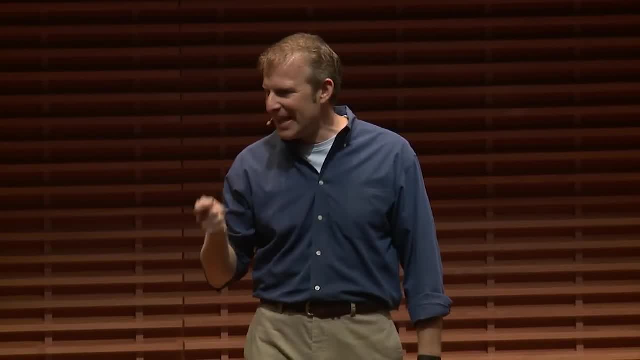 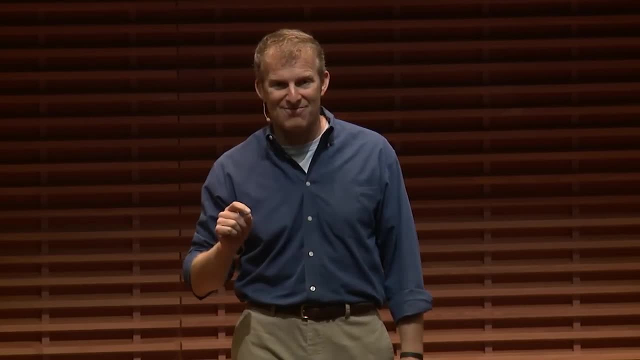 you are going to call out: Yeah, That's what I am talking about. We stockpile. You all are excellent game players. I told you the game Shout the wrong name And you have already begun figuring out how you are going to master the game. 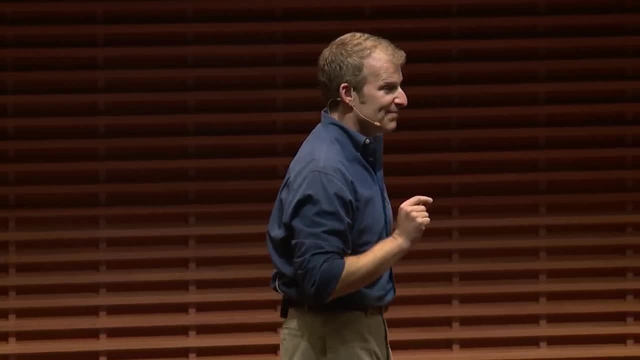 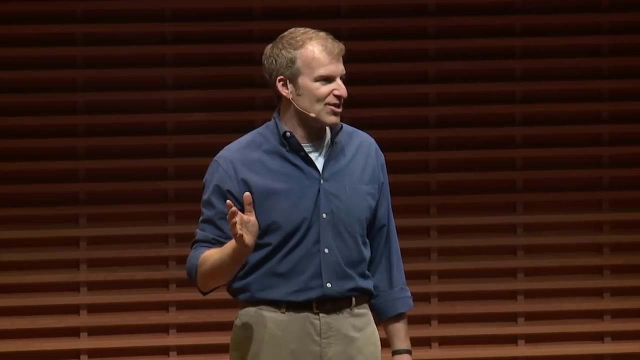 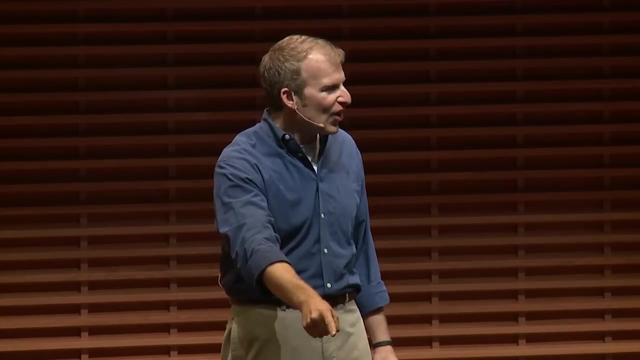 That's your brain trying to help you get it right. I would like to suggest the only way you can get this activity wrong is by doing what you have just done. There is no way to get this wrong, Even if I call this a chair. 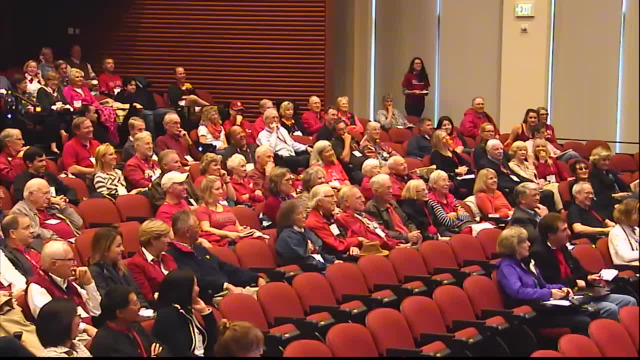 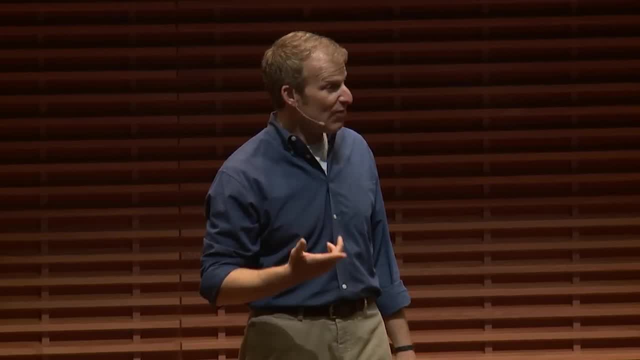 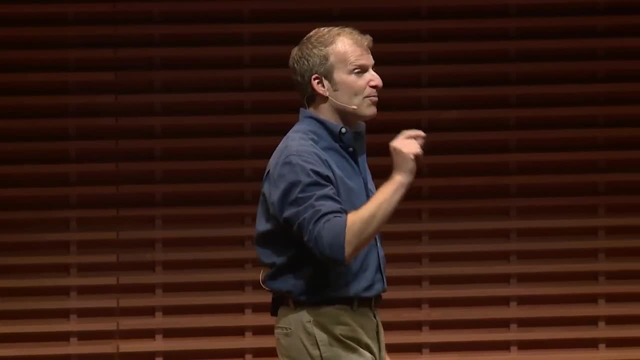 Yeah, That's what I'm talking about. We stockpile. You all are excellent game players. I told you the game Shout the wrong name And you have already begun figuring out how you are going to master the game. That's your brain trying to help you get it right. 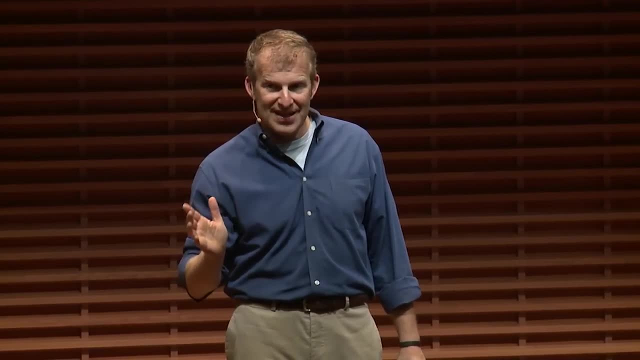 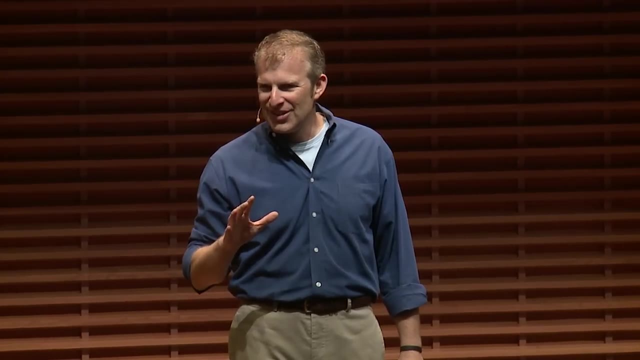 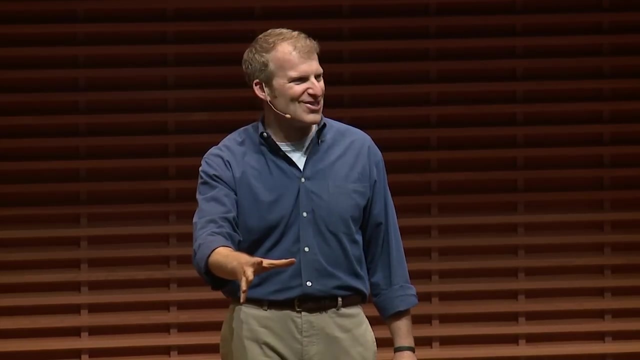 I would like to suggest: the only way you can get this activity wrong is by doing what you have just done. There is no way to get this wrong. Okay, Even if I call this a chair, no penalty will be bestowed upon you. Okay, Because I won't know what you were pointing. 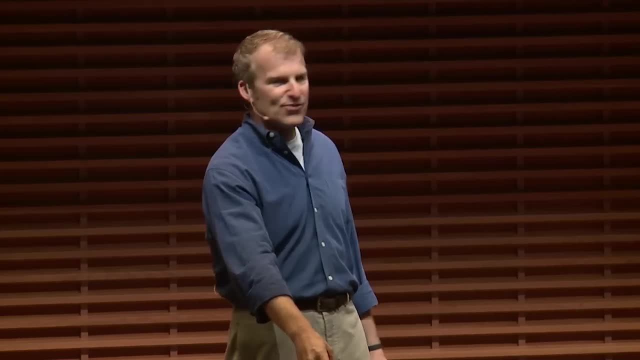 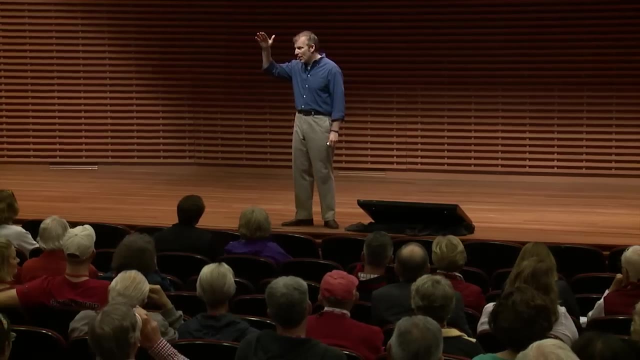 at. You could have been pointing at the floor under the chair and you called the floor the chair and you were fine. The point is we are planning and working to get it right, And there is no way to get it right, Just doing it gets it right. Okay, So let's try. 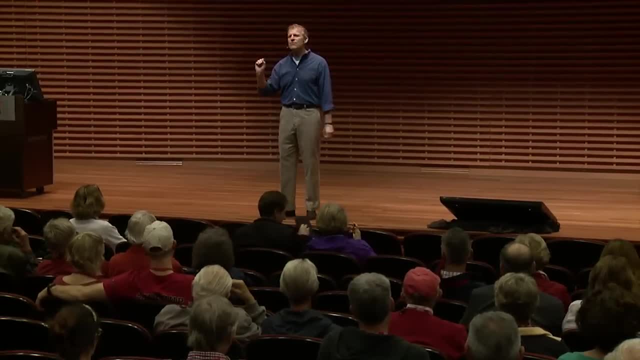 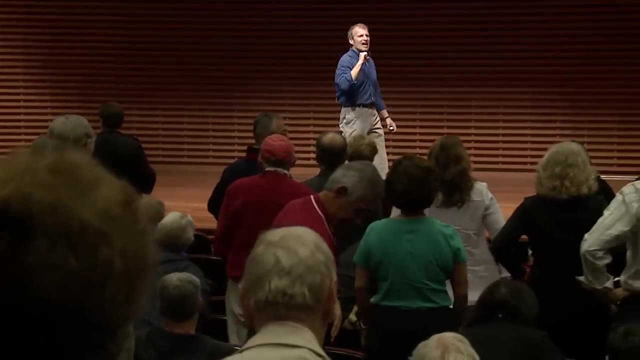 this. now We are going to play this game twice Again. it's for 30 seconds. If you are willing and able, will you please stand up? You can do this seated, by the way, But if you are willing and able, let's stand up. Okay, In a moment I am about to say go And I would 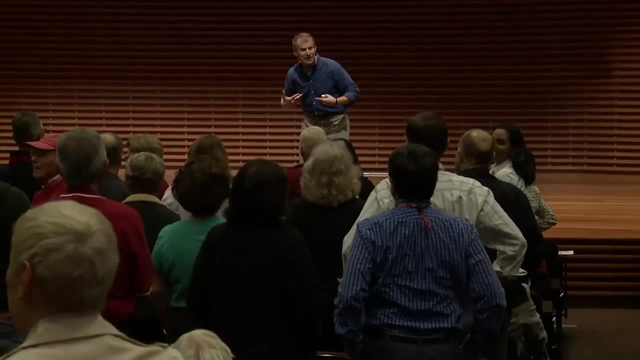 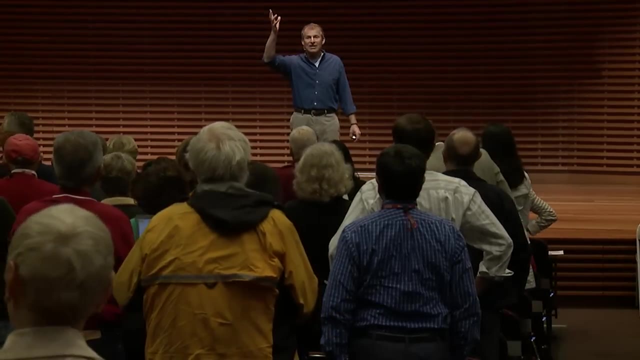 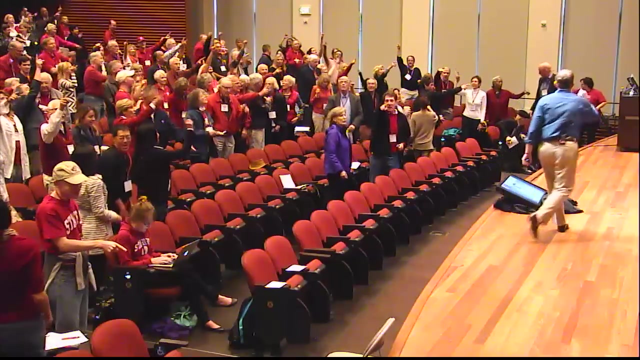 like for you to point at anything around here, including me. It's okay to point at me. I hope it's not a bad thing you say when you point at me, But point at different things and loudly and proudly call them different. Kim Wóg搖. 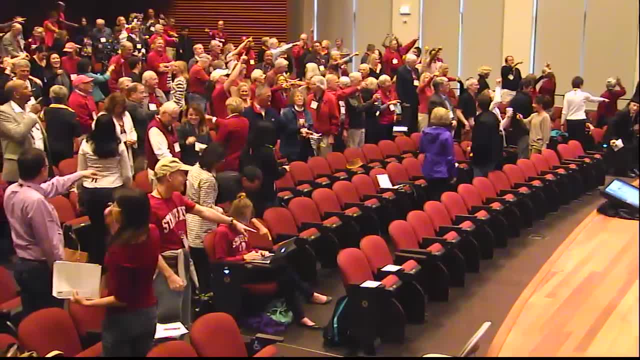 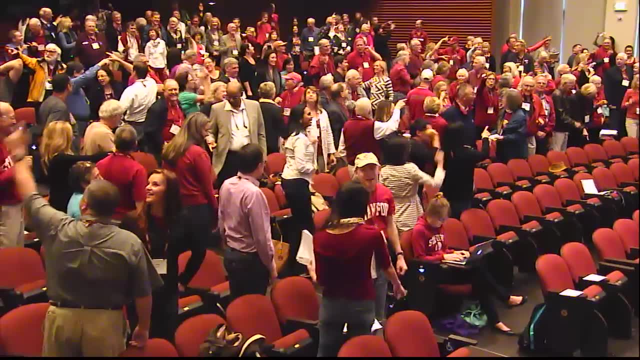 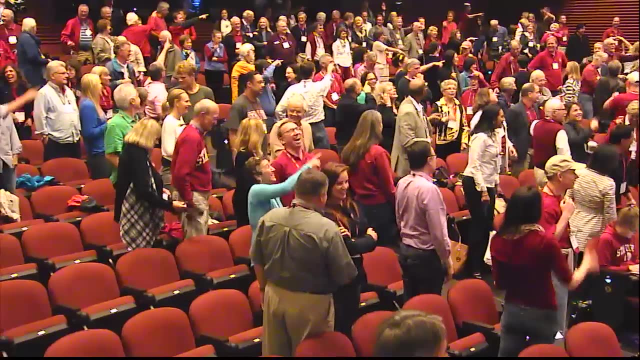 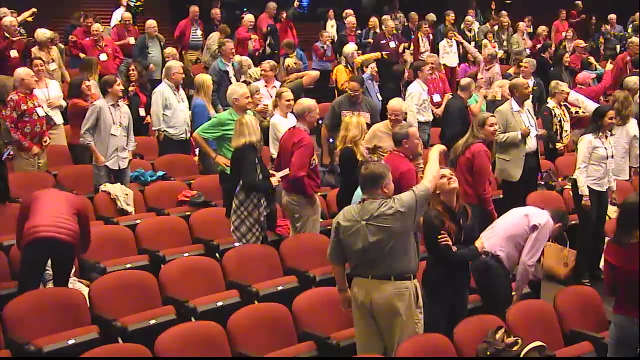 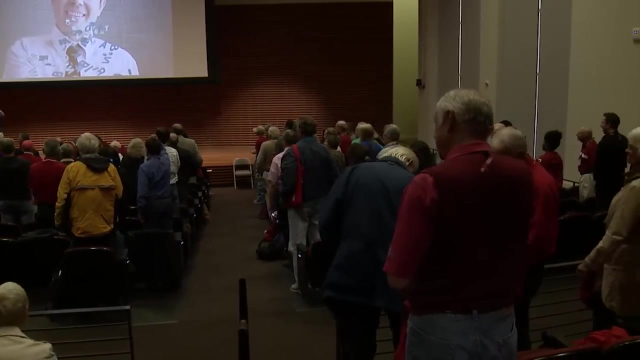 out in the sky. your worth is far more valuable than what they are. Ready Begin Porcupine, California, Salt shaker, Car Library, Tennis racket, Purple, Orange, Putrid, Hello Time, Time, Tommy time. You can stay standing because in mere moments we're going to do it again. So if you're 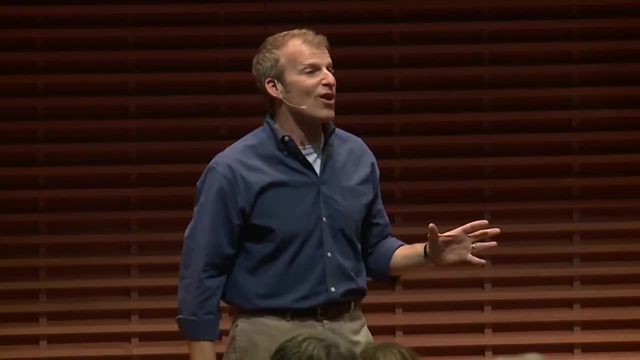 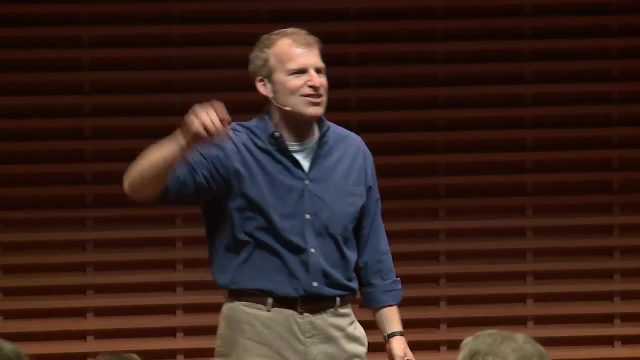 comfortable standing. we're about to do it again. First, thank you. That was wonderful. I heard great words being called out. It was fun, And some of you in the back were doing it in sync, so it looked like you were doing some 70s disco dance. It was awesome. Okay, this was great. Now, 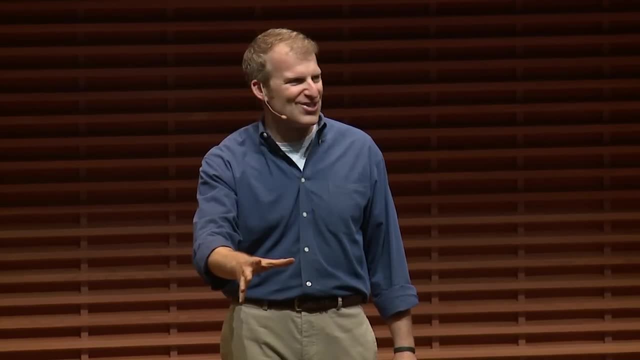 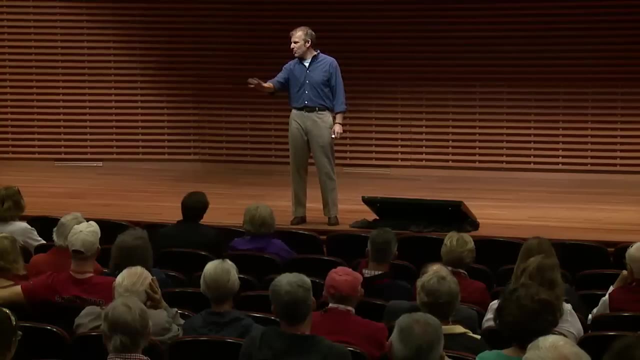 no penalty will be bestowed upon you Because I won't know what you were pointing at. You could have been pointing at the floor under the chair and you called the floor, the chair and you were fine. The point is we are planning and working to get it right. 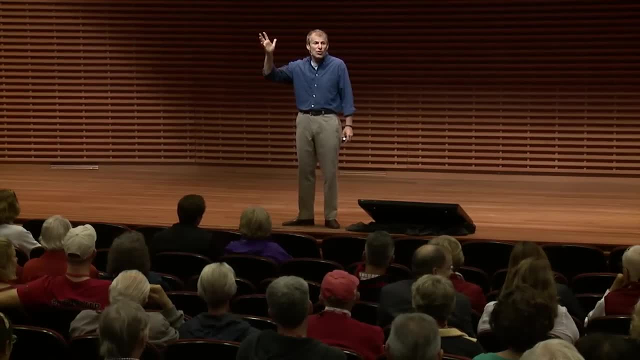 And there is no way to get it right. Just doing it gets it right. Okay, So let's try this now. We are going to play this game twice Again. it's for 30 seconds, If you are willing and able. 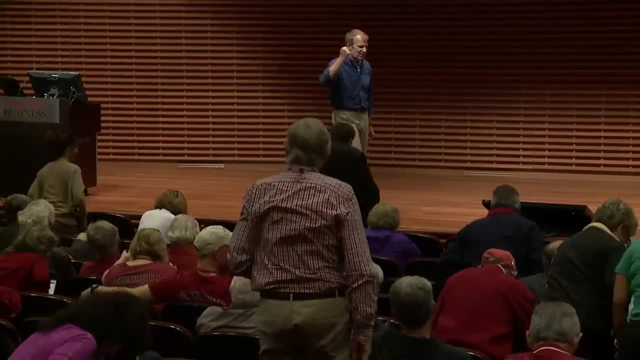 will you please stand up? You can do this seated, by the way, But if you are willing and able, let's stand up. Okay, In a moment. I am about to say go, And I would like for you to point at anything around here. 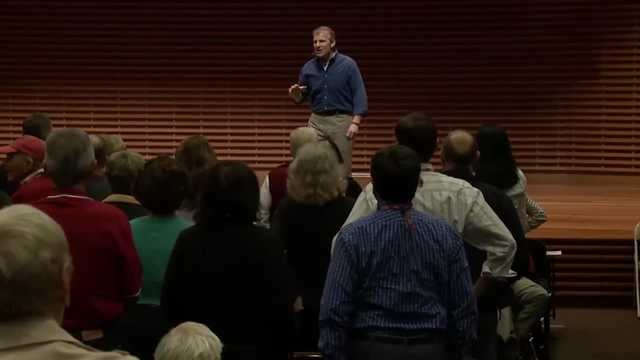 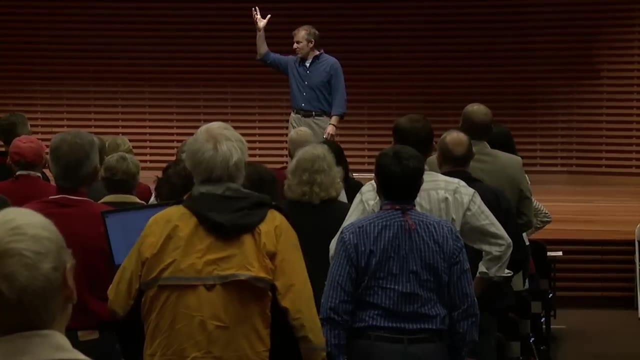 including me. It's okay to point at me- I hope it's not a bad thing you say when you point at me- But point at different things and loudly and proudly call this game. Call them different than what they are Ready. 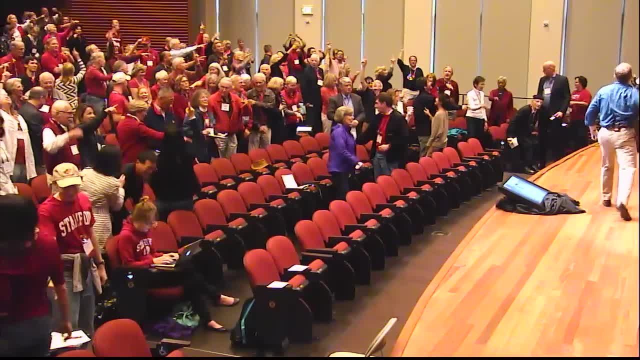 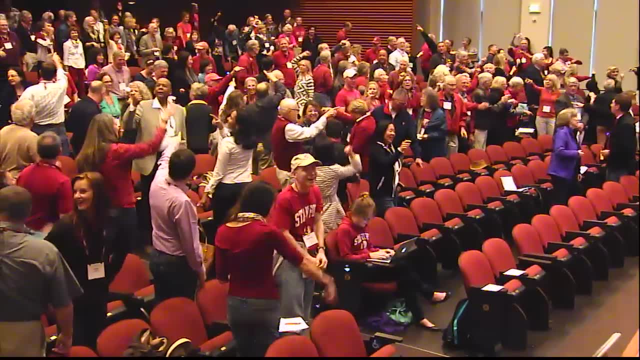 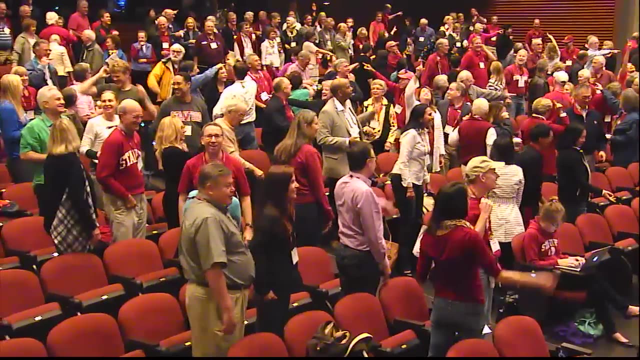 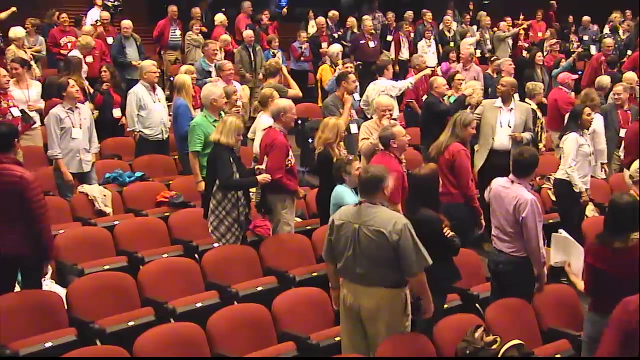 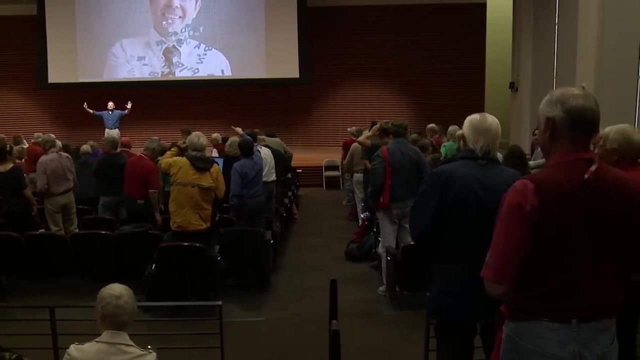 Begin: Porcupine, California, Salt shaker Car Library Tennis racket- Purple, Orange, Putrid Hello Time Time You can stay standing because in the mere moments we are going to do it again. So if you are comfortable standing, 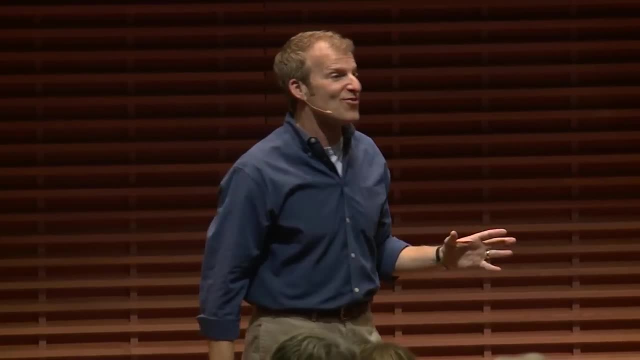 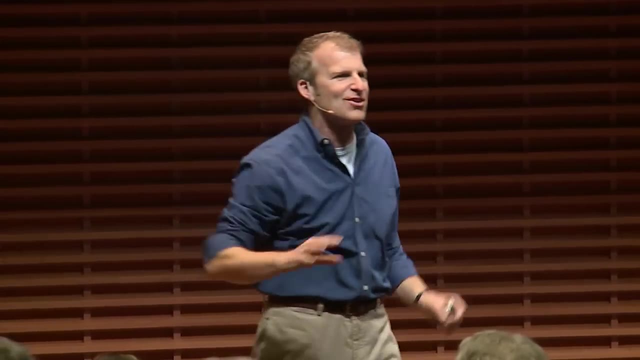 we are about to do it again. First, thank you. That was wonderful. I heard great words being called out. It was fun, And some of you in the back were doing it in sync, So it looked like you were doing some 70's disco dance. 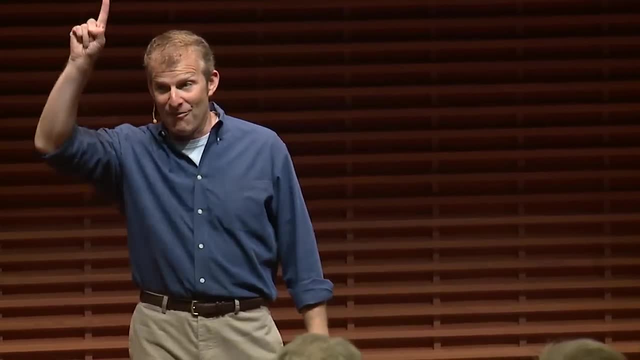 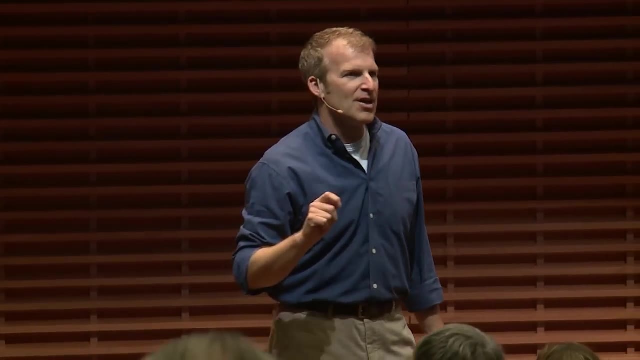 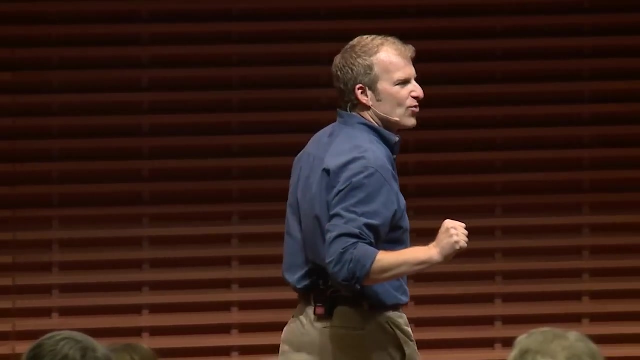 It was awesome. This was great. Now let me ask you just a few questions. Did you notice anything about the words that you were saying? did we find patterns, perhaps? maybe some of you were going through fruits and vegetables. a few of you were going through things that started with the letter a right that's your. 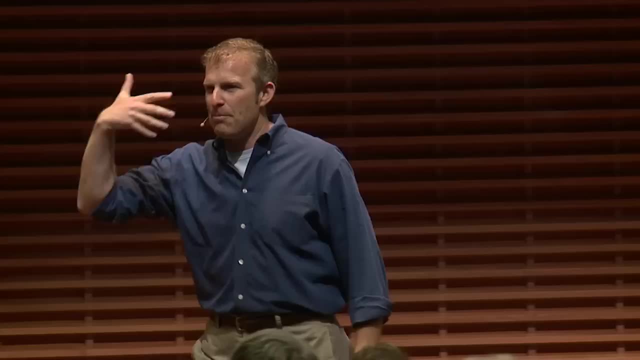 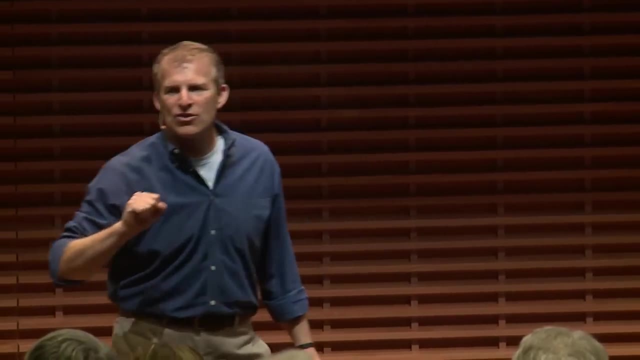 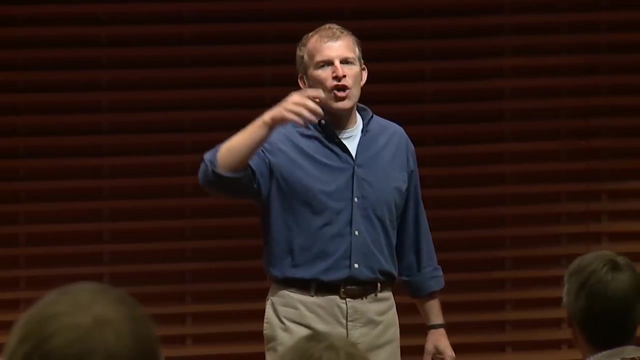 let me ask you just a few questions. Did you notice anything about the words that you were saying? Did we find patterns, perhaps? Maybe some of you were going through fruits and vegetables. A few of you were going through things that started with the letter A right That's your. 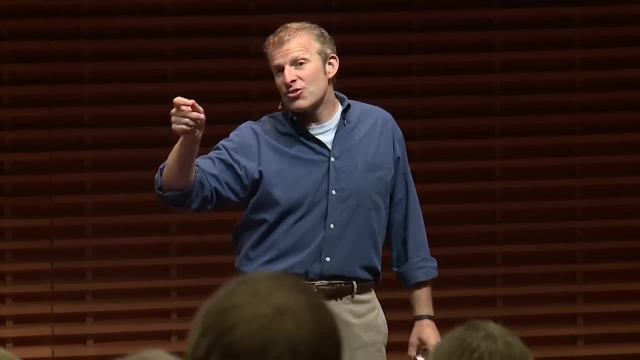 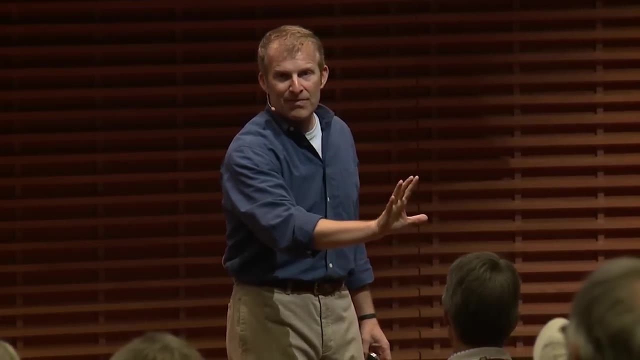 brain saying: okay, you told me not to stockpile, so I'm going to try to be a little more devious and I'm going to give you patterns. okay, Same problem When we teach that class- I told you about that improvisationally speaking class- we like to say: your brain is there to help you. 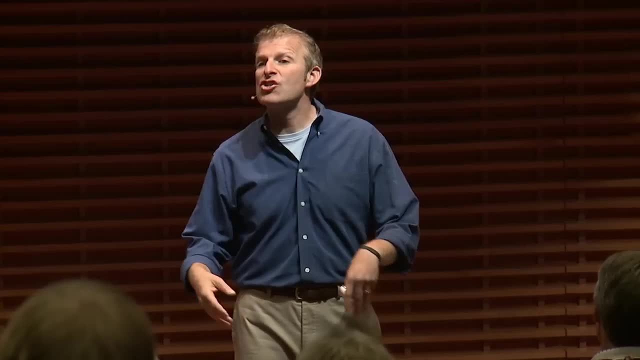 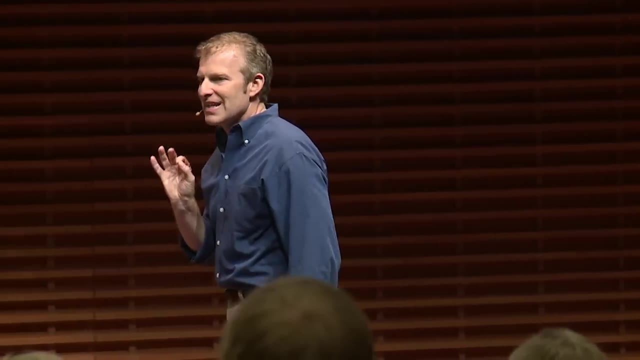 These things it's doing have helped you be successful. but, like a windshield wiper, we just want to wipe those suggestions away and see what happens. okay, So we're going to do this activity again This time. try the best you can to thank your brain if it provides you with patterns. 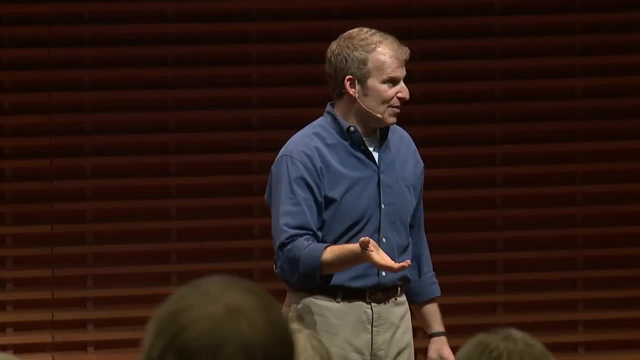 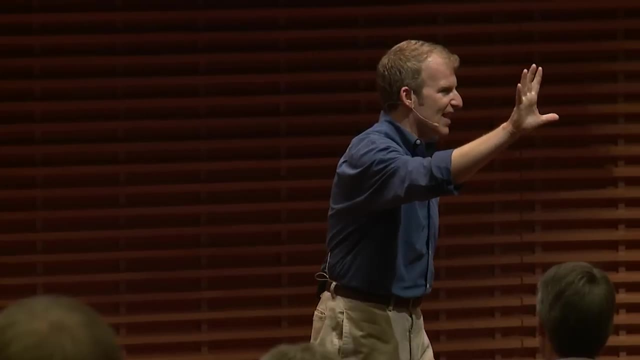 or stockpiles and just say thank you, brain, and disregard them, okay. So let's see what happens when we're not stockpiling and we're not playing off patterns. We'll do this for only 15 seconds. See how this feels- Baby steps. 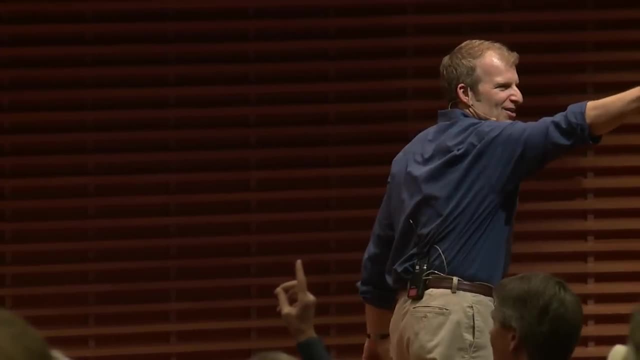 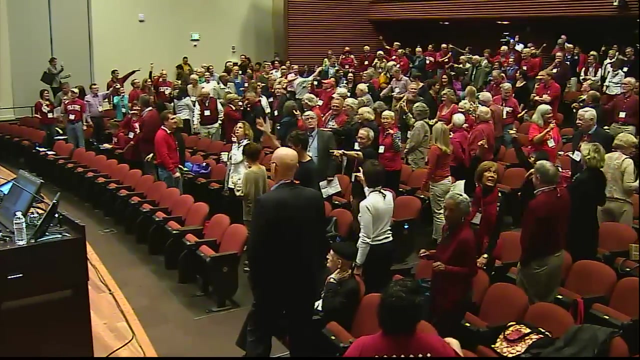 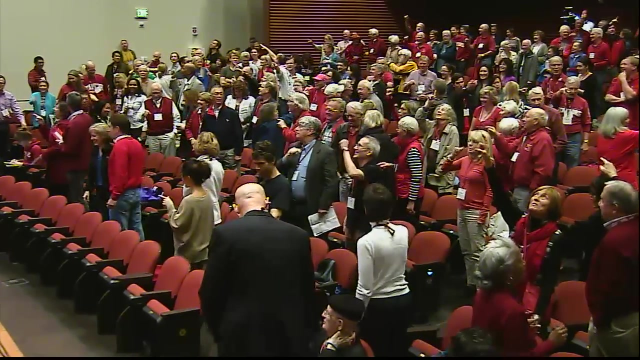 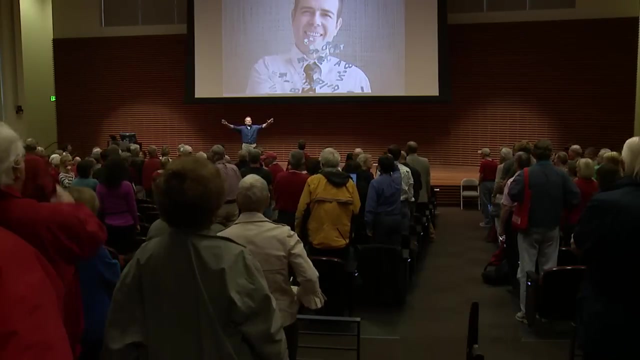 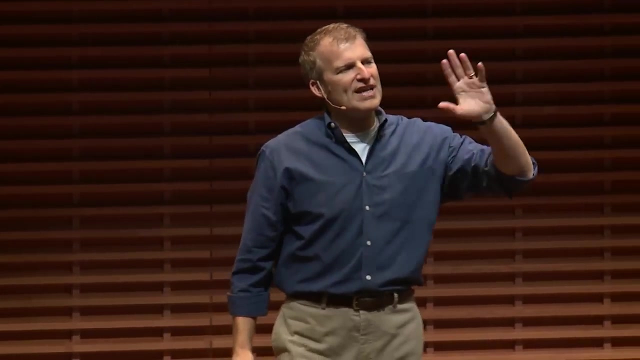 Ready Begin? Kodak Bicycle chain Skateboard- Bananas, Purple- Putrid Time Time. Please have a seat. Thank you again. The difference between the second time and the first time, Yes, Was it a little easier that? 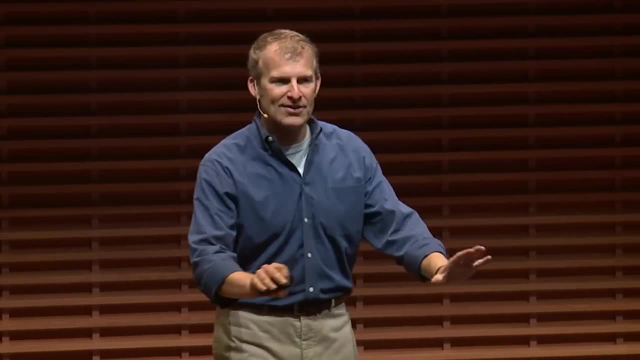 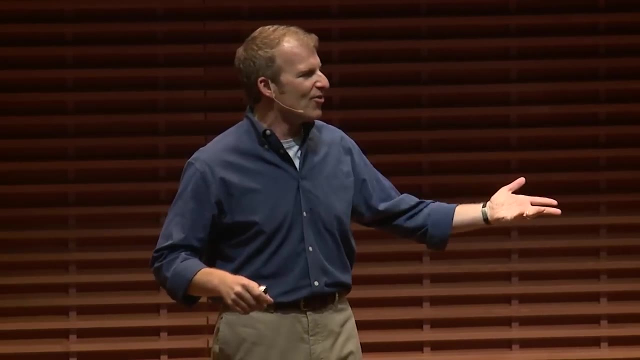 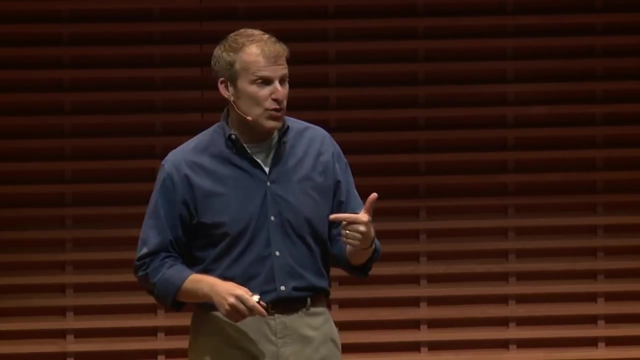 second time. No, That's okay, We're just starting. These skills are not like a light switch. It's not like you learn these skills and then, all of a sudden, you can execute on them. This is a wonderful game. This is a wonderful game to train your brain to get out of its own way. You can play this game. 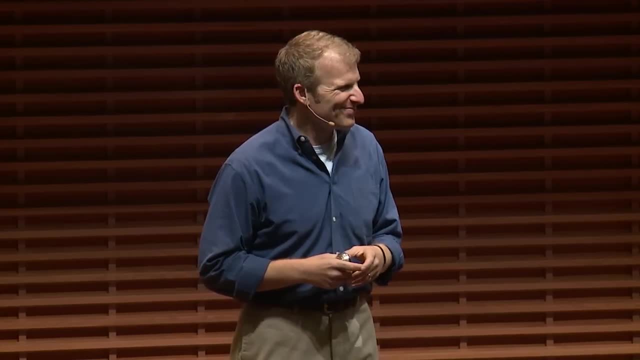 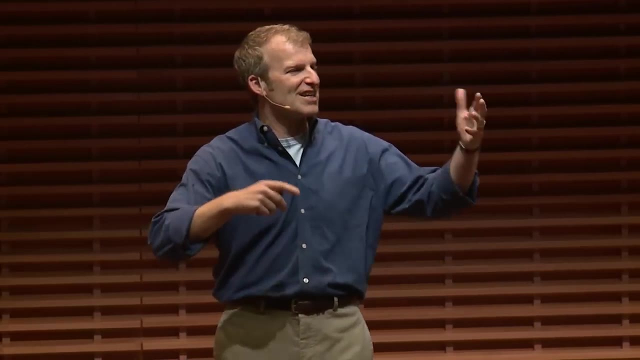 anywhere, anytime. I like to play this game when I'm sitting in traffic. Makes me feel better. I shout things out. They're not the naughty things that I want to be shouting out, but I shout out things and it helps. You're training yourself to get out of your own way. You're working. 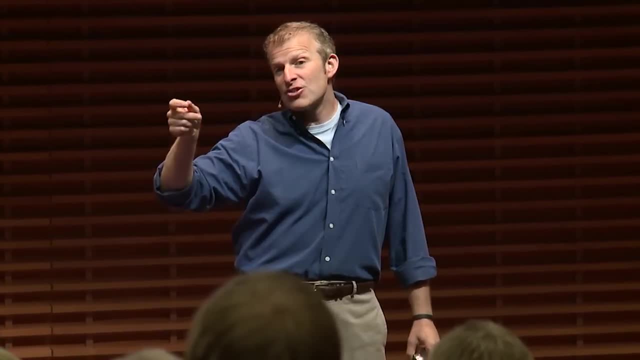 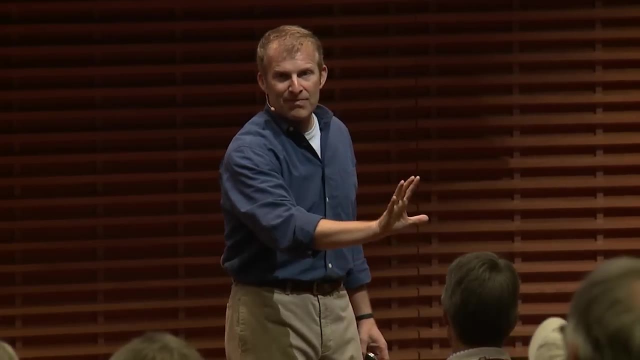 brain saying: okay, you told me not to stockpile, so i'm going to try to be a little more devious and i'm going to give you patterns. okay, same problem when we teach that class. i told you about that improvisationally speaking class. we like to say: your brain is there to help you. 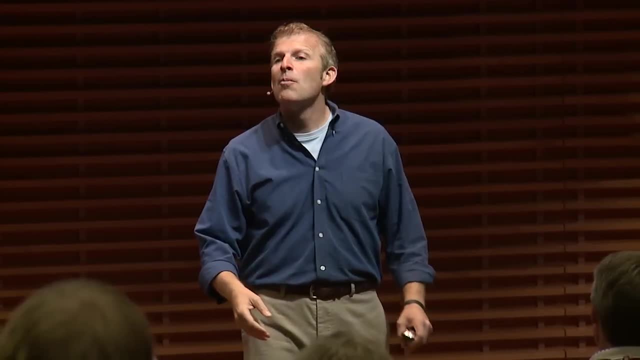 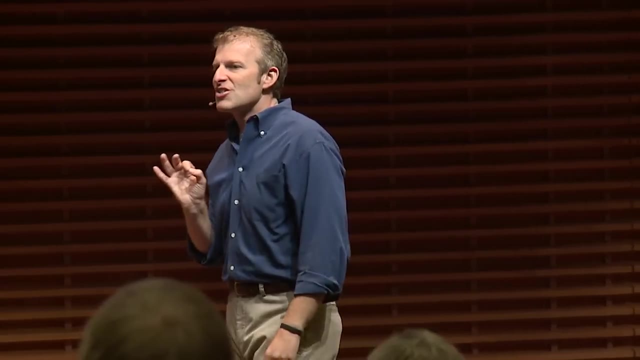 these things it's doing have helped you be successful, but, like a windshield wiper, we just want to wipe those suggestions away and see what happens. okay, so we're going to do this activity again this time. try the best you can to thank your brain if it provides you with patterns. 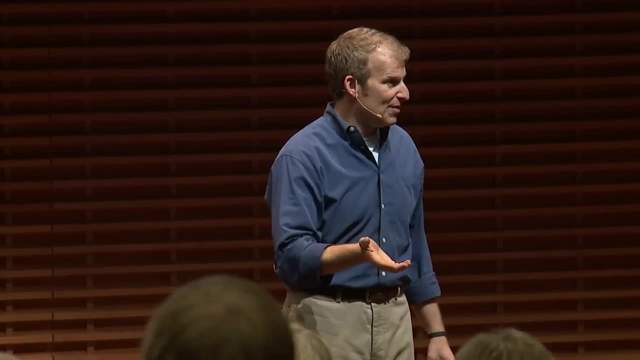 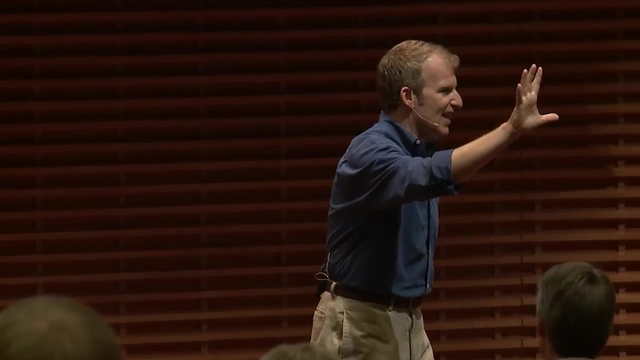 or stockpiles and just say thank you, brain, and disregard them. okay. so let's see what happens when we're not stockpiling and we're not playing off patterns. we'll do this for only 15 seconds. see how this feels. baby steps ready begin. 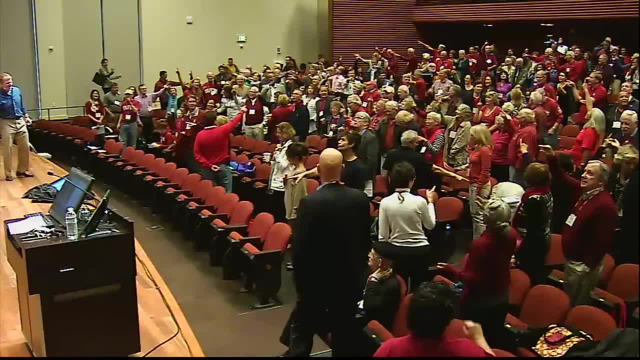 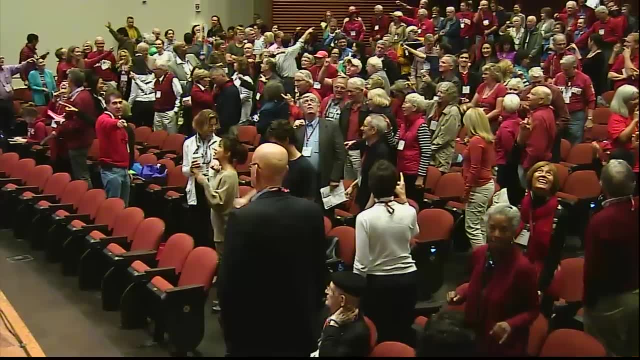 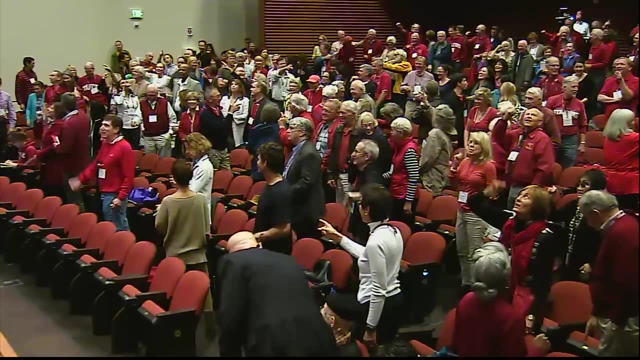 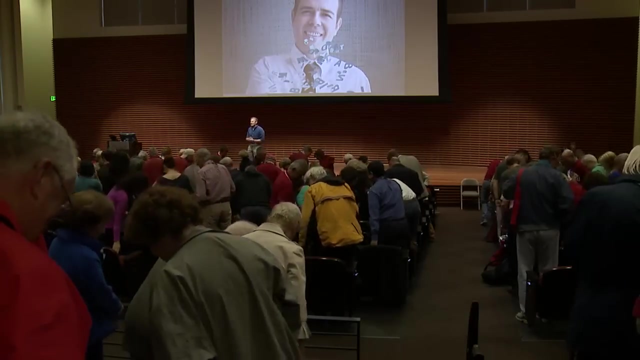 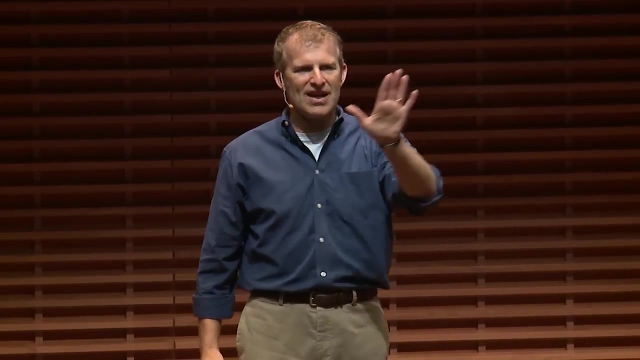 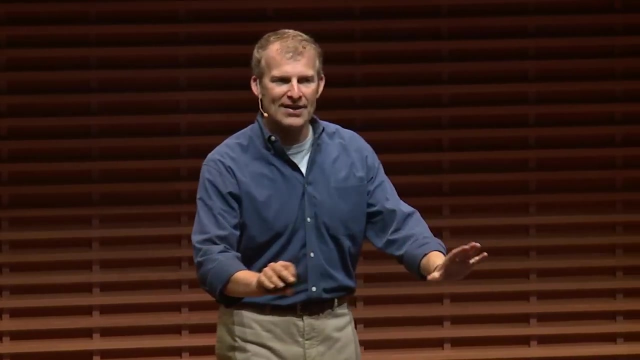 kodak bicycle chain skateboard- bananas- purple- putrid time. please have a seat. time, please have a seat. thank you again. did you notice a difference between the second time and the first time? yes, was it a little easier that second time? no, that's okay, we're just starting. these skills are not like a light. 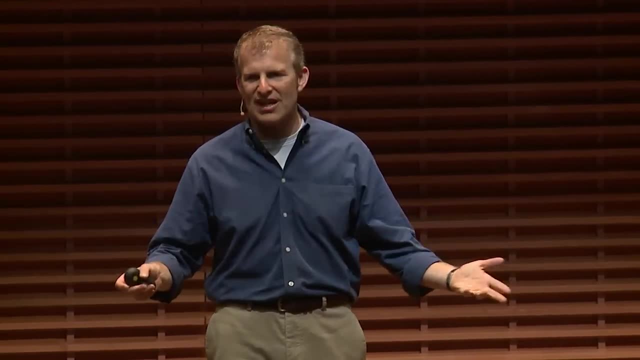 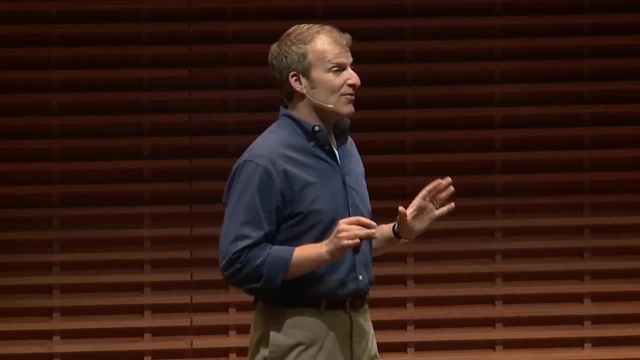 switch. it's not like you learn these skills, skills, and then all of a sudden you can execute on them. this is a wonderful game. this is a wonderful game to train your brain to get out of its own way. you can play this game anywhere, anytime. I like to play this game when I'm sitting in. 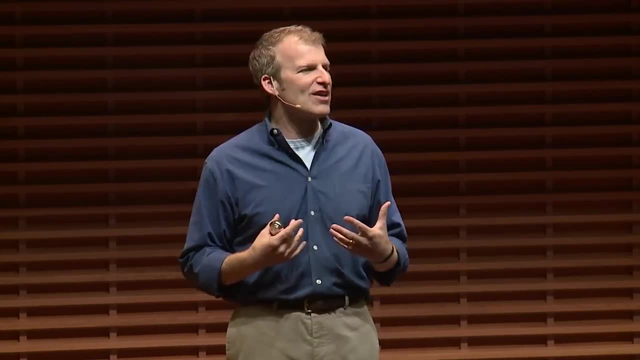 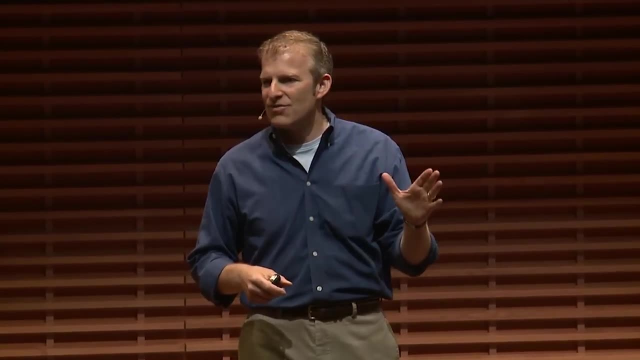 traffic makes me feel better than the. I shout things out. they're not the naughty things that I want to be shouting out, but I shout out things and it helps. you're training yourself to get out of your own way. you're working against the muscle memory that you've developed over the course of. 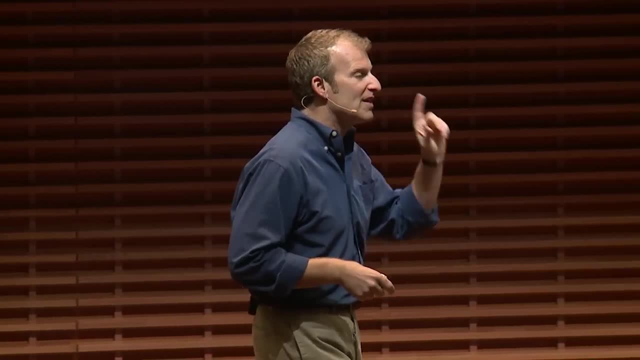 your life with a brain that acts very fast to help you solve problems, but in essence, in spontaneous speaking situations, you put too much pressure on yourself trying to figure out how to solve problems. you put too much pressure on yourself trying to figure out how to solve problems. you put too much. 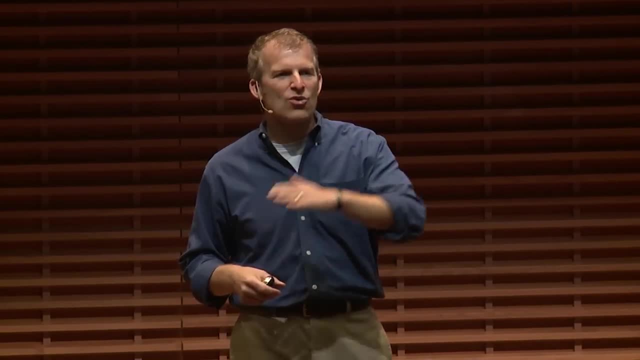 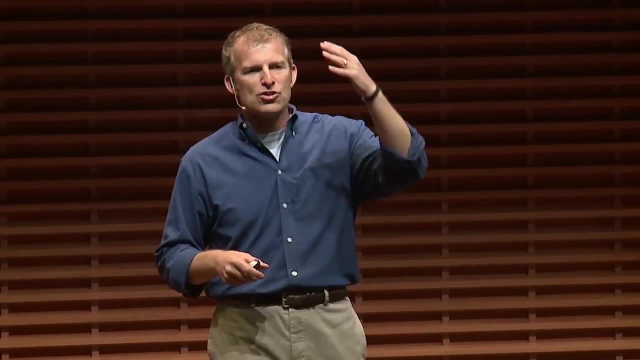 against the muscle memory that you've developed over the course of your life, with a brain that acts very fast to help you solve problems, But in essence, in spontaneous speaking situations you put too much pressure on yourself trying to figure out how to get it right. So a game-like. 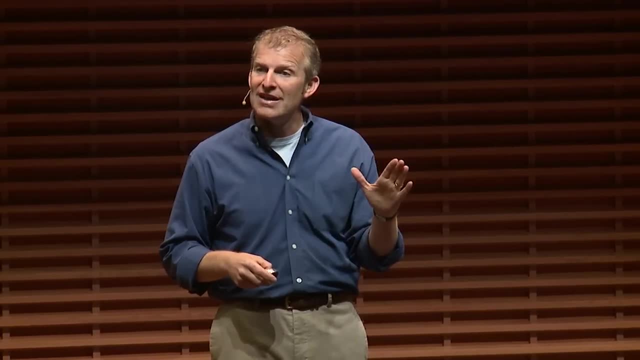 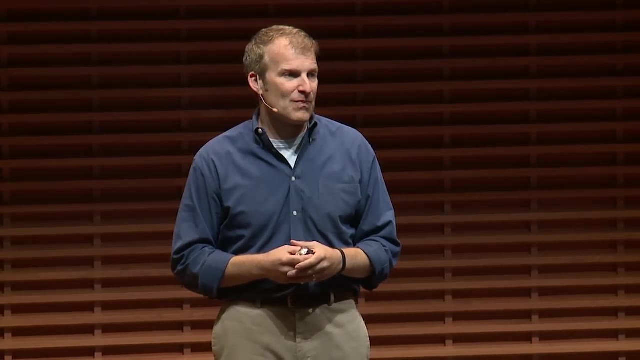 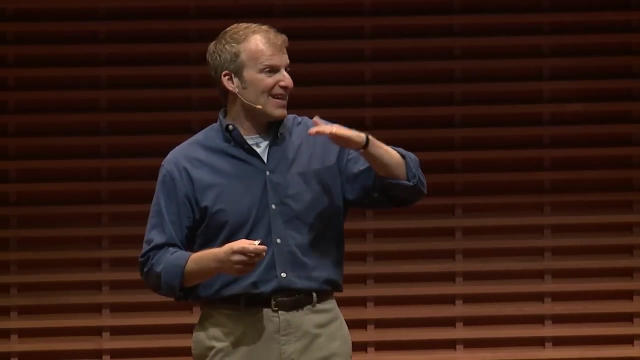 game, A game-like game, teaches us to get out of our own way. It teaches us to see the things that we do that prevent us from acting spontaneously. In essence, we are reacting rather than responding. To react means to act. again You've thought it and now you're acting on it. That takes too long, and 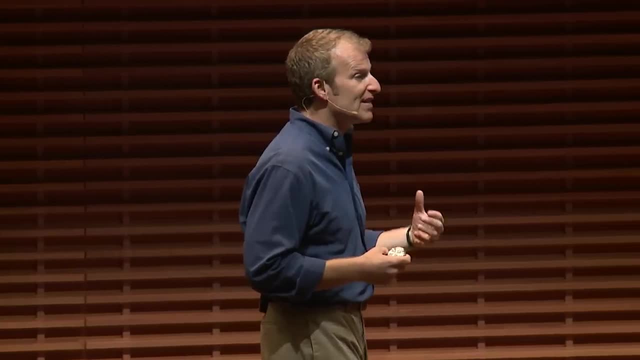 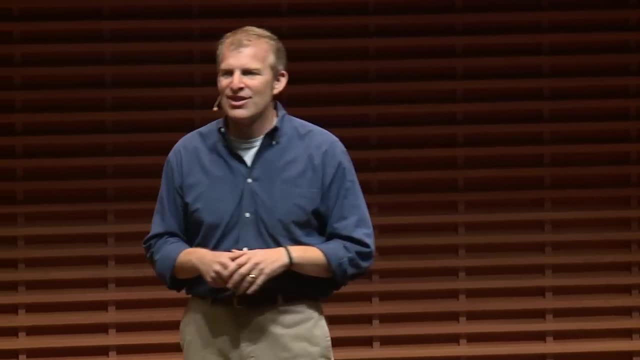 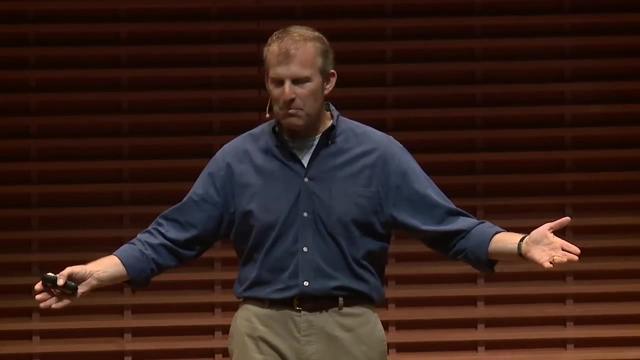 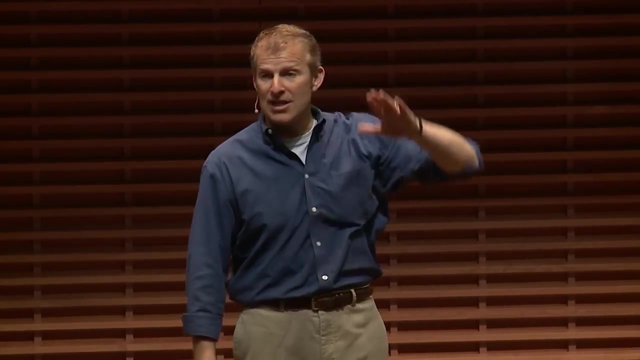 this and again. these maxims come from. improvisation is one of my favorite. Dare to be dull. And in a room like this, telling you dare to be dull is offensive and I apologize, But this will help. Rather than striving for greatness, dare to be dull. And if you dare to be dull, 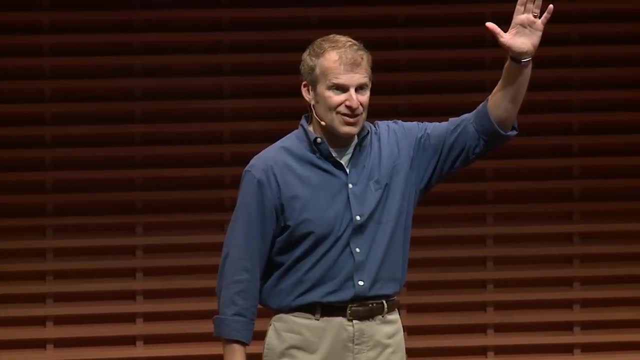 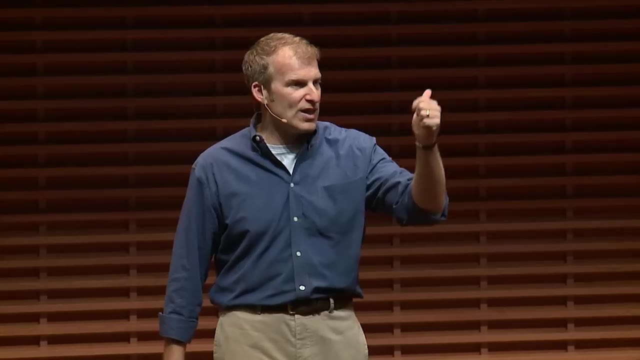 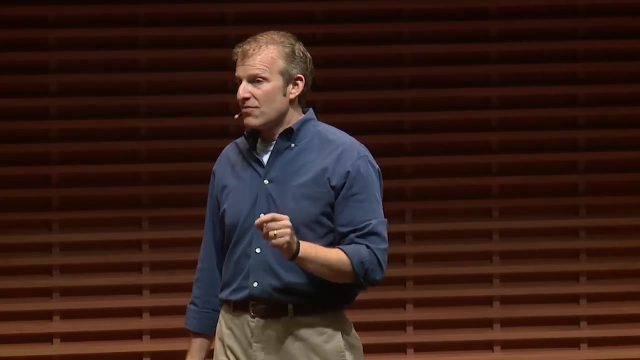 and allow yourself that you will reach that greatness. It's when you set greatness as your target that it gets in the way of you ever getting there, Because you over-evaluate, you over-analyze, you freeze up. So the first step in our process today is to get out of 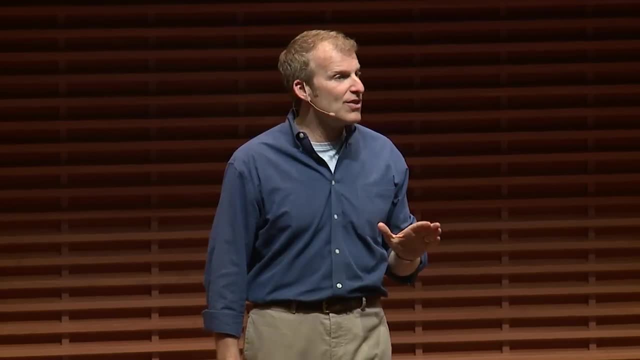 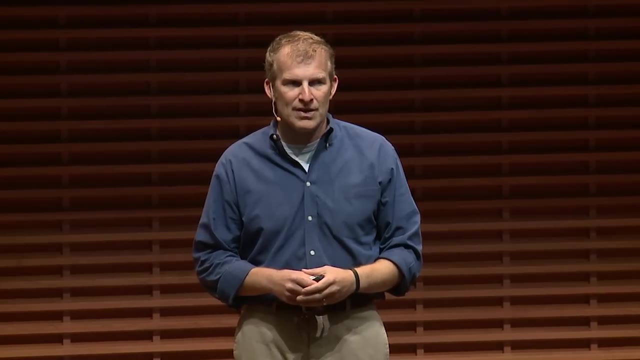 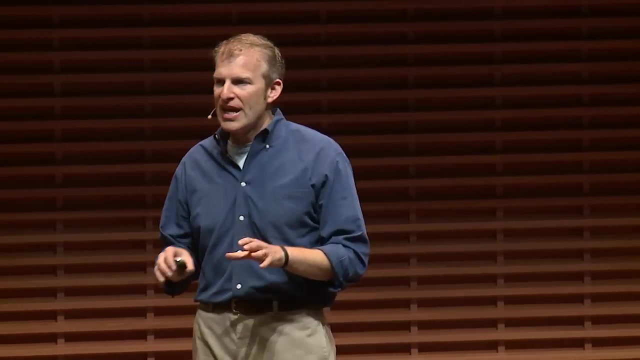 our own way. Dare to be dull. Easier said than done, But once you practice in a game just as simple as the one we practiced is a great way to do it. But that's not enough. Getting out of our own way is important, But the second step of our process has us change. 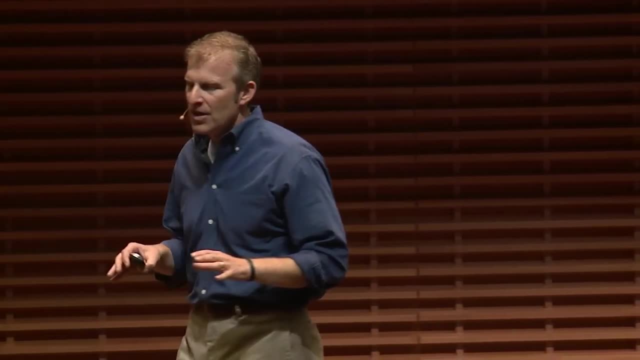 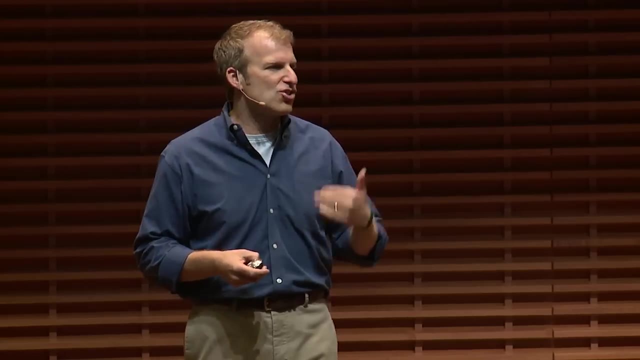 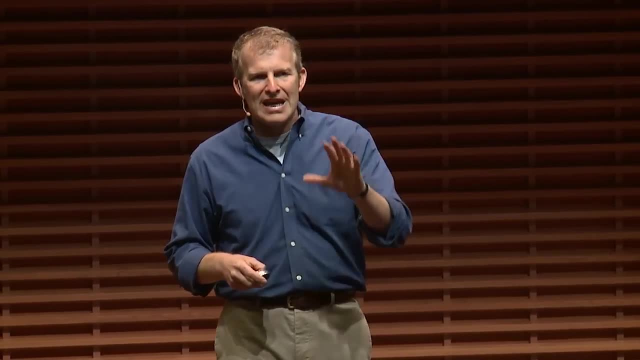 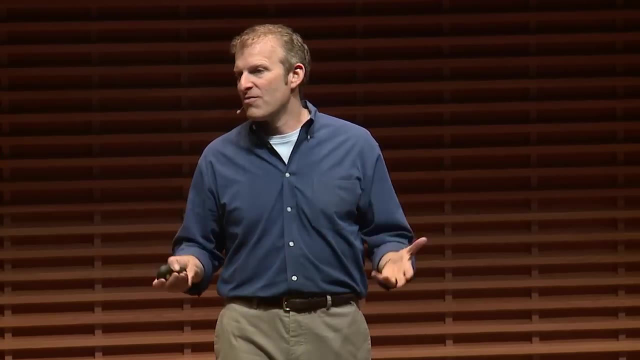 pressure on yourself trying to figure out how to solve problems. you put too much pressure on yourself how to get it right. so a game like this teaches us to get out of our own way. it teaches us to see the things that we do that prevent us from acting spontaneously. in essence, we are reacting rather 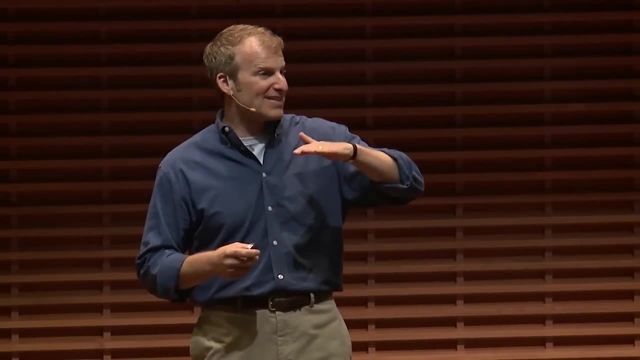 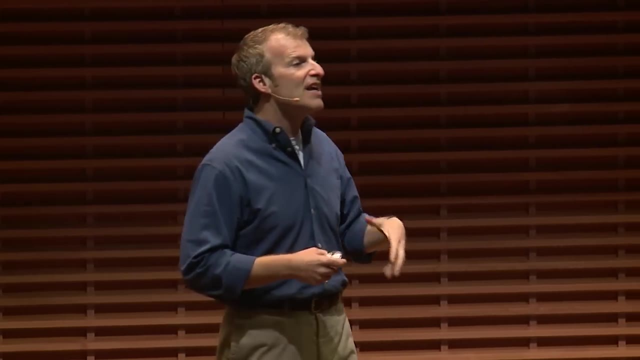 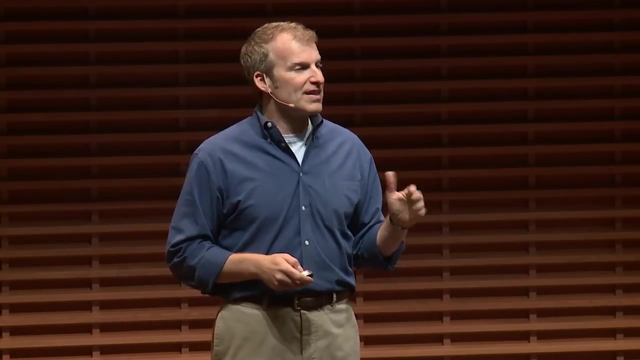 than responding. to react means to act. again, you've thought it and now you're acting on it. that takes too long and it's too thoughtful. we want to respond in a way that's genuine and authentic. so the maxim I would like for you to take from this and again- these maxims come from improvisation. 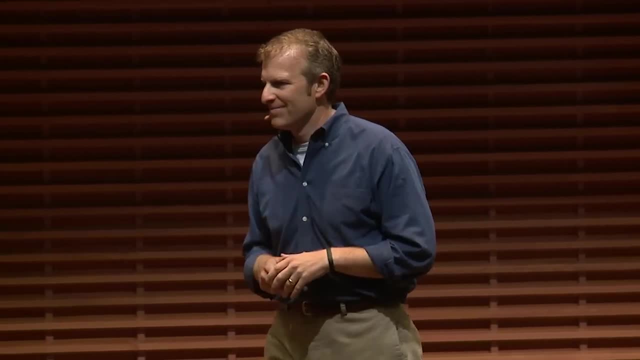 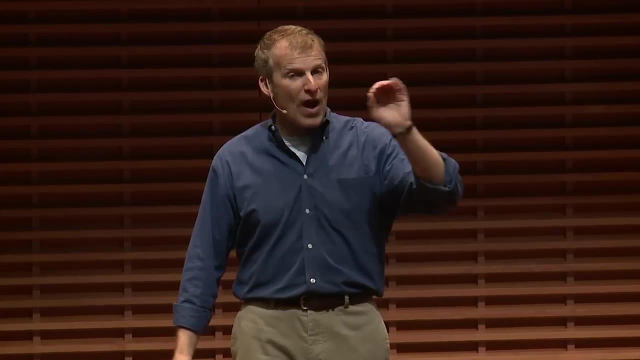 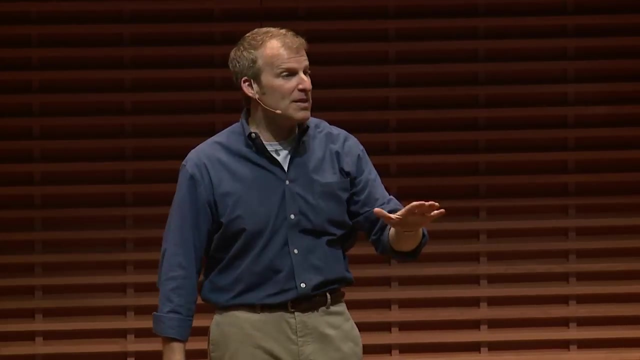 is one of my favorite. dare to be dull, and in a room like this, telling you dare to be dull is offensive and I apologize, but this will help. rather than street striving for greatness, dare to be dull. and if you dare to be dull and allow yourself that, you will reach that greatness. 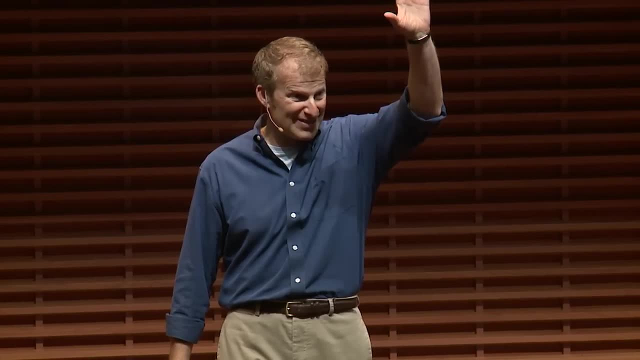 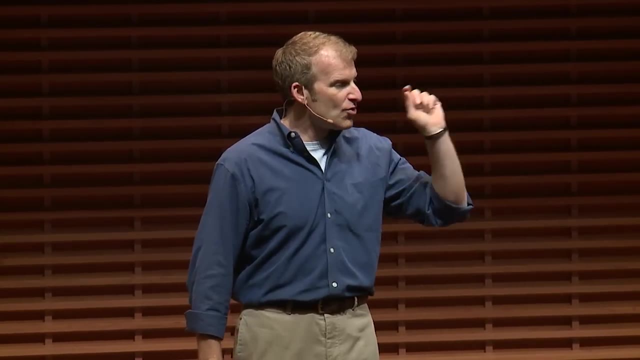 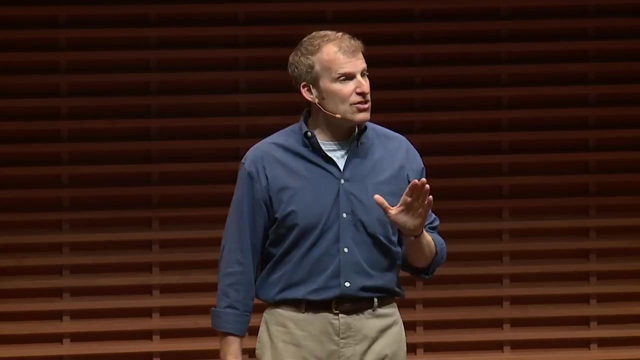 it's when you set greatness as your target that it gets in the way of you ever getting there, because you over evaluate, you over analyze, you freeze up. so the first step in our process today is to get out of our own way. dare to be dull, easier. 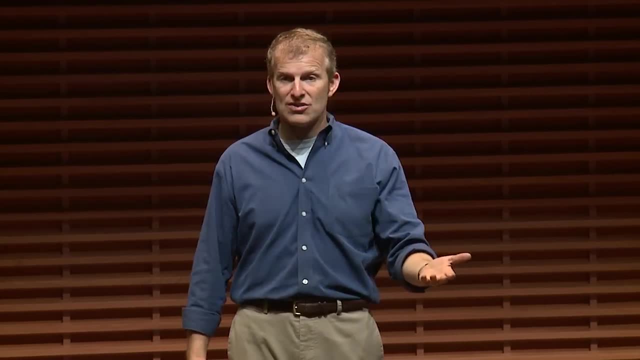 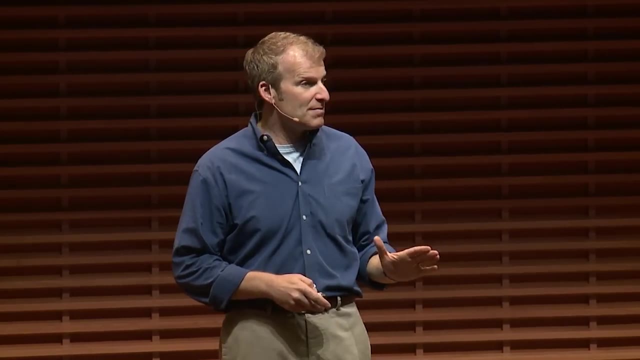 said than done, but once you practice in a game just as simple as the one we practiced is a great way to do it. but that's not enough. getting out of our own way is important, but the second step of our process has us change how we see the situation and how we see the situation and how we see the. 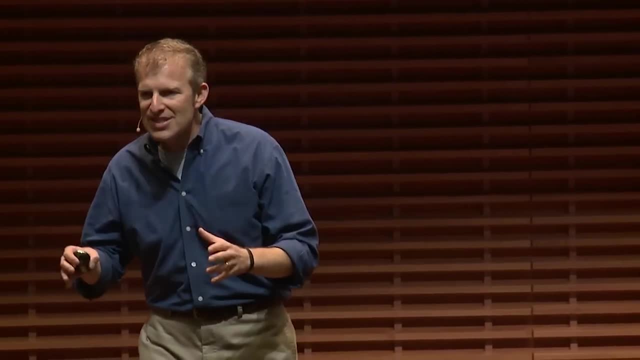 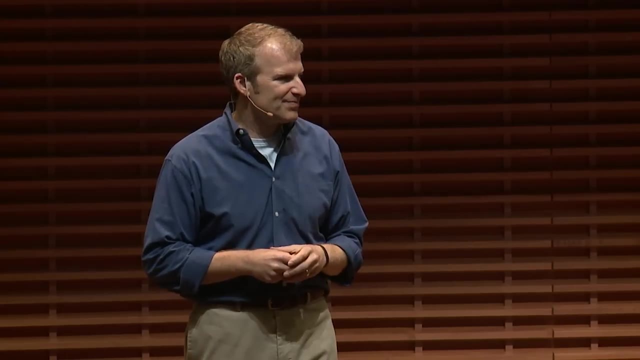 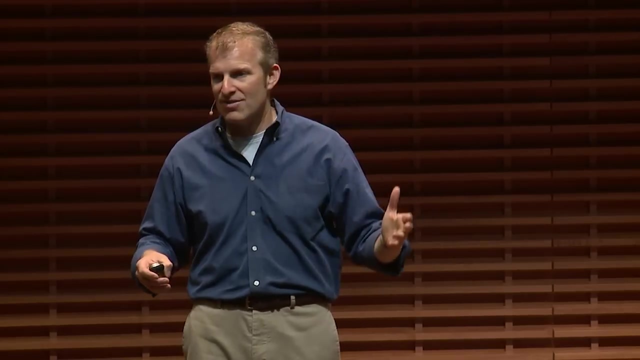 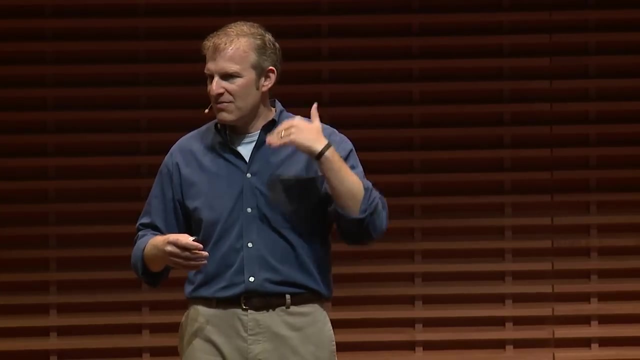 situation we find ourselves in. we need to see the speaking opportunity that we are a part of as an opportunity rather than a challenge and a threat. when I coach executives on Q&A skills, when they go in front of the media or whatever investors, they see it as an adversarial experience- me versus them. 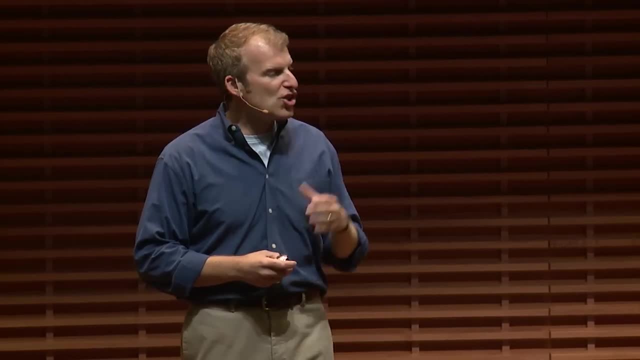 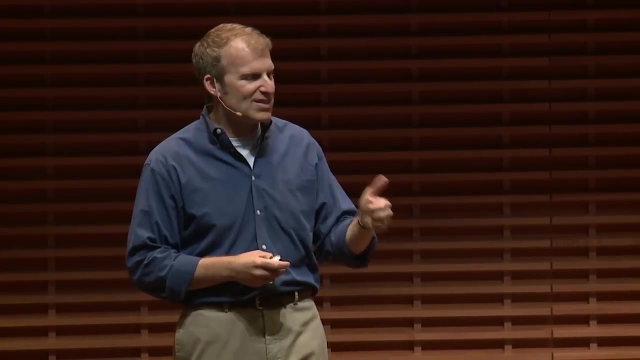 and one of the first things I work on is change the way you approach it. a Q&A session, for example, is an opportunity for you. it's an opportunity to clarify, it's an opportunity to understand what people are thinking. so if we look at it as an opportunity, it feels very. 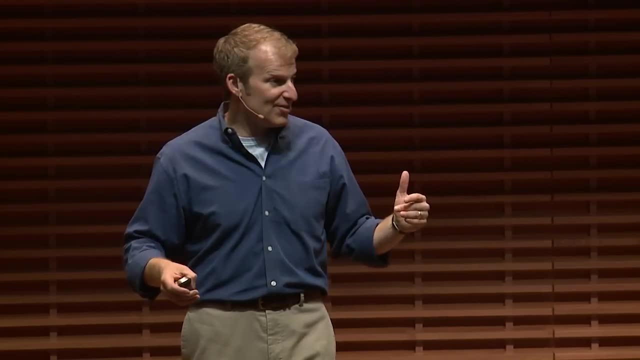 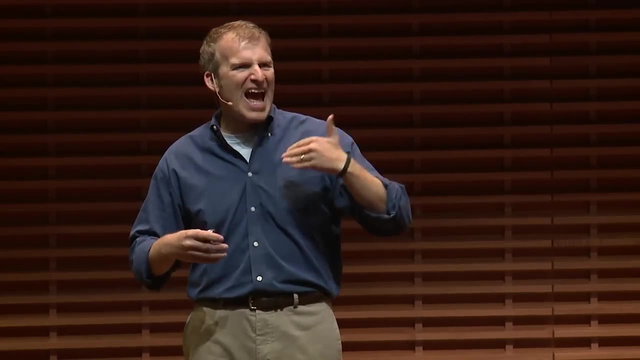 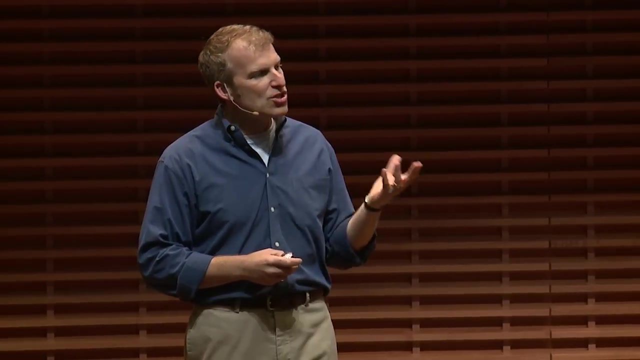 I coach executives on Q&A skills. when they go in front of the media or whatever investors, they see it as an adversarial experience- Me versus them- And one of the first things I work on is change the way you approach it. Change the way you approach it. Change the 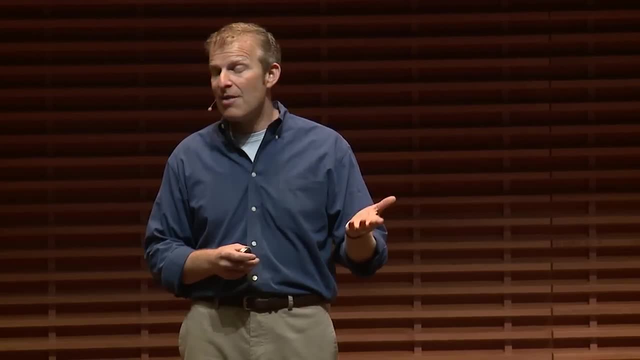 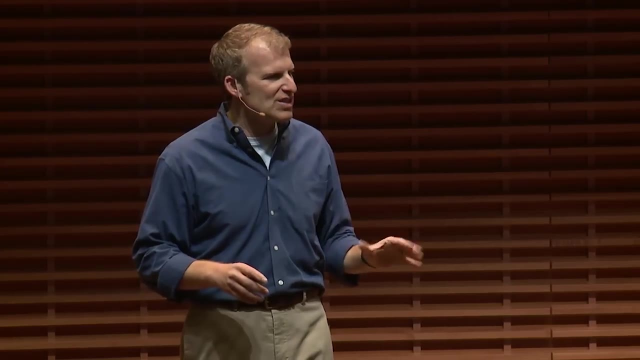 way you approach it. A Q&A session, for example, is an opportunity for you. It's an opportunity to clarify, It's an opportunity to understand what people are thinking. So if we look at it as an opportunity, it feels very different. We see it differently and therefore we have. 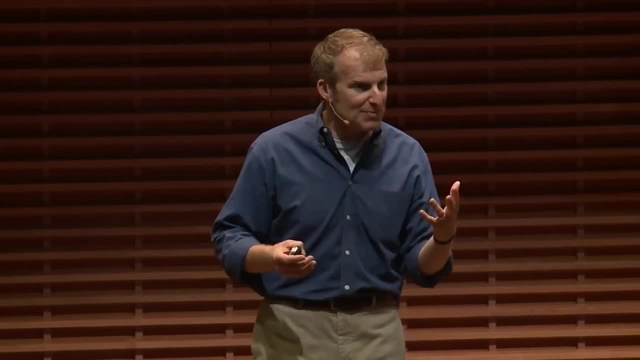 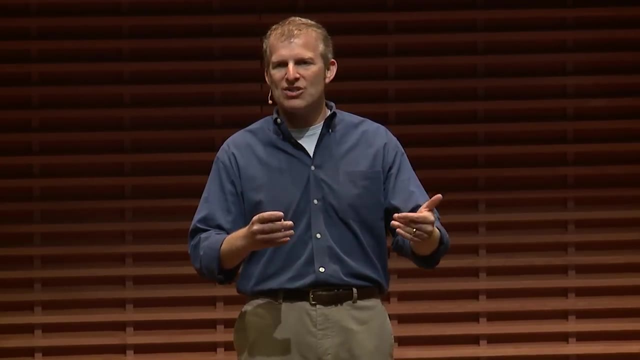 more freedom to respond. When I feel that you are challenging me, I am going to do the bare minimum to respond and protect myself. If I see this as an opportunity where I have a chance to explain and expand, I'm going to interpret it as an opportunity to respond. 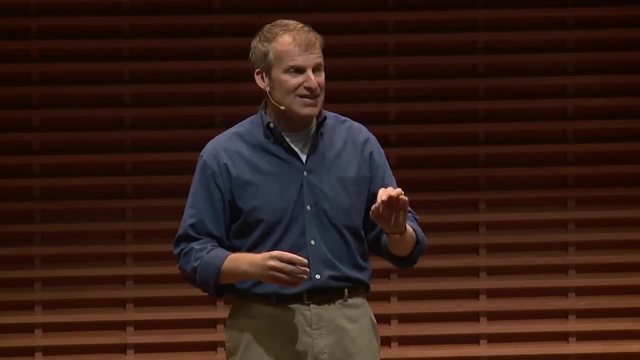 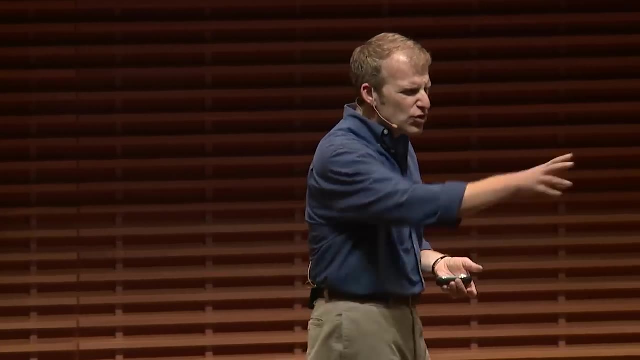 I'm going to interact differently with you, So spontaneous speaking situations are ones that afford you opportunities. So when you're at a corporate dinner and your boss turns to you and says: oh, you know him better than the rest, would you mind introducing him? 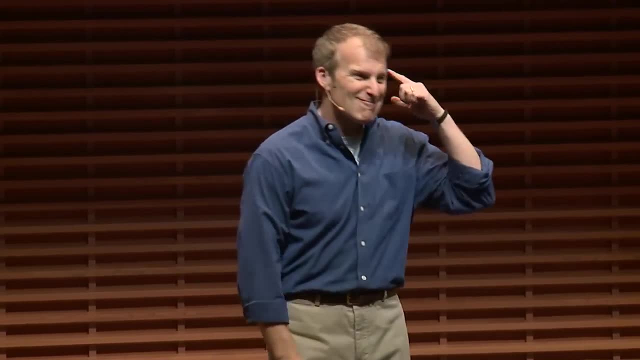 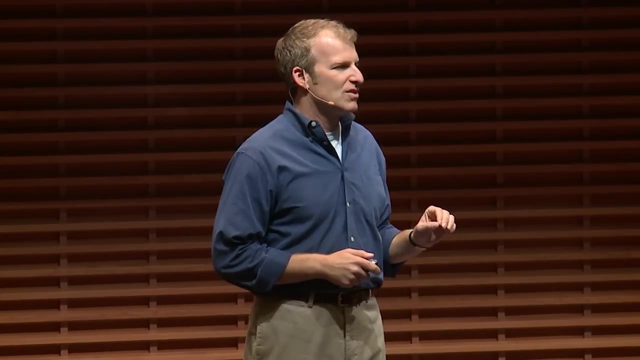 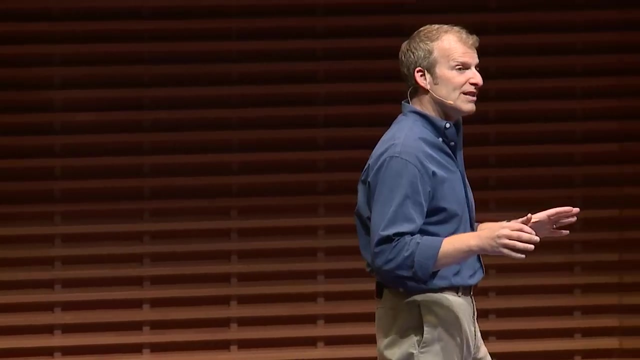 You say great. thank you for the opportunity. rather than right, I better get this right. So see things as an opportunity. I have a game to play to help us with this. This is a fun one. Holidays are approaching. We all in this room are going to give and receive gifts. 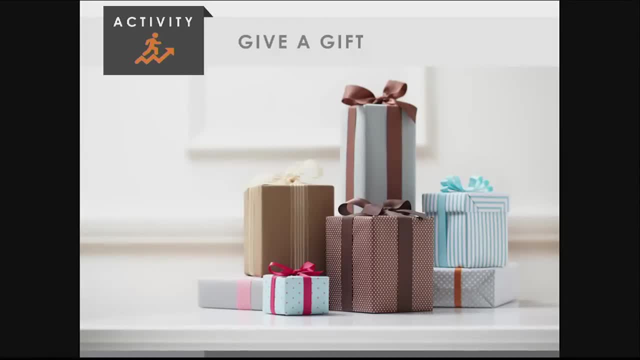 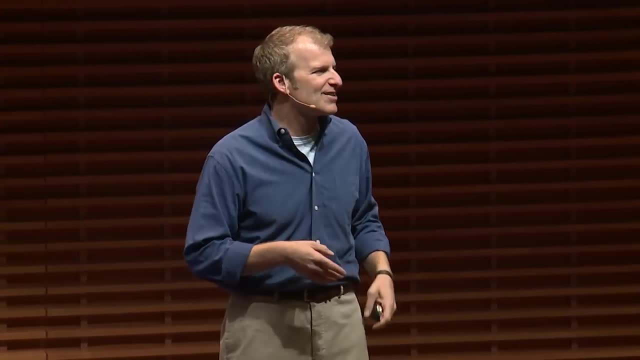 Here's how this game will work. It works best if you have a partner, So I'm hoping you can work with somebody sitting next to you. If there's nobody sitting next to you, turn around, introduce yourself- great way to connect. If not, you can play this game by yourself. 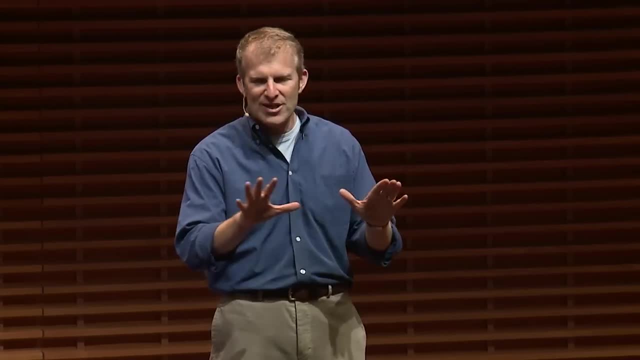 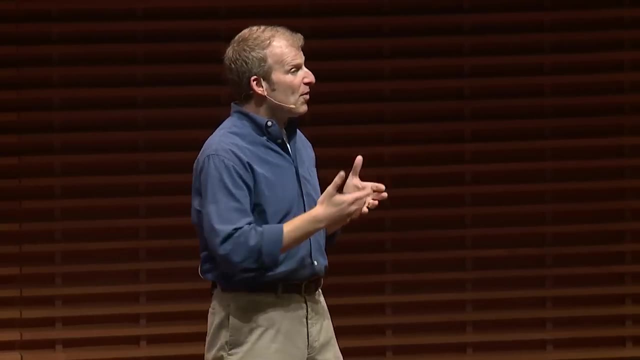 It's just a little harder and you can't do the second part of the game. So after I explain the game, this gives you a chance to get to know somebody. Here's how it works. If you have a partner, you and your partner are going to exchange. 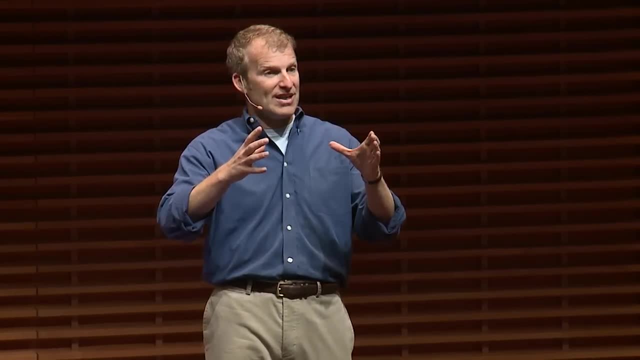 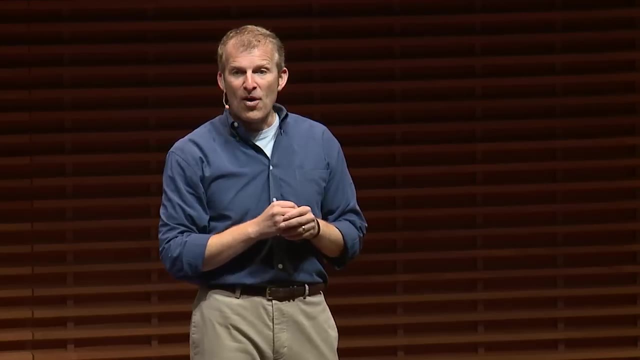 imaginary gifts. Pretend you have a gift. It can be a big gift, It can be a small gift- And you will give your gift to your partner. Your partner will take the gift and open it up and will tell you what you gave them, Because you have no idea. you just gave them a gift. 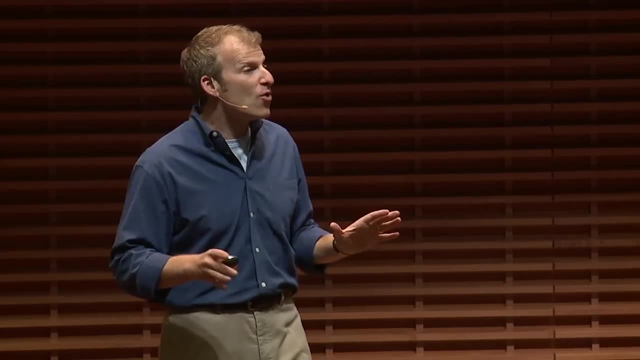 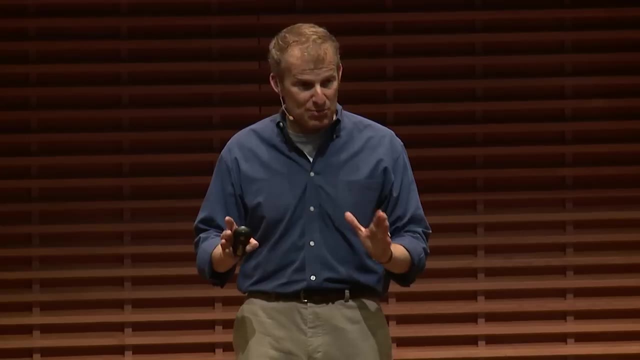 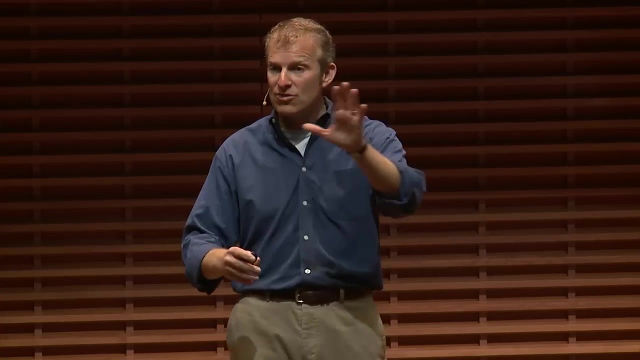 different. we see it differently and therefore we have more freedom to respond. when I feel that you are challenging me, I am going to do the bare minimum to respond and protect myself. if I see this as an opportunity where I have a chance to explain and expand, I'm going to interact. 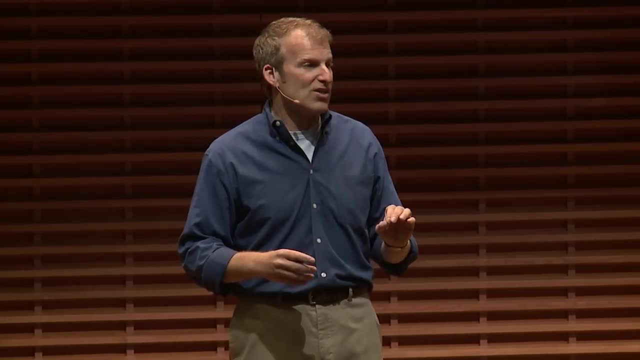 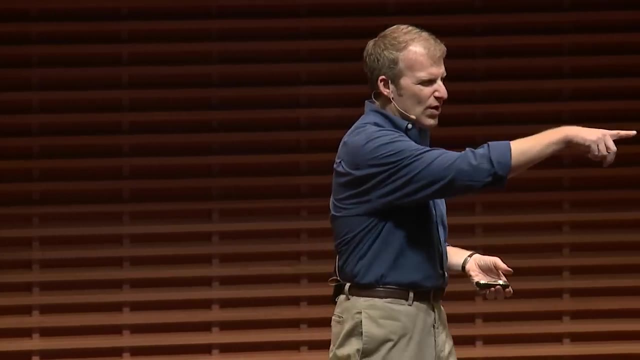 differently with you. so spontaneous speaking situations are ones that afford you opportunities. so when you're at a corporate dinner and your boss turns to you and says, oh, you know him better than the rest, would you mind introducing him? you say great, thank you for the opportunity, rather than 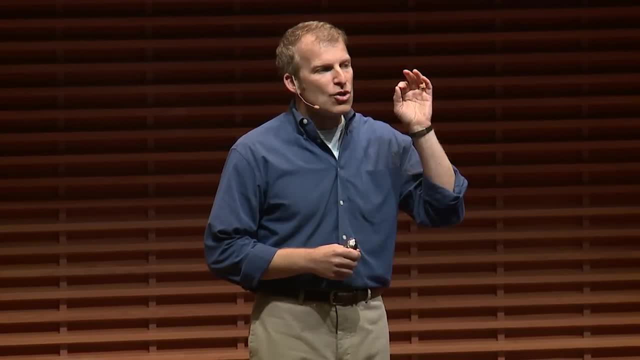 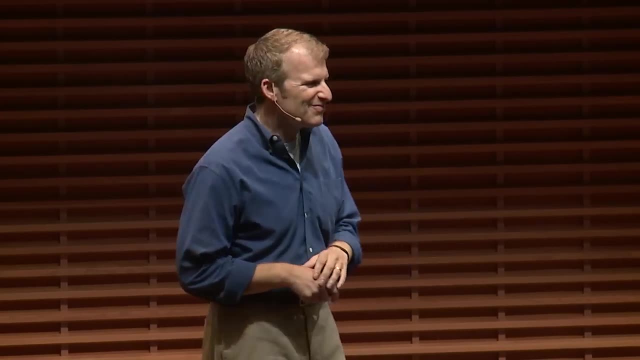 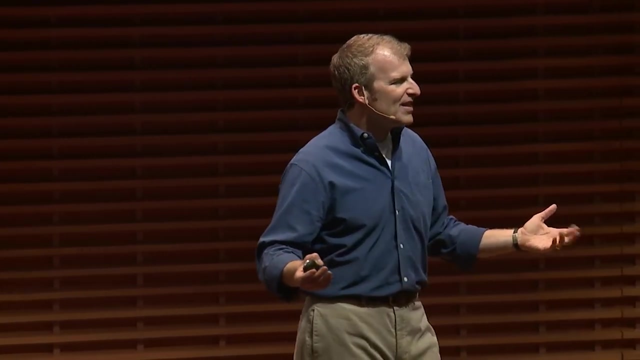 right. I better get this right, so see things as an opportunity. I have a game to play to help us with this. this is a fun one. the holidays are approaching. we all in this room are going to give and receive gifts. here's how this game will work. it works best if you have a partner, so I'm hoping you can work with somebody sitting next to. 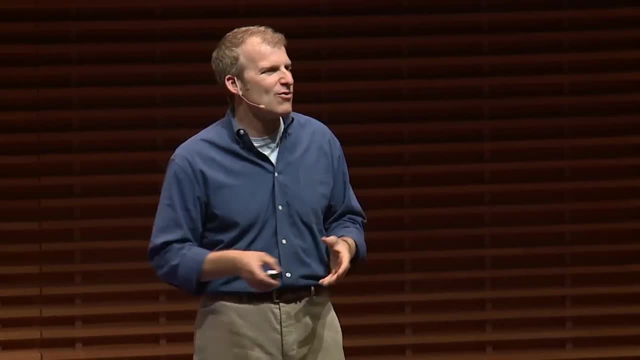 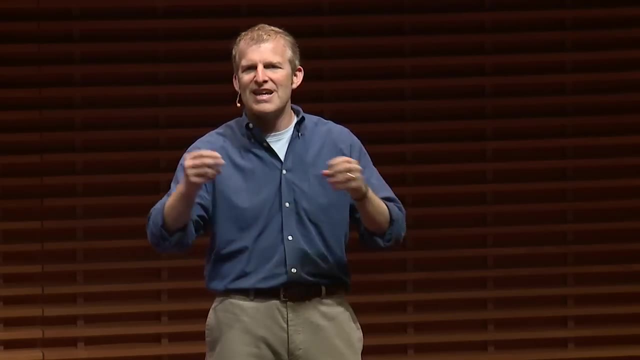 you. if there's nobody sitting next to you, you turn around, introduce yourself. great way to connect. if not, you can play this game by yourself. it's just a little harder and you can't do the second part of the game. so after I explain the game, give this. gives you a chance to to get to know somebody. 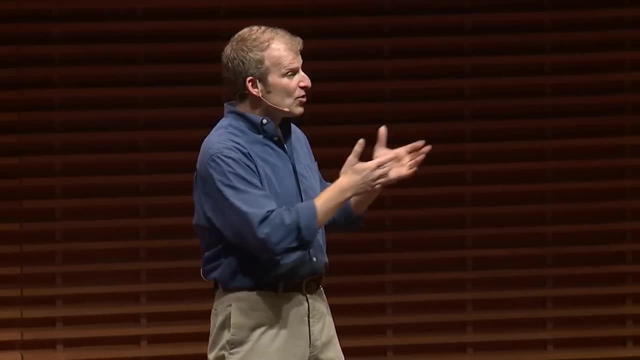 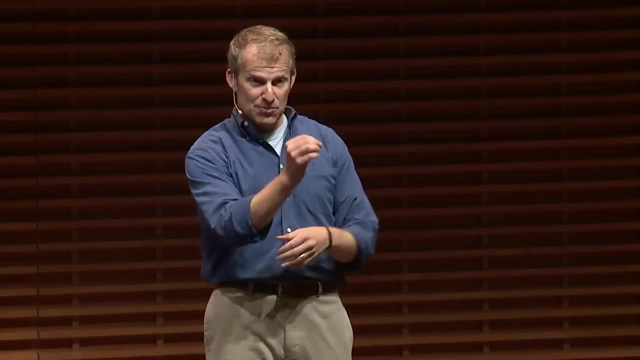 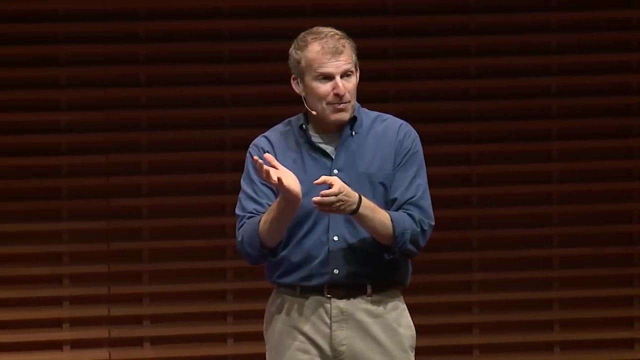 here's how it works. if you have a partner, you and your partner are going to exchange imaginary gifts. okay, pretend you have a gift. it can be a big gift, it can be a small gift and you will give your gift to your partner. your partner will take the gift and open it up and will tell: 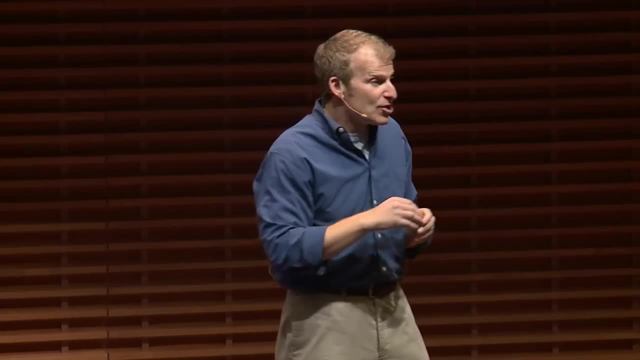 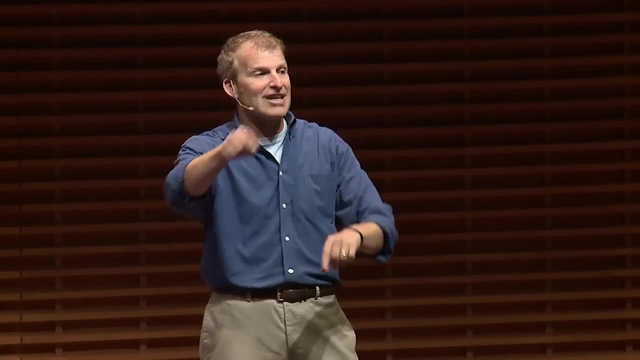 you what you gave them? because you have. no, you just gave them a gift. so you are going to open up the box and you're going to look inside and you are going to say the first thing that comes to your mind in the moment, not the thing you have all just thought of or the thing after that. remember, 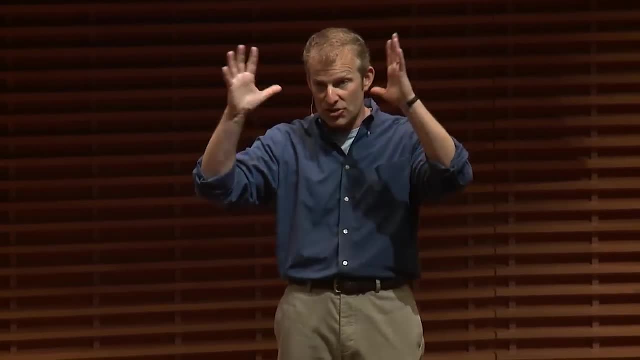 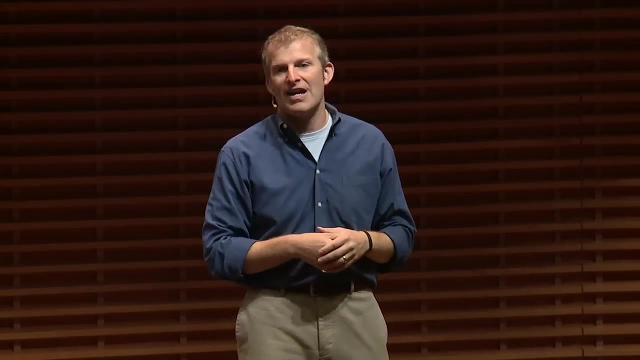 we talked about before. that still plays. that's still in play. okay, you're stockpiling. look in there. my favorite that I said somebody gave me this a gift during playing this game. I looked inside and I saw a frog leg. I don't know why I saw a frog leg, but that's what I said. that's the. 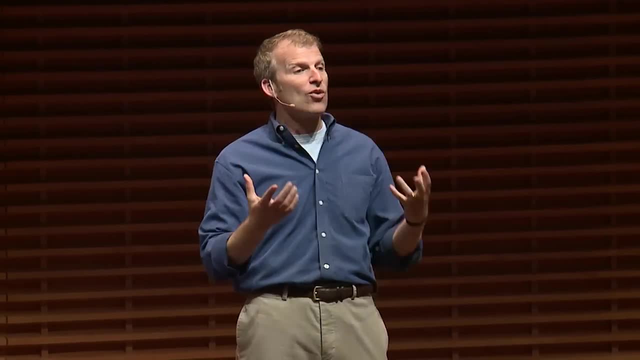 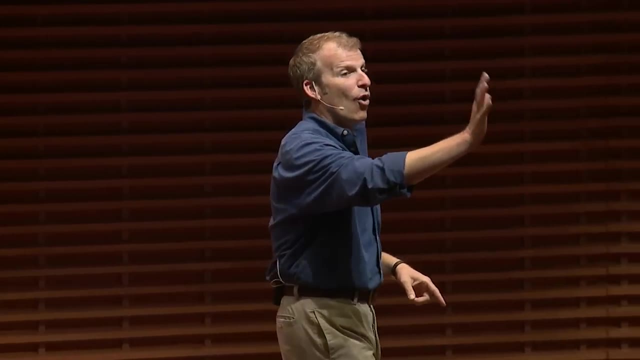 So you are going to open up the box and you're going to look inside and you are going to say the first thing that comes to your mind in the moment, Not the thing you have all just thought of Or the thing after that. Remember what we. 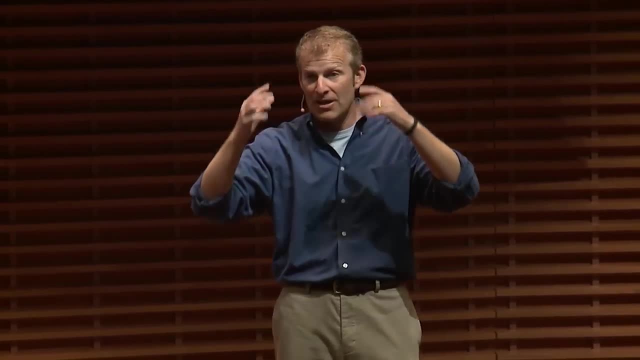 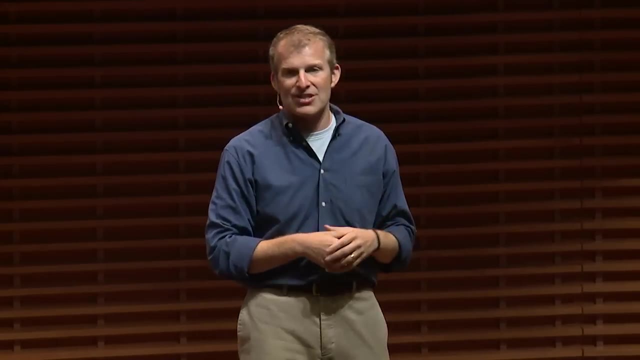 talked about before. that still plays. That's still in play. Okay, you're stockpiling. Look in there, My favorite that I said somebody gave me a gift during playing this game. I looked inside and I saw a frog leg. I don't know why I saw a frog leg, but that's what. 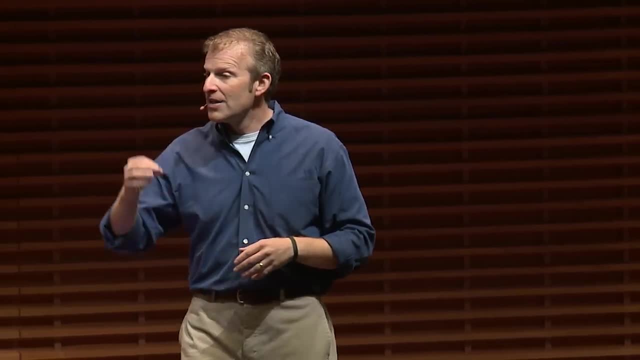 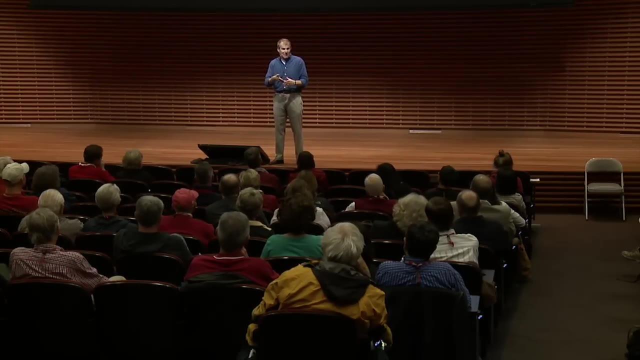 I said, That's the first part of the activity. Now the opportunity is twofold in this game. The opportunity is for you, the gift receiver, to name a gift. That's kind of fun, That's an opportunity, It's not a threat. But the real opportunity is for the gift giver because 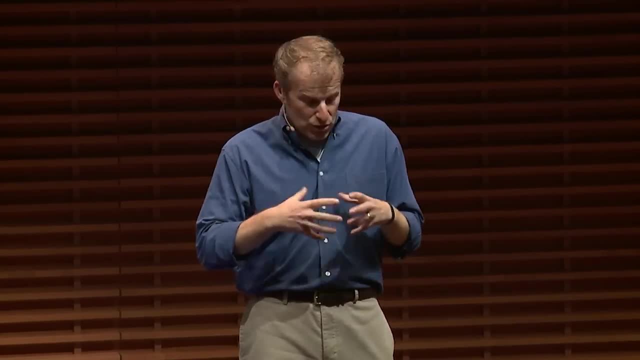 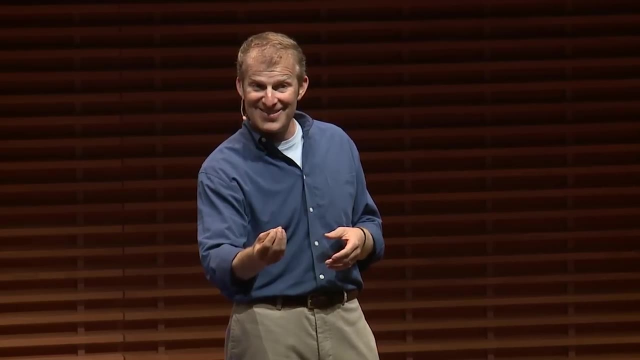 the gift giver then has to say: so you look and you say thank you for giving me a frog's leg, and the person will look at you and say I knew you wanted a frog's leg because. So, whatever you find, the person who has received it is going to say: absolutely, I'm so glad. 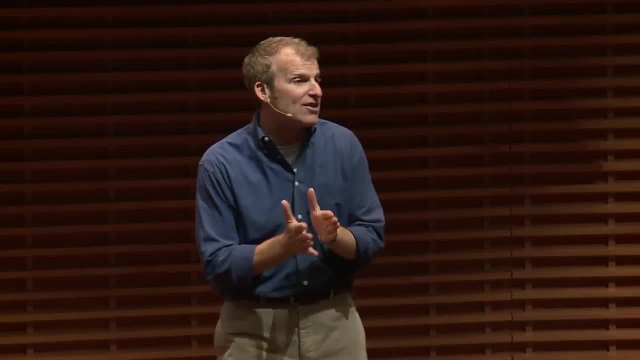 you're happy I got it for you because So you have to respond to whatever they say, right? What a great opportunity. Now some of you are sitting there going, oh, that's hard, I don't want to do it, I'm. 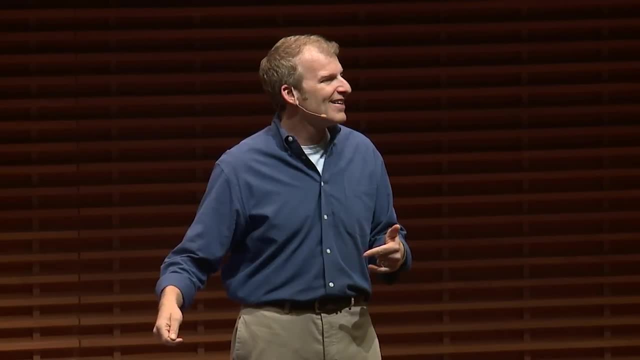 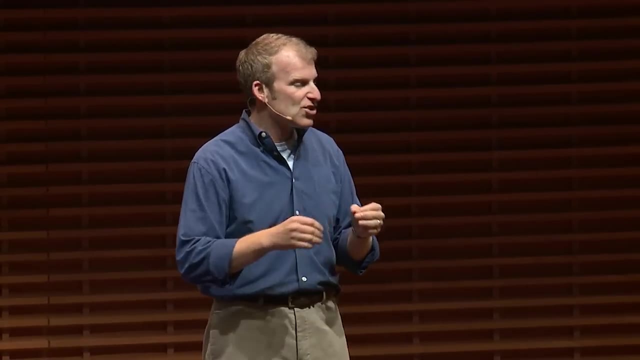 going to make a fool out of myself. Others of you are, if you're following this advice, are saying: what a great opportunity, right? So the game again is played like this: You and your partner will exchange, each will exchange a gift. One will start then the 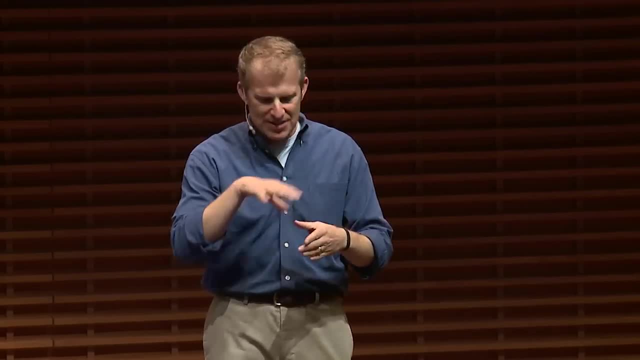 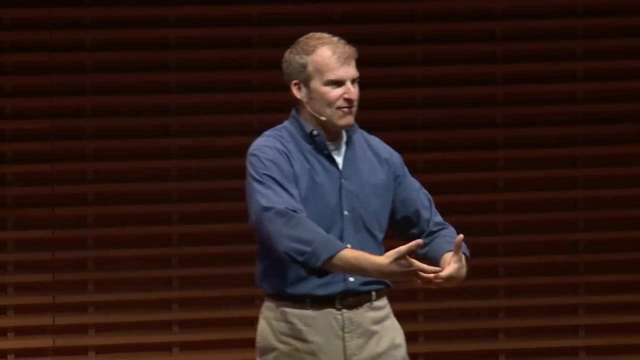 other will follow. The first person will give a gift to the second person. Second person opens the box, however big the box is- And if the box is big and you find a penny in it, perfect. Doesn't matter. If the box is heavy and you find a feather in it, fine. 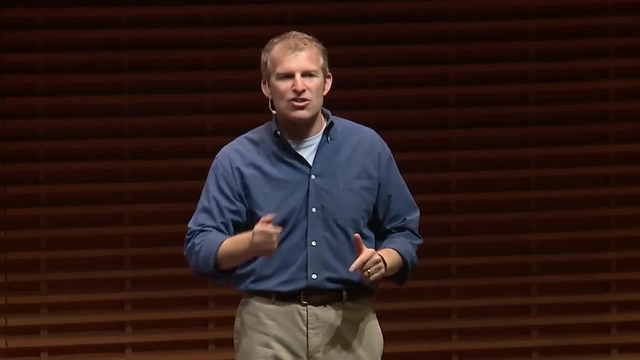 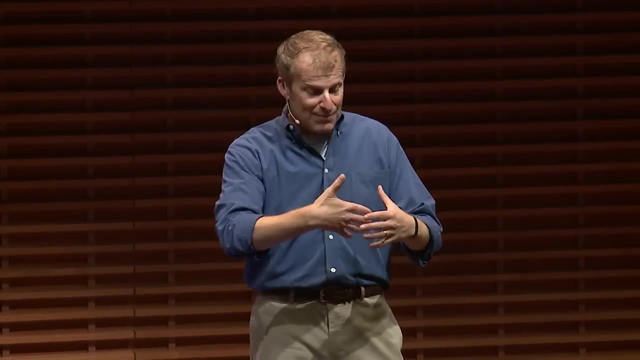 It does. there's no way to get it wrong. okay, Whatever's in the box is in the box. You're going to return it and get what you wanted later. okay, The person then you will name it. you will say thank you for the whatever you saw in. 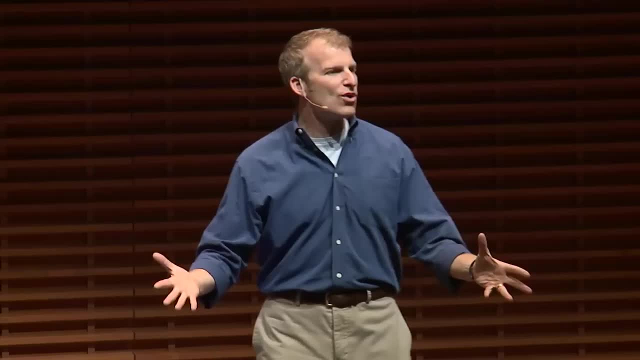 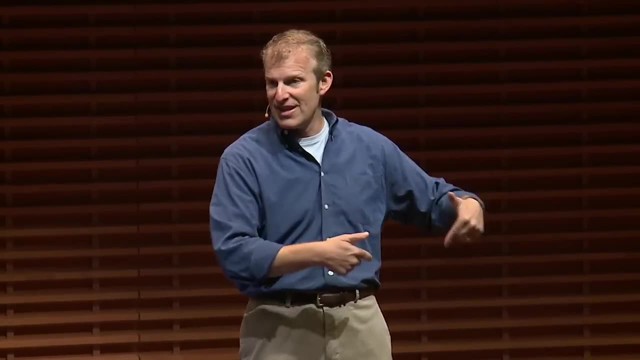 the box. The person who gave it to you will say I'm so glad, you're excited I got it for you because- And you will give a reason that you got them- whatever they decided you gave them Make sense. All right, So very quickly, just in five seconds, find a partner. 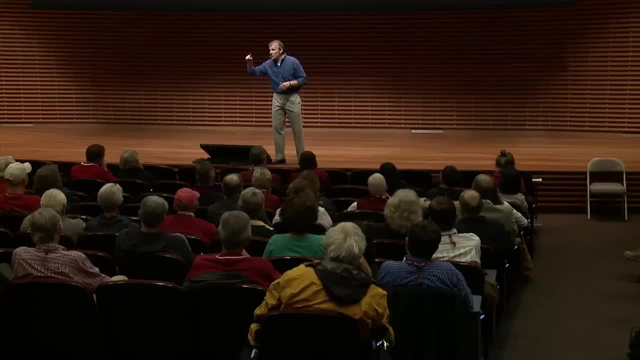 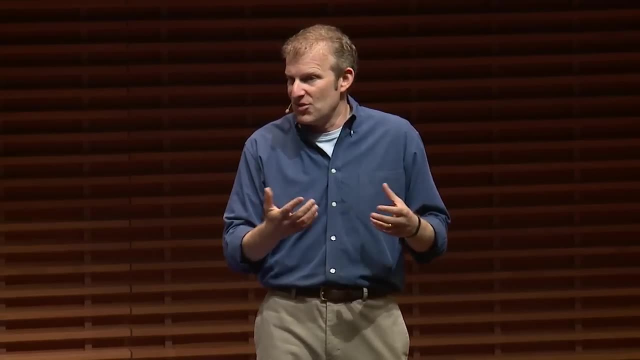 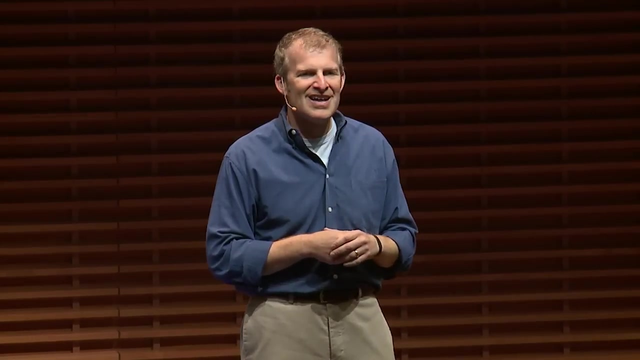 first part of the activity. now the opportunity is twofold in this game. the opportunity is for you, the gift receiver, to name a gift. that's kind of fun, that's an opportunity. it's not a threat, but the real opportunity for the gift giver, because the gift giver then has to say so. you look and you say thank you for. 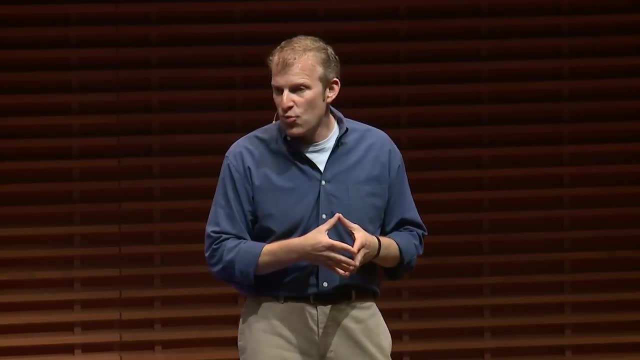 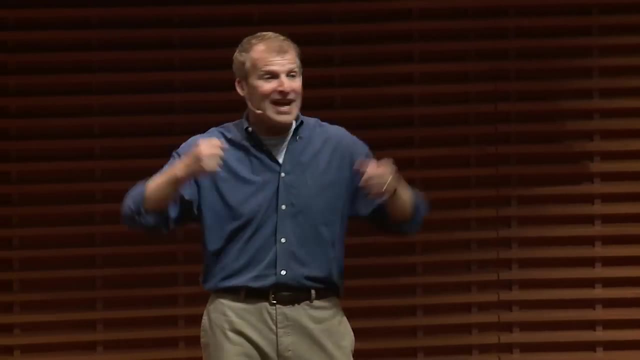 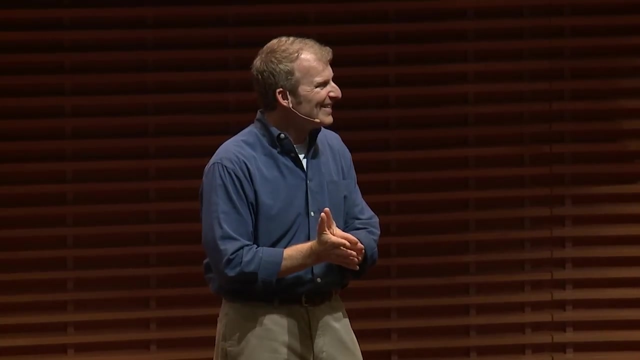 giving me a frog's leg and the person will will look at you and say I knew you wanted a frog's leg because so, whatever you find, the person who has received it is going to say, absolutely, I'm so glad, you're happy I got it for you, because so you have to respond to whatever they say, right? 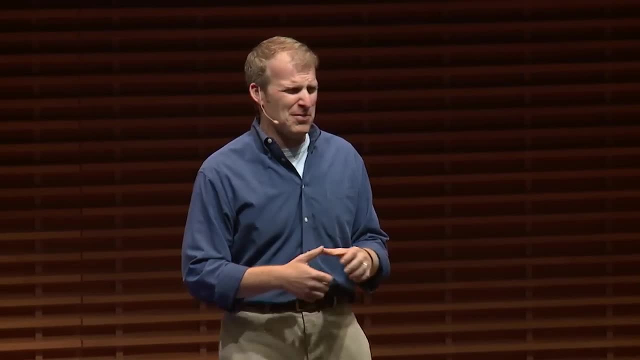 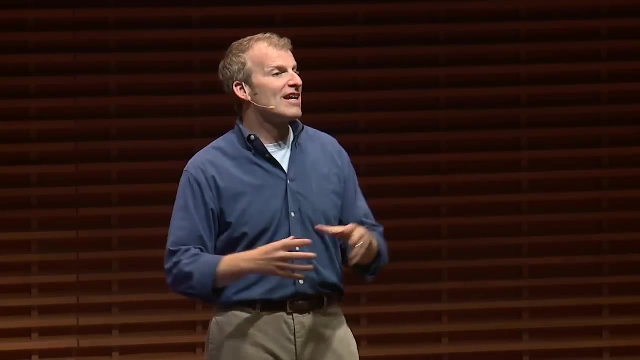 what a great opportunity. now some of you are sitting there: oh, that's hard, I don't want to do. I'm gonna make a fool of myself. others of you are, if you're following this advice, are saying: what a great opportunity, right? so the game again is played like this: you and your partner will exchange, each will exchange a gift. one will start. 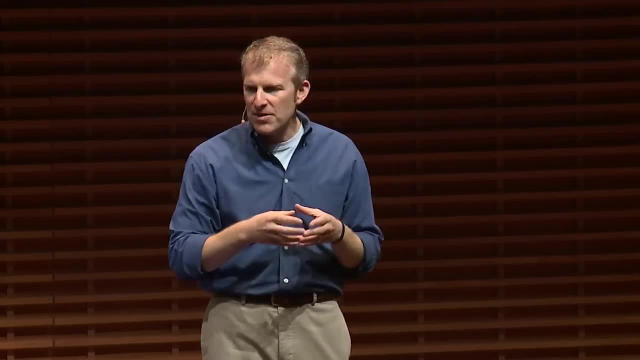 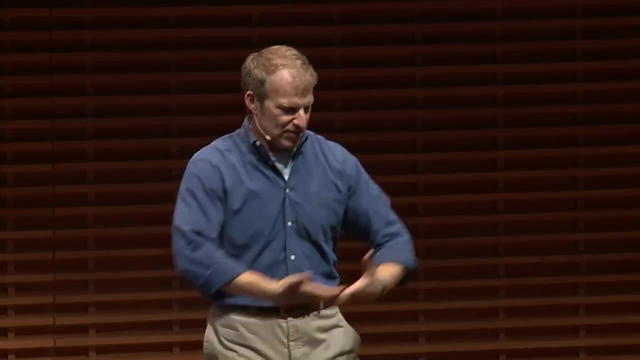 then the other will follow. the first person will give a gift to the second person. second person opens the box, however big the box is- and if the box is big and you find a penny in it, perfect, doesn't matter. the box is heavy and you find a feather in it, fine it does. there's no way to get. 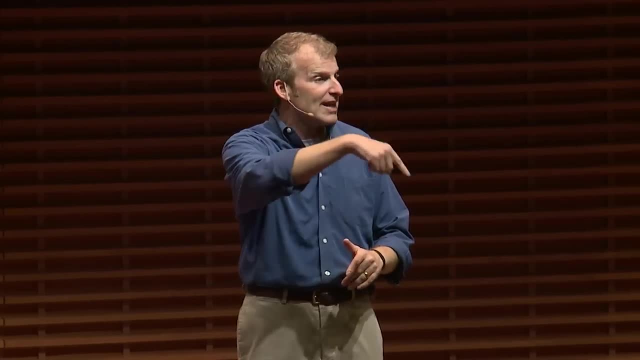 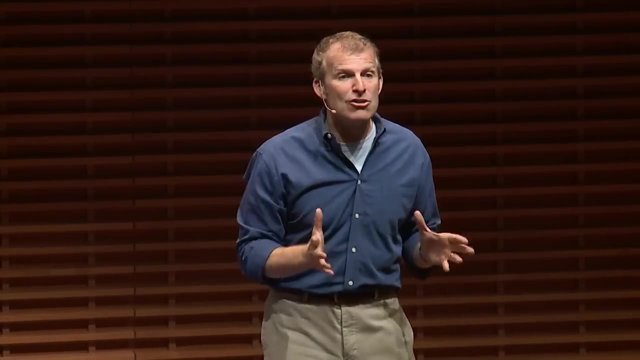 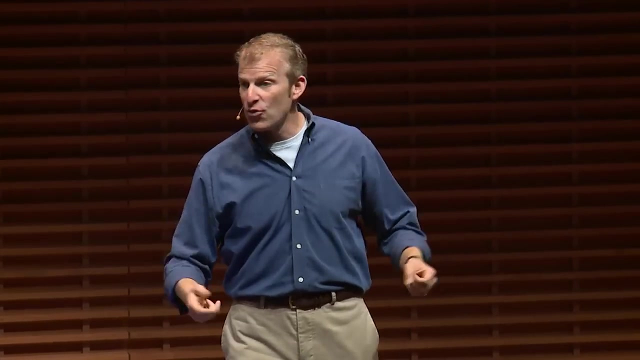 it wrong. okay, whatever's in the box is in the box. you can return it and get what you wanted later. okay, the person then you will name it. you'll say thank you for the whatever you saw in the box. the person who gave it to you will say: I'm so glad, you're excited, I got it for you because. 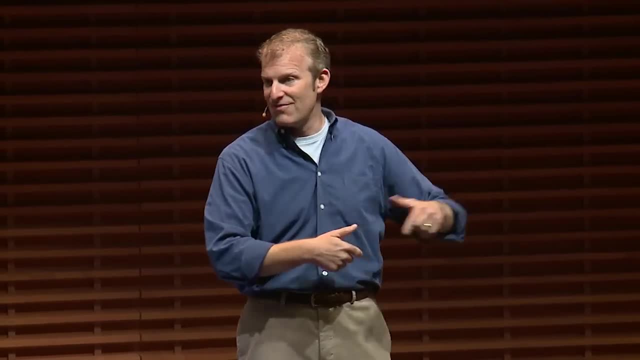 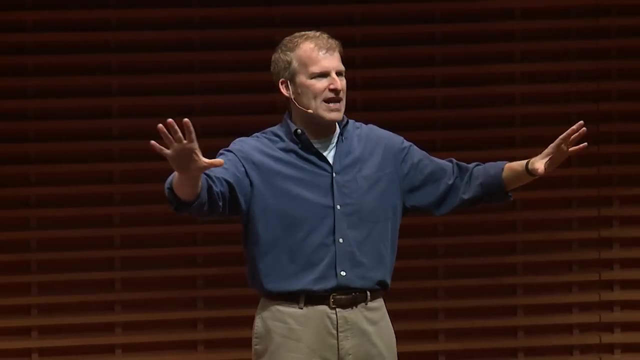 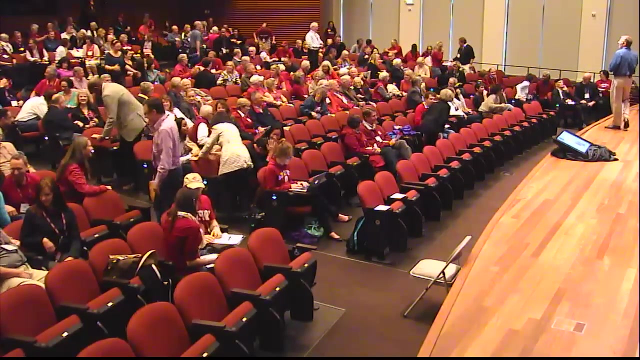 and you will give a reason that you got them. whatever they decided you gave them make sense. all right, so very quickly, just in five seconds, find a partner. if you're willing to do this with a partner, everybody have a partner, okay, all right. in your partnerships, in your partnerships, pick an, a person. 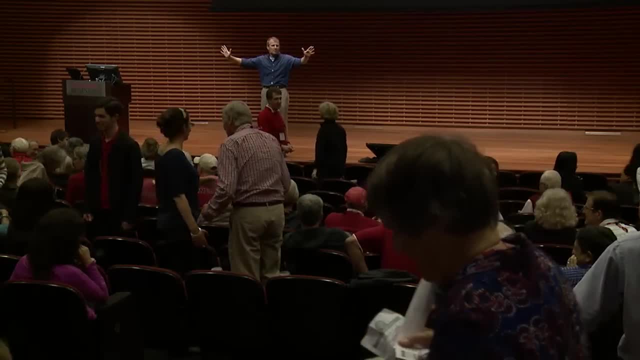 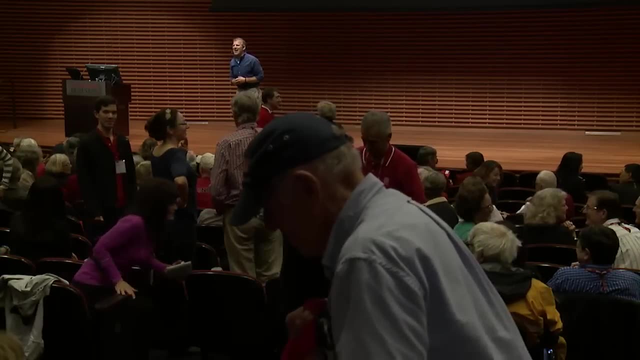 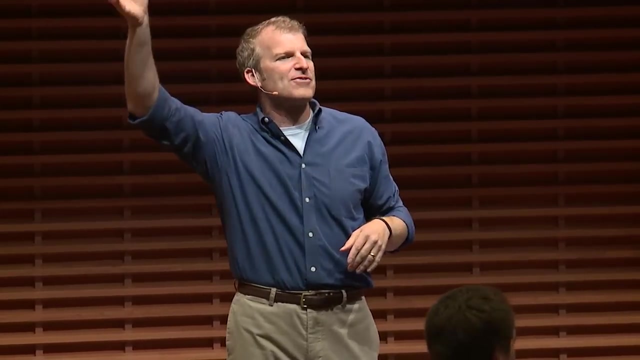 and a bee person. you may stand or sit, it's totally up to you. pick an a and pick a B. okay, B goes first. alright. B give A a gift. B give a a gift. A thank them, and then B will name and give reason they gave it to him. 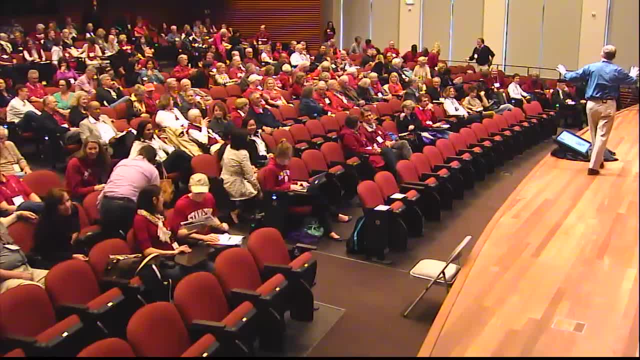 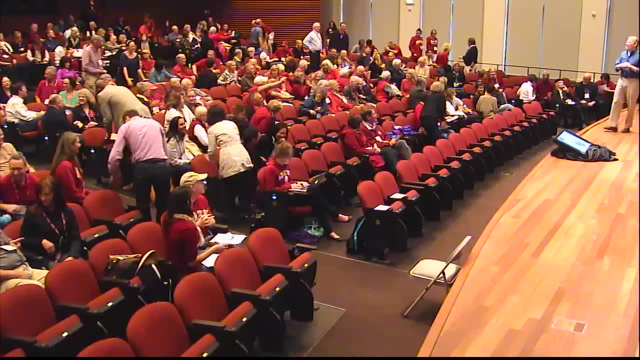 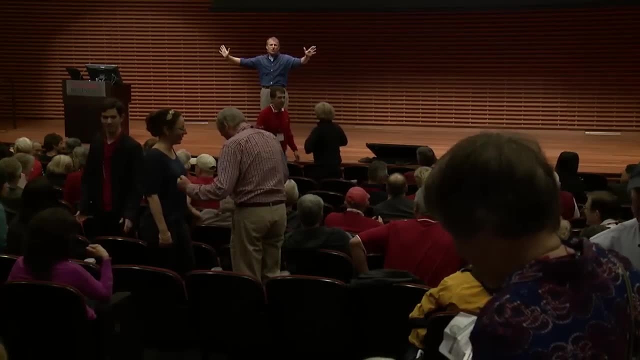 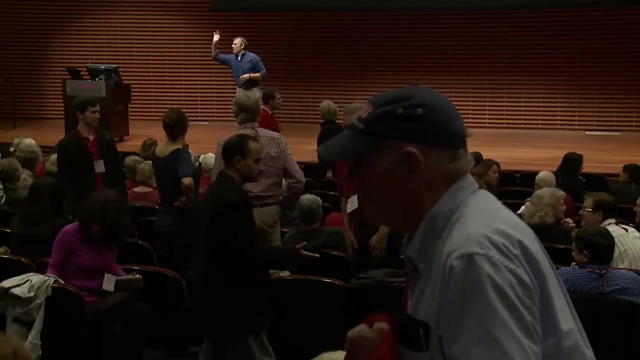 if you're willing to do this with a partner. Everybody have a partner. Okay, All right. In your partnerships. in your partnerships, pick an A person and a B person. You may stand or sit, It's totally up to you. Pick an A and pick a B. Okay, B goes first. 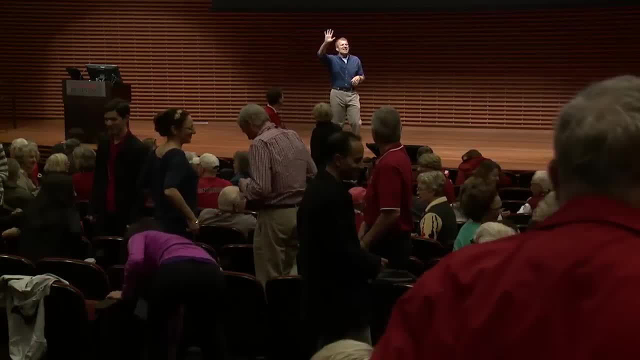 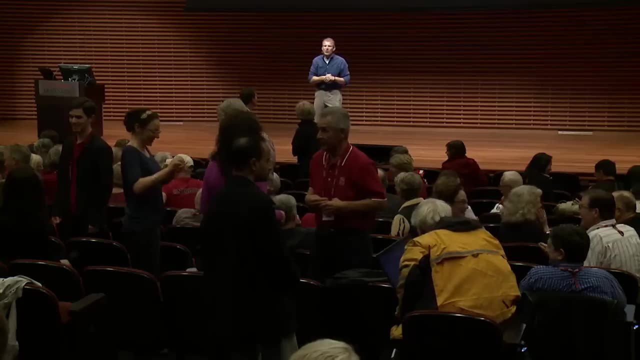 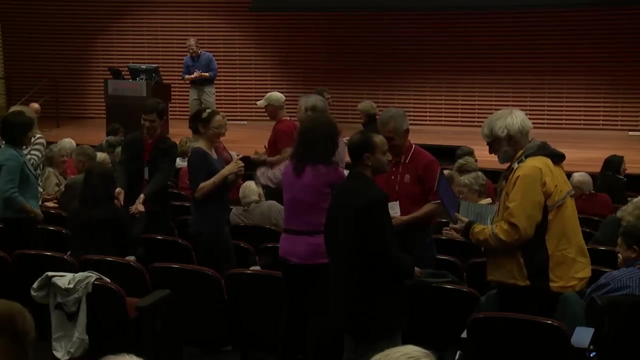 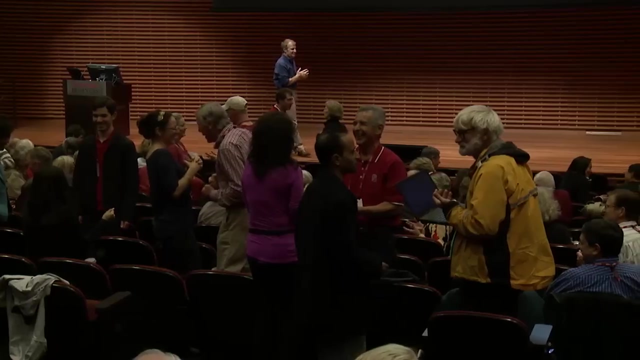 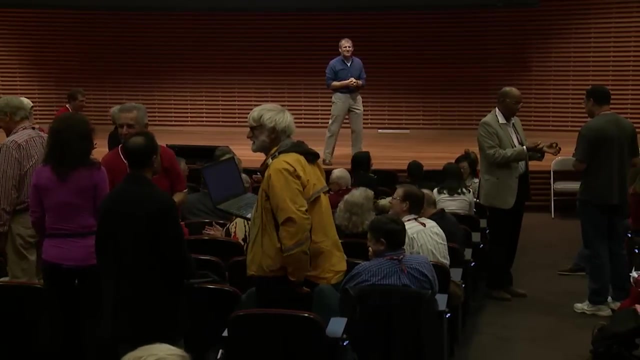 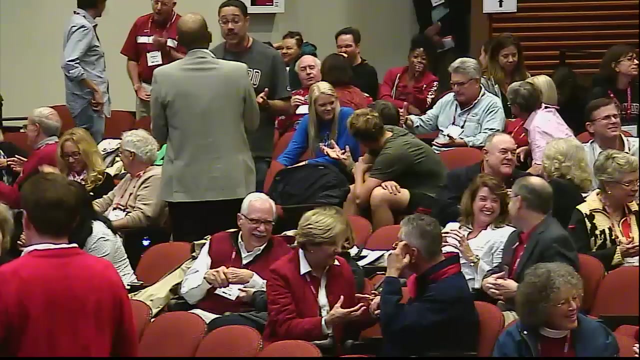 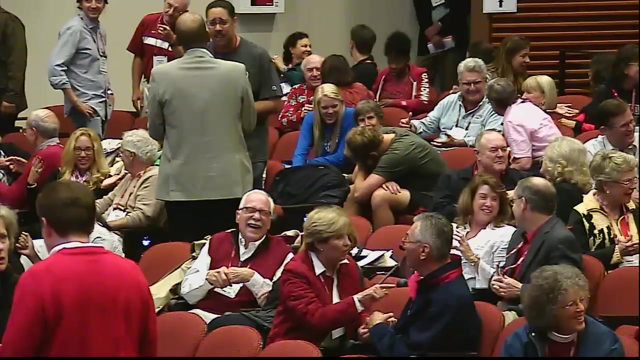 Ha, ha ha, All right. B give A a gift. B give A a gift, A thank them. B give A a gift, A thank them. And then B will name and give the reason they gave it to them. If you have not switched switch please. If you have not switched, switch please. 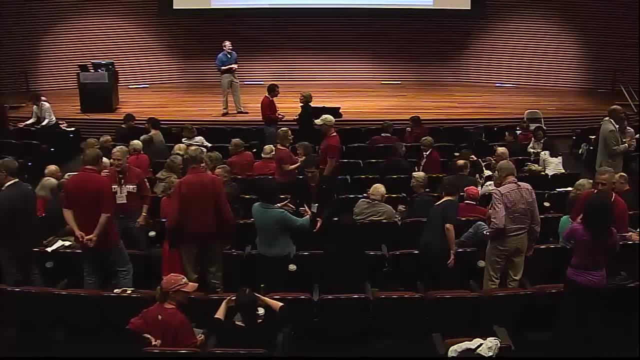 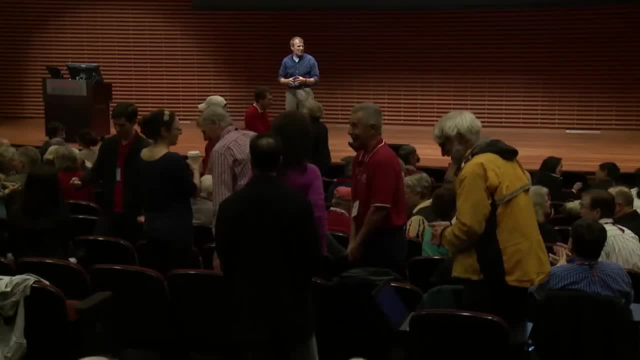 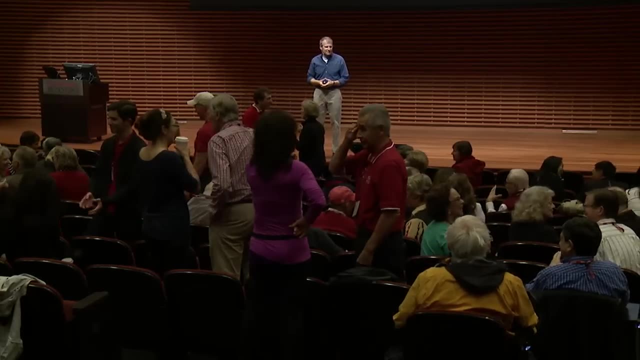 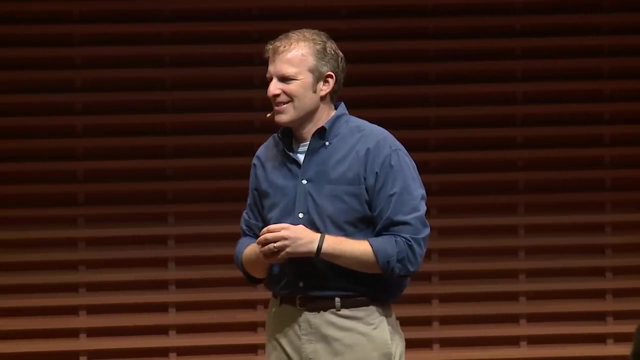 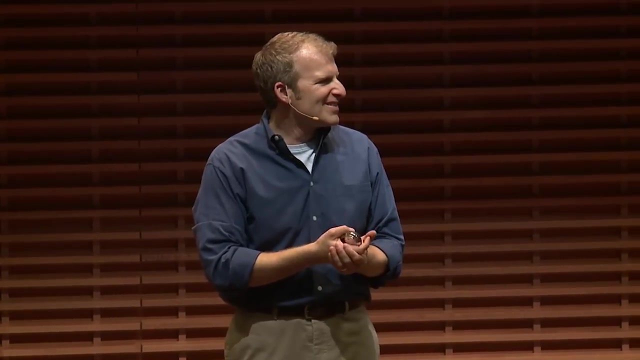 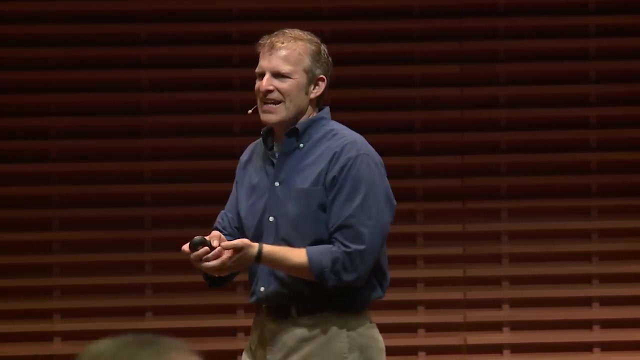 Okay, Okay, Let's wrap it up in 30 seconds, please. Let's wrap it up. All right, If we can all have our seats, If we can all take our seats, please. I know I'm telling a room of many MBA alums to stop talking. 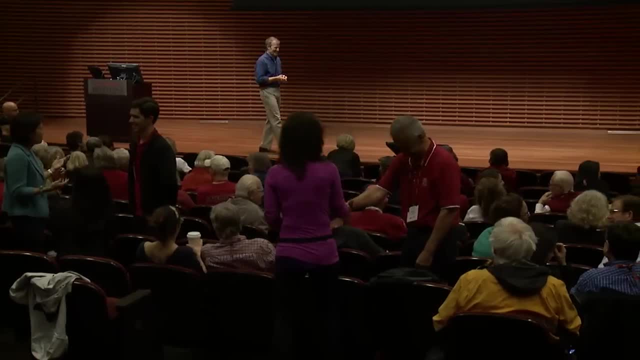 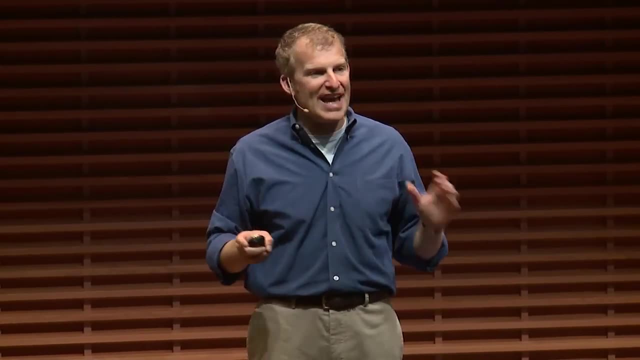 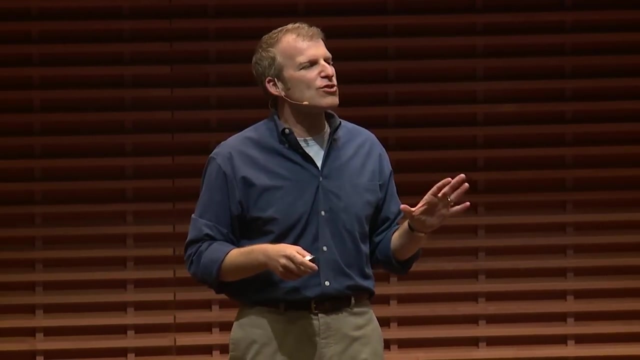 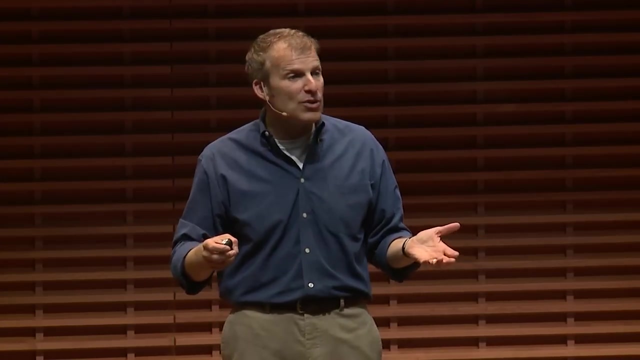 and that's hard. all right, ladies and gentlemen, did you get what you wanted? pretty neat, huh, you always get what you want. now, for some of you, this was really hard because you were really taking the challenge and not seeing what was in the box until you looked in there. okay, was anybody surprised by what you found in? 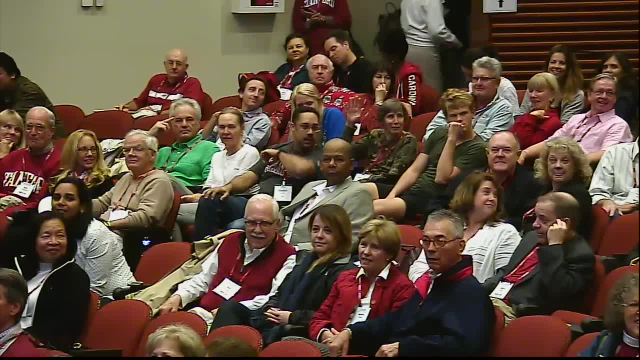 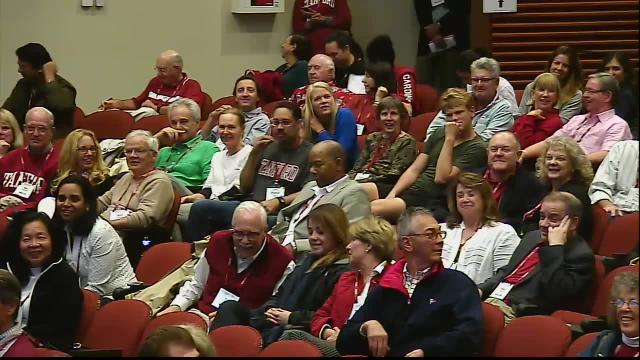 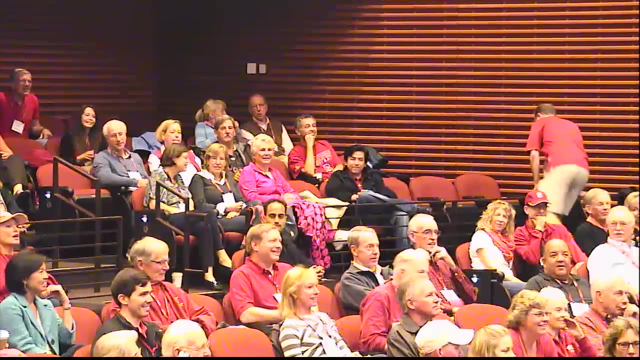 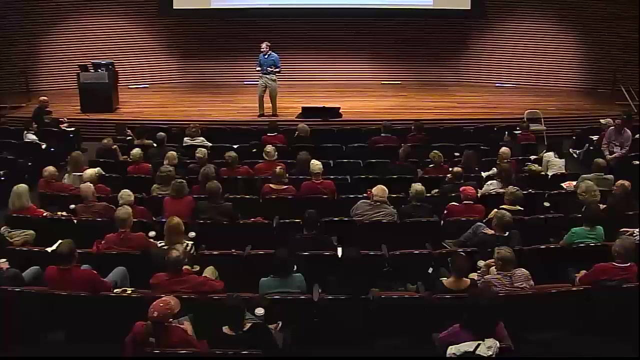 the box. what did you find, sir? what was in the box? what? wow, nice, nice, if you've got a Ferrari, you need a transmission. I like it. who else found something that was surprising? what did you find? a live unicorn. that's a great gift, right, okay, how was it? as the gift giver, were you surprised at what your partner found in? 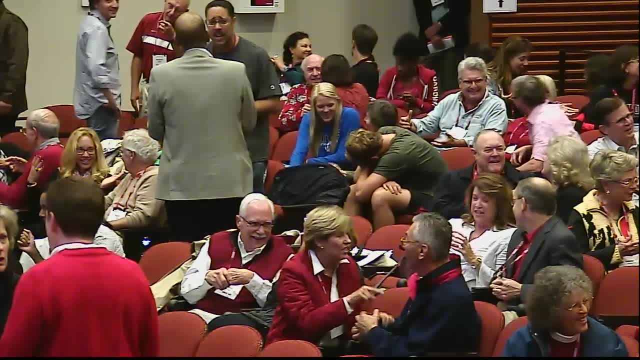 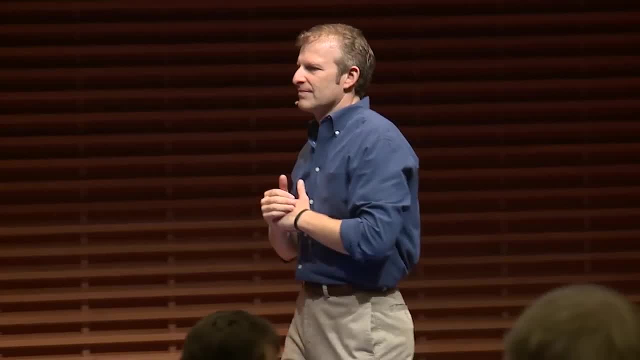 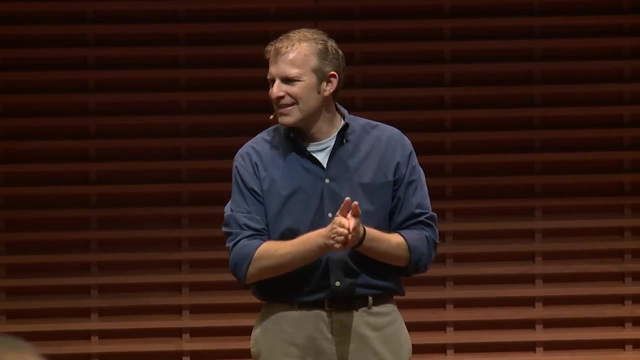 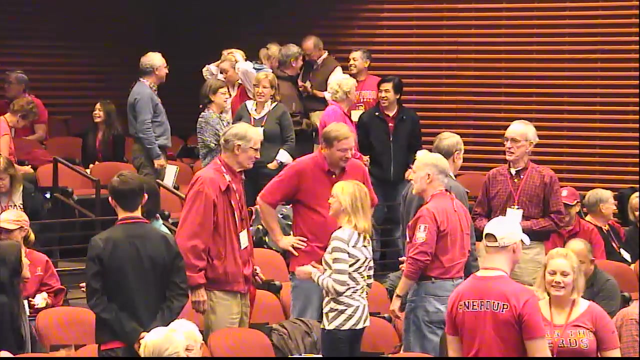 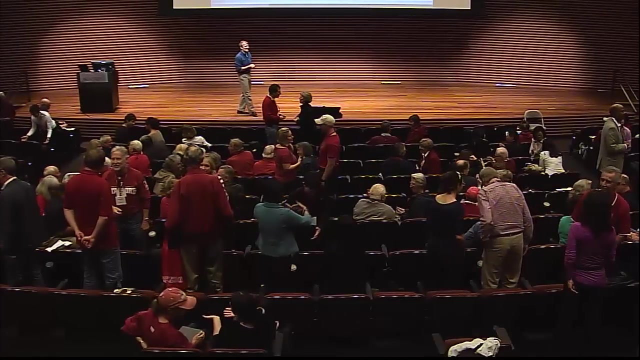 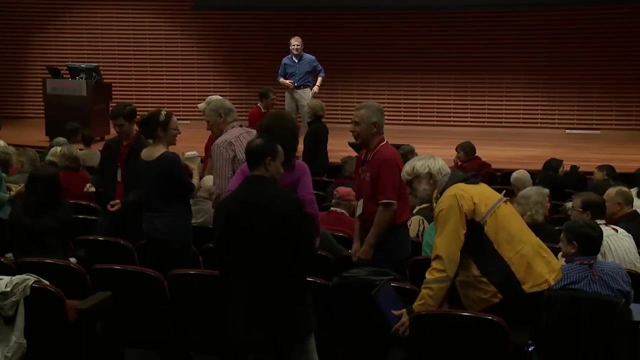 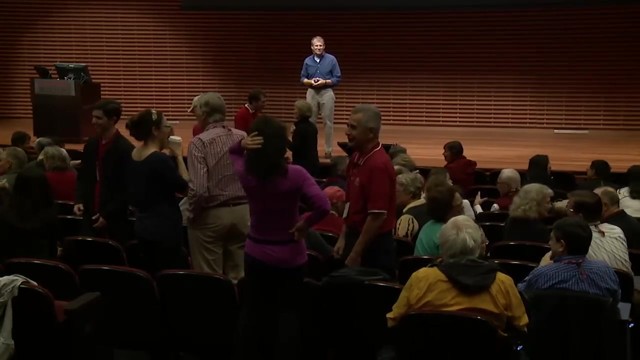 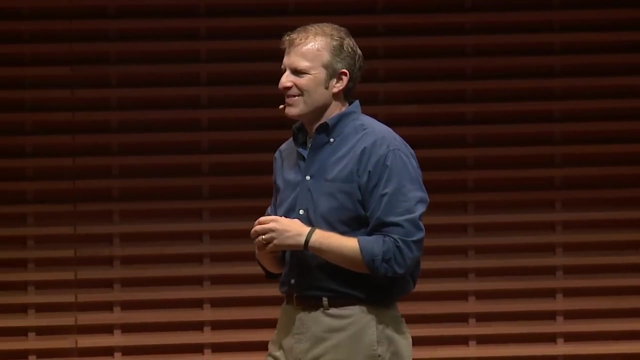 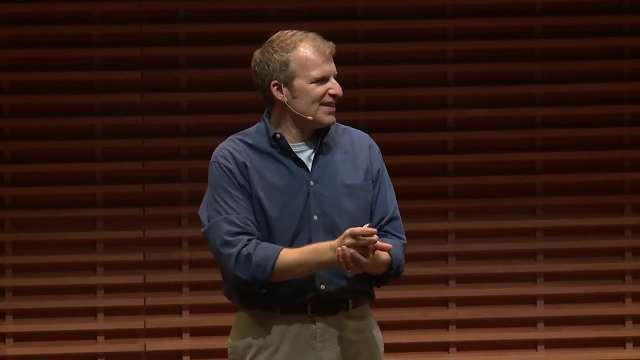 If you have not switched switch, please. If you have not switched switch, please, Let's wrap it up in 30 seconds. please, Let's wrap it up. All right, if we can all have our seats, If we can all take our seats, please. 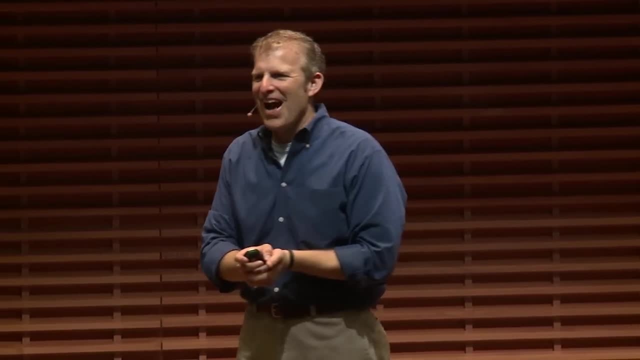 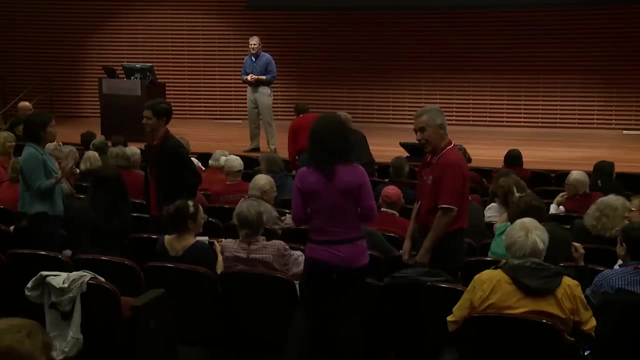 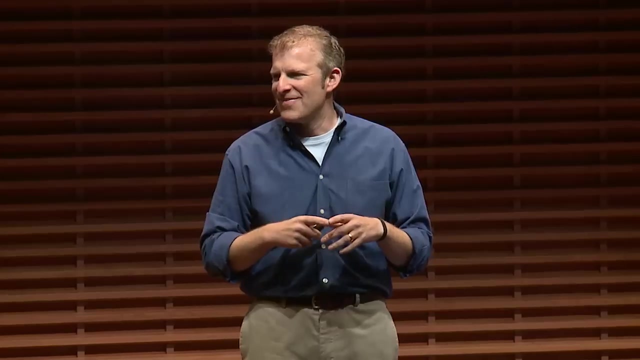 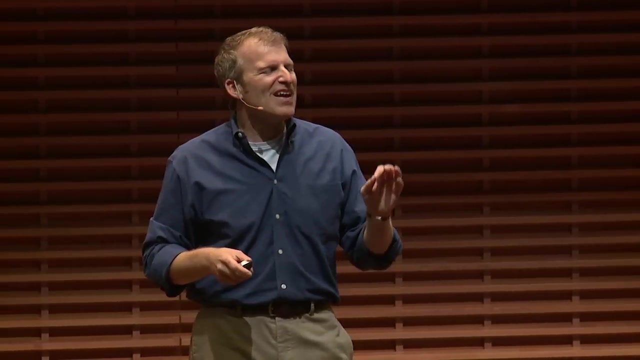 I know I'm telling a room of many MBA alums to stop talking, and that's hard, All right. ladies and gentlemen, did you get what you wanted? Pretty neat, huh, You always get what you want. Now, for some of you, this was really hard because you were 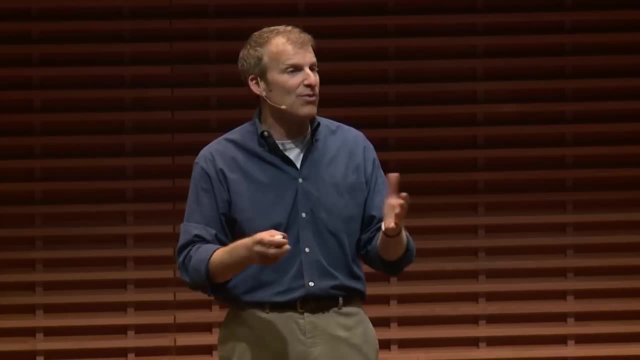 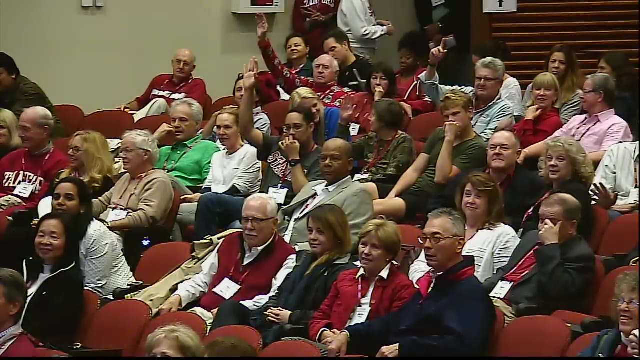 really taking the challenge and not sticking to it. You were not seeing what was in the box until you looked in there. Okay, Was anybody surprised by what you found in the box? What did you find, sir? What was in the box? 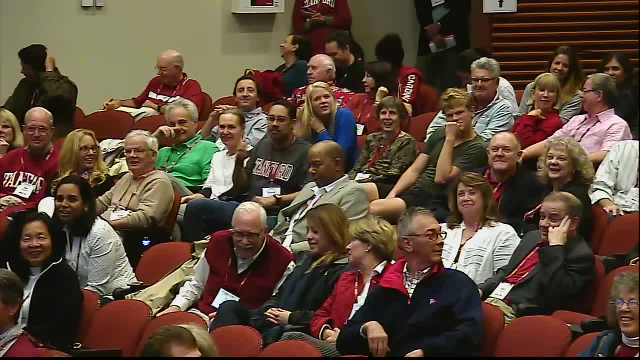 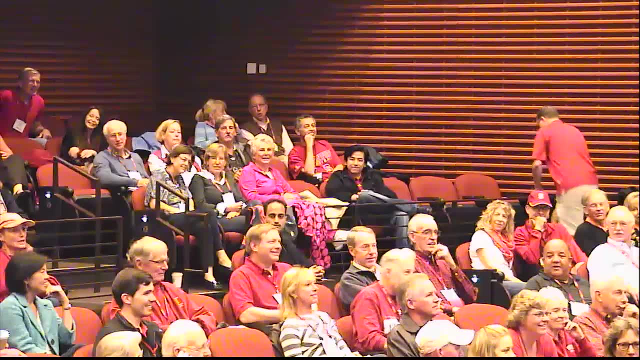 Wow, Nice, Nice. If you've got a Ferrari, you need a transmission. I like it. Who else found something that was surprising? What did you find? A live unicorn. That's a great gift, right? How was it as the gift giver? 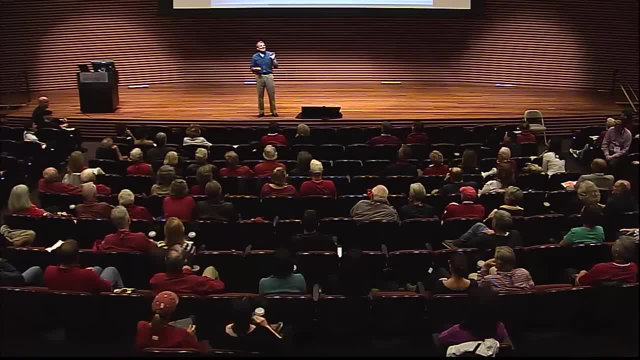 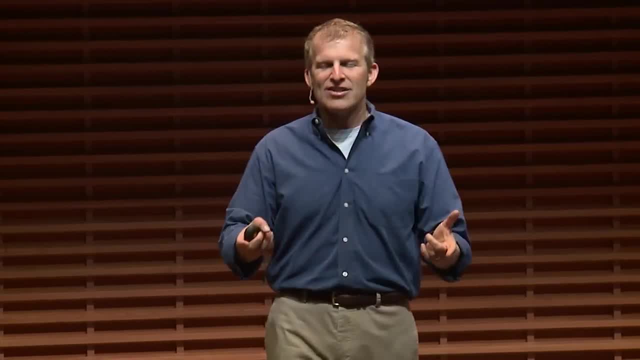 Were you surprised at what your partner found in the box? Isn't it interesting that when we give an imaginary gift, knowing that the person is going to name it, we already have in mind what they're going to find, And when they say live unicorn, we go. well, that's interesting, right. 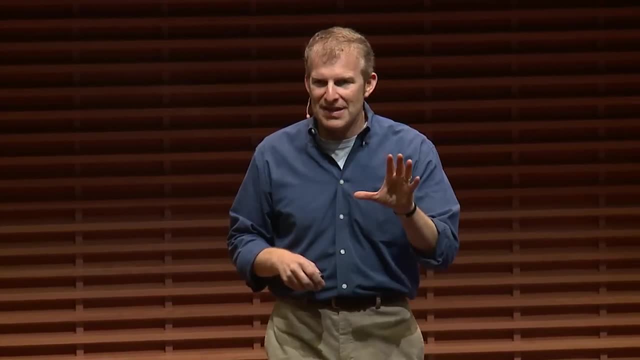 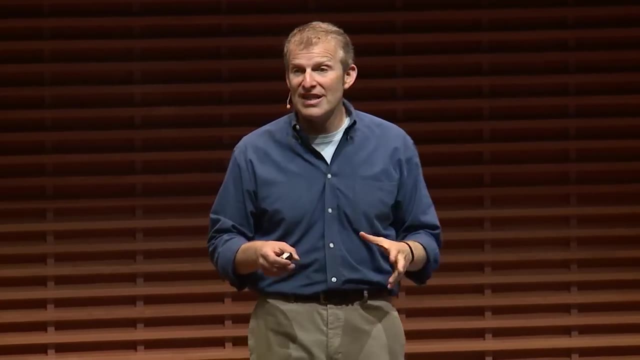 So the point of this game is to one remind ourselves we have to get out of our own way, like we talked about before, but to see this as an opportunity and to have fun. I love watching people play this game. The number of smiles that I saw amongst you. 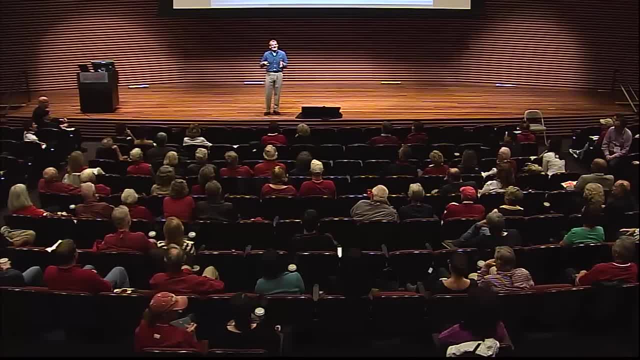 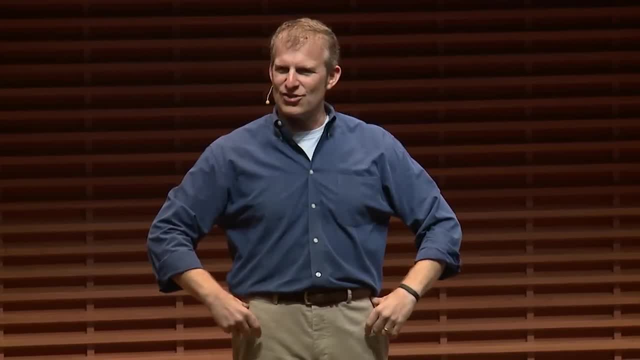 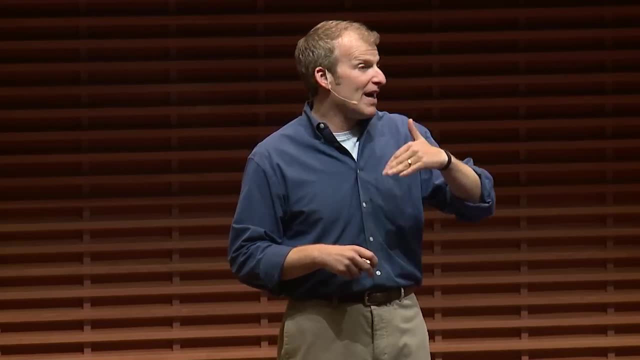 the box. isn't it interesting that when we give an imaginary gift, knowing that the person's going to name it, we already have in mind what they're going to find, and when they say live unicorn, we go. well, that's interesting, right? so the point of this game is to one remind ourselves: we have to get out of our own. 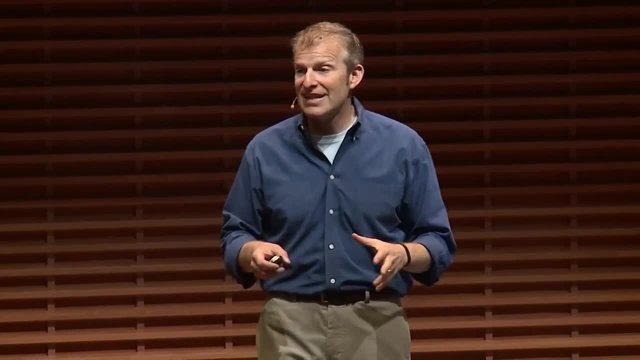 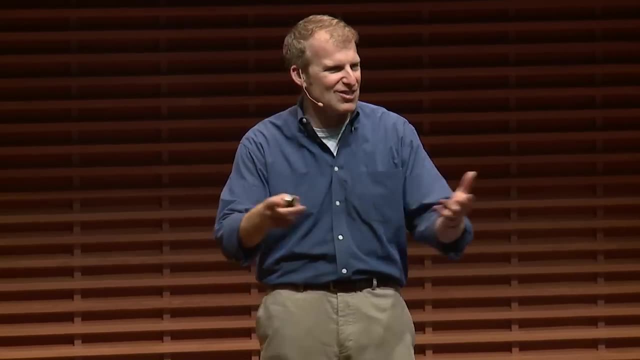 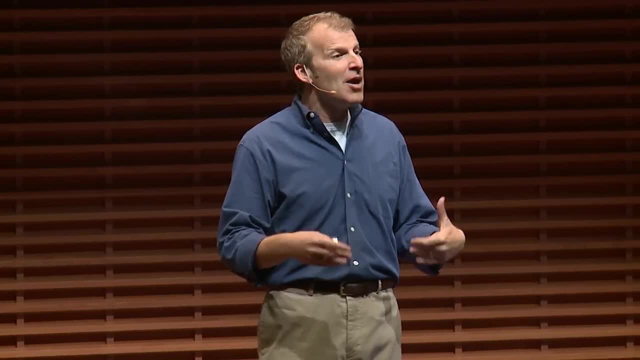 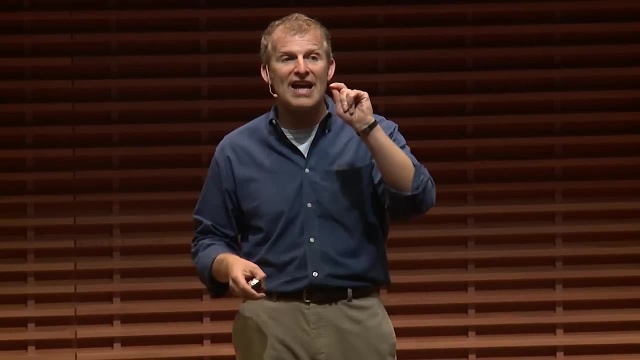 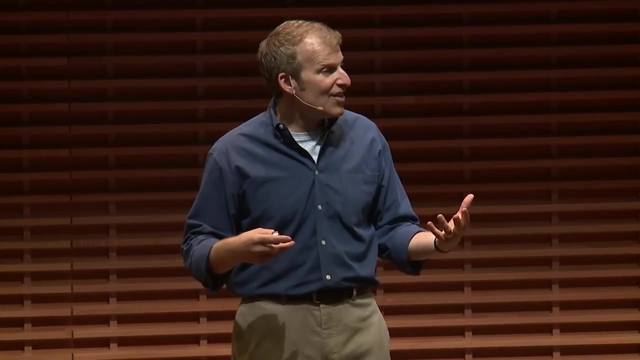 I first started, some of you looked a little dour, a little doubting, okay, but in that last game you were all smiling and looked like you were having fun. so when you reframe the spontaneous speaking opportunity as as an opportunity, as something that you can co-create and share, all the sudden you 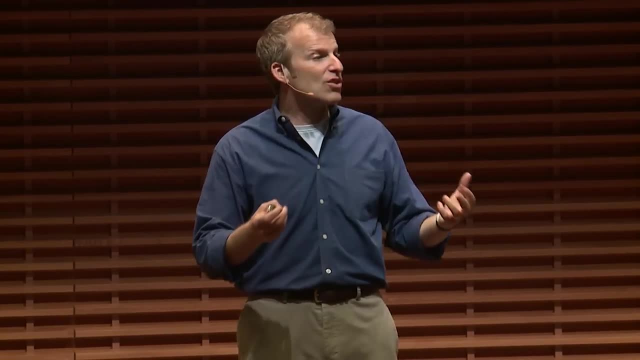 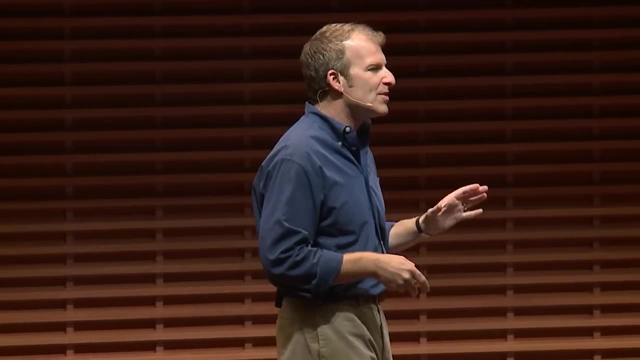 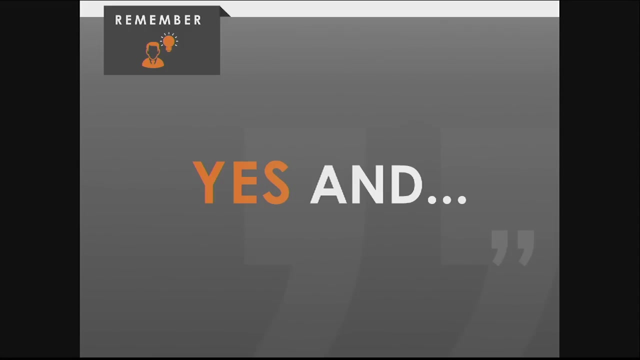 are less nervous, less defensive, and you can accomplish something pretty darn good, in this case, a fun game. This reminds us of perhaps the most famous of all: improvisation sayings yes, and a lot of us live our communication lives saying no but yes- and opens up a 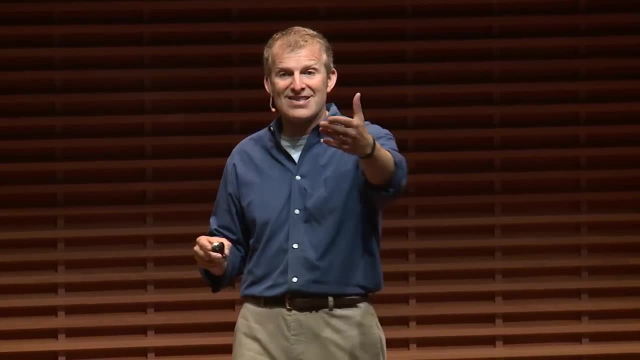 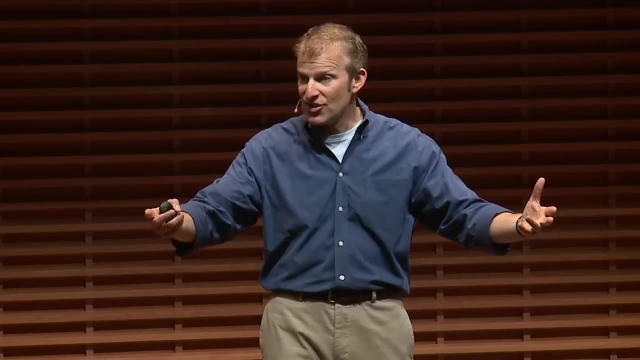 tremendous amount of opportunities, and this doesn't mean you have to say yes and to a question somebody asked. this just means the approach you take to the situation. so you're going to ask me questions. that's an opportunity. yes, and I will follow through Versus. 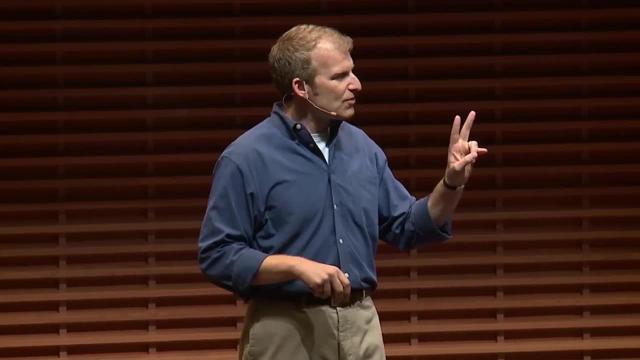 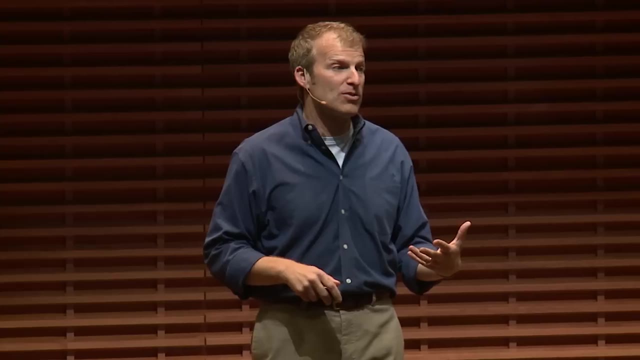 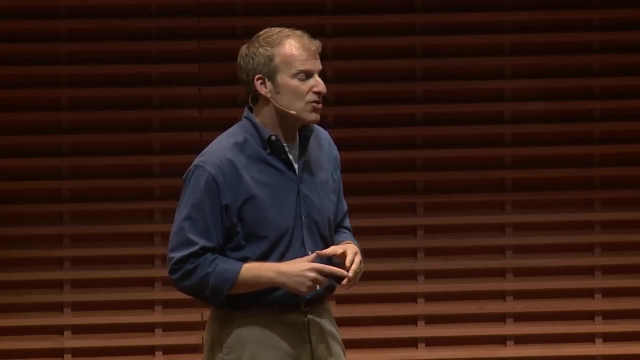 no and being defensive. so we've accomplished the first two steps of our process. first, we get out of our own way and second we reframe the situation as an opportunity. the next phase is also hard but very rewarding, and that is to slow down and listen. you need to understand the demands of the requirement you find. 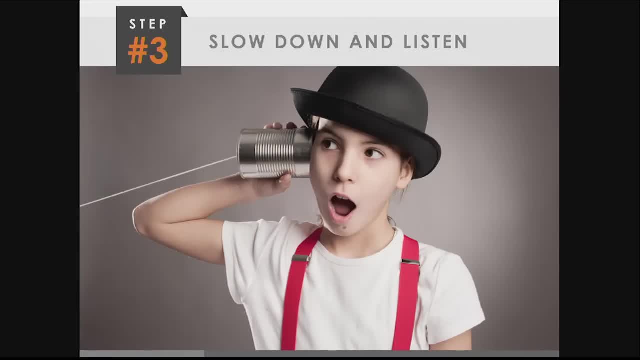 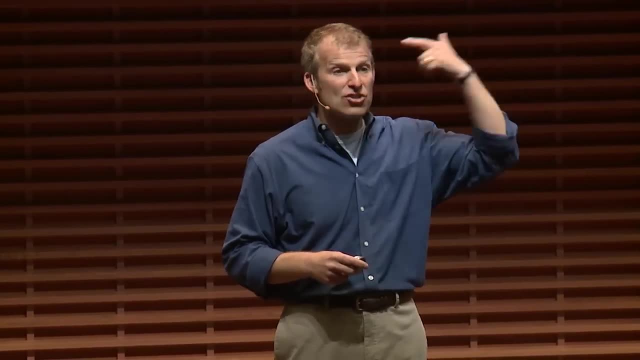 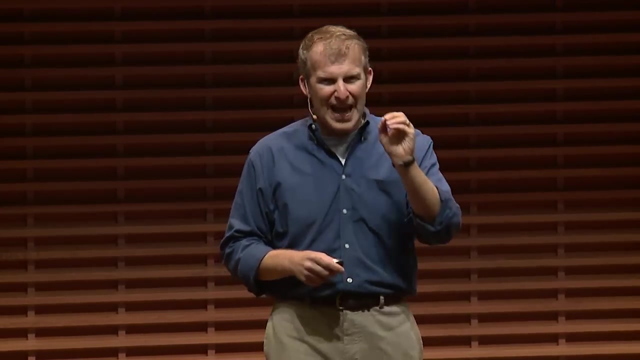 yourself in in order to respond appropriately. but often we jump ahead, we listen just enough to think we got it, and then we go ahead starting to think about what we're going to respond, and then we respond. we really need to listen because fundamentally, as a communicator, your job is to be in. 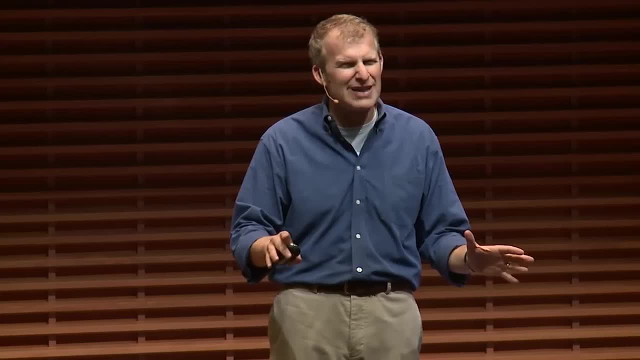 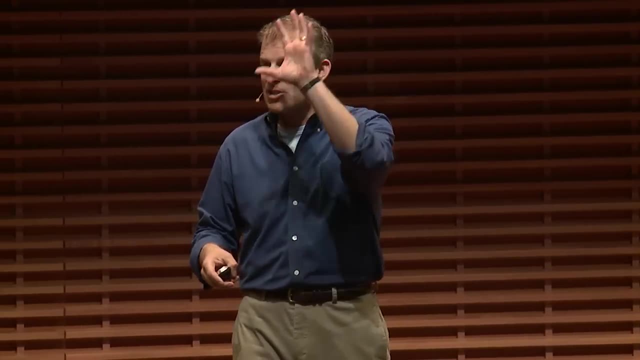 and I have to admit, when I first started some of you looked a little dour, a little doubting, okay, But in that last game you were all smiling and looked like you were having fun. So when you reframe the spontaneous speaking opportunity as an opportunity, 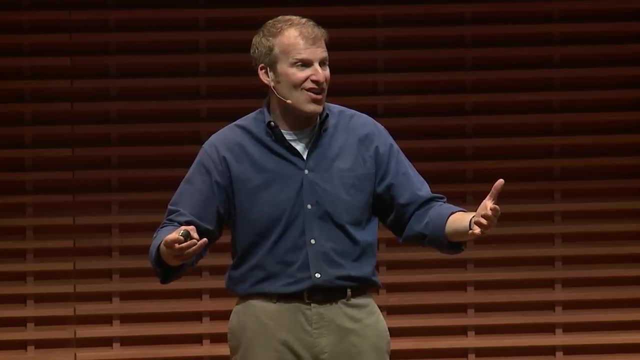 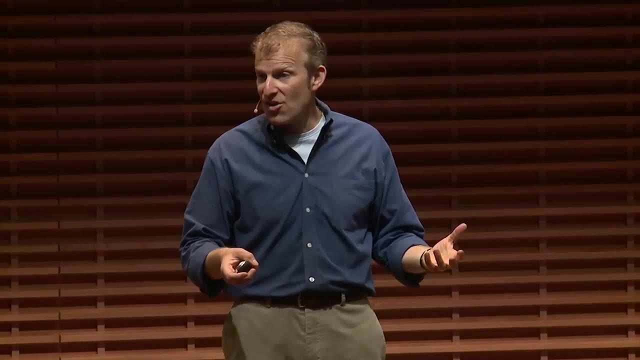 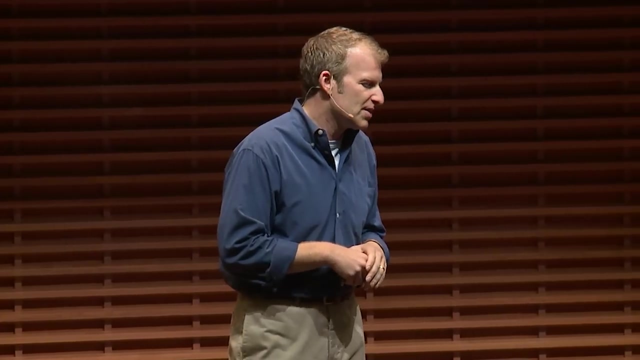 as something that you can co-create and share. all of a sudden, you are less nervous, less defensive and you can accomplish something pretty darn good- in this case, a fun outcome. This reminds us of perhaps the most famous of all improvisation sayings. 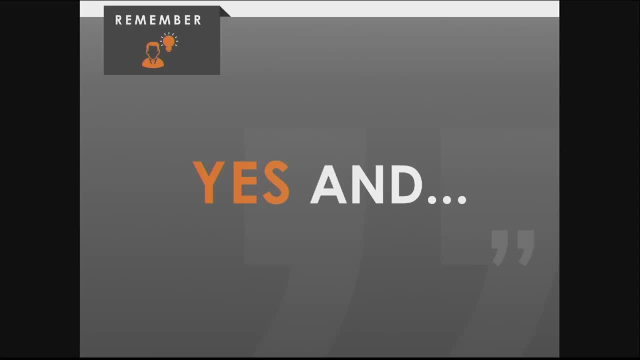 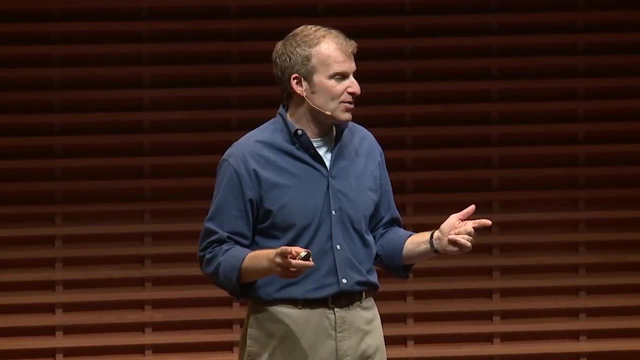 yes and A lot of us live our communication lives saying no but Yes and opens up a tremendous amount of opportunities. And this doesn't mean you have to say yes and to a question somebody asks. This just means the approach you take to the situation. 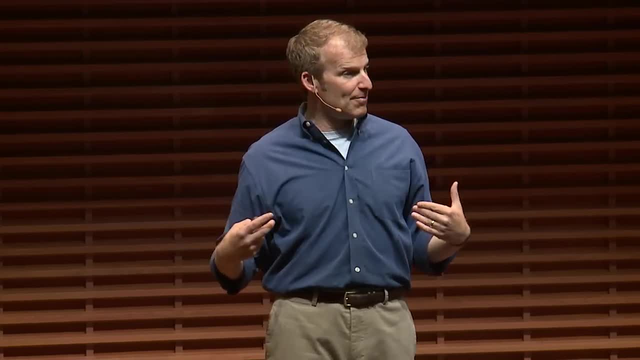 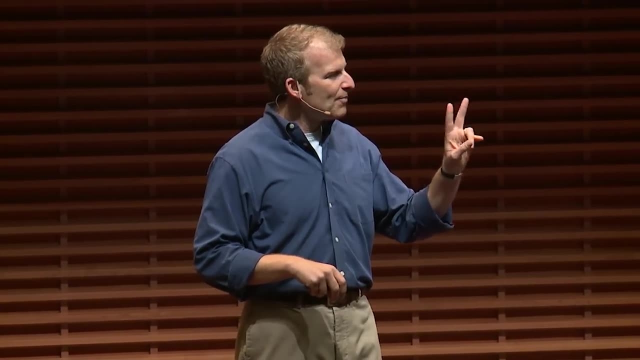 So you're going to ask me questions. That's an opportunity, Yes, and I will follow through Versus no, and being nervous Versus being defensive. So we've accomplished the first two steps of our process. First, we get out of our own way. 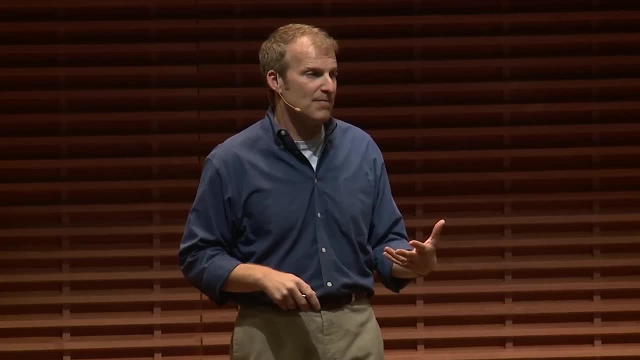 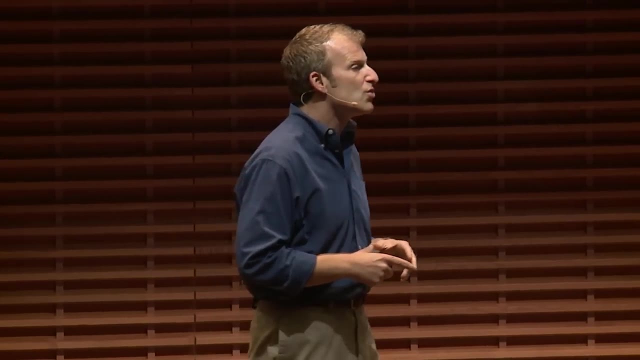 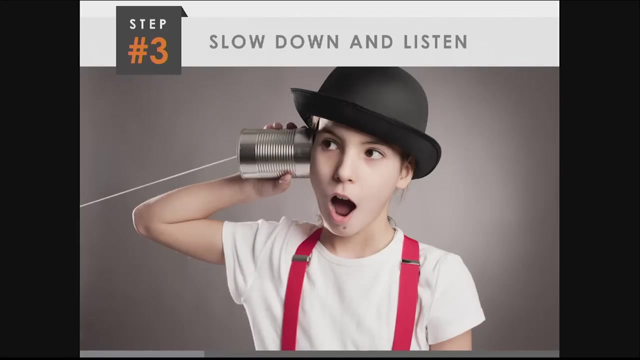 In Sepkin, we reframe the situation as an opportunity. The next phase is also hard but very rewarding, And that is to slow down and listen. You need to understand the demands of the requirement you find yourself in in order to respond appropriately. 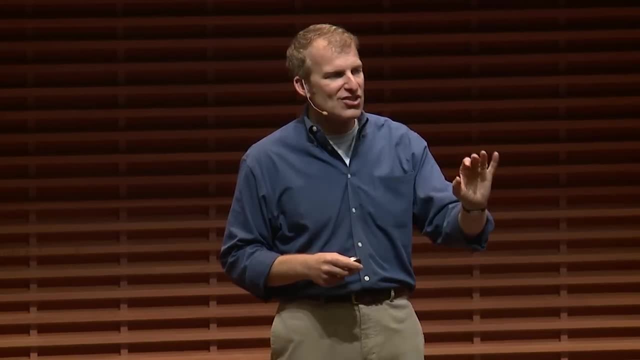 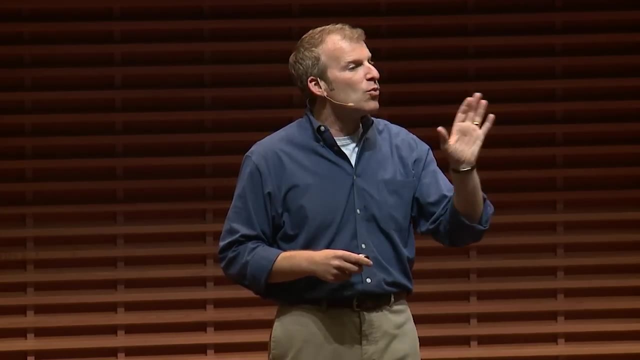 But often we jump ahead, We listen just enough to think we got it, And then we go ahead starting to think about what we're going to respond, And then we respond. We really need to listen Because fundamentally, as a communicator, your job is to be in service of your audience. 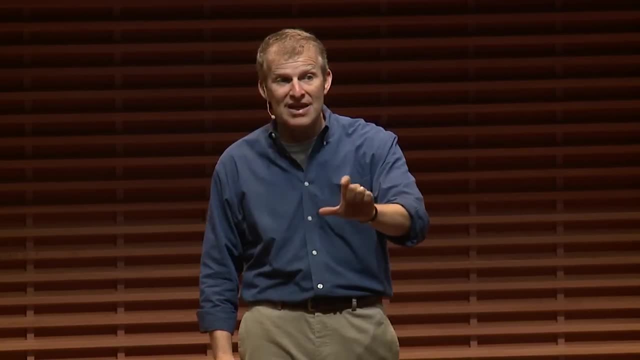 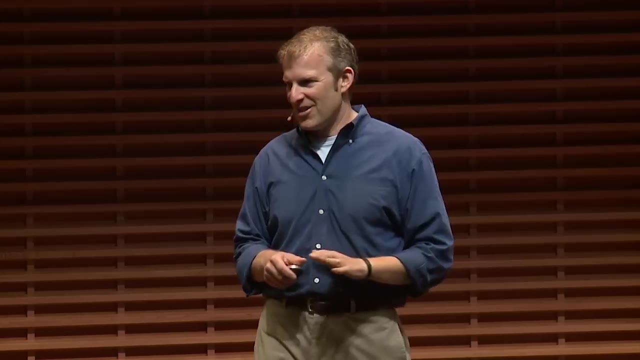 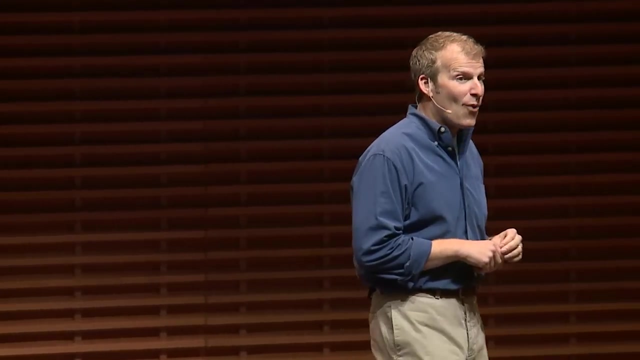 And if you don't understand what your audience is asking or needs, you can't fulfill that obligation. So we need to slow down and listen. I have a fun game to play. In this game, you are going to SPLL S-P-L-L-E-V-E-R-Y-T-H-I-N-G-Y-O-U-S-A-Y. 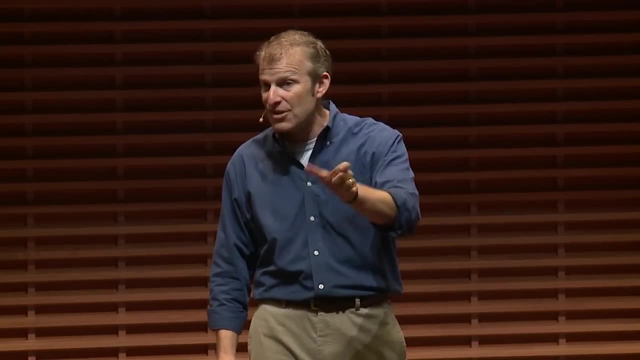 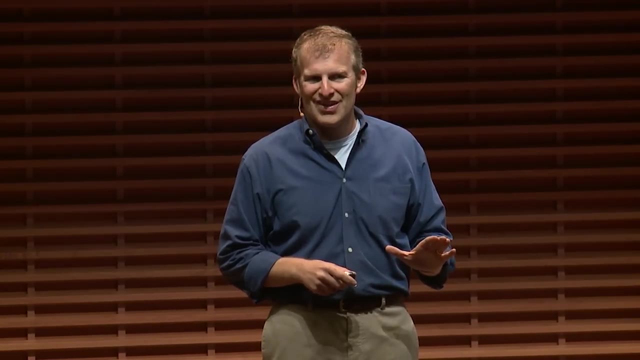 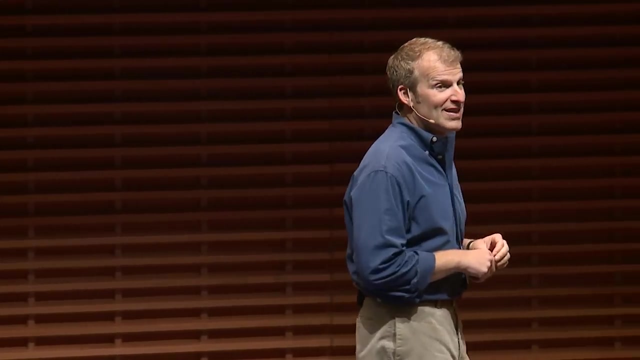 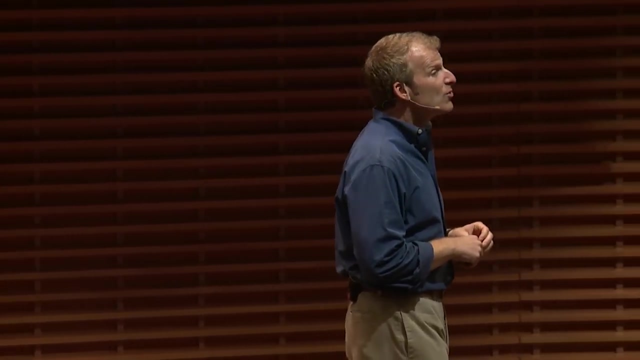 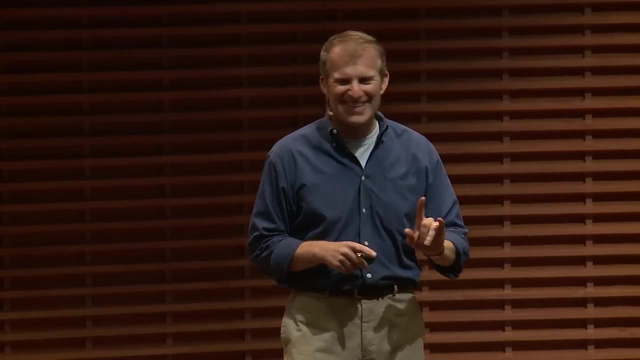 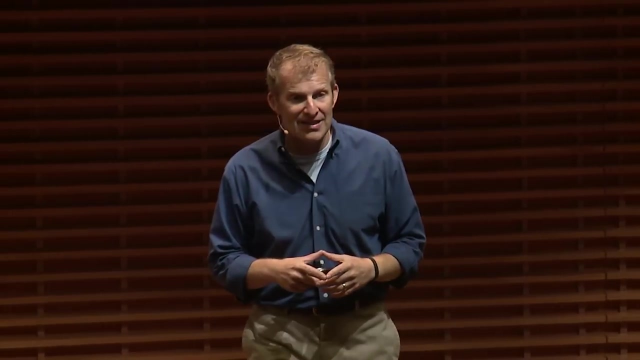 service of your audience, and if you don't understand what your audience is asking or needs, you can't fulfill that obligation. so we need to slow down and listen. I have a fun game to play. in this game, you are going to SP and the you're going to tell your. 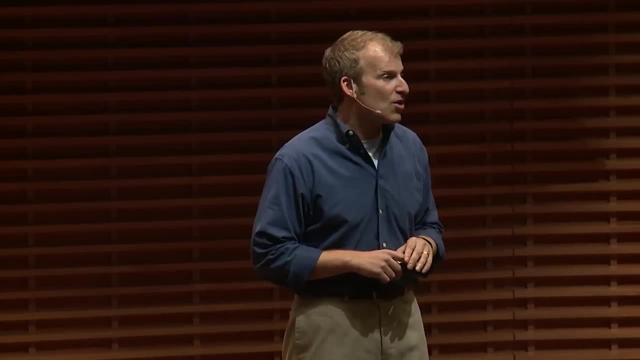 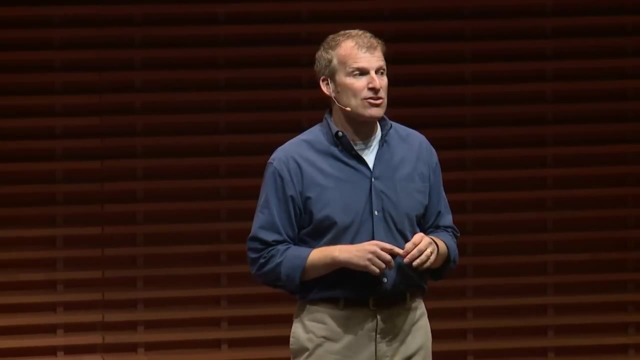 partner, what you are going to do, that will be fun today, but you are going to do so by S-P-E-L-L-I-N-G-I-T. Okay, So you're going to spell it. It's okay if you are not a good speller. 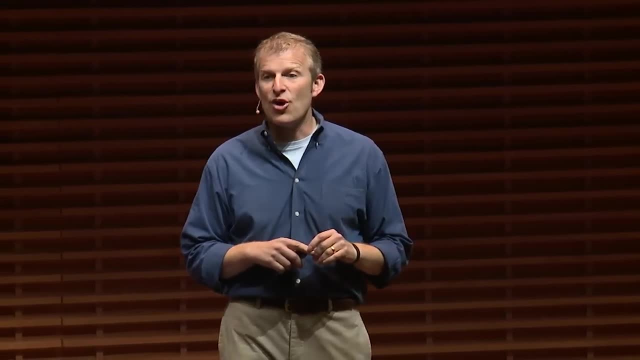 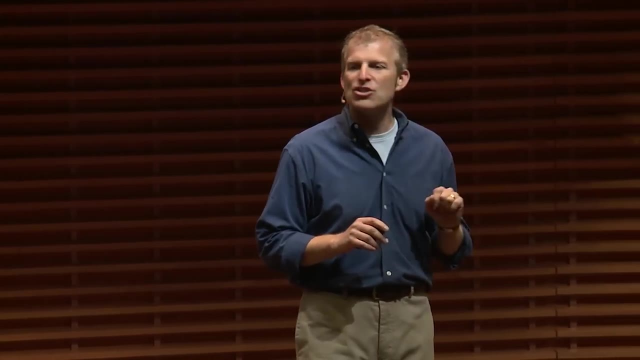 Okay, You'll see the benefit of doing this. So, with the partner you just worked with, person A is going to go first. this time, You are simply going to tell your partner. actually, you're going to spell to your partner what it is of fun, something of fun. 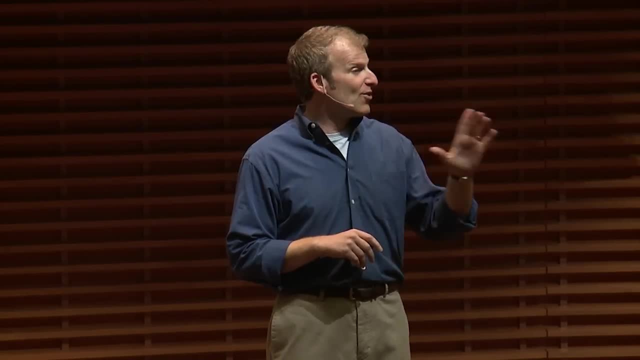 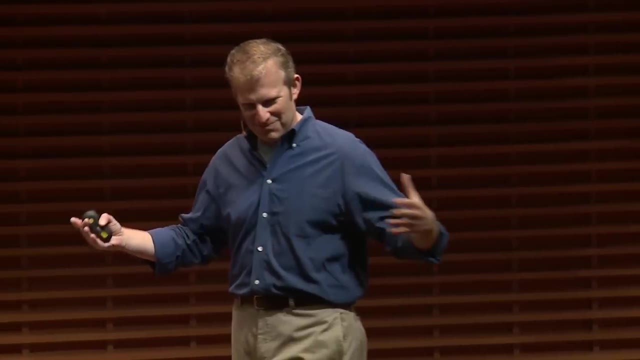 that you're going to do today. Okay, Do what you were really going to do for fun, and not do things like F-E-E-D-T-H-E-C-A-T right, Just because you don't want to spell right? So you can use big. 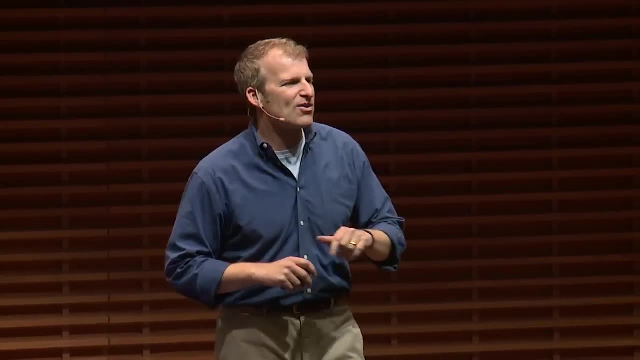 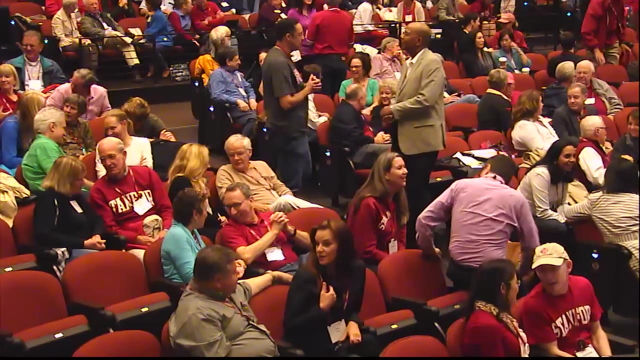 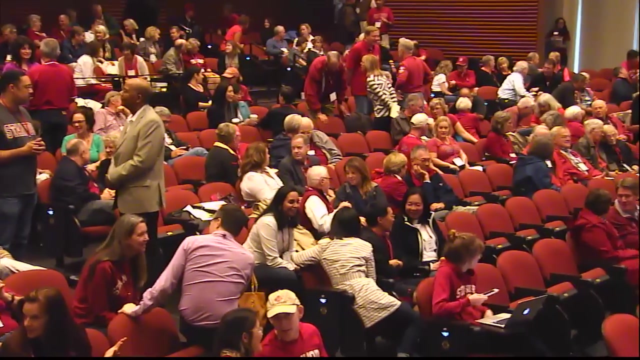 words, All right, 30 seconds each Spell to your partner, something fun that you're going to do today. Would you like to play? Go ahead, G-O-T-H-E-G-A-M-E. Oh, my goodness, Say it again. Spell it again. 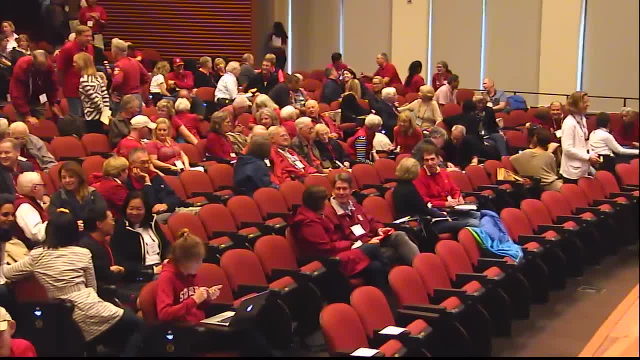 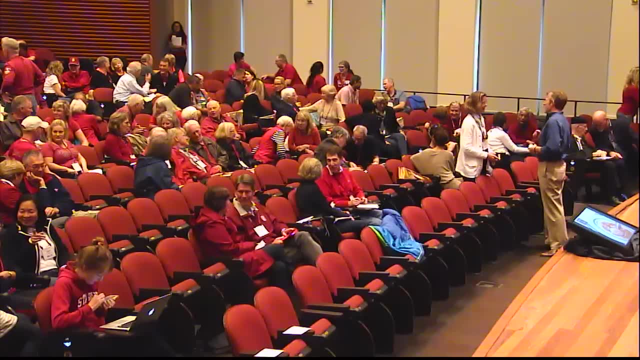 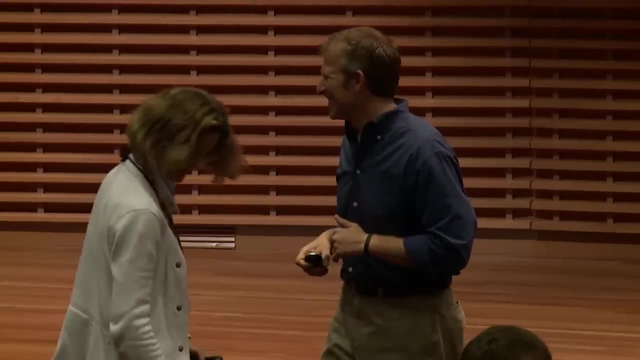 G-O-T-H-E-G-A-M-E, E-X-C-E-E-L-L-E-N-T. I-H-O-P-E-T-H-A-T-T-H-E-Y-W-I-N. E-X-L-C-E-L-L-E-N-T. Thank you, That was very good. Thank you. 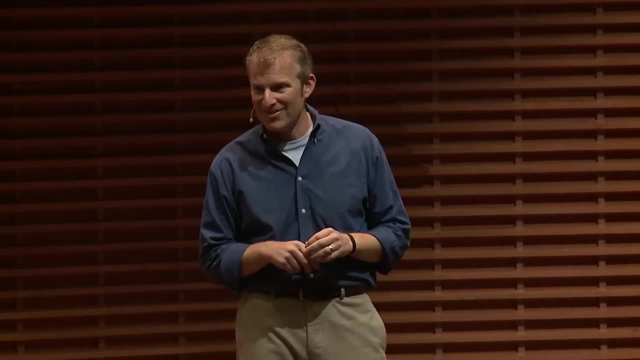 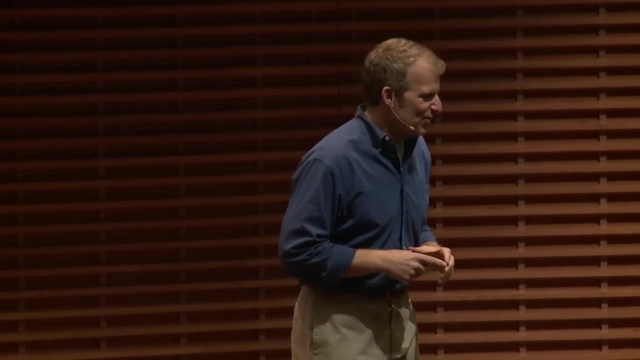 T-O-Y-O-U-R-P-A-R-T-N-E-R. I will translate. You are going to get with the same partner you just worked with And you are going to have a very brief conversation about something fun that you plan to do today. 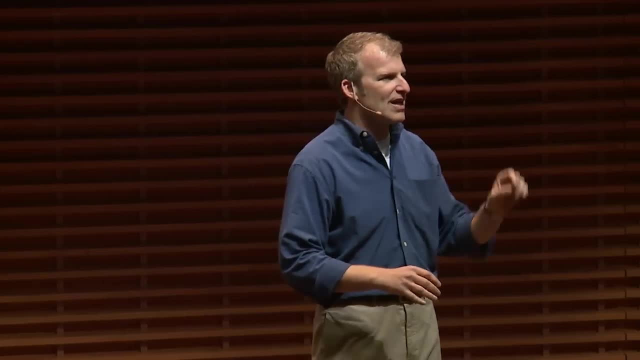 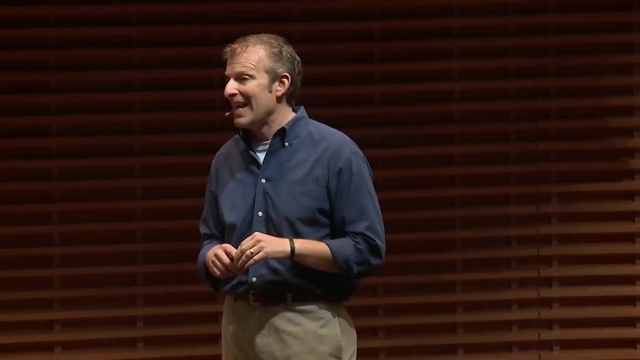 I know this is the most fun you're going to have all day, But the next fun thing you're going to do today you're going to tell your partner what you are going to do. that will be fun today, But you are going to do so by S-P-E-L-L-I-N-G-I-T. 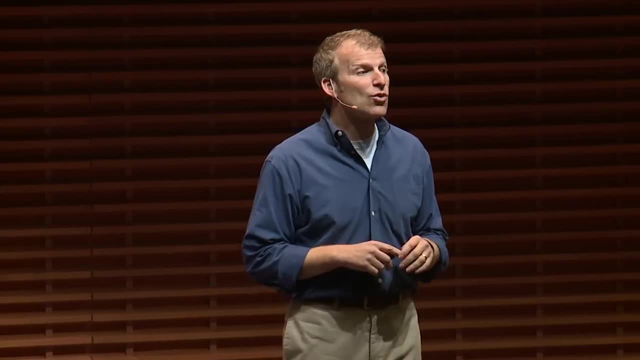 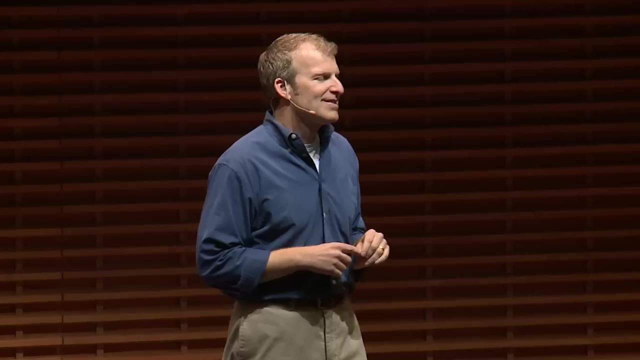 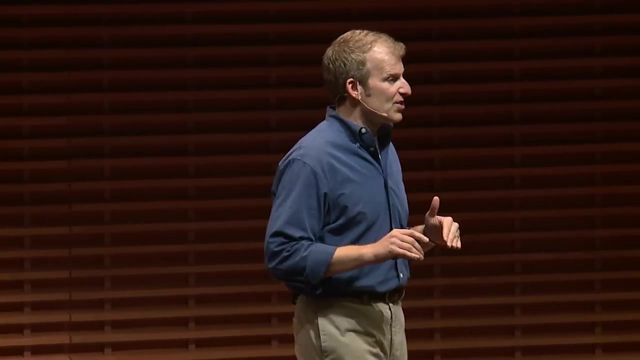 Okay, So you're going to spell it. It's okay if you are not a good speller. Okay, You'll see the benefit of doing this. So, with the partner you just worked with, person A is going to go first this time. 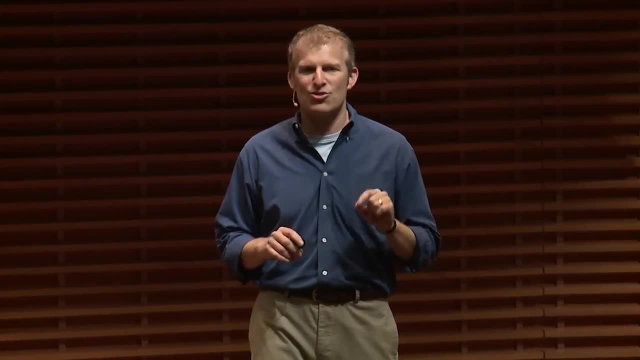 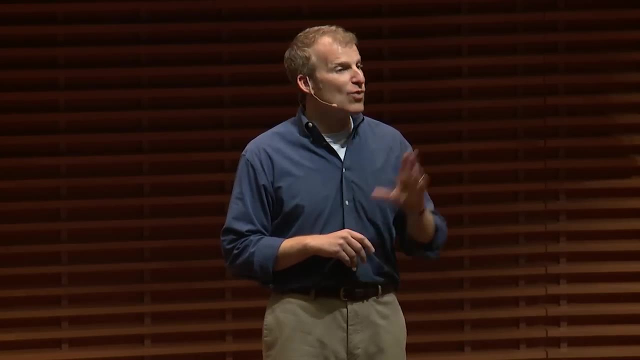 You are simply going to tell your partner- Actually, you're going to spell to your partner What it is of fun, something of fun that you are going to do today. Okay, Do what you were really going to do for fun, and not do things like F-E-E-D-T-H-E-C-A-T. 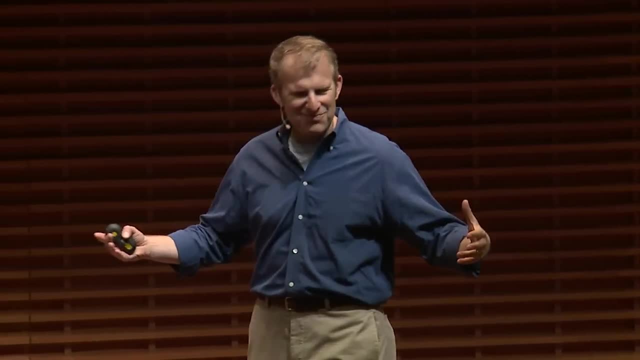 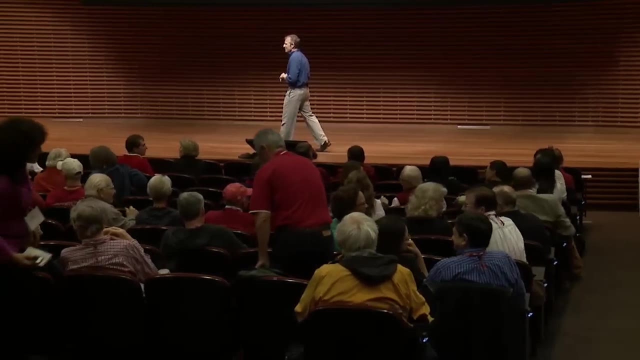 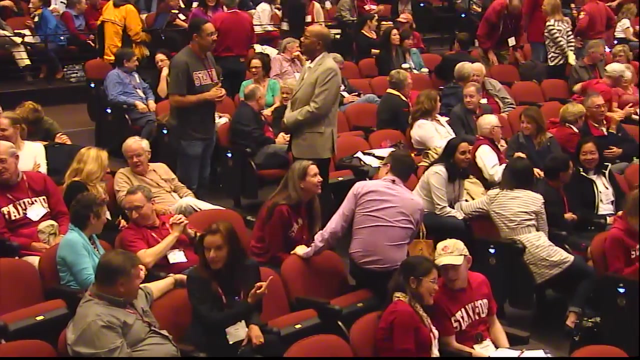 Right, Just because you don't want to spell Right, So you can use big words. Alright, 30 seconds each Spell to your partner. something fun that you are going to do today. Would you like to play? Go ahead. 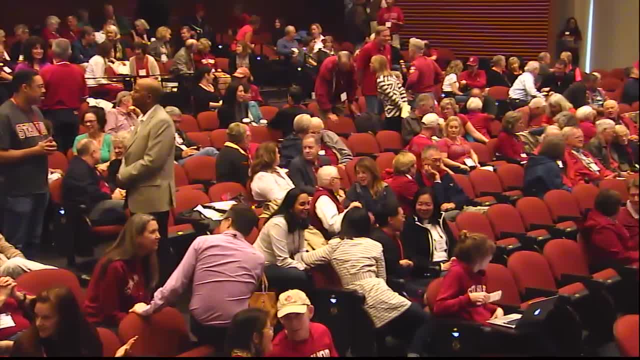 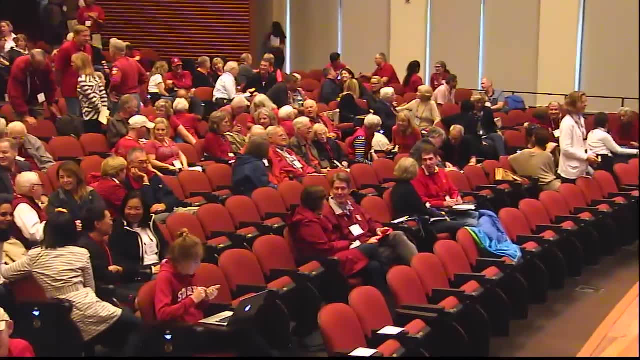 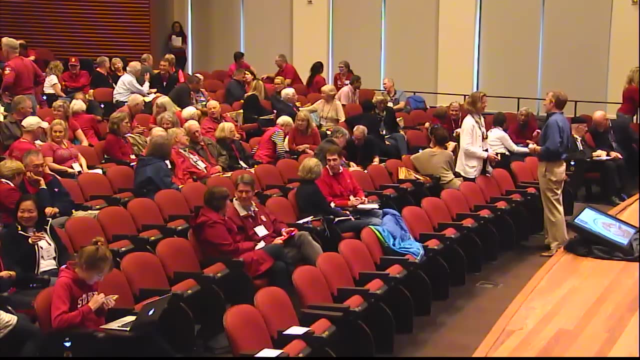 G-O-T-H-E-G-A-M-E. Oh, my goodness, Say it again. Spell it again. G-O-T-H-E-G-A-M-E, E-X-C-E-E-L-L-E-N-T, I-H-O-P-E-T-H-A-T-T-H-E-Y-W-I-N. 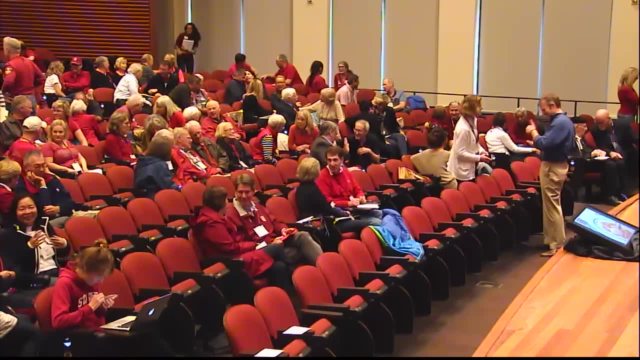 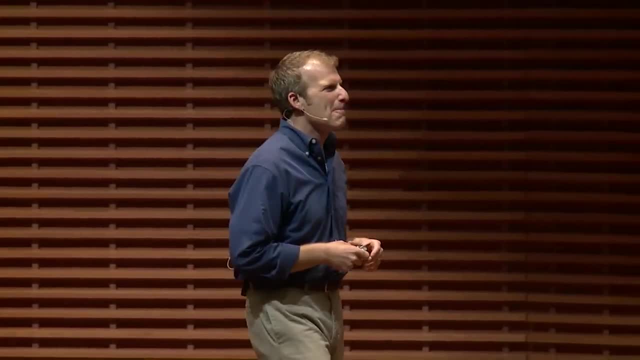 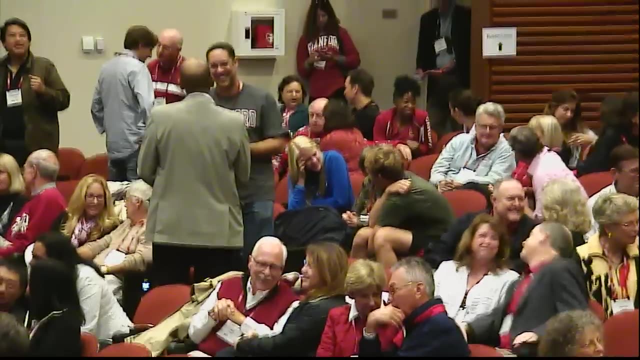 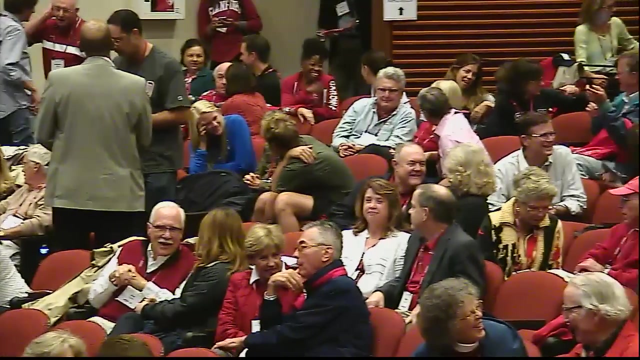 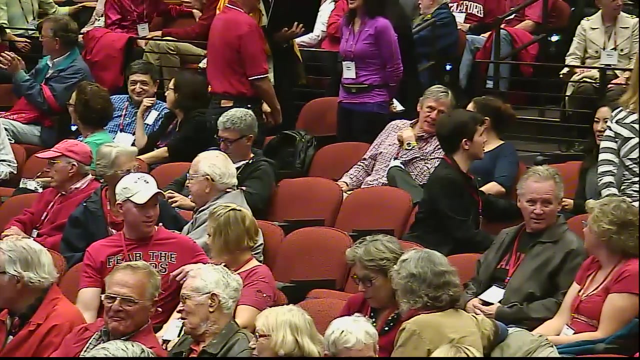 E-X-C-E-E-L-L-E-N-T. Thank you, That was very good. Thank you, If you have not switched, switch. Take 30 more seconds with the new partner spelling: E-X-C-E-E-L-L-E-N-T. 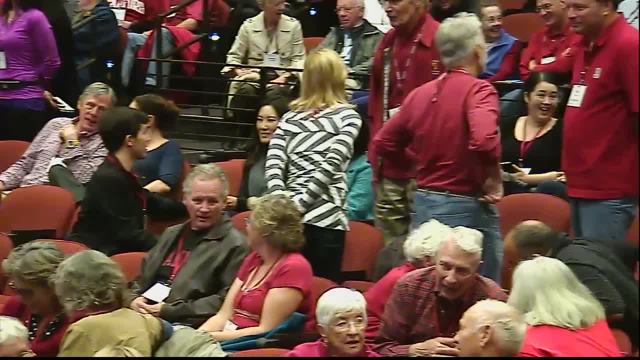 E-X-C-E-E-L-L-E-N-T, E-X-C-E-E-L-L-E-N-T, E-X-C-E-E-L-L-E-N-T, E-X-C-E-E-L-L-E-N-T, E-X-C-E-E-L-L-E-N-T. 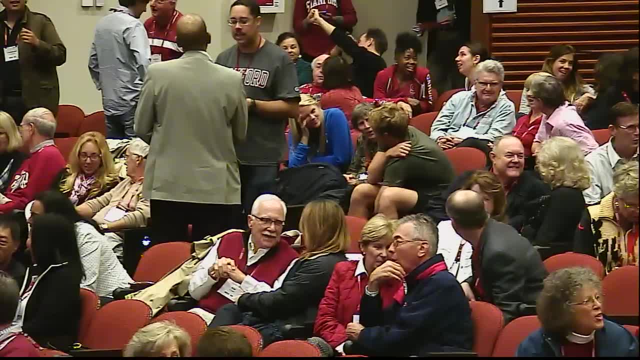 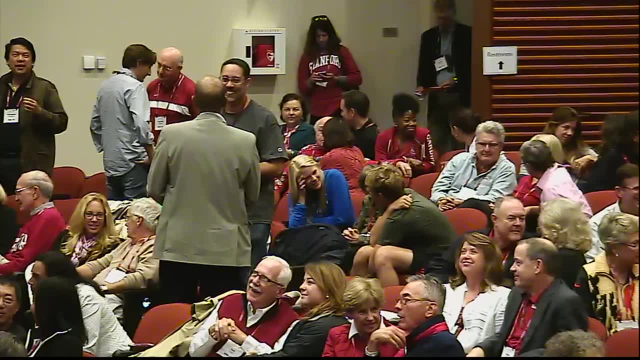 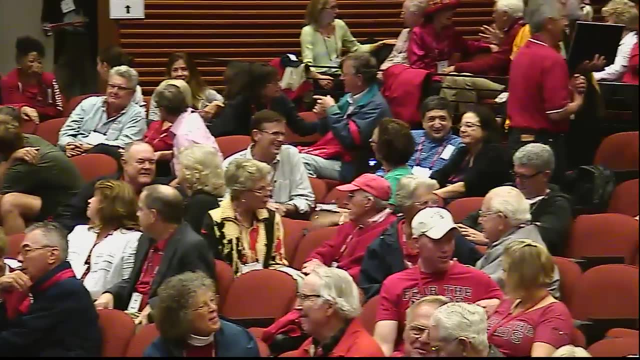 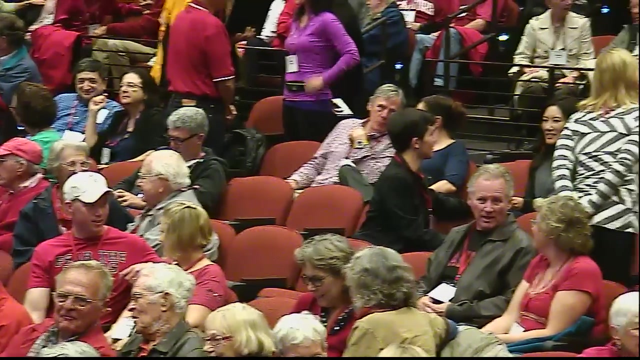 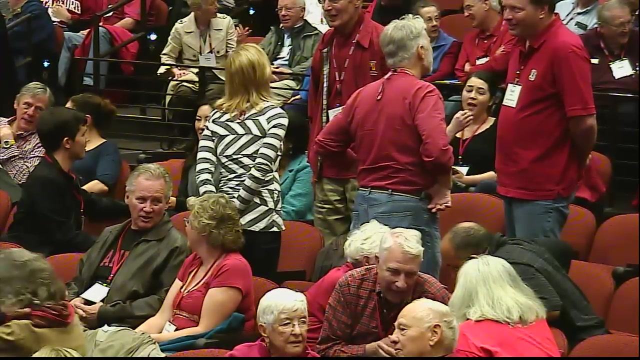 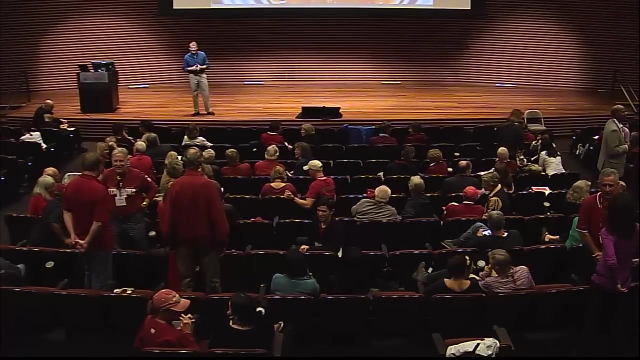 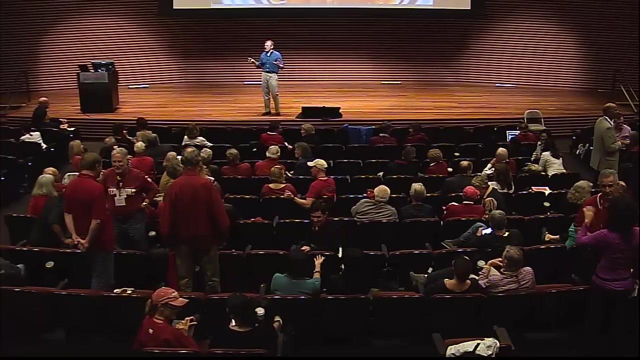 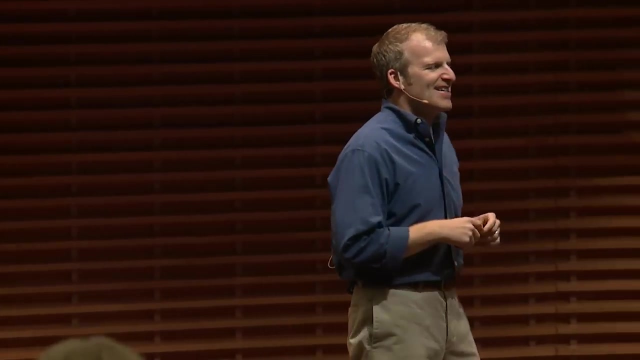 If you have not switched switch. Take 30 more seconds with the new partner spelling: E-X-L-C-E-L-L-E-N-T. I-H-O-P-E-T-H-A-T-H-A-T-H-E-N-G. Thank you, Y-O-U-R-S-E-A-T. 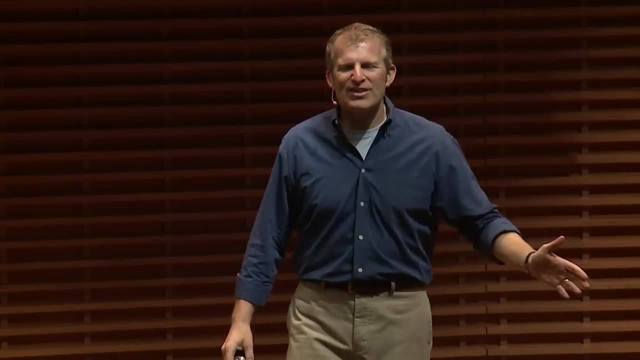 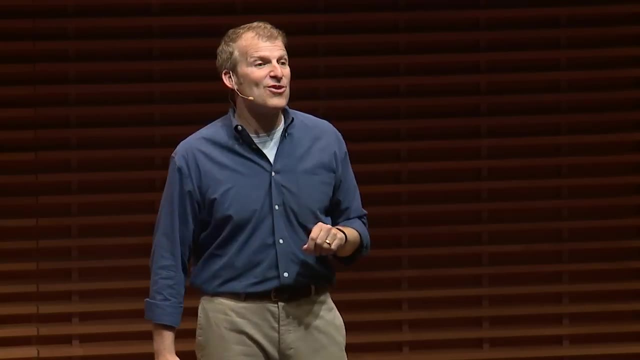 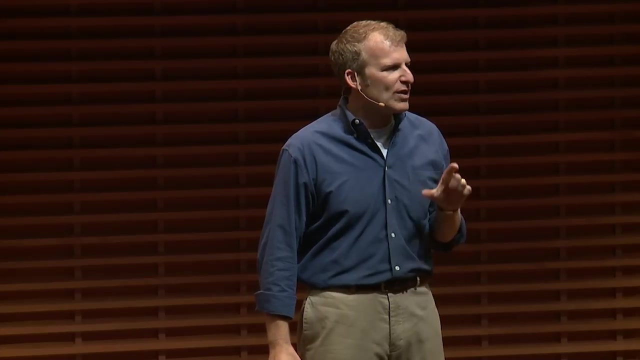 So what did we learn? What did we learn Besides that we're not so good at spelling. You have to pause between the words. How did this change your interaction with the person you were interacting with? What did you have to do? Focus? 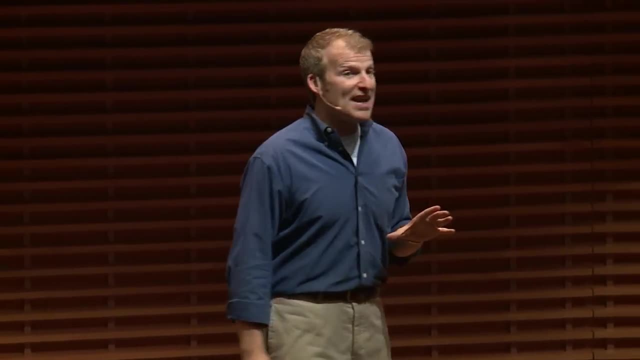 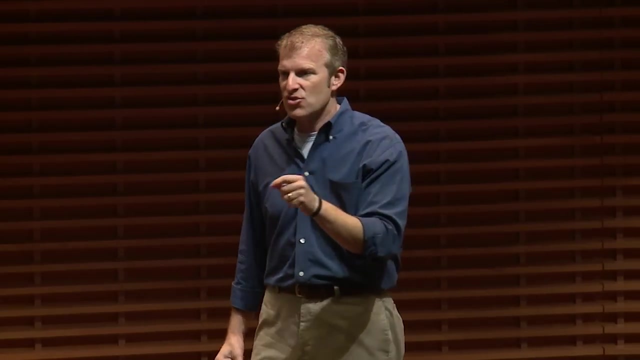 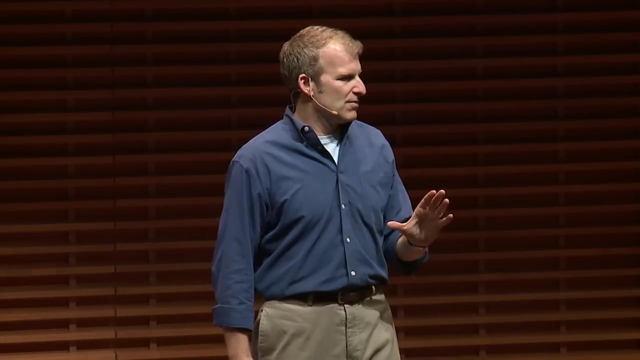 And listen And you can't be thinking ahead. You have to be in the moment, When you listen and truly understand what the person is trying to say. then you can respond in a better way, a more targeted response. We often don't listen. 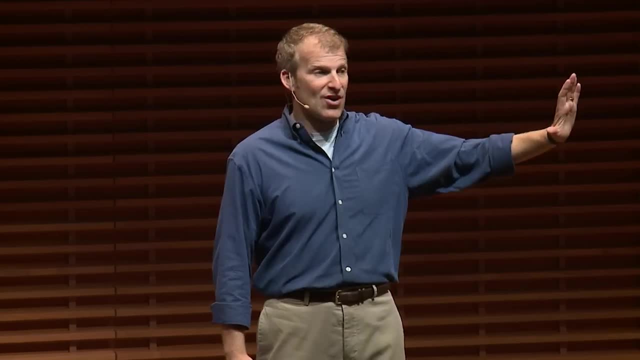 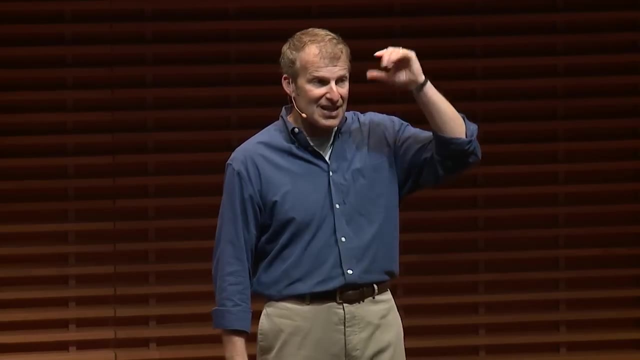 So we start by getting out of our own way. We then reframe the situation as an opportunity. Those are things we do inside our head, But in the moment of interacting we have to listen first before we can respond to the spontaneous request. 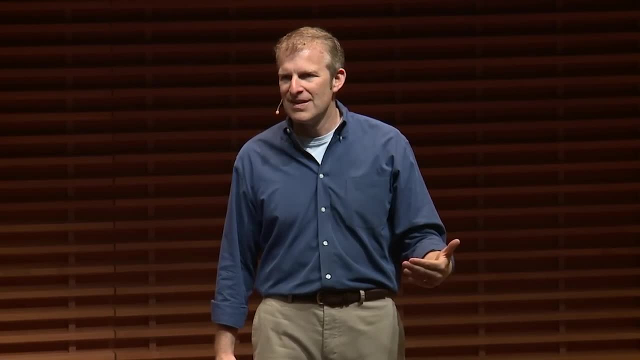 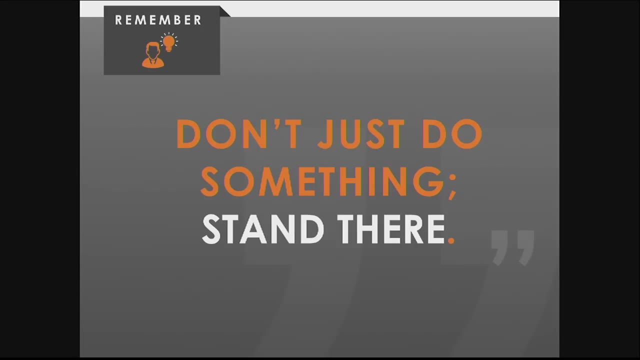 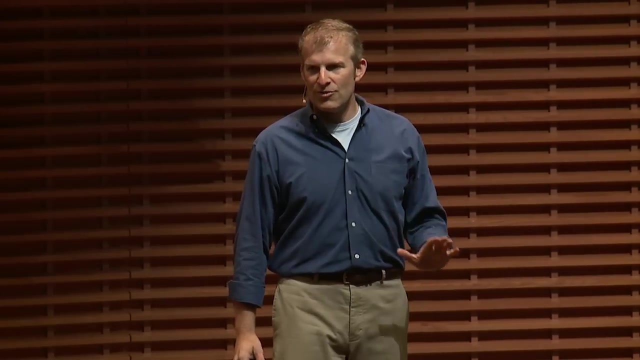 Perhaps my most favorite maxim comes from this activity. Don't just do something. Stand there, Listen, Listen And then respond. Now, how do we respond? That brings us to the fourth part of our process, And that is we have to tell a story. 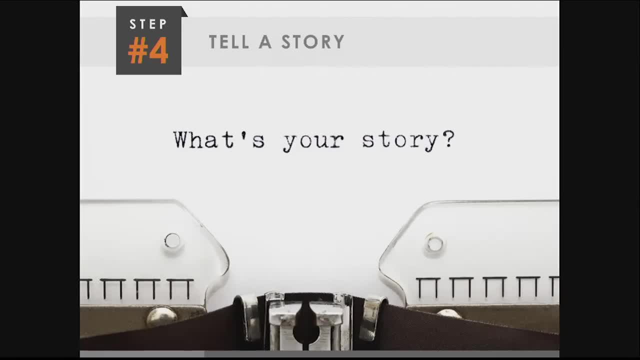 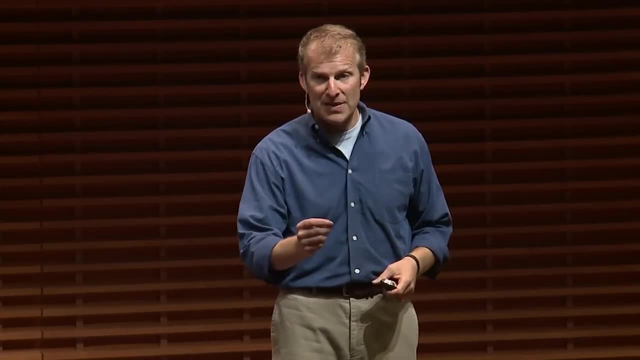 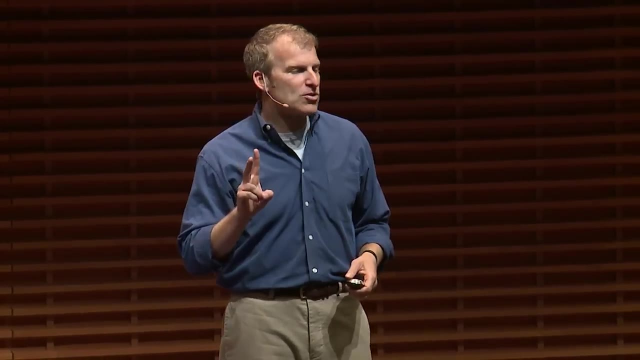 We respond in a way that has a structure. All stories have structure. We have to respond in a structured way. The key to successful spontaneous speaking and, by the way, planned speaking- is having a structure. I would like to introduce you to two of the most prevalent and popular. 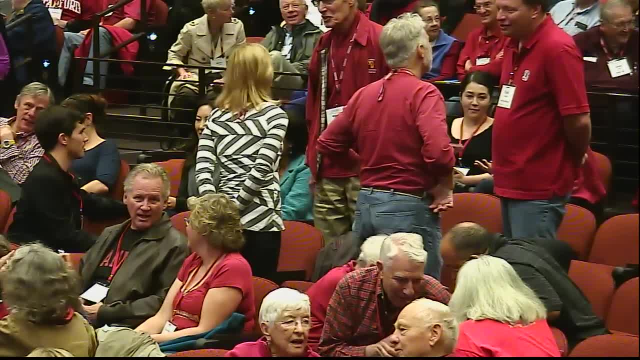 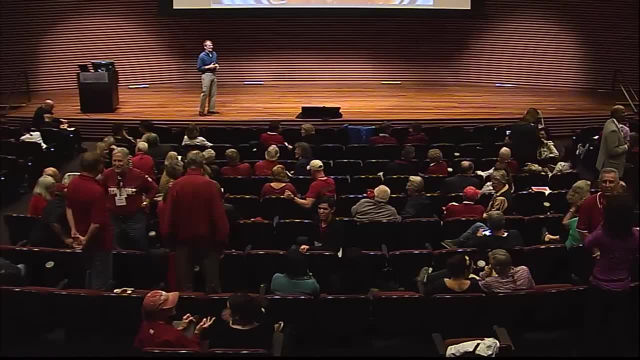 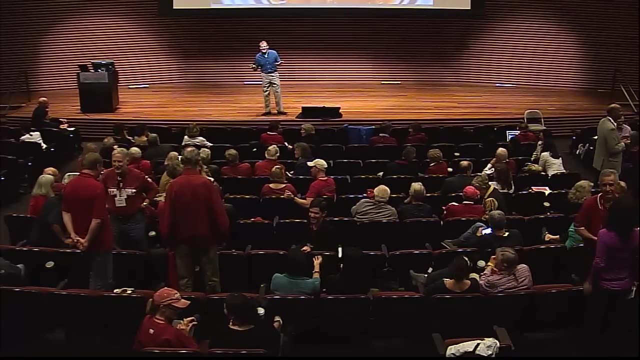 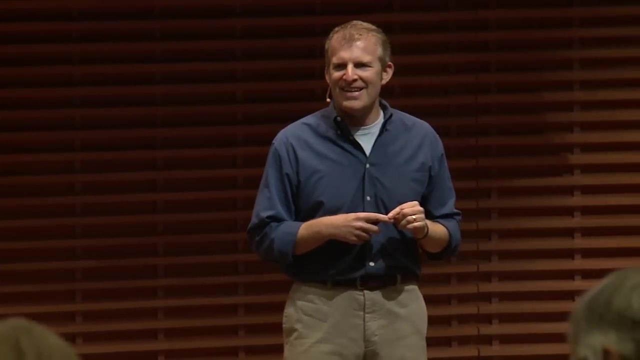 E-X-C-E-E-L-L-E-N-T, E-X-C-E-E-L-L-E-N-T, r-e-a-t, G-r-e-a-t, T-h-a-n-k-y-o-u-p-l-e-a-s-e-t-a-k-e-y-o-u-r-s-e-a-t. 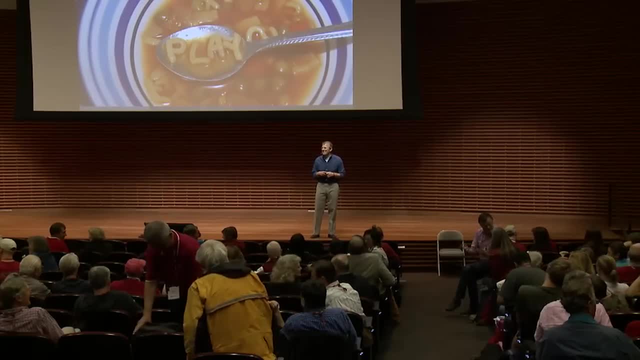 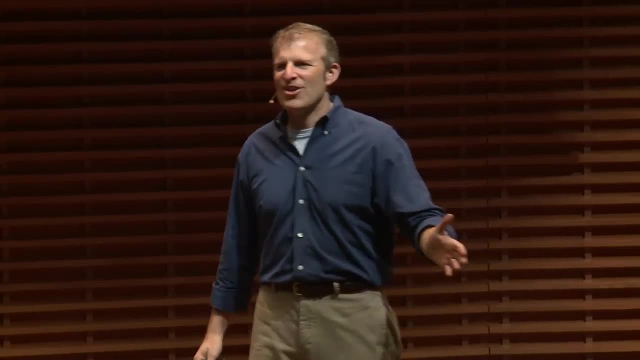 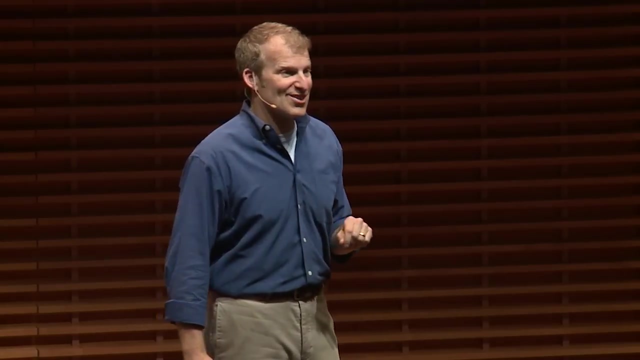 Thank you, YO-U-C-H-A-a-m. So what did we learn? What did we learn besides that? we're not so good at spelling. You have to pause between the words. How did this change your interaction with the person you were interacting with? 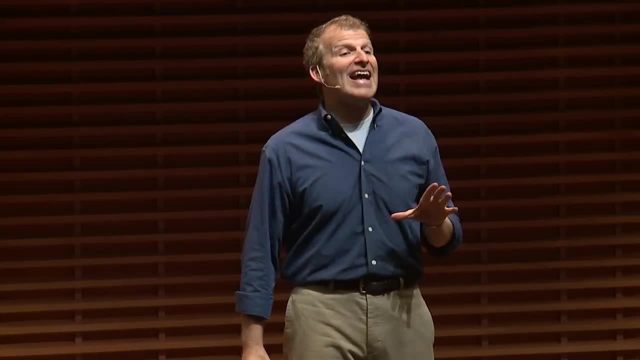 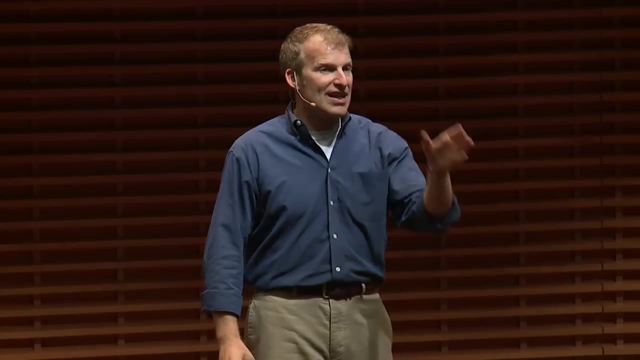 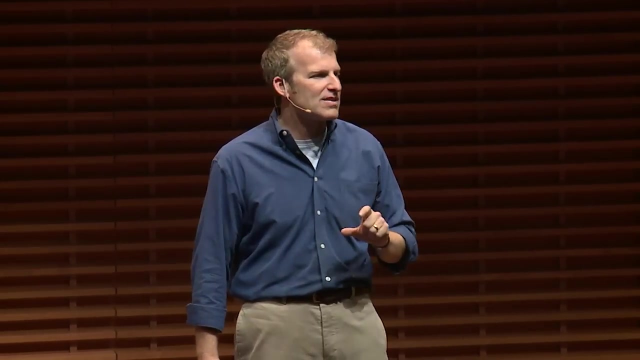 What did you have to do? Focus and listen, And you can't be thinking ahead. You have to be in the moment, When you listen and truly understand what the person is trying to say. then you can respond in a better way. a more targeted response. 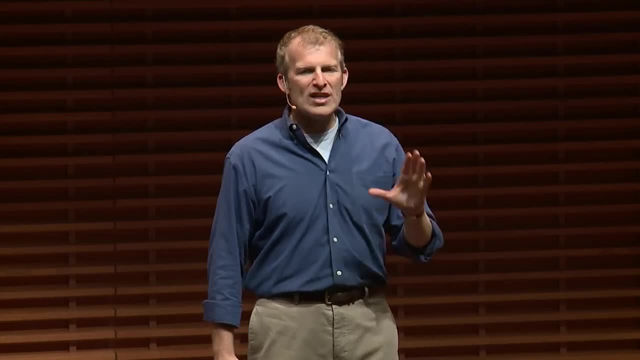 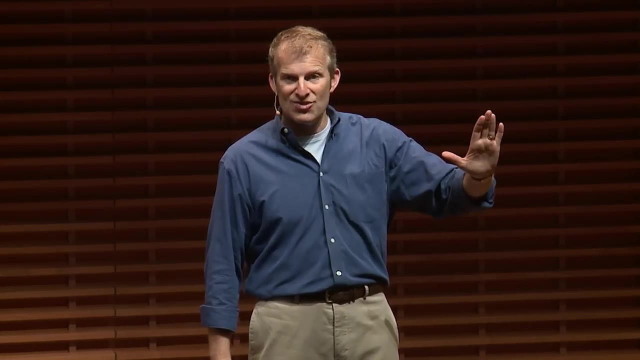 We often don't listen, So we start by getting out of our own way. We then reframe the situation as an opportunity. Those are things we do inside our head, But in the moment of interacting we have to listen first before we can respond to the 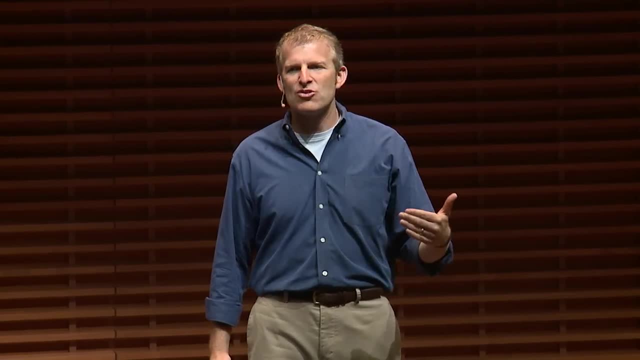 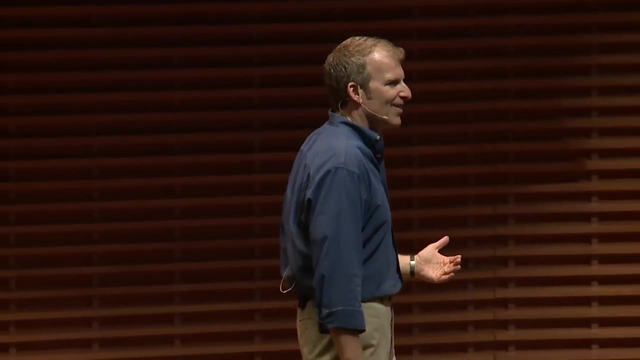 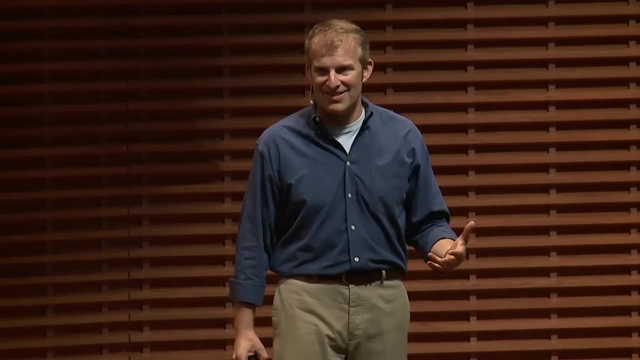 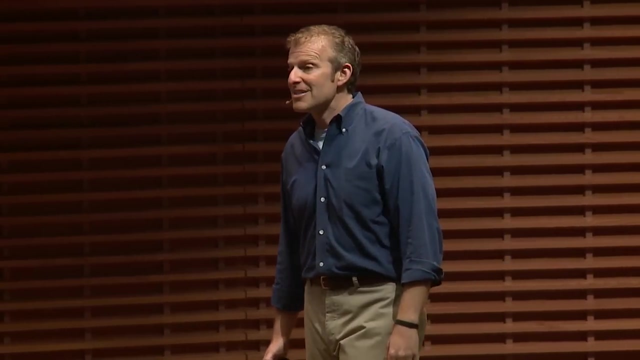 spontaneous request. Perhaps my most favorite maxim comes from this activity. Don't just do something, stand there, Listen, Listen and then respond. Now, how do we respond? That brings us to the fourth part of our process, And that is we have to tell a story. 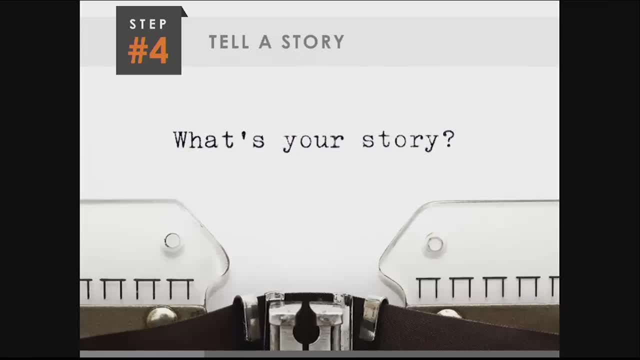 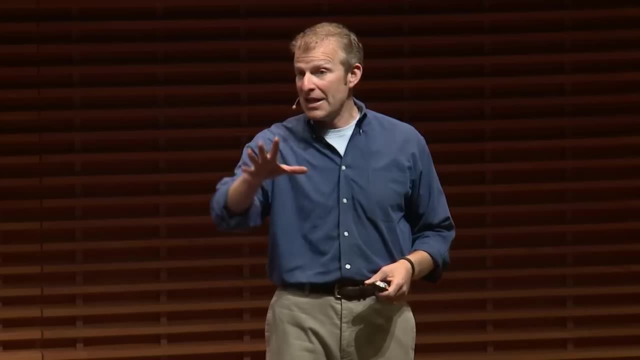 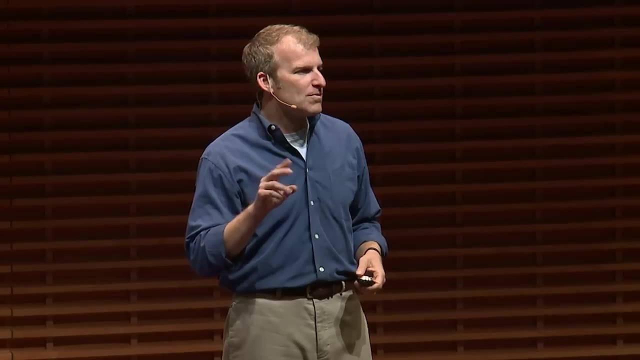 We respond in a way that has a structure. All stories have structure. We have to respond in a structured way. The key to successful spontaneous speaking and, by the way, planned speaking, is having a structure. I would like to introduce you to two of the most prevalent and popular and useful structures. 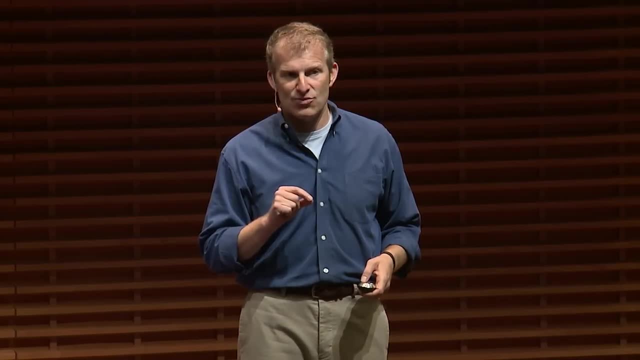 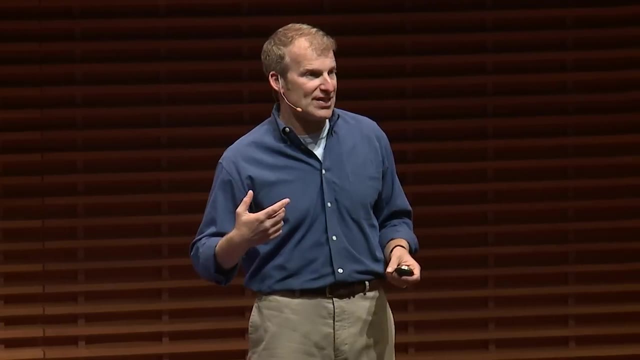 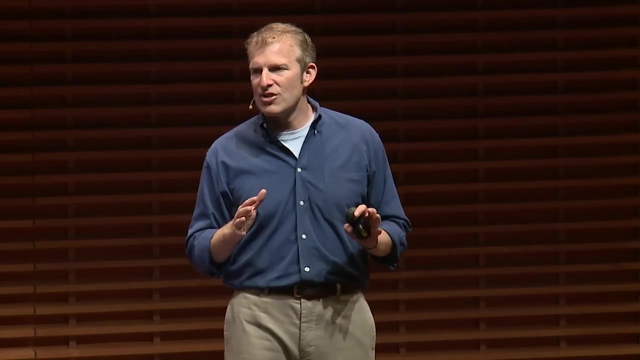 you can use to communicate a message in a spontaneous situation, But before we get there, we have to talk about the value of structure. It increases what is called processing fluency, the effectiveness of which, or through which, we process information. We actually process structured information roughly 40% more effectively and efficiently. 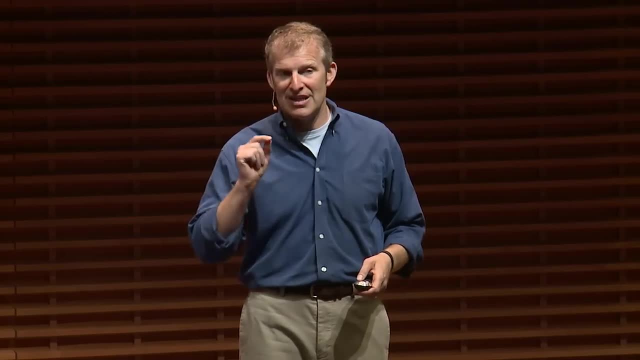 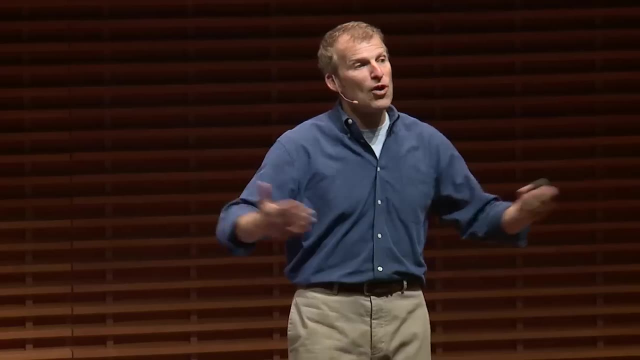 and useful structures you can use to communicate a message in a spontaneous situation. But before we get there, we have to talk about the value of structure. It increases what is called processing fluency, the effectiveness of which, or through which we process information. 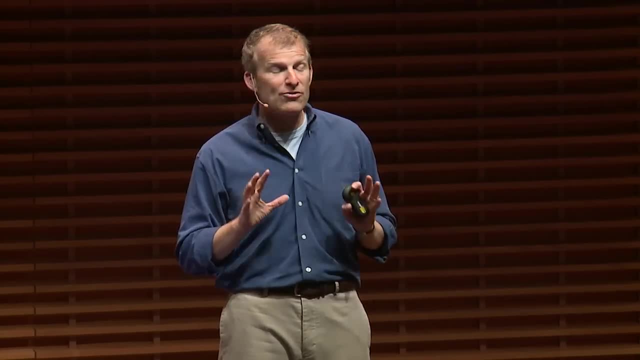 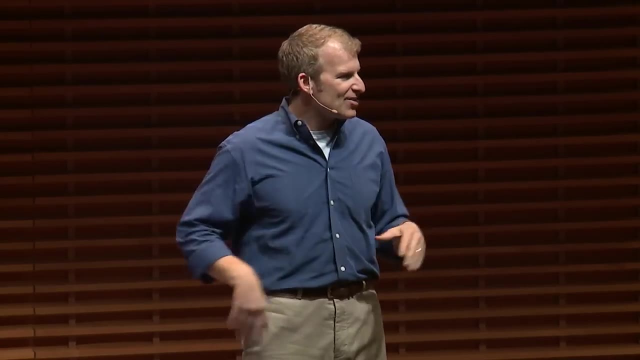 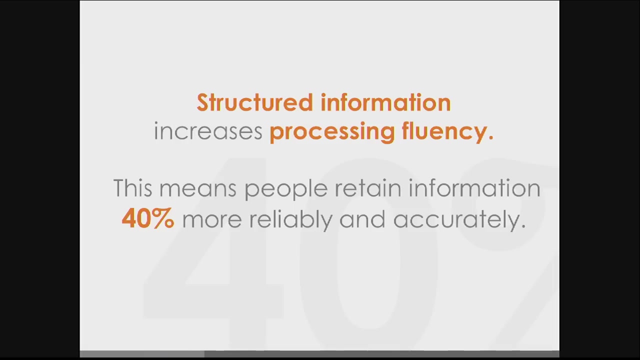 We actually process structured information roughly 40% more effectively and efficiently than information that's not structured. I love looking out in this audience because you will remember, as I remember, phone numbers when you had to remember them if you wanted to call somebody. Young folks today don't need to remember phone numbers. 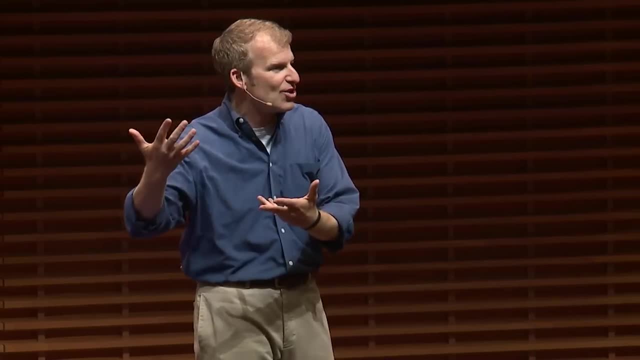 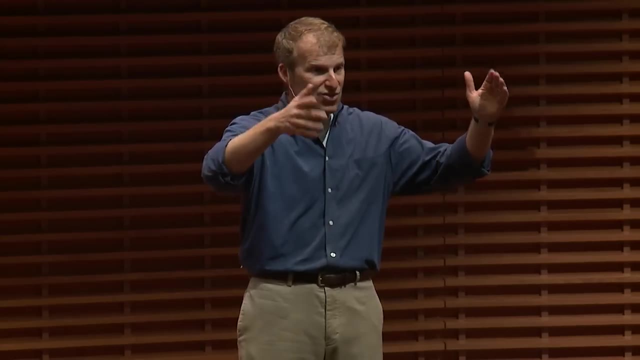 They just need to look at a picture, push a button and then the voice starts talking on the other end. Ten-digit phone numbers. it's actually hard to remember ten-digit phone numbers. How did you do it? You chunked it into a structure: three, three and four. 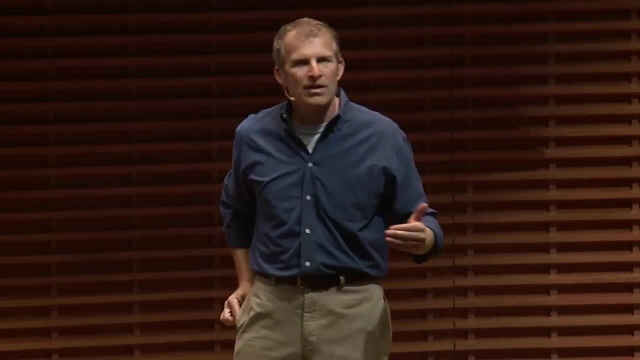 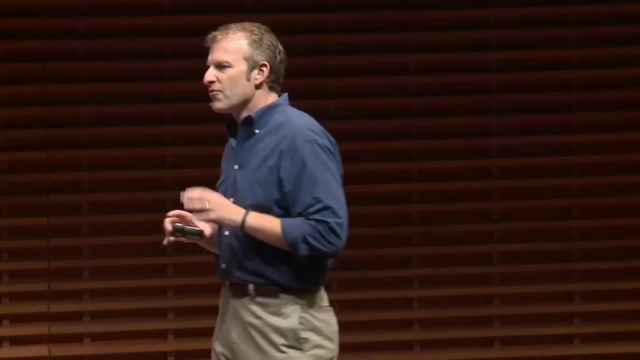 Structure helps us remember. The same is true when speaking spontaneously or in a planned situation. So let me introduce you to two useful structures. The first useful structure you have probably heard or used in some incarnation: It is the problem-solution-benefit structure. 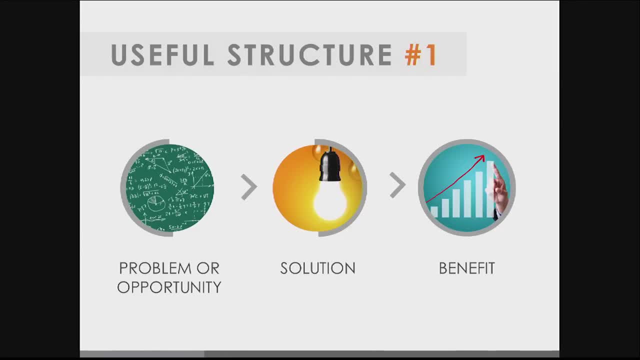 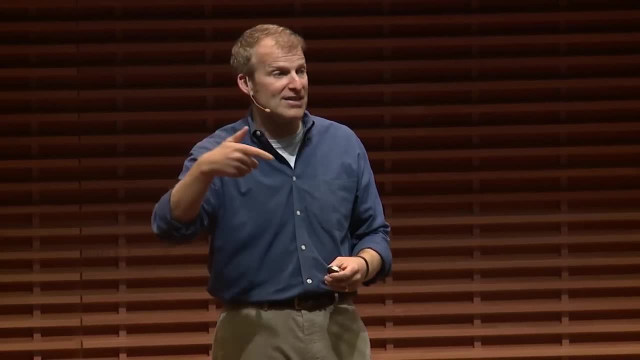 You start by talking about what the issue is, the problem. you then talk about a way of solving it and then you talk about the benefits of following through on it. Very persuasive, very effective. helps you, as the speaker, remember it, helps your audience know where you're going with it. 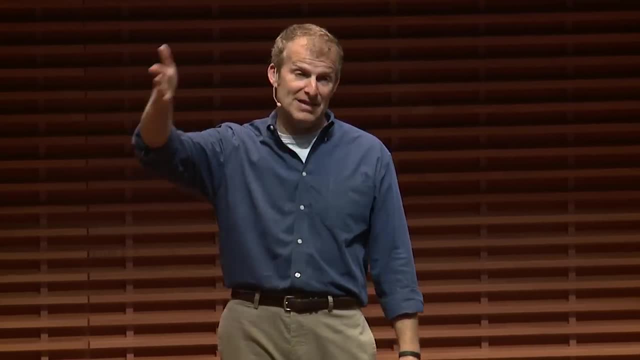 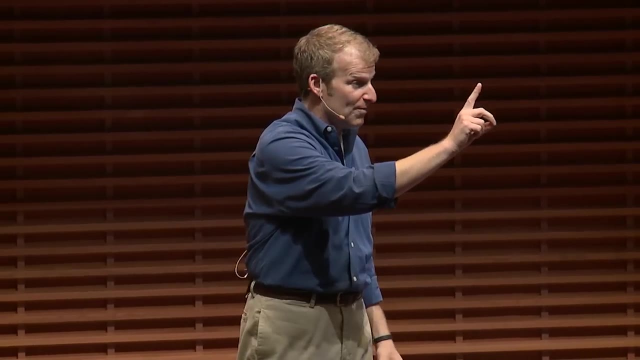 When I was a tour guide on this campus many, many, many years ago, what do you think the single most important thing they drilled into our heads? It took a full quarter, by the way, to train to be a tour guide here. 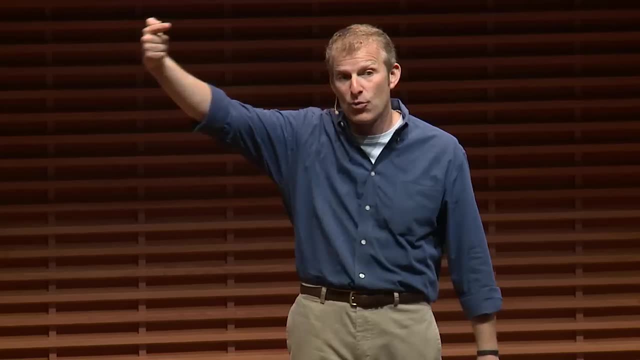 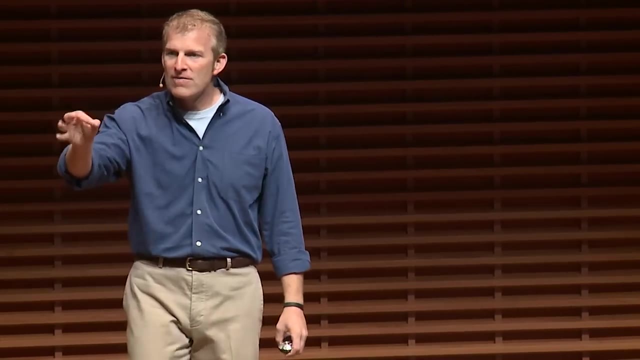 They used to line us up at one end of the quad and have us walk backwards straight, and if you failed, you had to start over. To this day, I can walk backwards in a straight line because of that. As part of that training, what do you think the most important thing they taught us was? 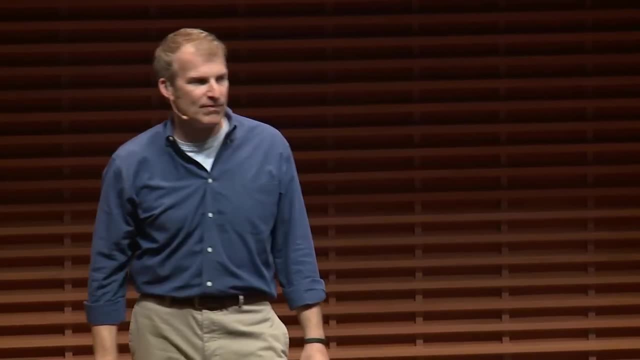 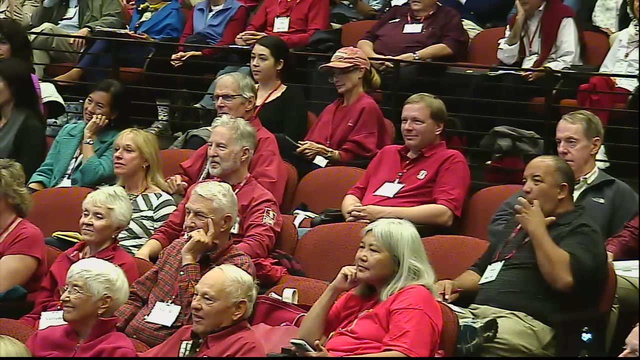 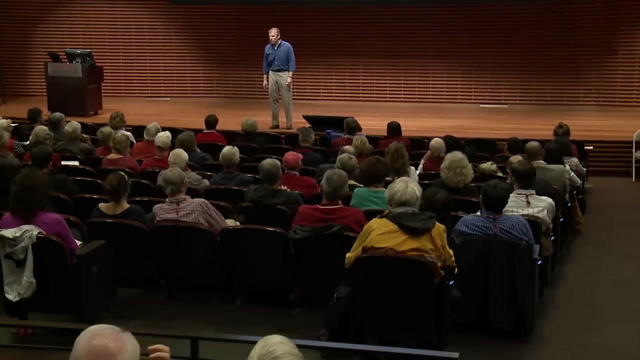 Never lose your tour group. I'm not joking: Never lose your tour group. The same is true as a presenter: Never lose your audience. The way you keep your audience on track is by providing structure. None of you would go on a tour with me if I said: 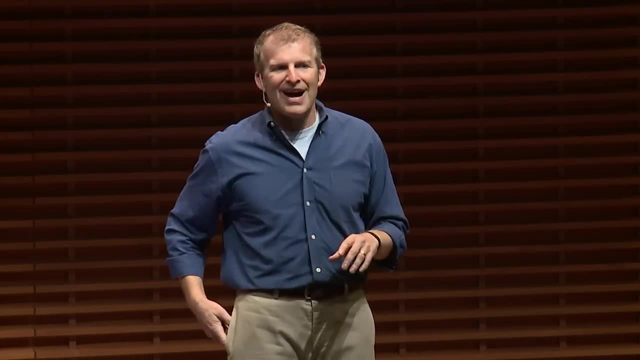 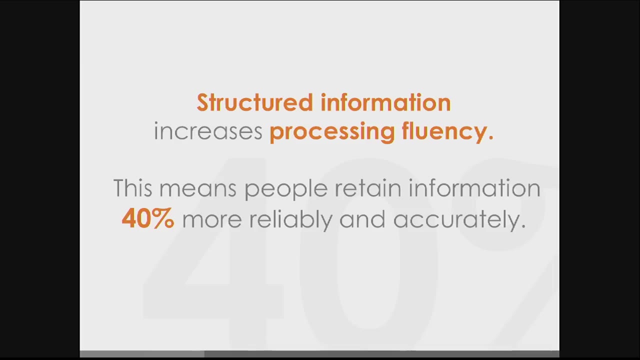 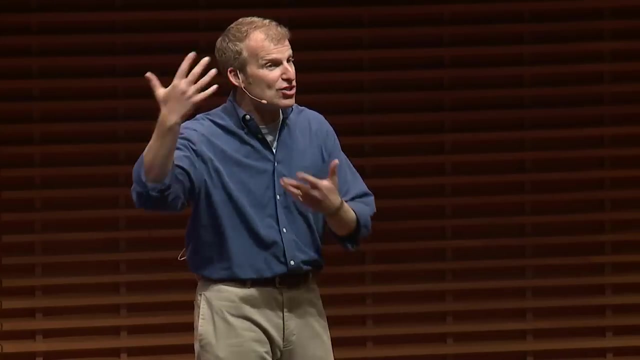 than information that's not structured. I love looking out in this audience because you will remember, as I remember, phone numbers when you had to remember them if you wanted to call somebody. Okay, young folks today don't need to remember phone numbers. They just need to look at a picture, push a button and then the voice starts talking. 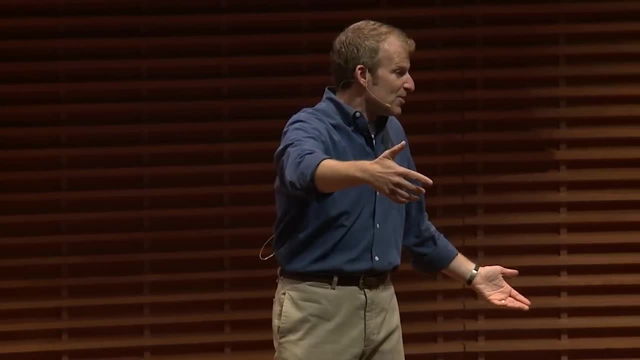 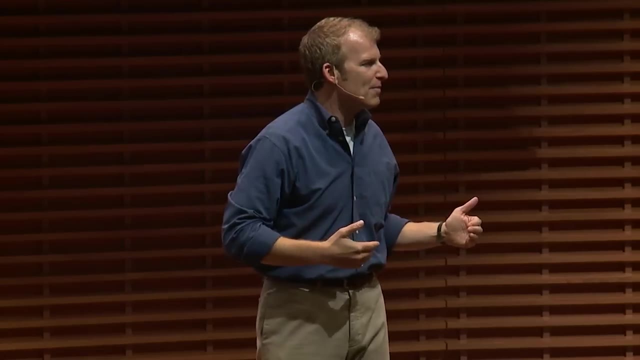 on the other end Ten-digit phone numbers. it's actually hard to remember ten-digit phone numbers. How did you do it? You chunked it into a structure: three, three and four. Structure helps us remember. The same is true when speaking spontaneously or in a planned situation. 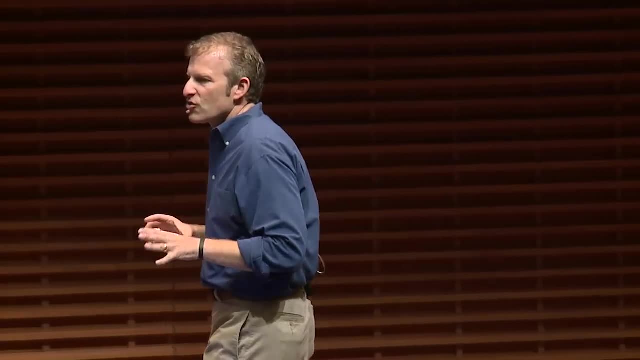 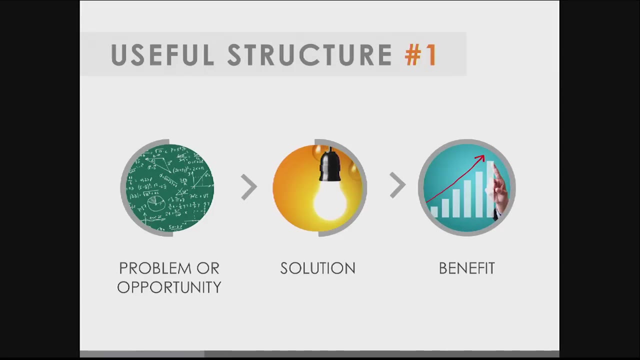 So let me introduce you to two useful structures. The first useful structure you have probably heard or used in some incarnation It is the problem-solution-benefit structure. You start by talking about what the issue is, the problem. You then talk about a way of solving it. 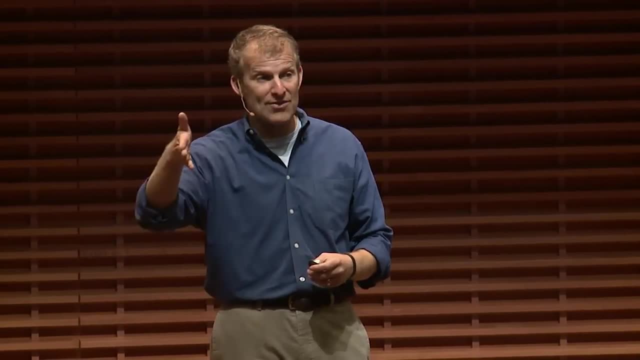 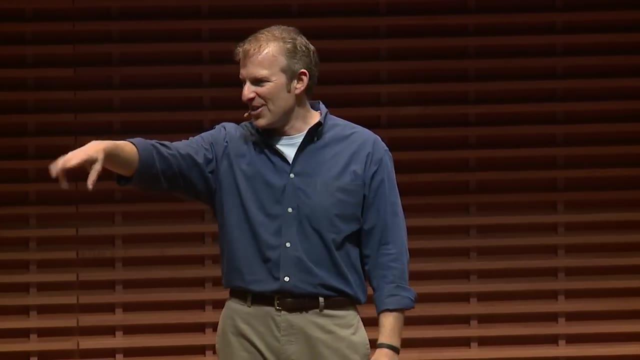 and then you talk about the benefits of following through on it. Very persuasive, very effective, Helps you, as the speaker, remember it, Helps your audience know where you're going with it. When I was a tour guide on this campus many, many, many years ago. 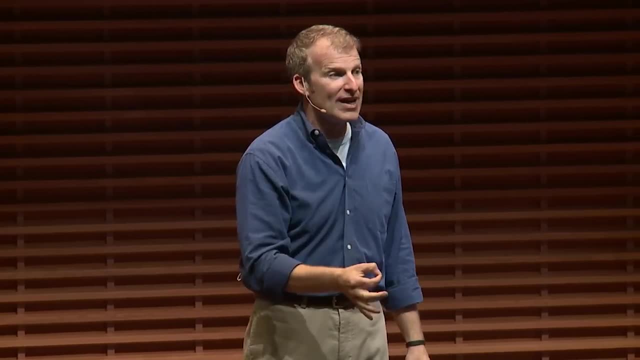 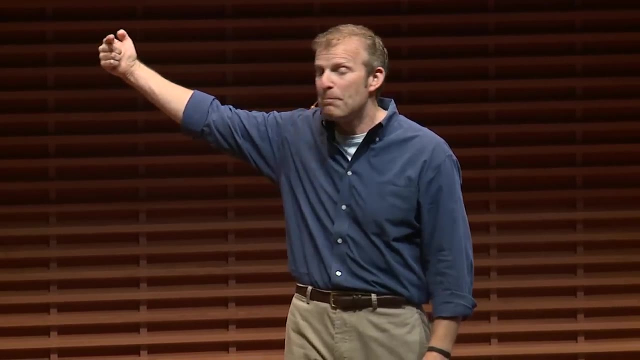 what, do you think, the single most important thing they drilled into our head? It took a full quarter, by the way, to train to be a tour guide here. They used to line us up at one end of the quad and have us walk backwards straight. 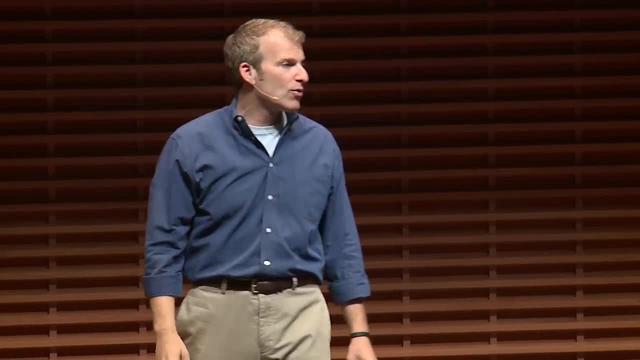 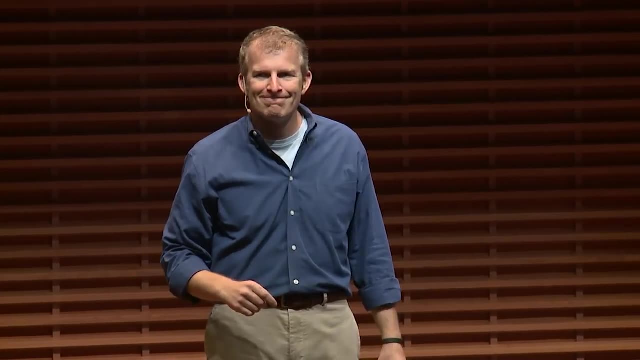 and if you failed, you had to start over. To this day, I can walk backwards in a straight line because of that. As part of that training, what do you think the most important thing they taught us was Never lose your tour group. 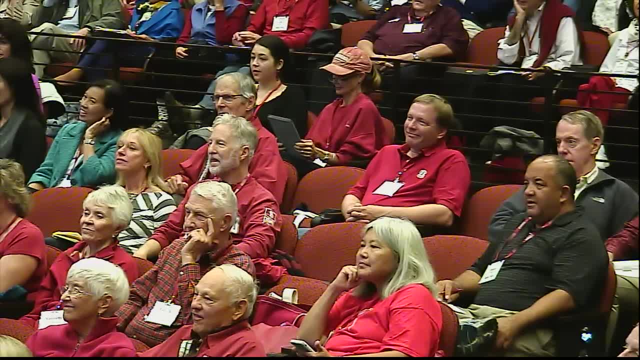 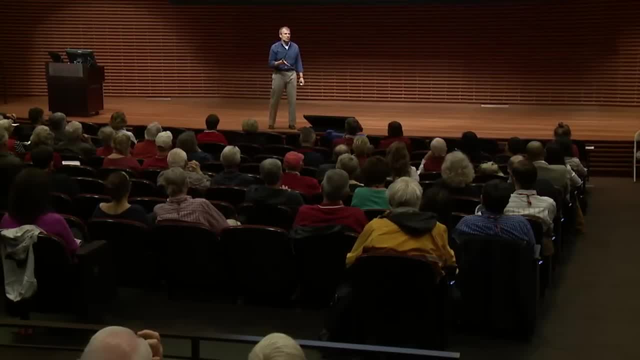 I'm not joking. Never lose your tour group. The same is true as a presenter. Never lose your audience. The way you keep your audience on track is by providing structure. None of you would go on a tour with me if I said: 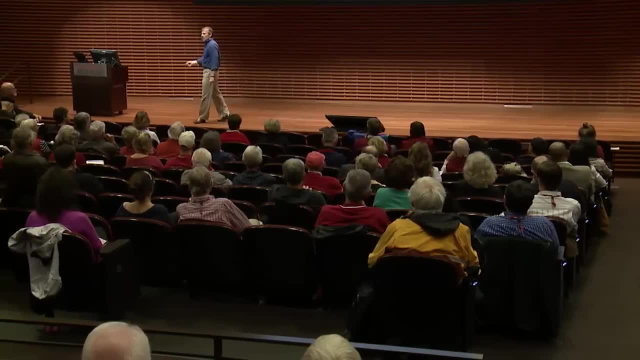 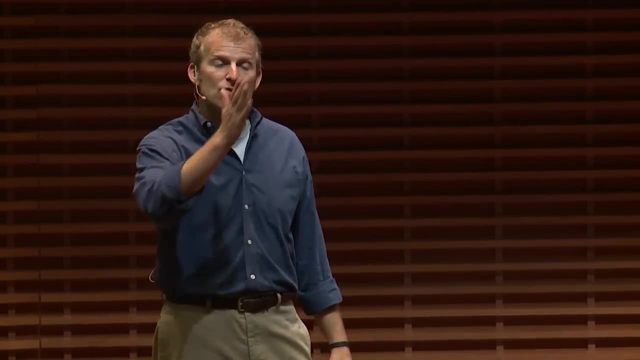 Hi, my name's Matt. Let's go. You want to know where you're going, why you're going there, how long it's going to take. You need to set expectations And structure does that Problem-solution-benefit is a wonderful structure to have in your back pocket. 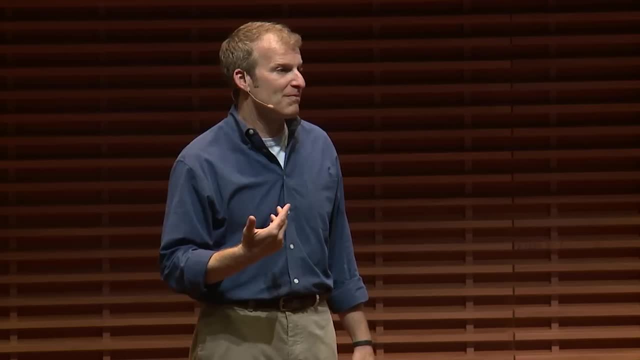 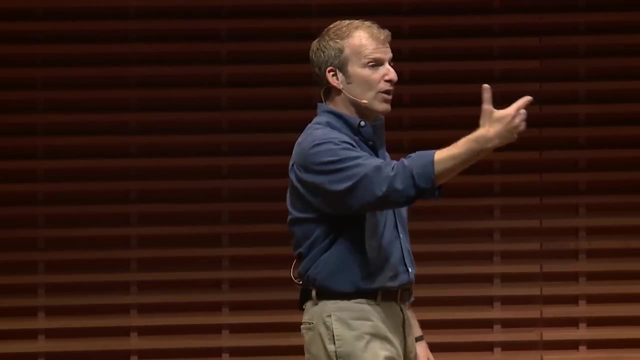 It's something that you can use quickly when you're in the moment. It can be reframed, so it's not always a problem you're talking about. Maybe it's an opportunity, Maybe there's a market opportunity you want to go out and capture. 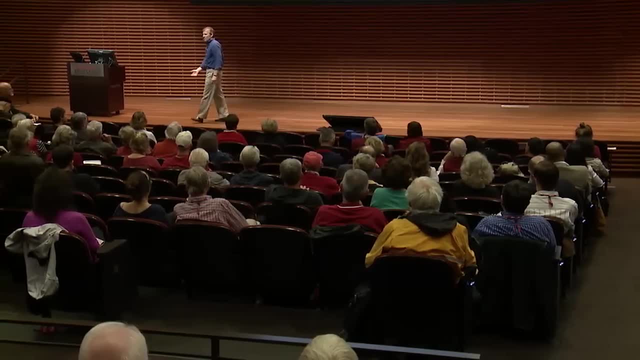 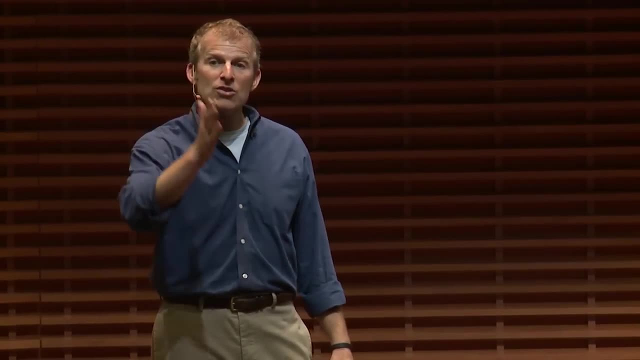 Hi, my name's Matt. Let's go. You want to know where you're going, why you're going there, how long it's going to take. You need to set expectations and structure does that Problem-solution benefit is a wonderful structure to have in your back pocket. 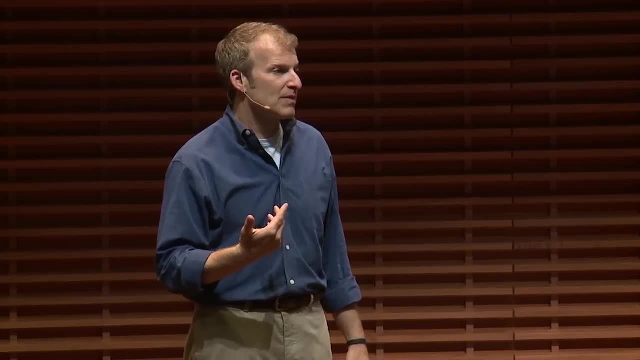 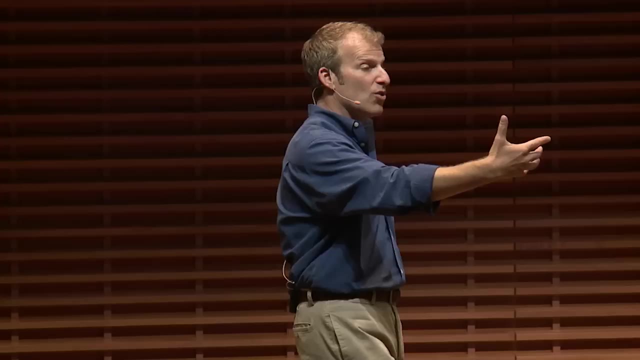 It's something that you can use quickly when you're in the moment. It can be reframed, so it's not always a problem you're talking about. Maybe it's an opportunity, Maybe there's a market opportunity you want to go out and capture. 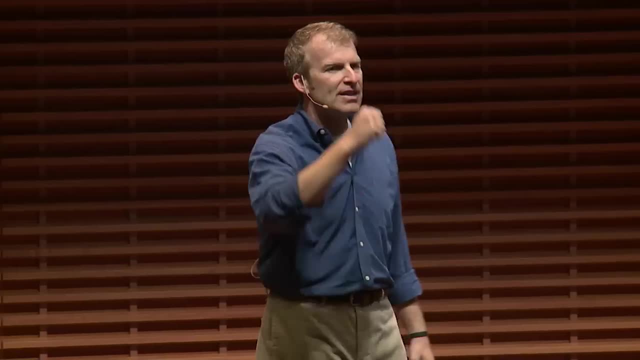 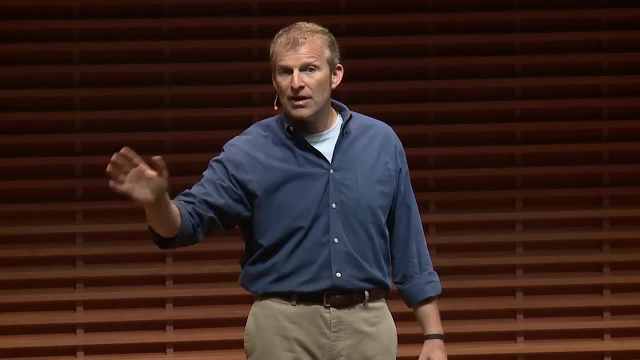 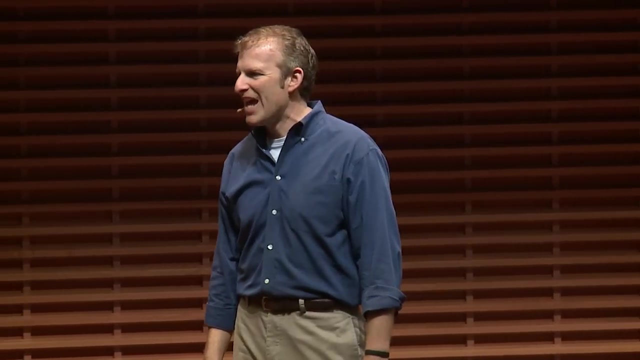 It's not a problem that we're not doing it, but maybe we'd be better off if we did So. it becomes opportunity, solution, which are the steps to achieve it, and then the benefit. Another structure which works equally well is the what. so what now? what structure? 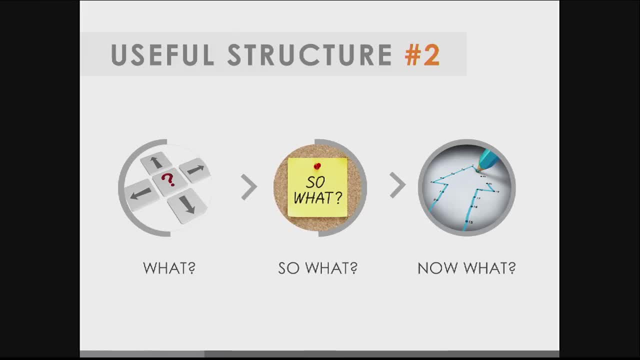 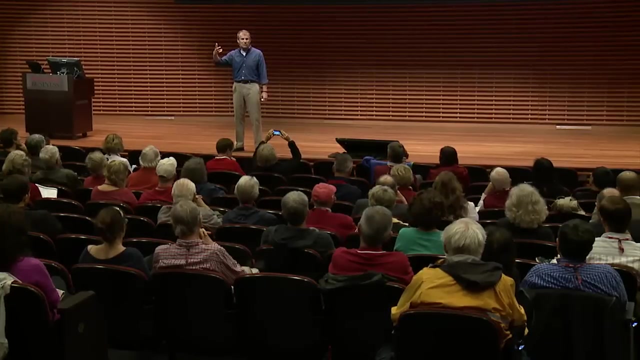 You start by talking about what it is, Then you talk about why it's important and then what the next steps are. This is a wonderful formula for answering questions, for introducing people. So if, in the moment, somebody asks me to introduce somebody, I change the what to who. 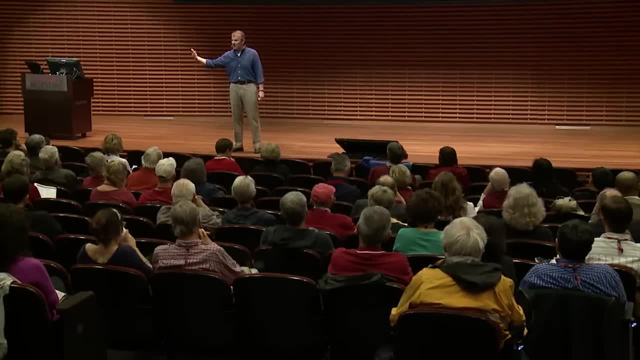 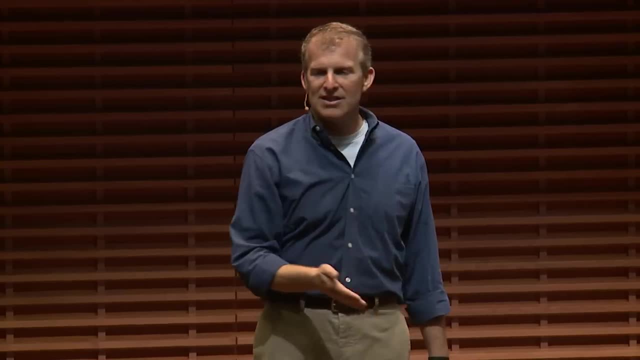 I say who they are, why they're important and what we're going to do next. Maybe listen to them, maybe drink our wine, whatever, What. so what now? what? The reality is this: When you are in a spontaneous speaking situation, you have to do two things simultaneously. 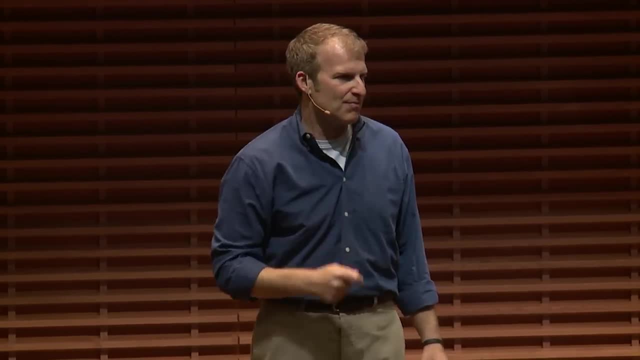 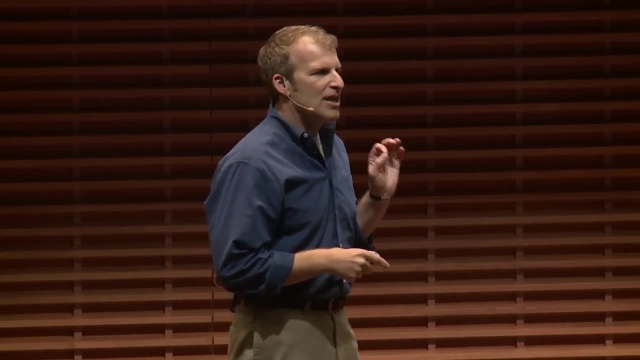 You have to figure out what to say and how to say it. These structures help you by telling you how to say it. If you can get it right, you can get it right. If you can become comfortable with these structures, you can be in a situation where 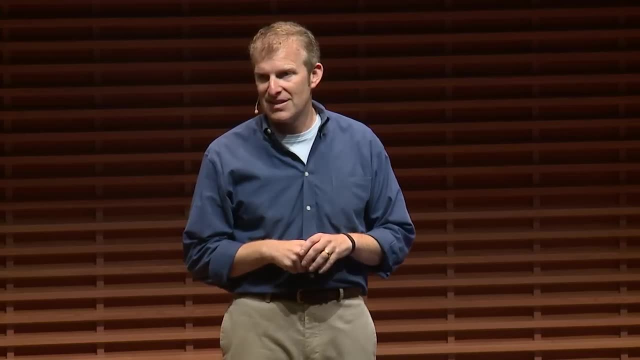 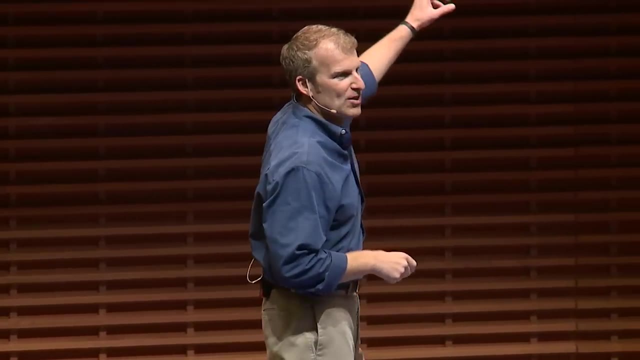 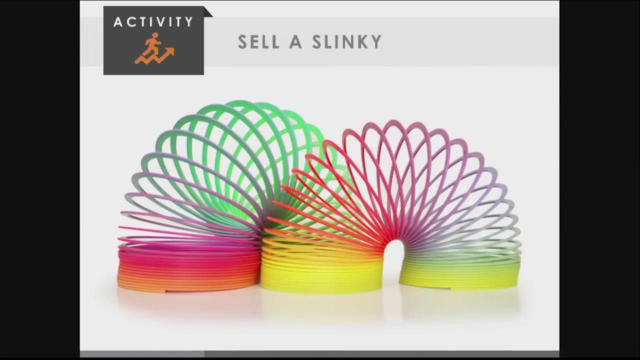 you can respond very ably to spontaneous speaking situations. We're going to practice, because that's what we do. Here's the situation. Is everybody familiar with this child's toy? It's a Slinky. You are going to sell this Slinky to your partner. using either problem solution benefit. 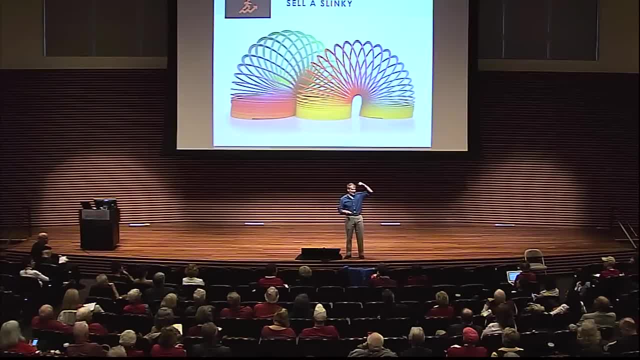 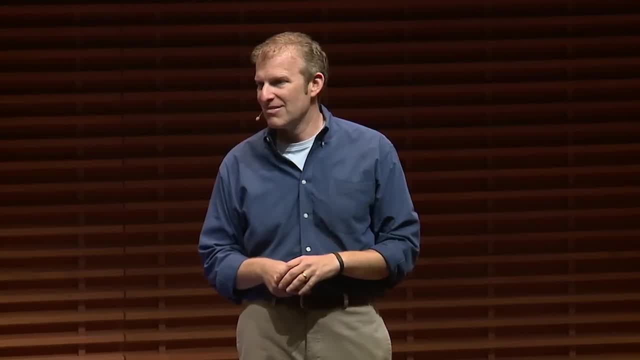 or opportunity solution benefit. What does the Slinky provide you, Or you could use what. so what now? what? What is it? Why is it important? The next steps might be to buy it By using that structure. see how, already, it helps you. 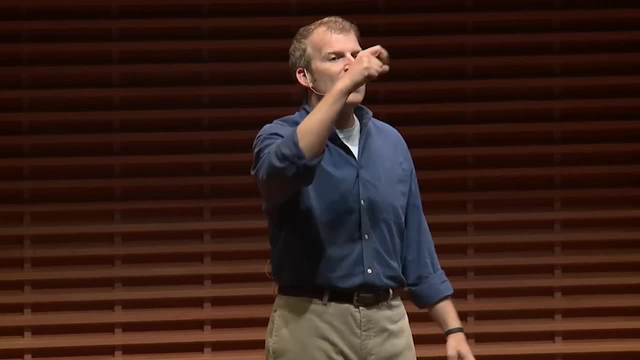 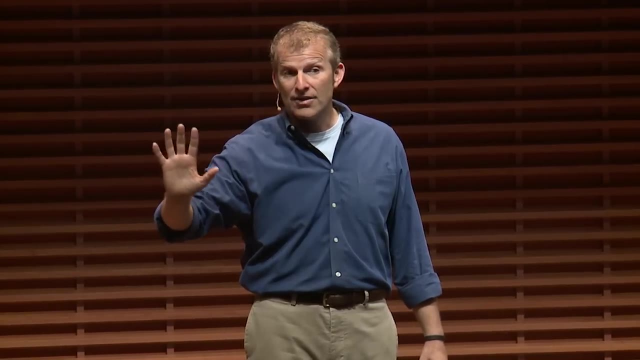 It's not a problem that we're not doing it, but maybe we'd be better off if we did So. it becomes opportunity-solution, which are the steps to achieve it. and then the benefit: Another structure which works equally well. 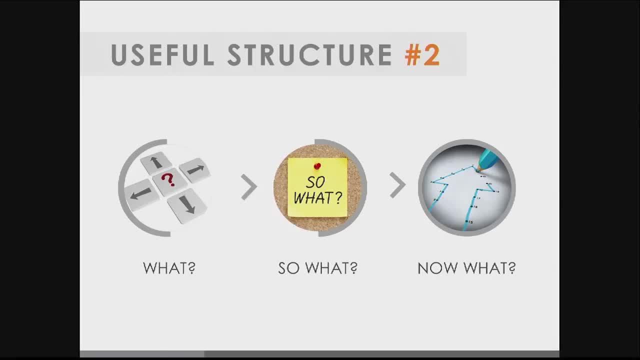 is the what? so what now? what structure? You start by talking about what it is, Then you talk about why it's important and then what the next steps are. This is a wonderful formula for answering questions, for introducing people. So if, in the moment, somebody asks me to introduce somebody, 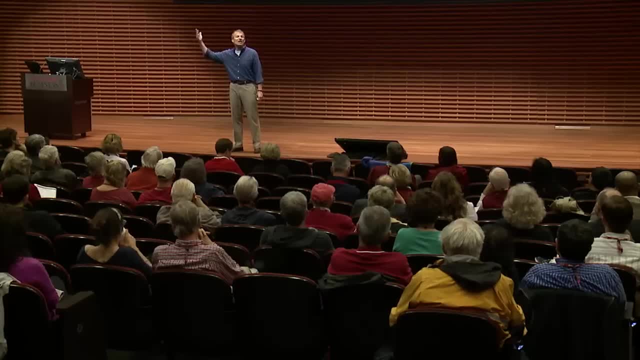 I change the what to who. I say who they are, why they're important and what we're going to do next. Maybe listen to them, maybe drink our wine, whatever right, What? so what now? what? The reality is this. 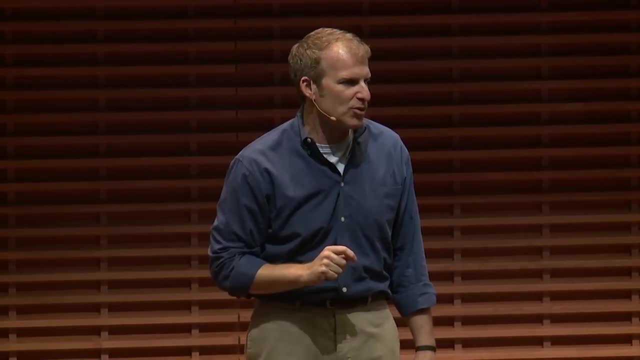 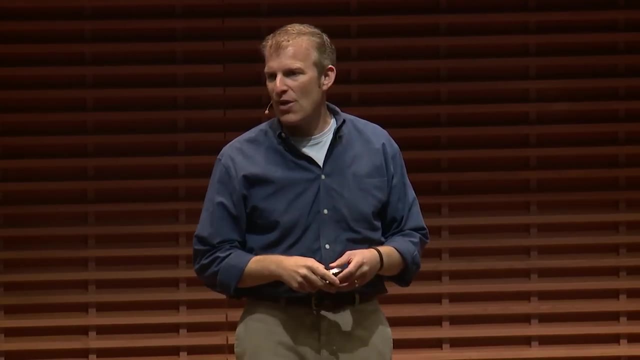 When you are in a spontaneous speaking situation, you have to do two things simultaneously. You have to figure out what to say and how to say it. These structures help you by telling you how to say it. If you can become comfortable with these structures, 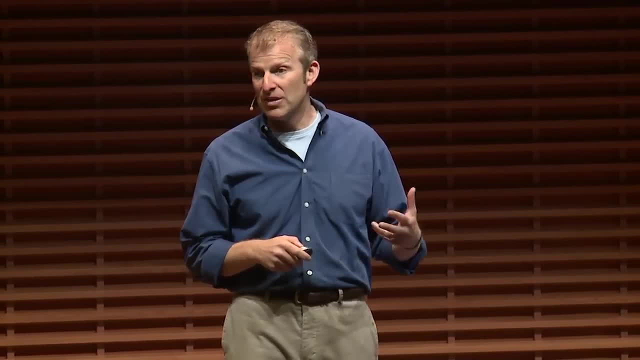 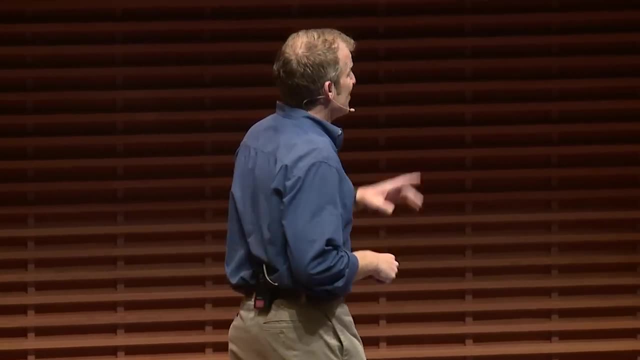 you can be in a situation where you can respond very ably to spontaneous speaking situations. We're going to practice, Because that's what we do. Here's the situation. Is everybody familiar with this child's toy? It's a slinky. 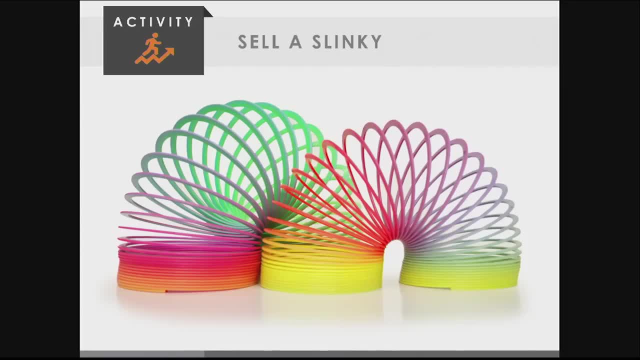 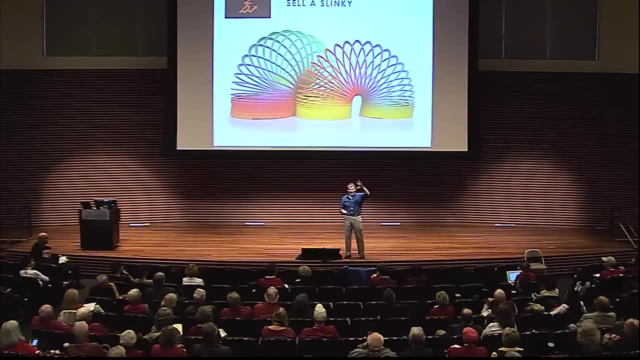 Okay, You are going to sell this slinky to your partner using either problem solution benefit or opportunity solution benefit. What does the slinky provide you? Or you could use what. so what now? what? What is it? Why is it important? 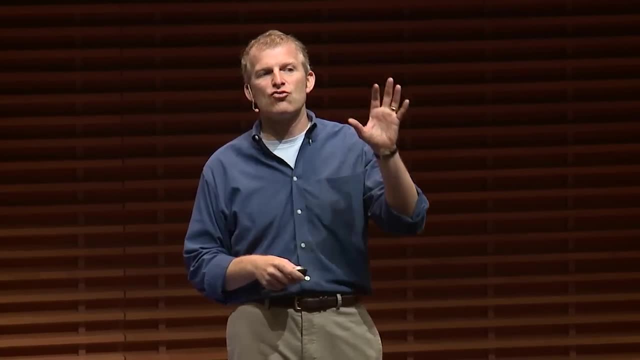 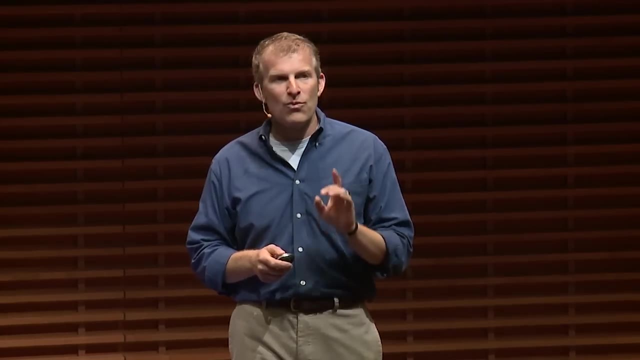 And the next steps might be to buy it. okay. So by using that structure, see how already it helps you. It helps you focus, Get with your partner And we're only going to have one partner sell to the other partner. okay. 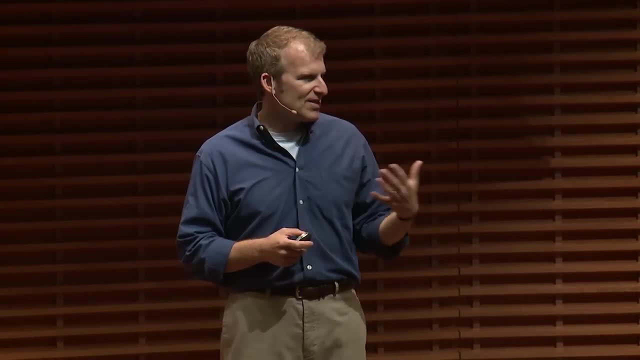 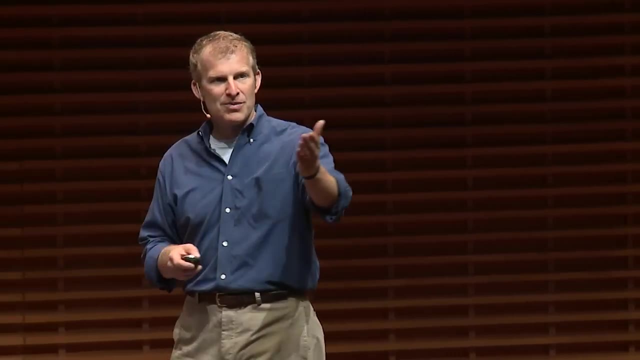 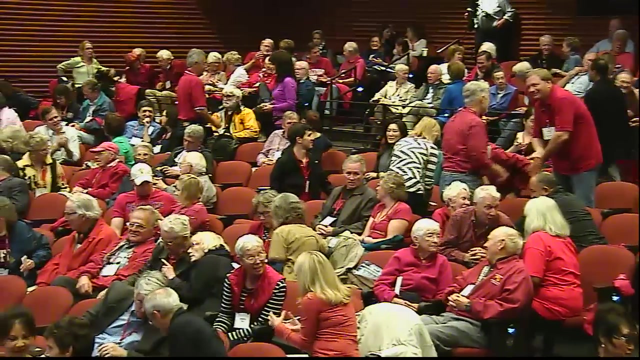 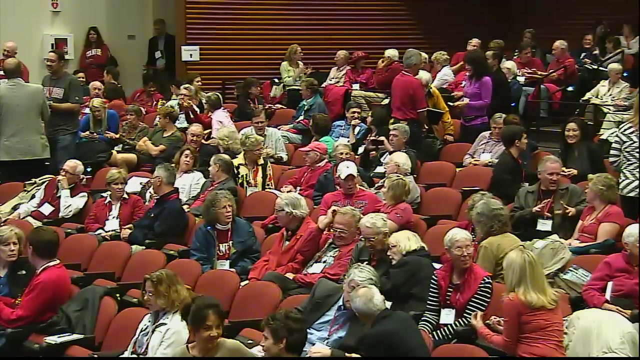 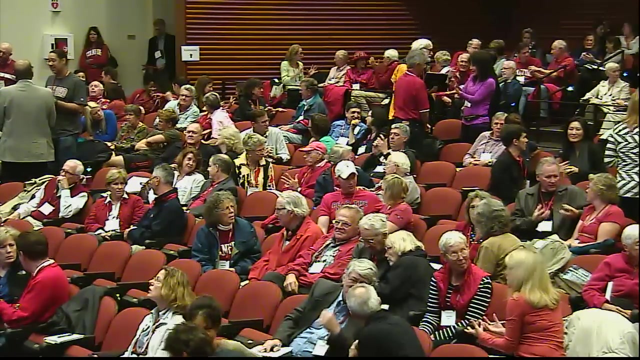 So get with your partner. One of you will volunteer to sell to the other. okay, Sell a slinky using problem solution benefit, or what. so what now? what, Please begin. So we have the handouts, but I'm also going to be doing the mic. 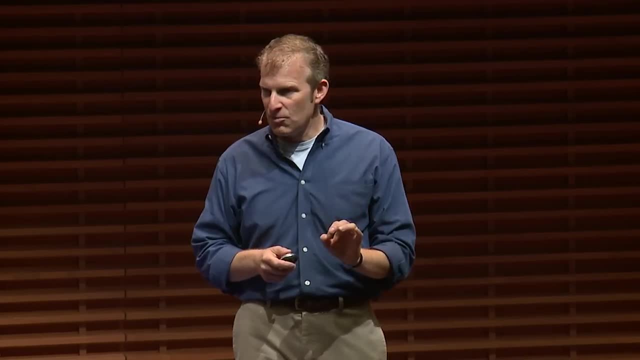 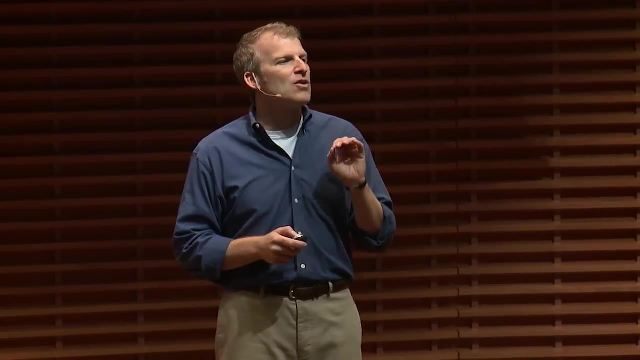 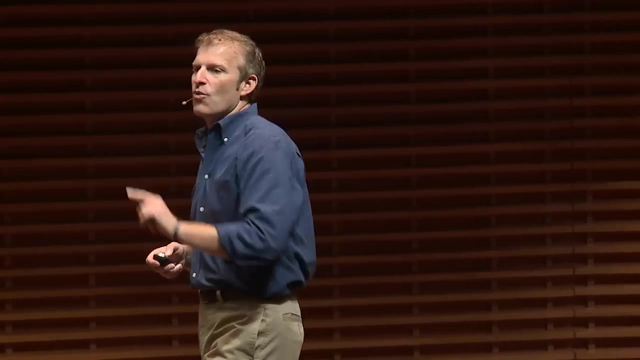 It helps you focus. Get with your partner. We're only going to have one partner sell to the other partner. Get with your partner. One of you will volunteer to sell to the other. Sell a Slinky using problem solution benefit or what. so what now? what? 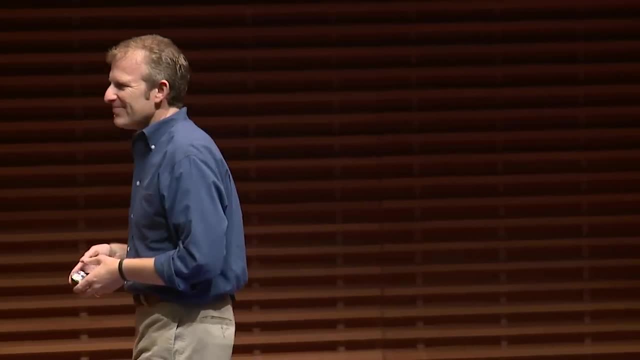 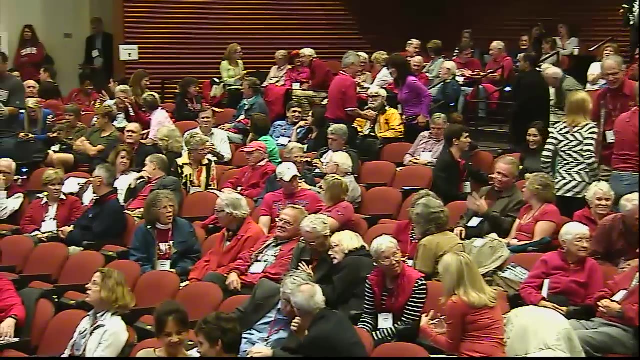 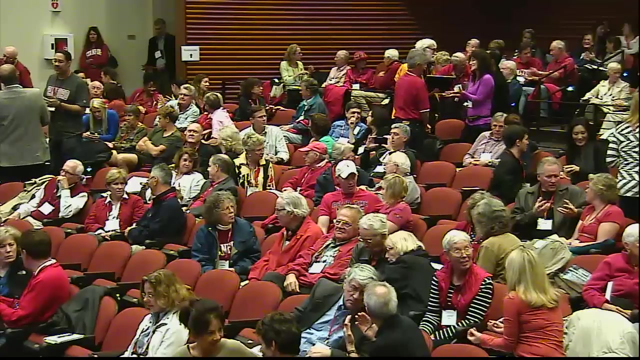 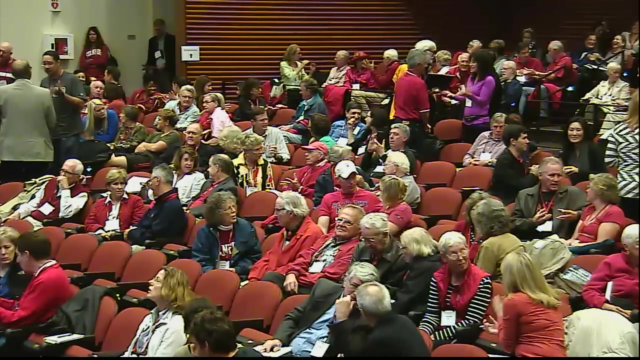 Please begin. We're going to do the hand out. I'm also going to be doing the mic When I debrief this. you can go ahead and pass them out. Does that make sense? After Q&A: No, no, After this activity. 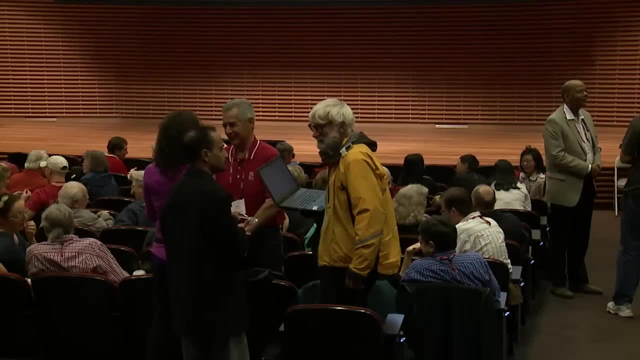 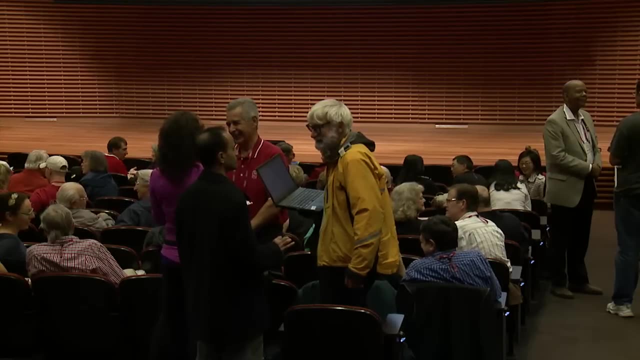 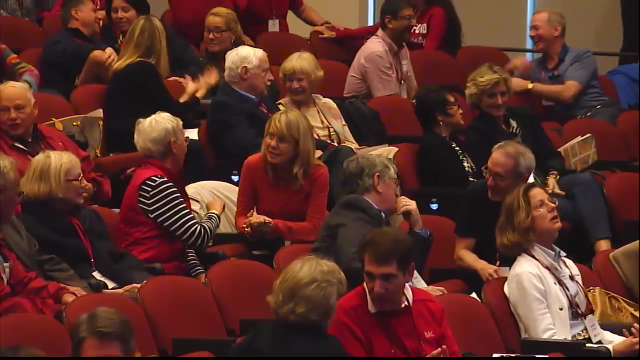 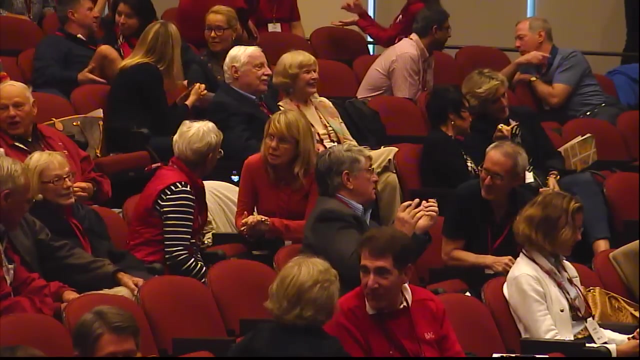 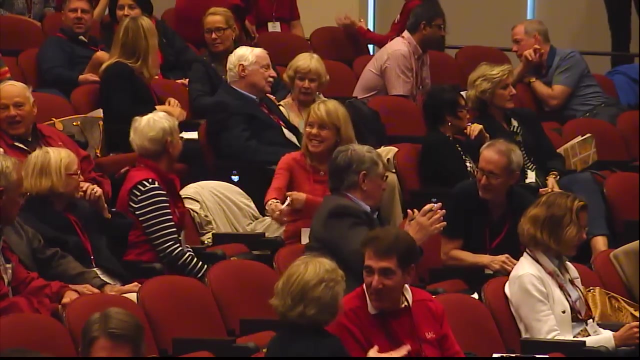 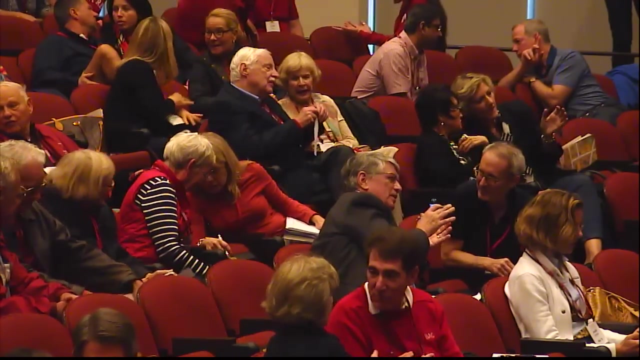 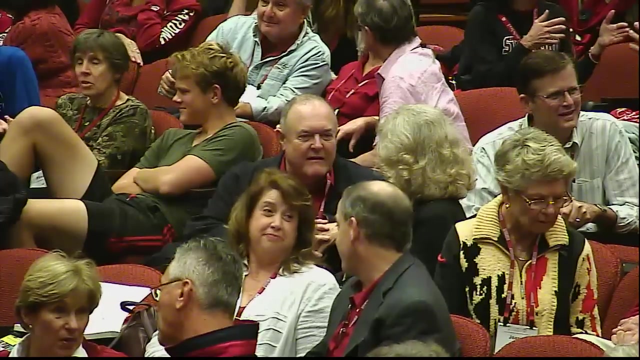 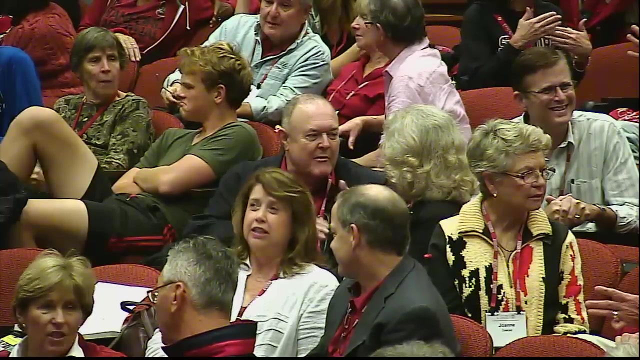 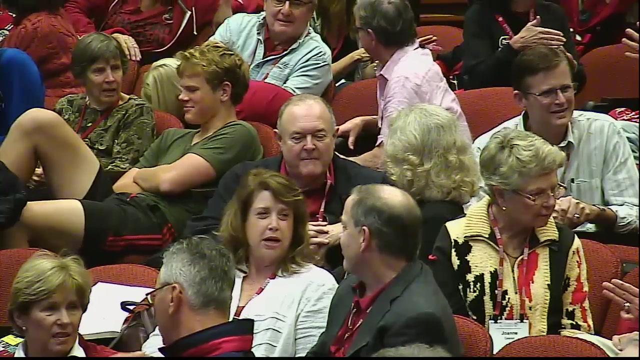 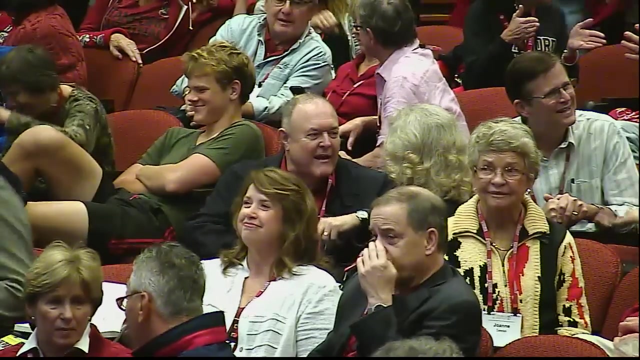 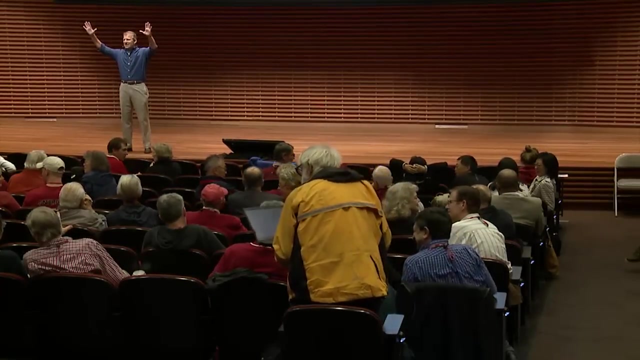 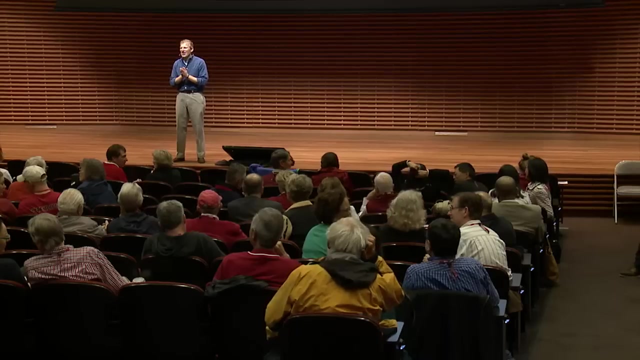 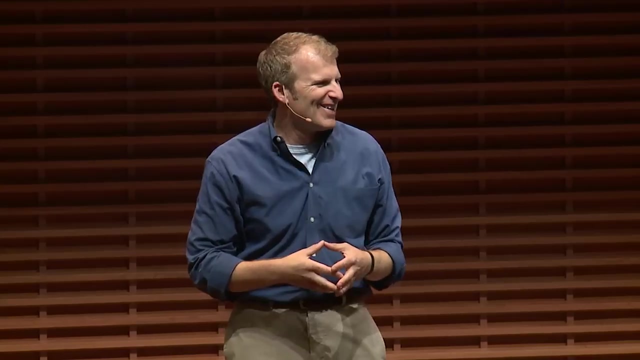 Okay, After that we'll do Q&A. All right, 30 more seconds please. Excellent, Let's all close the deal. seal the deal. I have never seen more people in one place doing this at the same time. I love it. 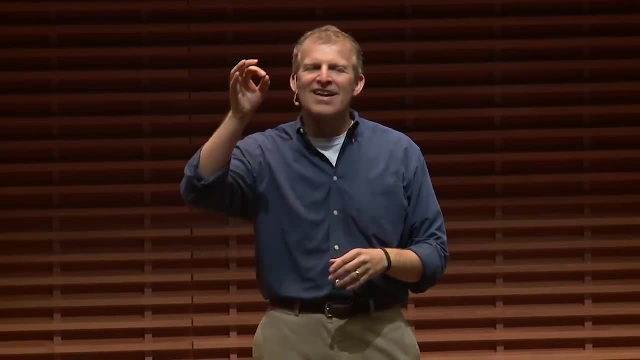 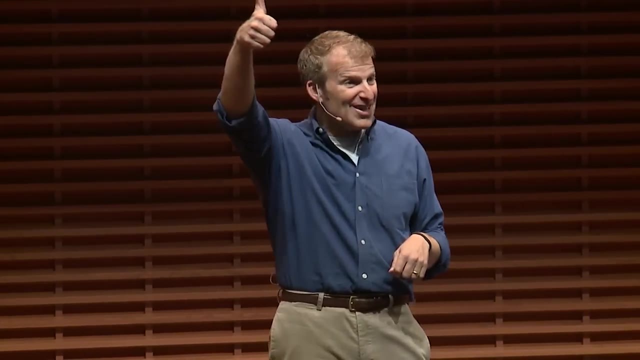 I teach people to gesture, and gesture big. It's great, I love it. So if you were the recipient of the sales pitch, thumbs up. Did they do a good job? Did they use the structure? Awesome. I'm recruiting you all for my next business as my sales people. 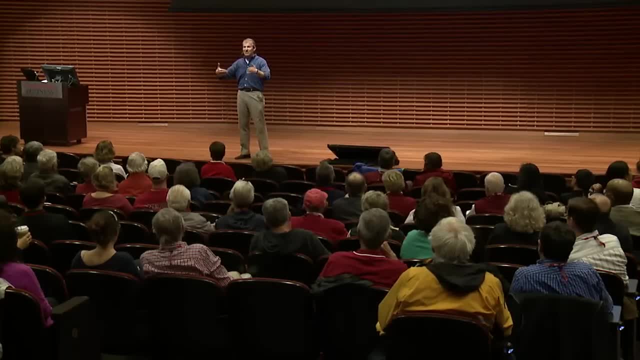 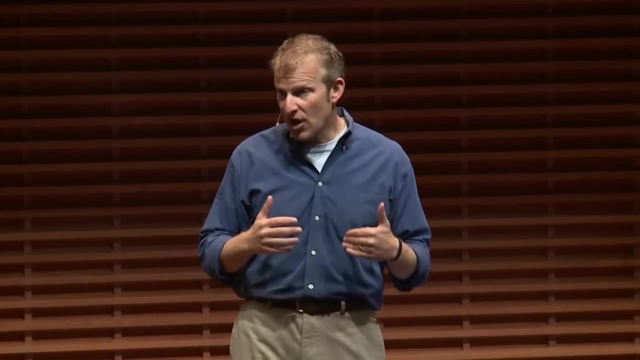 Please try to ignore this, but, as we're speaking, the handout I told you about is coming around. On the back of that handout, you are going to see a list of structures: the two we talked about and several others that can help you in spontaneous speaking situations. 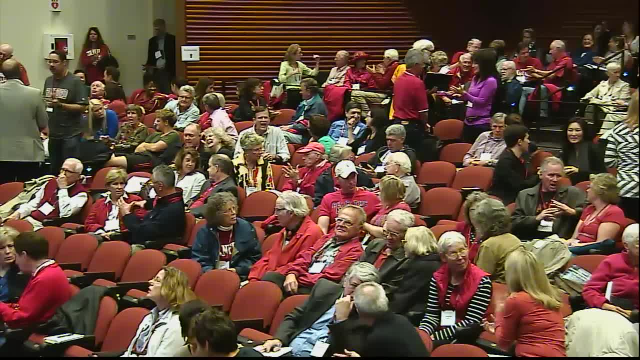 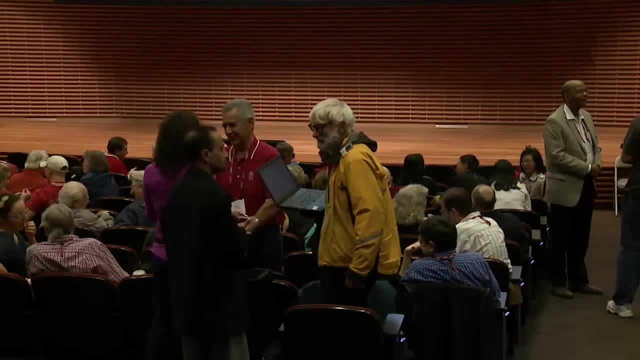 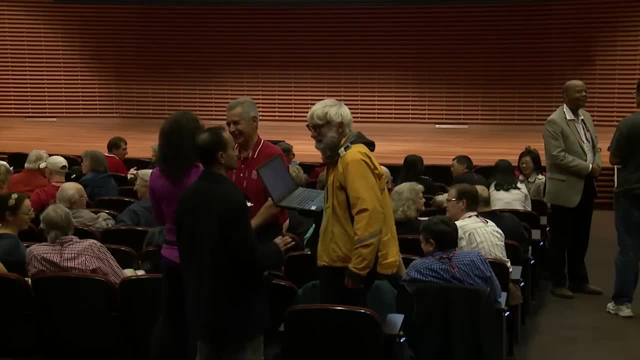 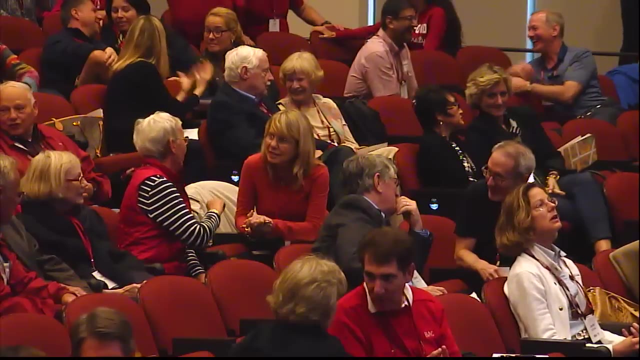 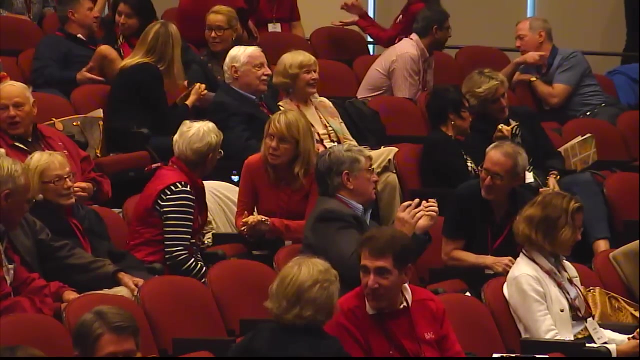 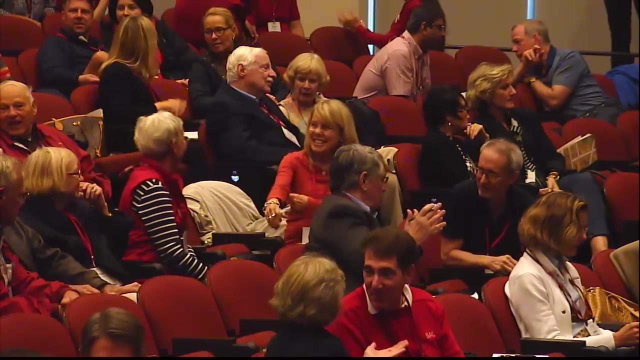 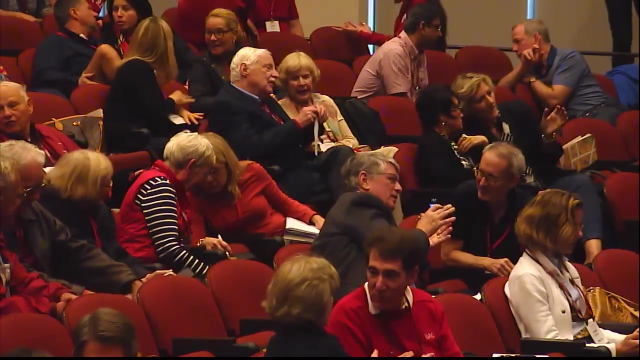 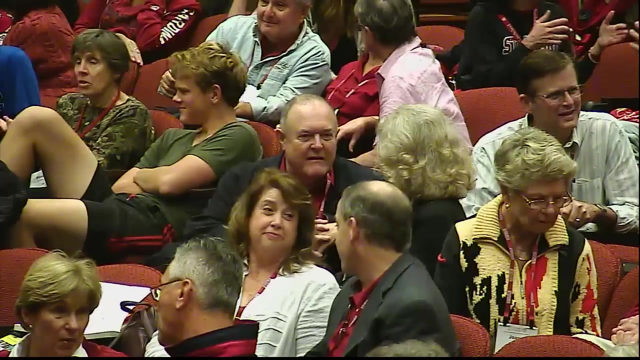 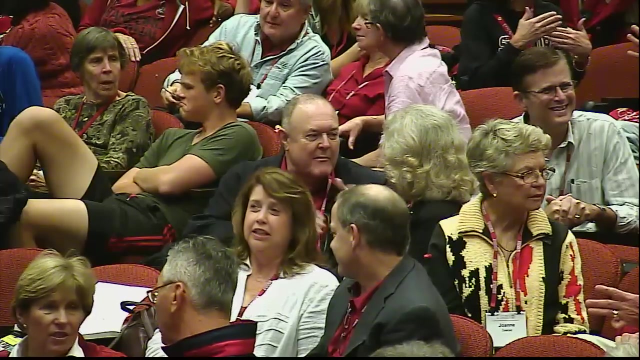 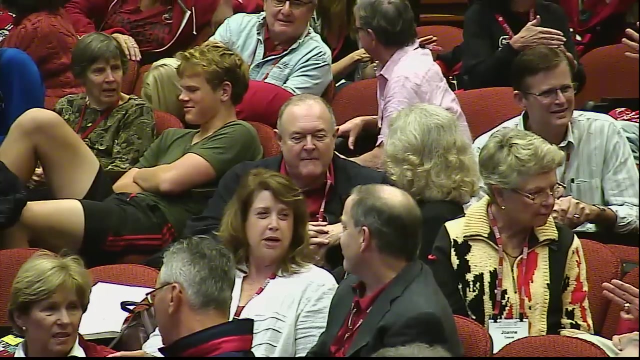 So when I debrief this, you can go ahead and pass them out. Does that make sense? After Q&A: No, no, after this activity: Okay, and then after that we'll do Q&A. Correct, Thank you. 30 more seconds, please. 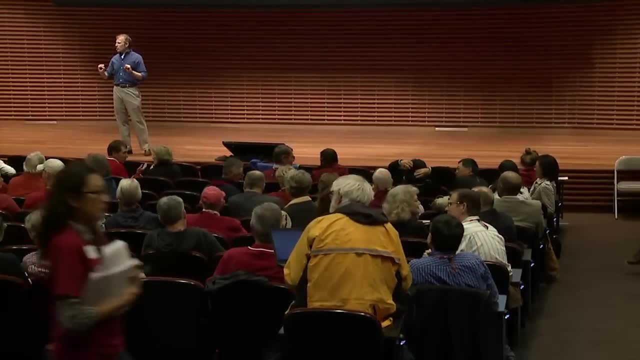 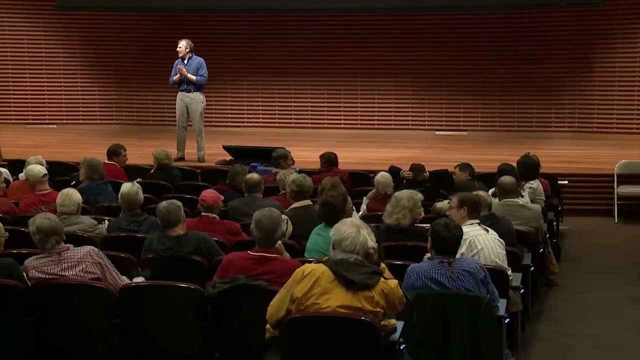 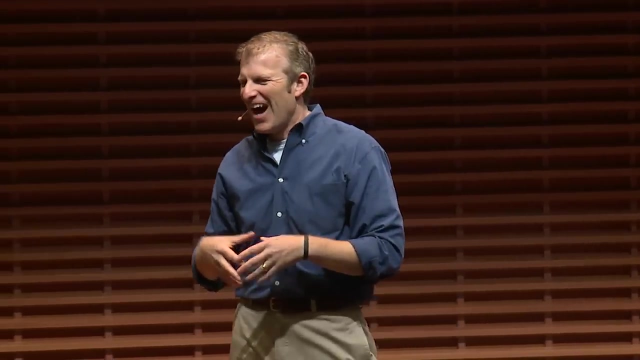 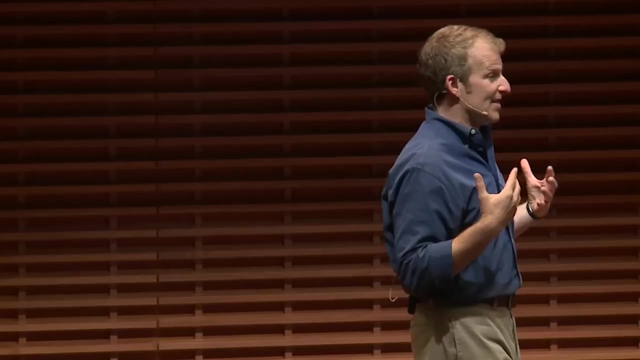 Excellent. Let's all close the deal, seal the deal. I have never seen more people in one place doing this at the same time. I love it. I teach people to gesture and gesture big. It's great, I love it. So if you were the recipient of the sales pitch, thumbs up. 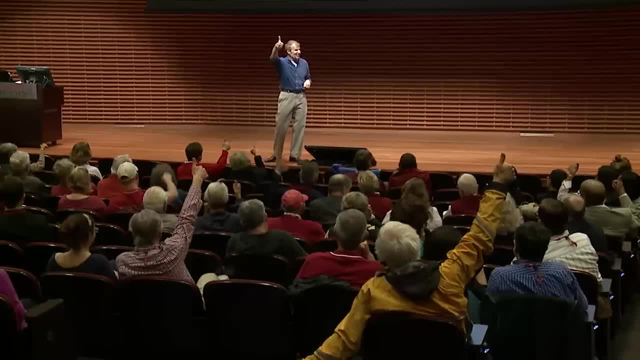 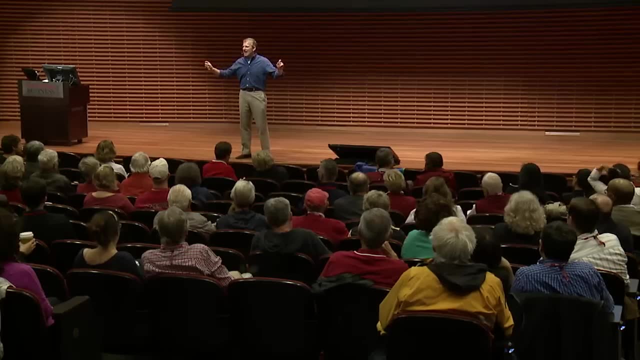 Did they do a good job? Did they use the structure? Awesome. I'm recruiting you all for my next business as my salespeople. Please try to ignore this, but as we're speaking, the handout I told you about is coming around. 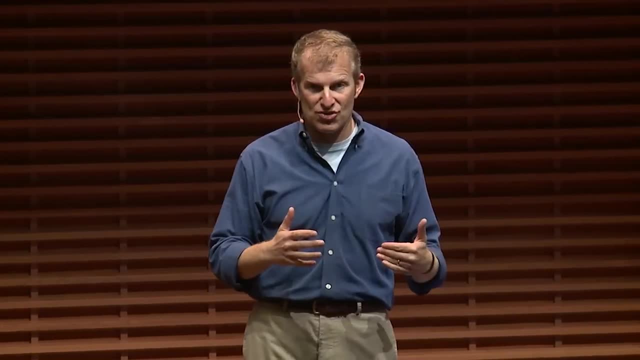 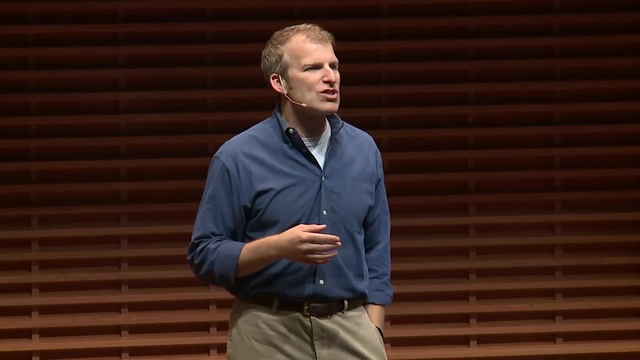 On the back of that handout you are going to see a list of structures- the two we talked about and several others that can help you in spontaneous speaking situations. These structures help because they help you understand how you're going to say what you. 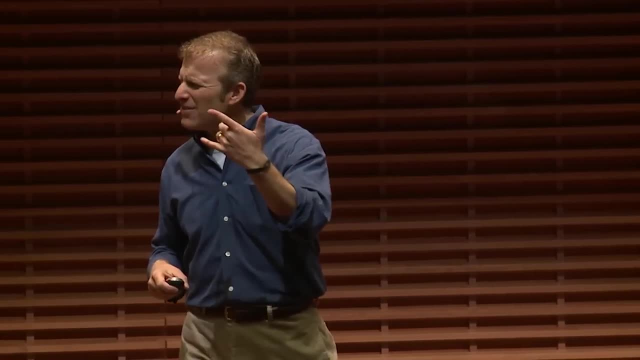 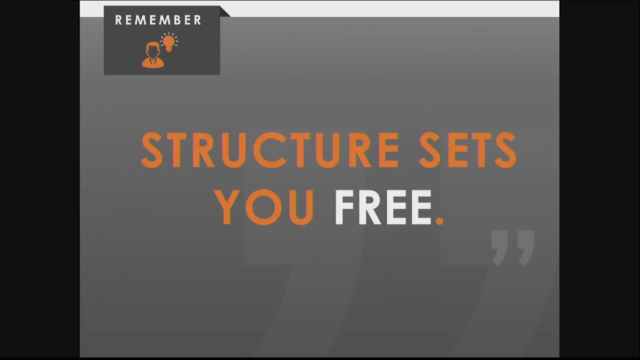 say: Structure sets you free- And I know that's kind of ironic But it's true. If you have that structure, then you're free to think about what it is you're going to say. It reduces the cognitive load of figuring out what you're saying and how you're going. 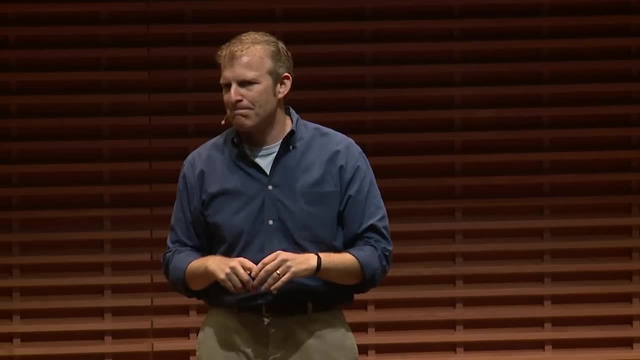 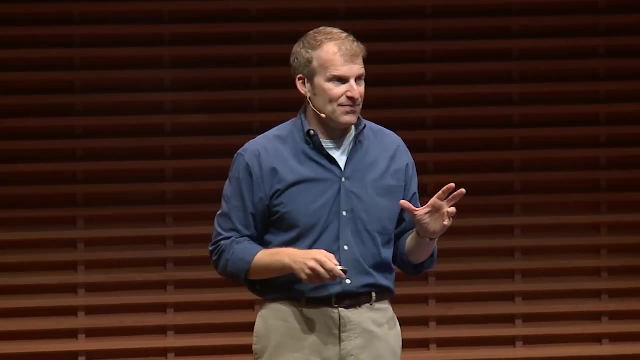 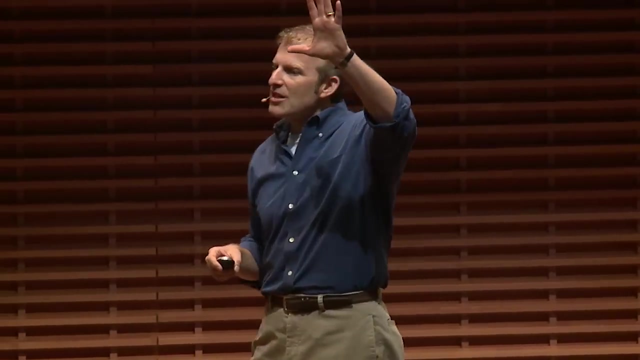 to say it, All of this is on that handout. So what does this all mean? It means that we have, within our ability, the tools and the approaches to help us in spontaneous speaking situations. The very first thing we have to do is manage our anxiety. 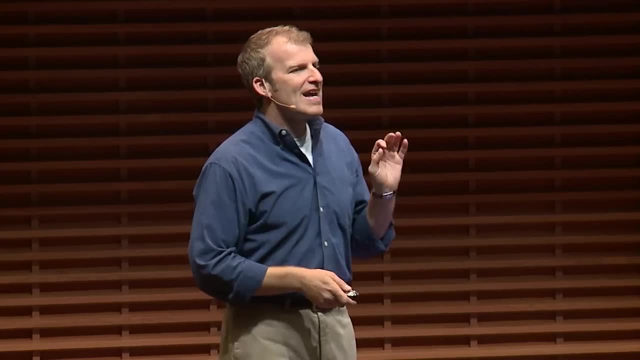 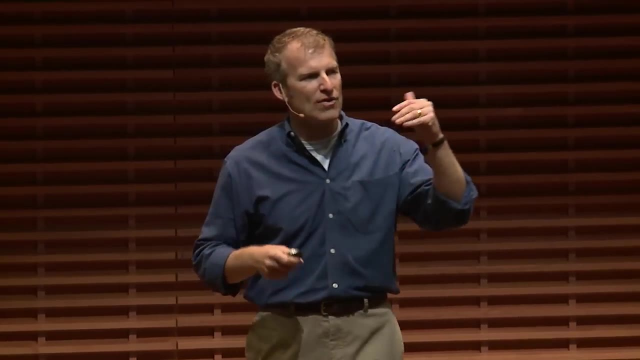 These structures help because they help you understand how you're going to say what you say. Structure sets you free- and I know that's kind of ironic, but it's true. If you have that structure, then you're free to think about what it is you're going to say. 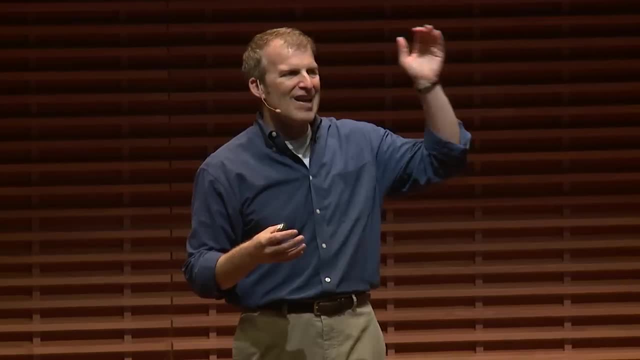 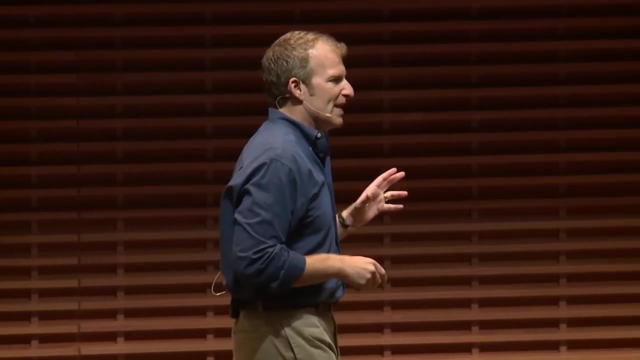 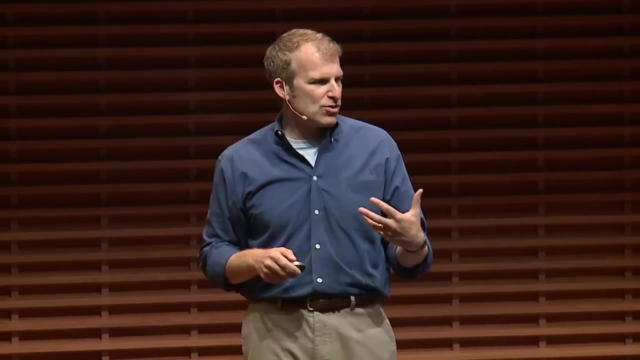 It reduces the cognitive load of figuring out what you're saying and how you're going to say it. All of this is on that handout, Okay. So what does this all mean? It means that we have, within our ability, the tools and the approaches to help us in spontaneous speaking situations. 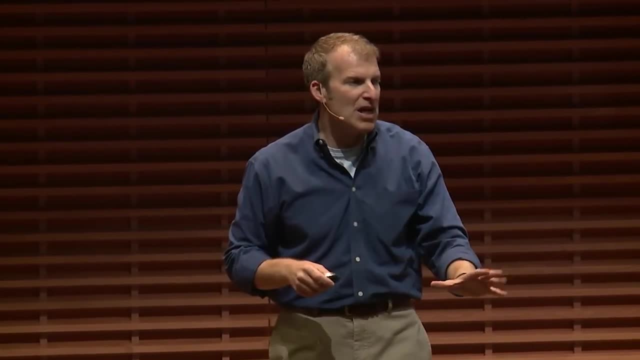 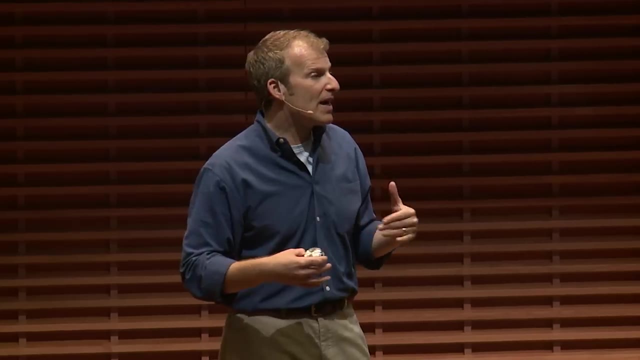 The very first thing we have to do is manage our anxiety, because you can't be an effective speaker if you don't have your anxiety under control, And we talked about how you can do that by greeting your anxiety, reframing as a conversation and being in the present moment. 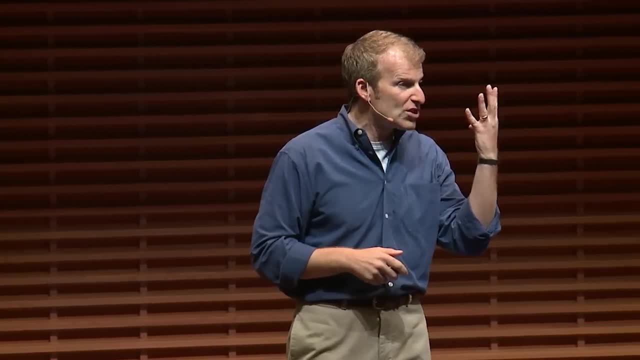 Once you do that, you need to practice a series of four steps that will help you speak spontaneously. First, you need to be able to communicate. Second, you need to be able to communicate. Third, you need to be able to communicate. 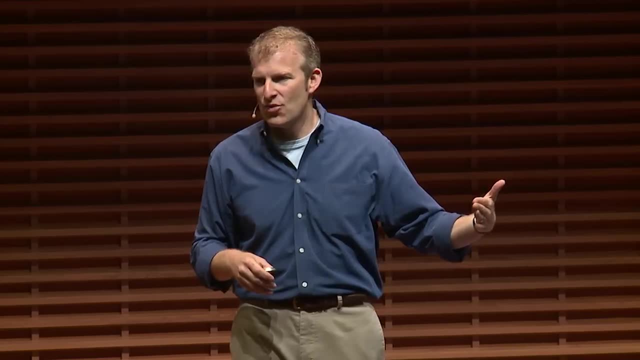 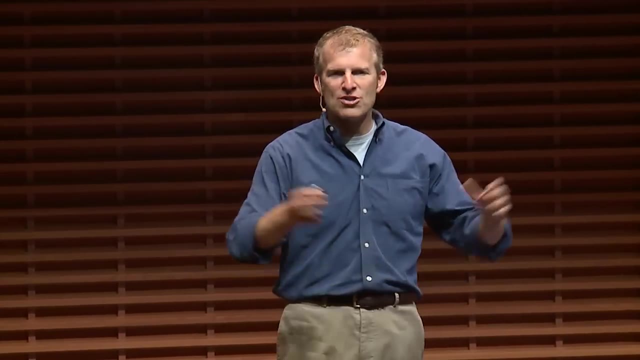 First, you get out of your own way. I would love it if all of you, on your way from here to the football game, point at things and call them the wrong name. It'll be fun. If most of us do it, then it won't be weird. 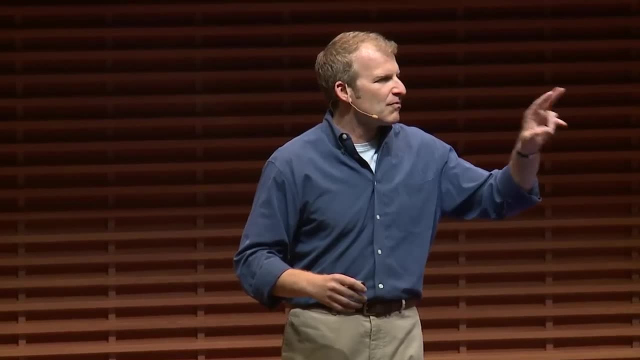 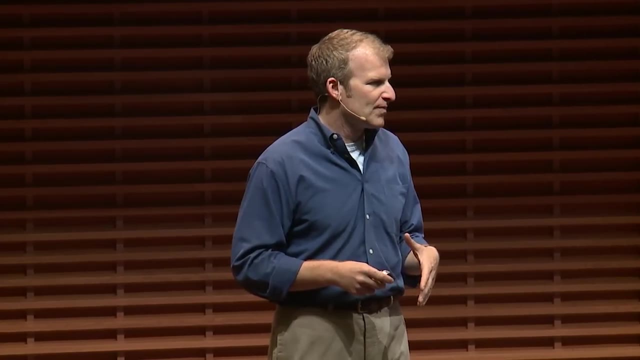 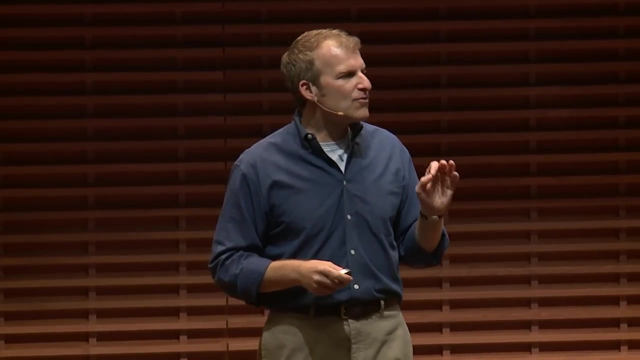 If only one in two of us do it, it'll be weird. Second, give gifts. By that I mean see your interactions as ones of opportunity, not challenges. Third, take the time to listen, Listen And then finally use structures. 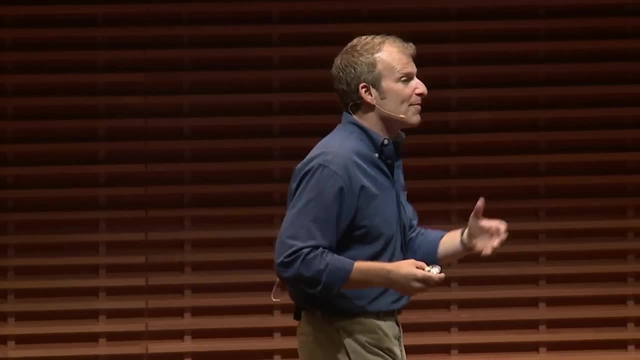 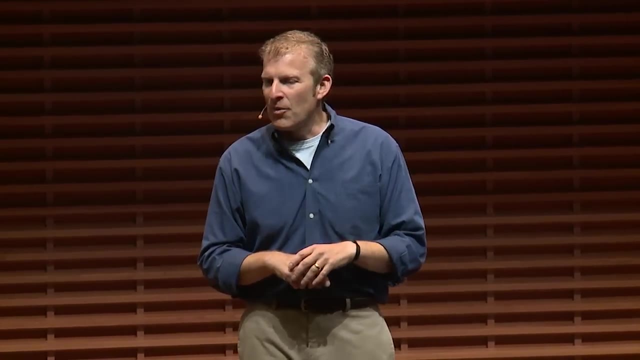 And you have to practice these structures. I practice these structures on my kids. I have two kids. When they ask me questions, I usually answer them in what so? what? now what? They don't know it. But when they go over to their friends' houses and 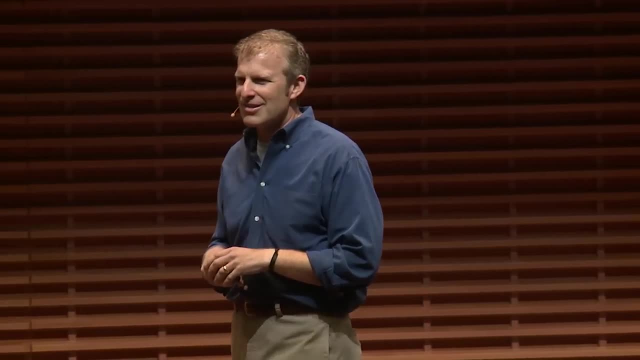 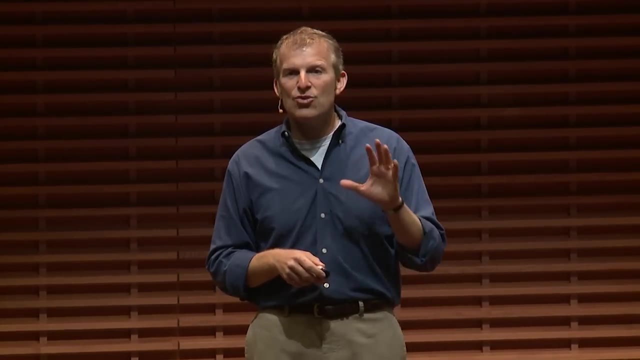 they see their friends ask their dad's questions. they don't get what. so what now? what? So you know you have to practice. The more you practice, the more comfortable you will become. Ultimately, you have the opportunity before you to become more compelling. 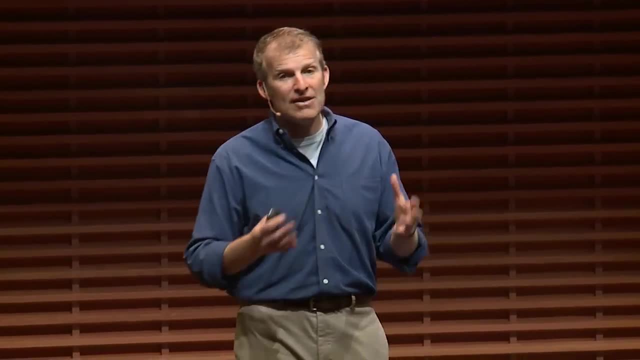 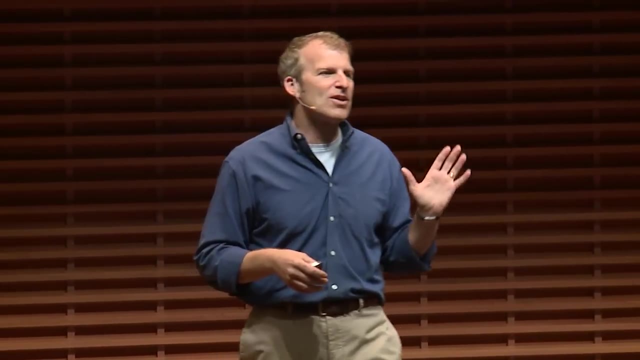 more confident, more connected as a speaker If you leverage these techniques, If you're interested in learning more, this is where I do a little plug. Okay, I've written a book. many of the MBA students who take the strategic communication classes here that I and others teach read it. 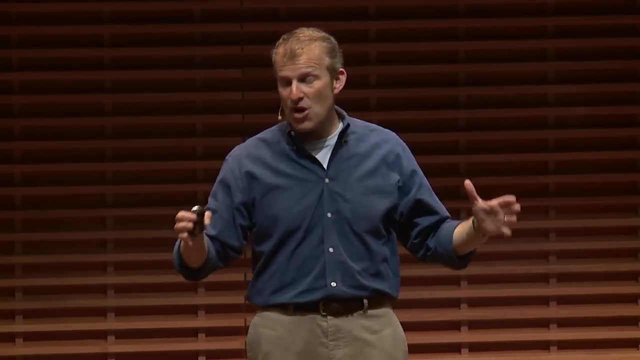 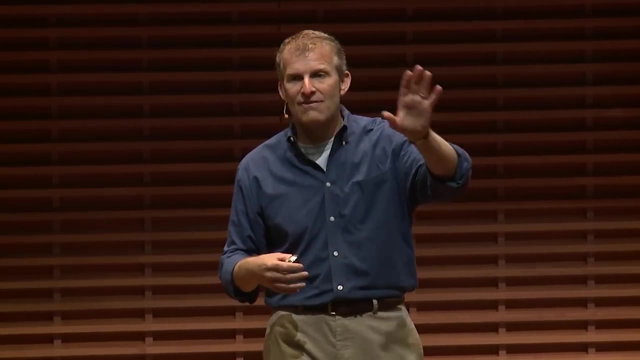 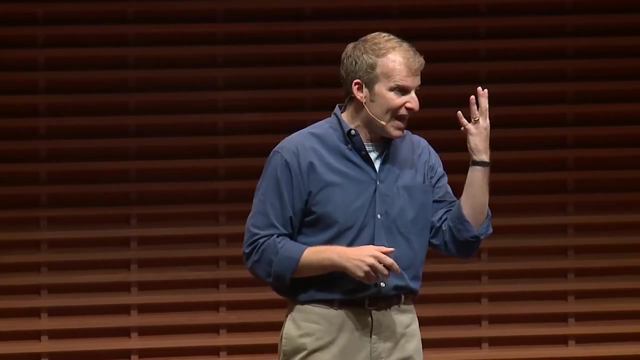 Okay, So you can't be an effective speaker if you don't have your anxiety under control, And we talked about how you can do that by greeting your anxiety, reframing as a conversation and being in the present moment. Once you do that, you need to practice a series of four steps that will help you speak spontaneously. 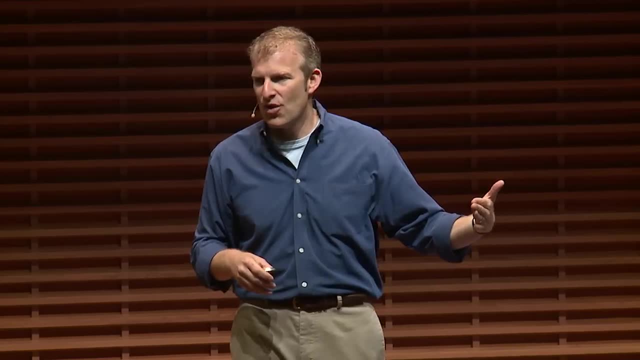 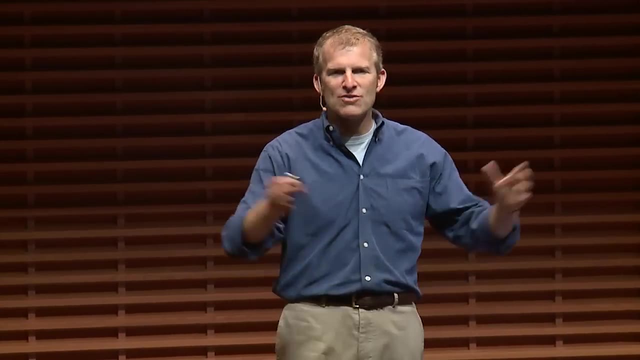 First, you get out of your own way. I would love it if all of you, on your way from here to the football game, pointed things and called them the wrong name. It'll be fun. If most of us do it, then it won't be weird. 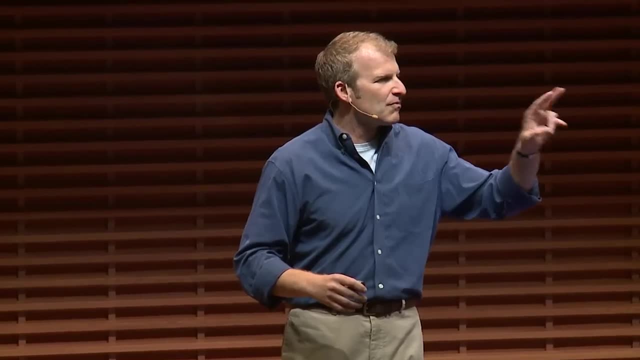 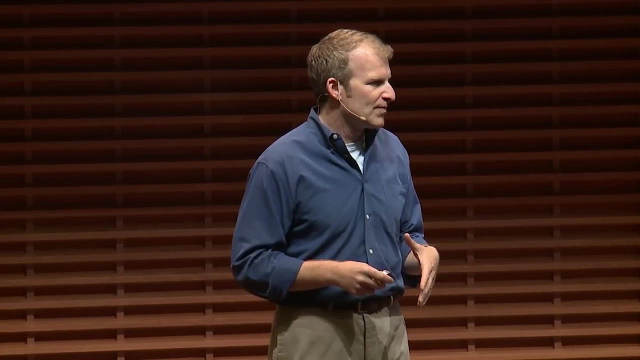 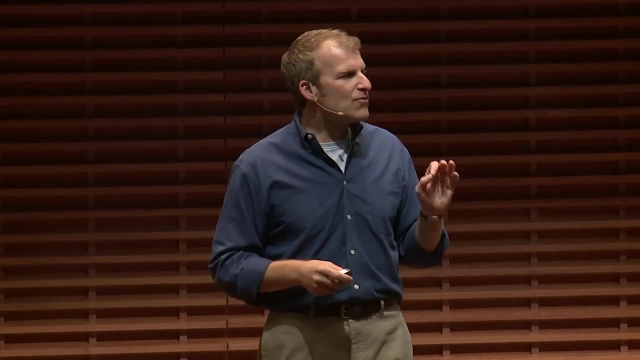 If only one or two of us do it, it'll be weird. Second, give gifts. By that I mean see your interactions as ones of opportunity, not challenges. Third, take the time to listen, Listen And then finally use structures. 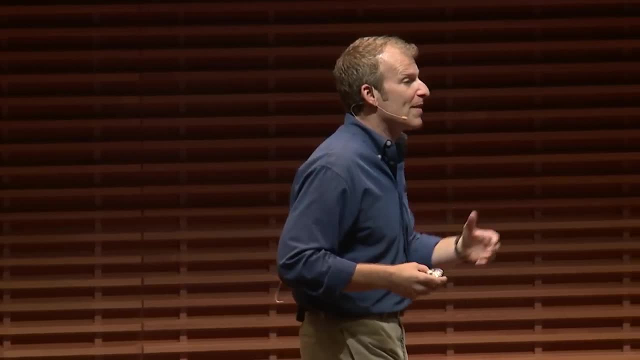 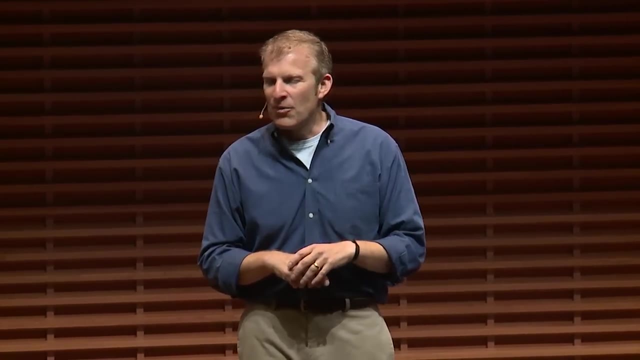 And you have to practice these structures. I practice these structures on my kids. I have two kids. When they ask me questions, I usually answer them in what so? what? now? what? Okay, They don't know it. But when they go over to their friends' houses and they see their friends ask their dad's, 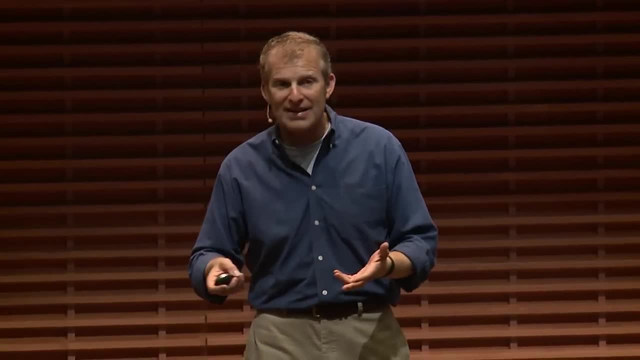 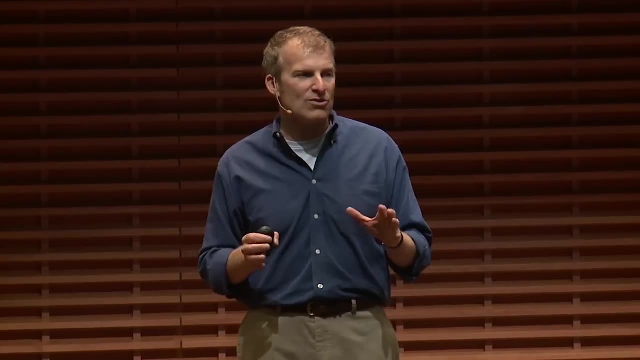 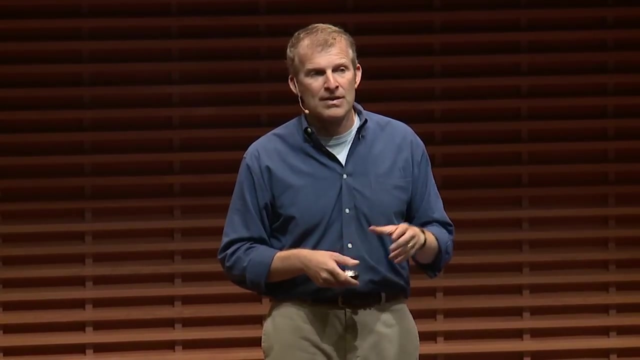 questions. they don't get. what so what now? what So? you have to practice. The more you practice, the more comfortable you will become. Ultimately, you have the opportunity before you to become more compelling, more confident, more connected as a speaker if you leverage these techniques. 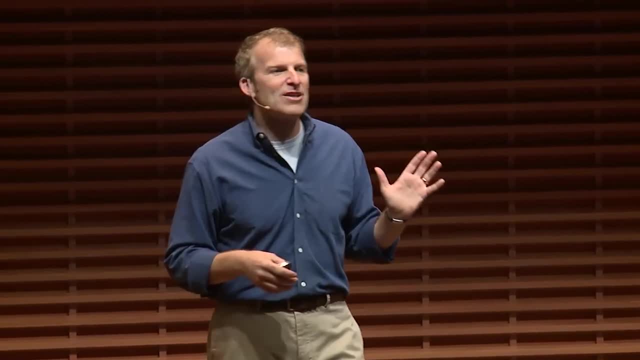 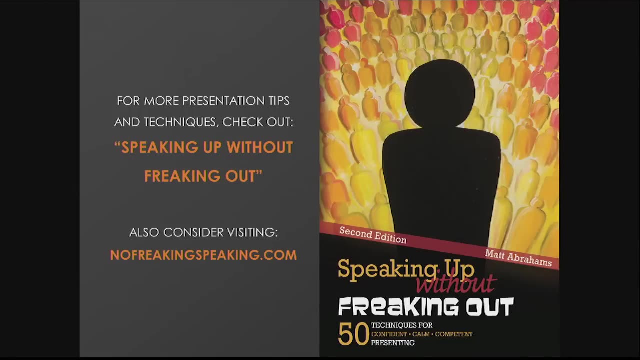 If you're interested in learning more. this is where I do a little plug. Okay, I've written a book. Many of the MBA students who take the strategic communication course. they're going to be interested. It's called Speaking Up Without Freaking Out. 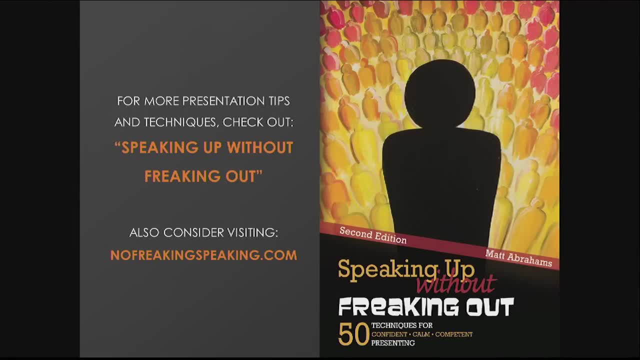 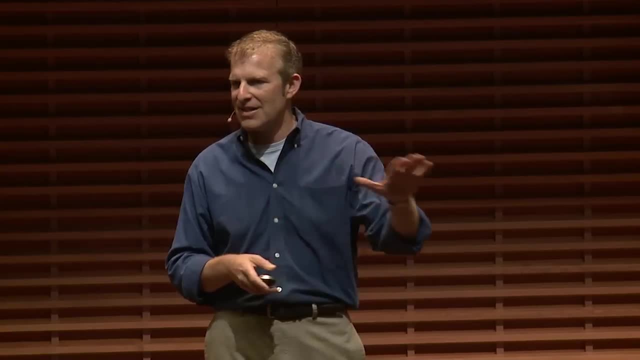 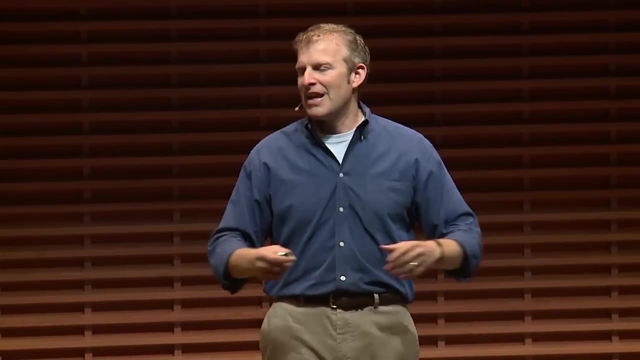 More importantly, there's a website here that I curate called No Freaking Speaking, and it has lots of information that I've written and others have written, about how to become more effective at speaking. So that's the end of my plug. What I'd really like to do is enter into a spontaneous speaking situation with you. 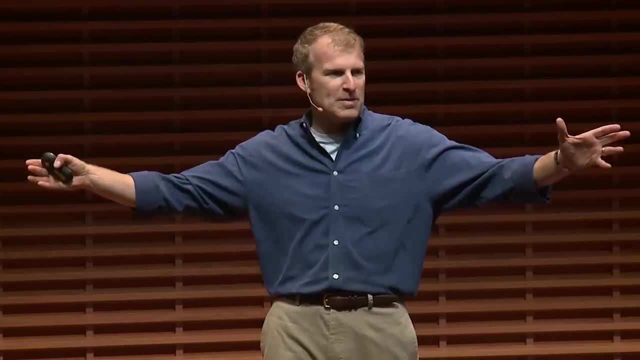 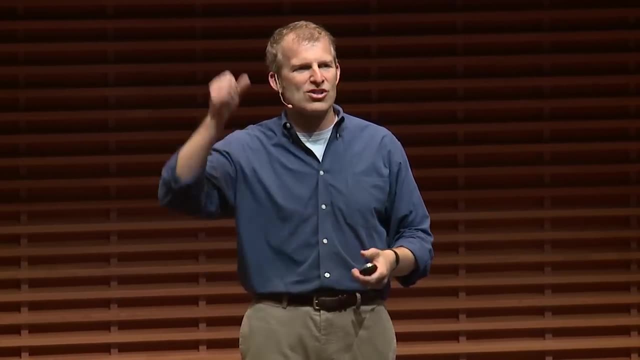 And I would love to entertain any questions that you have. There are two people who are running around with microphones, So some of us who remember We're going to do a little bit of that. If you have a question, the microphone will come and I'm happy to answer it. 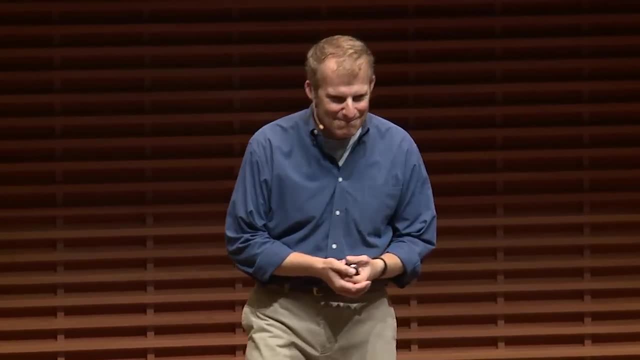 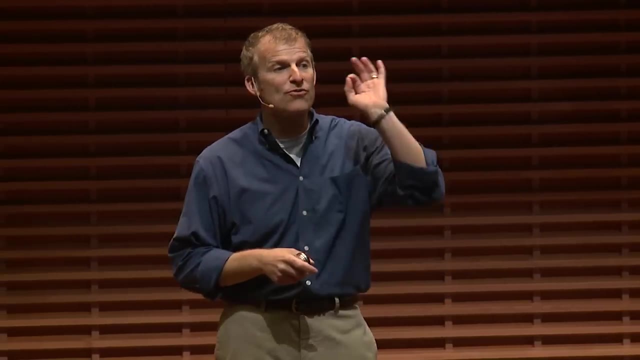 I think if you Is it on, Yeah, Yeah, We can hear you. Great, Can you talk about hostile situations, Hostile situations? Yes, So when you find yourself in a challenging situation first, it should not become a surprise. 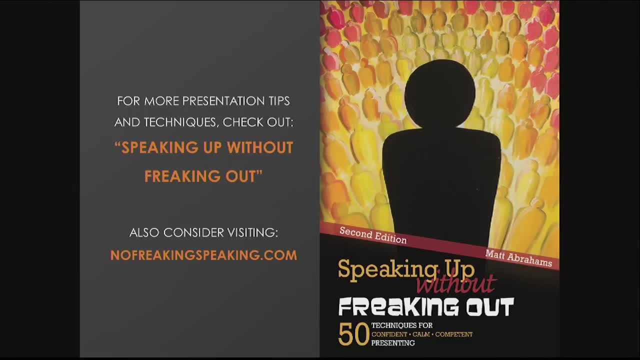 It's called Speaking Up Without Freaking Out. More importantly, there's a website here that I curate called No Freaking Speaking, And it has lots of information that I've written and others have written about how to become more effective at speaking. 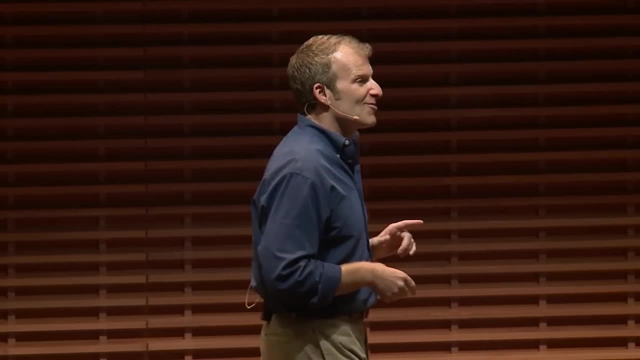 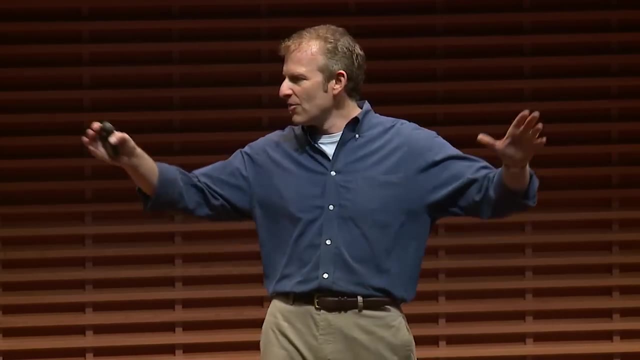 So that's. that's the end of my plug. What I'd really like to do is enter into a spontaneous speaking situation with you, And I would love to entertain any questions that you have. There are two people who are running around with microphones, so 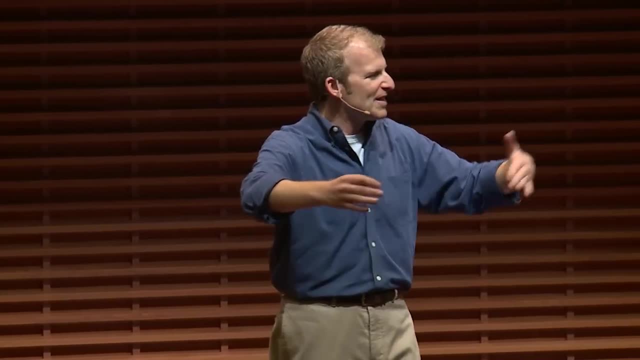 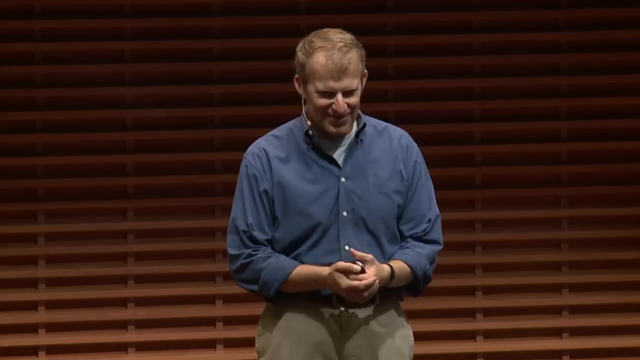 some of us who remember the Phil Donahue show. We're going to do a little bit of that. If you have a question, the microphone will come and I'm happy to answer it. There you go, I think. if you Is it on. 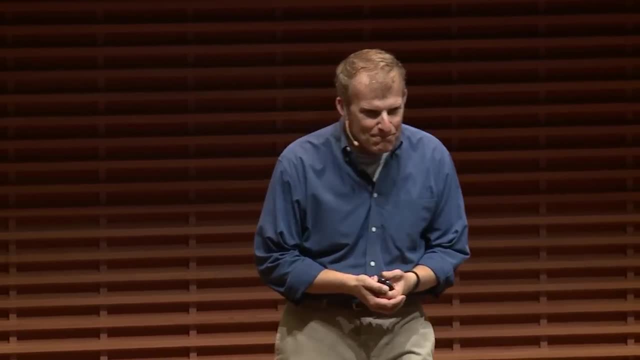 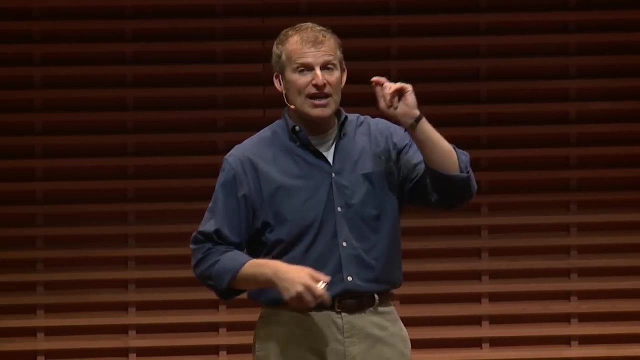 Yeah, yeah, We can hear you Great. Can you talk about hostile situations, Hostile situations, yes. So when you find yourself in a challenging situation, first, it should not become a surprise to you. It should not be a surprise. 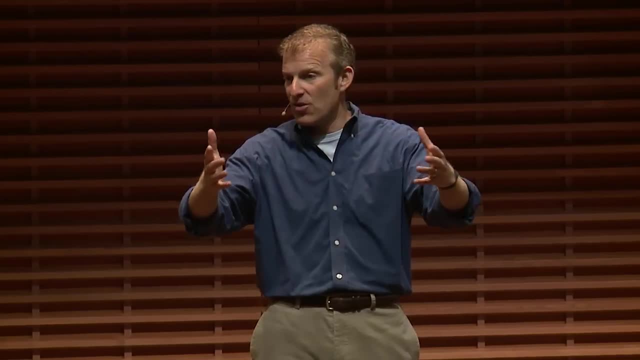 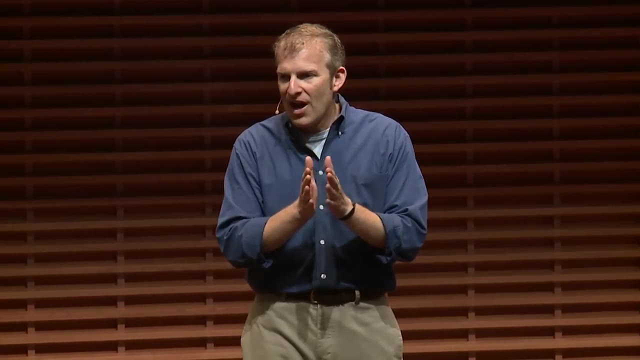 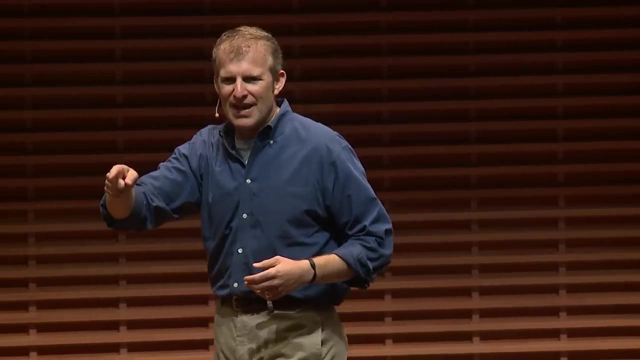 Before you ever speak you should think about what is the environment going to be like. so it shouldn't surprise you that there might be some challenges in the room. When there are hostile situations that arise, you have to acknowledge it. So if somebody says that's a ridiculous idea, why did you come up with that? 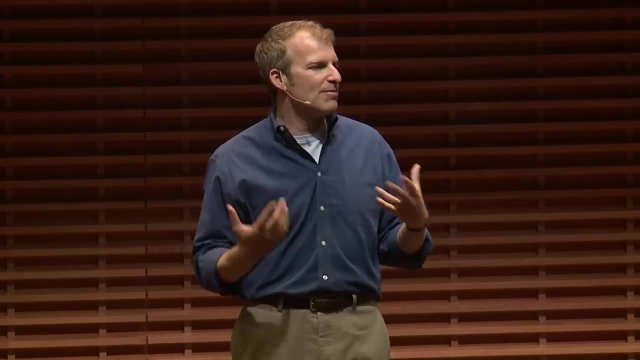 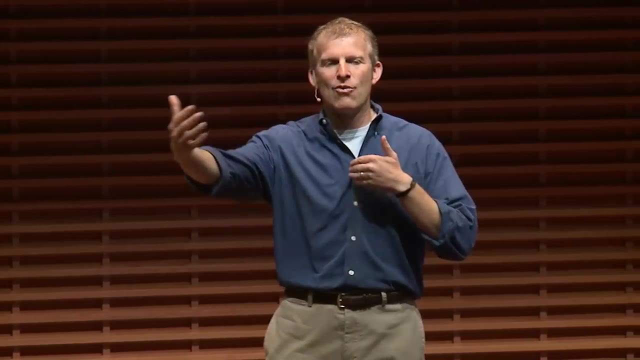 To simply say so. the idea I came up with was right: acknowledge the emotion. I recommend not naming the emotion okay, So you sound really angry. the person says I'm not angry, I'm frustrated. Now we're arguing over their mental state. right emotional state. 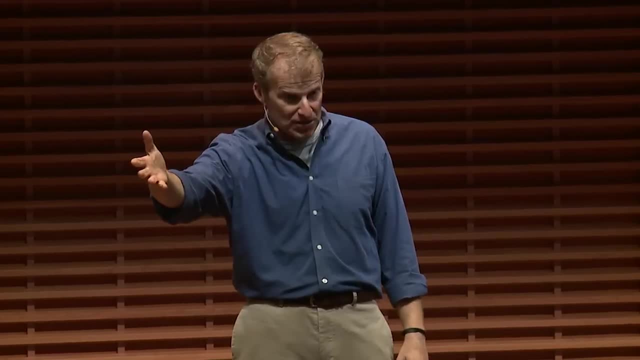 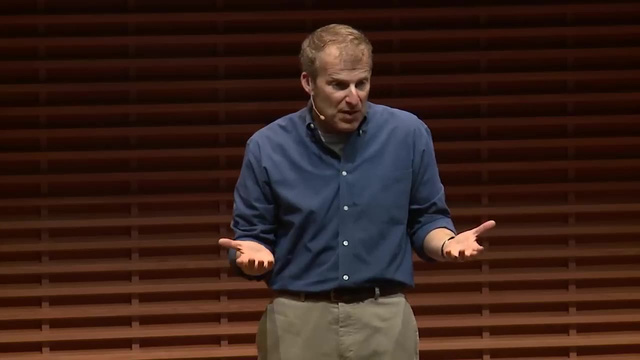 So I say something like: I hear you have a lot of passion on this issue, or I hear there's great concern from you, so you acknowledge the emotion, because otherwise it sits in the room And then reframe or respond the way that makes sense. 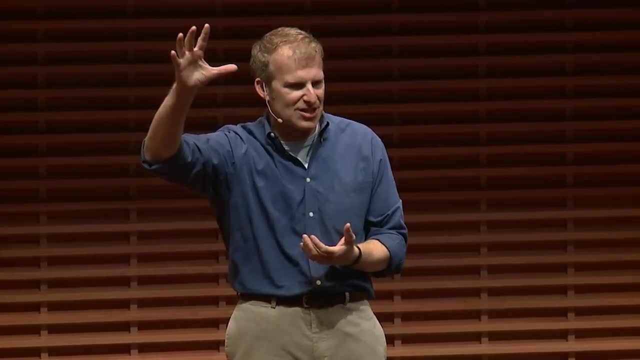 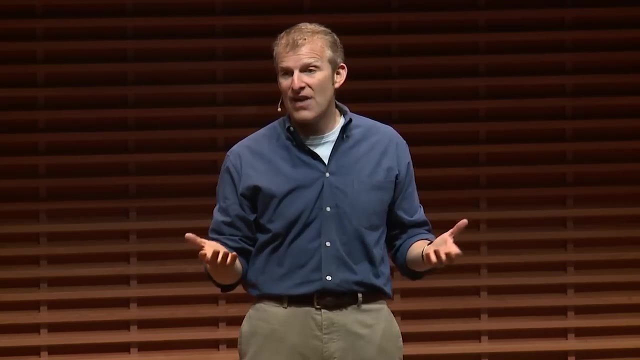 So if somebody raises their hand and says your product is ridiculously priced, why do you charge so much? I might say I hear great concern And what you're really asking about is the value of our product, And I would give my value proposition. and then I would come back and say and: 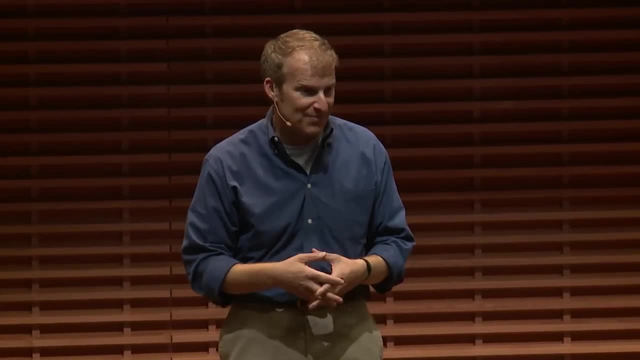 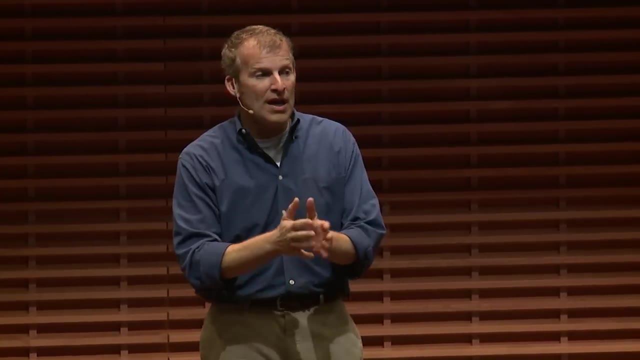 because of the value we provide, we believe it's priced fairly. So you answer the question about price, but you reframe it in a way that you feel more comfortable answering it. So the way to do this is to practice all the skills we just talked about. 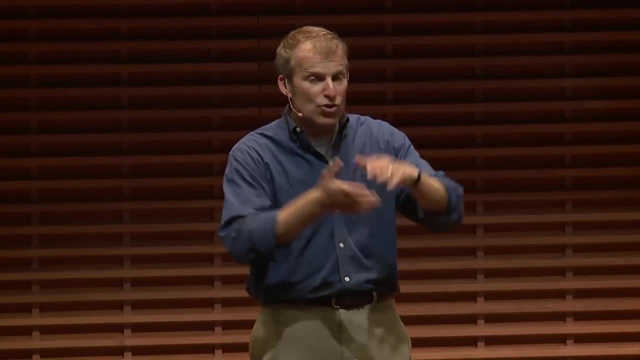 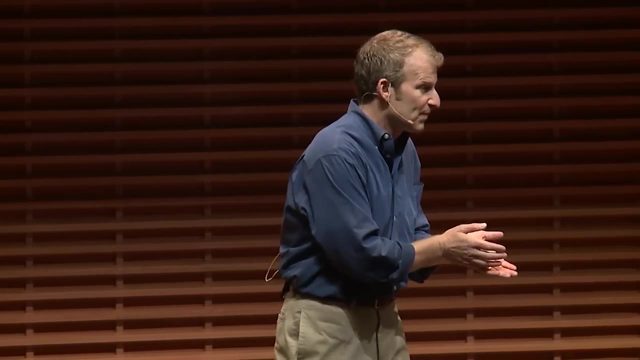 to you. It should not be a surprise. Before you ever speak, you should think about what is the environment going to be like. So it shouldn't surprise you. It shouldn't surprise you that there might be some challenges in the room When there are hostile situations that arise. you have to acknowledge it. 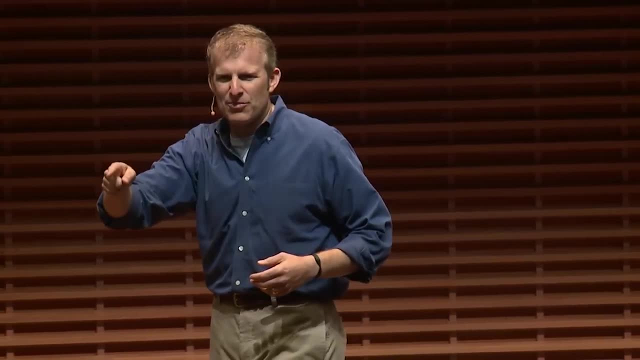 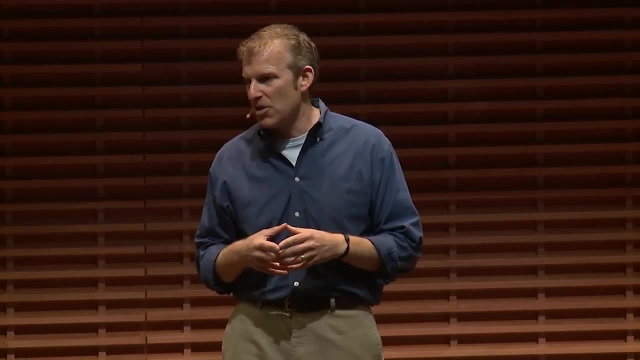 So if somebody says that's a ridiculous idea, Why did you come up with that? To simply say so. the idea I came up with was acknowledge the emotion. I recommend not naming the emotion So you sound really angry. The person says I'm not angry. 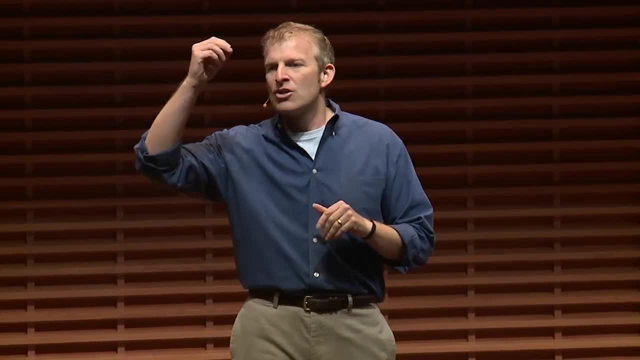 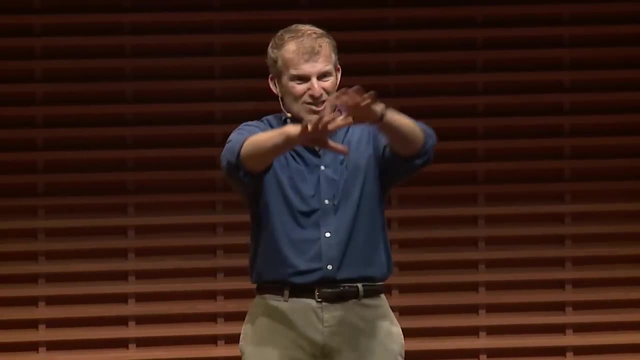 I'm frustrated. Now we're arguing over their mental state, emotional state, So I say something like: I hear you have a lot of passion on this issue, Or I hear there's great concern from you, So you acknowledge the emotion, because otherwise it sits in the room. 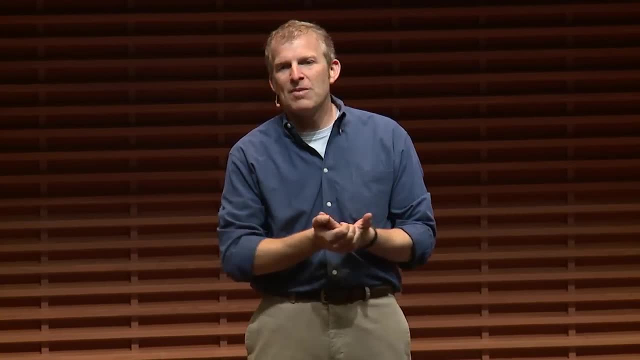 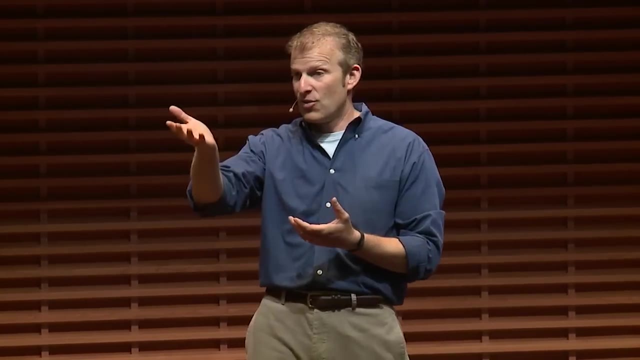 And then reframe or respond the way that makes sense. So if somebody raises their hand and says your product is ridiculously priced, Why do you charge so much? I might say I hear great concern, And what you're really asking about is the value of our product. 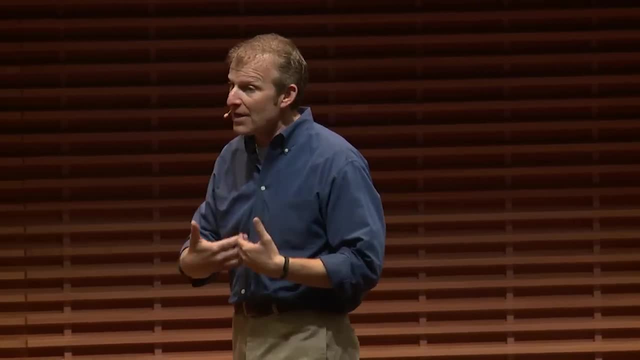 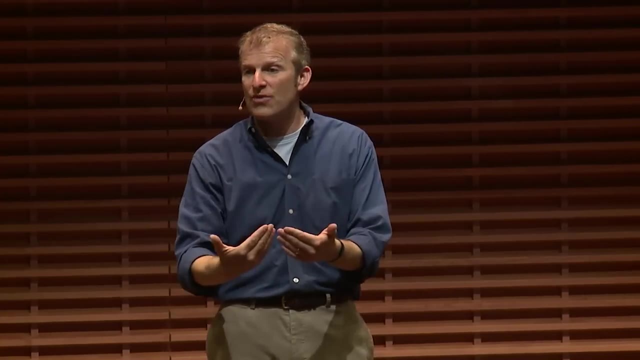 And I would give my value proposition. And then I would come back and say: and because of the value we provide, we believe it's priced fairly. So you answer the question about price But you reframe it And that's the way that you feel more comfortable answering it. 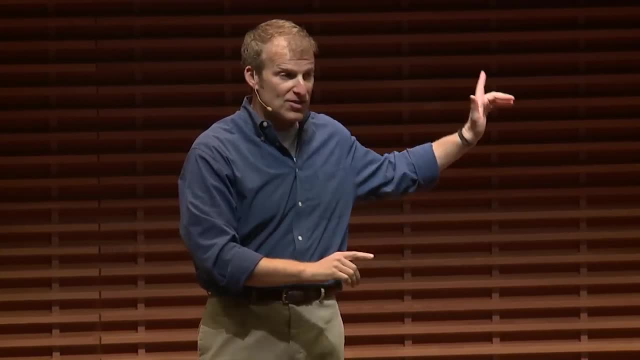 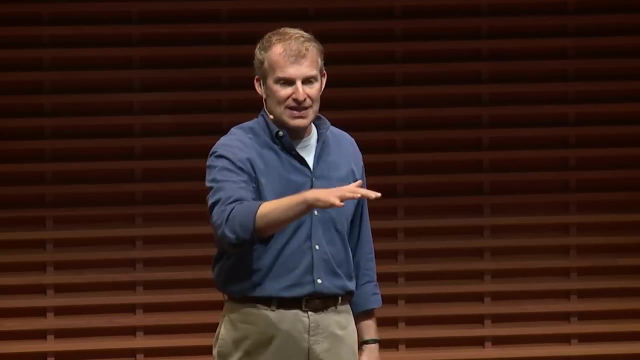 So the way to do this is to practice all the skills we just talked about. The only skill that I'm adding to this is the awareness in advance that you might be in that situation. First, I have to truly listen to what I'm hearing. 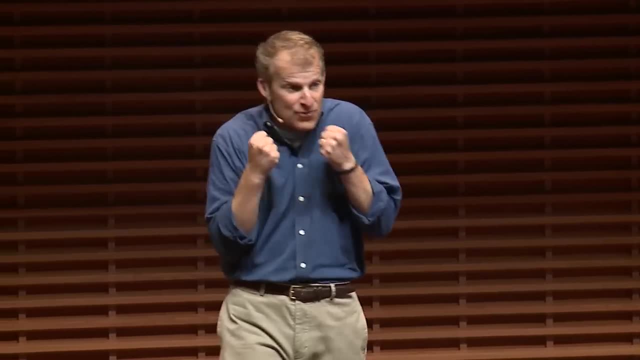 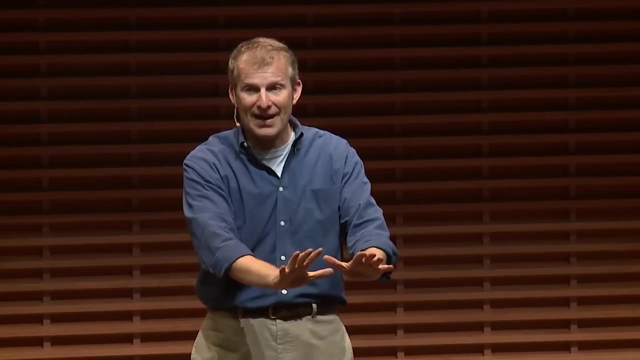 It's very easy for me, when I hear a challenging question, to get all defensive and not hear what the person's asking. I see it as an opportunity to reframe and explain. So again, you have to practice, But that's how I think you address it. 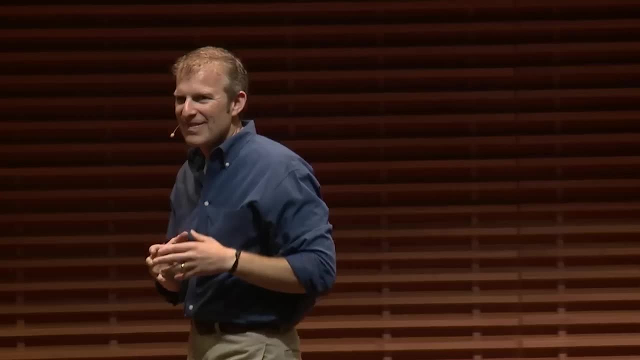 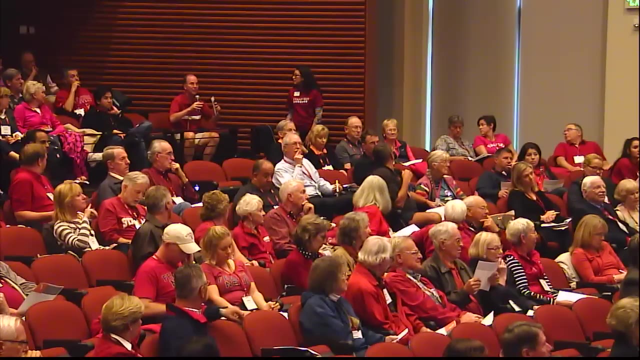 Are there other questions? I see a question back here. Yes, please, Yes. first of all, thank you very much. Great, great presentation. Thank you For a lot of the speaking I do. I have remote audiences, audiences distributed all over. 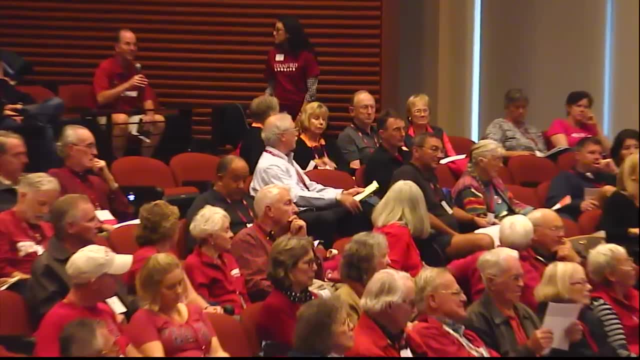 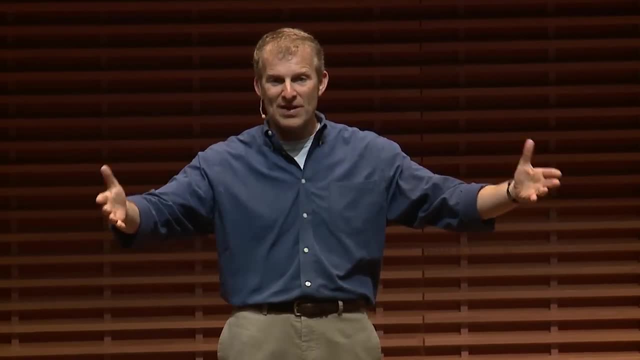 the country with telecom, Any tips for those kinds of audiences? So when you are speaking in a situation where not everybody is co-located- in fact, right at this very moment, there are people watching this presentation remotely- What you need to do is be mindful of it. 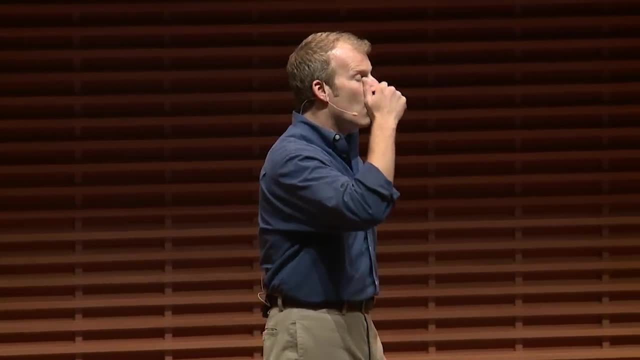 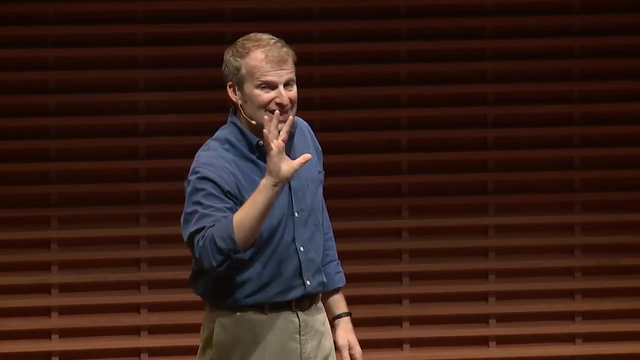 The only skill that I'm adding to this is the awareness in advance that you might be in that situation. First, I have to truly listen To what I'm hearing, right. It's very easy for me, when I hear a challenging question, to get all defensive. 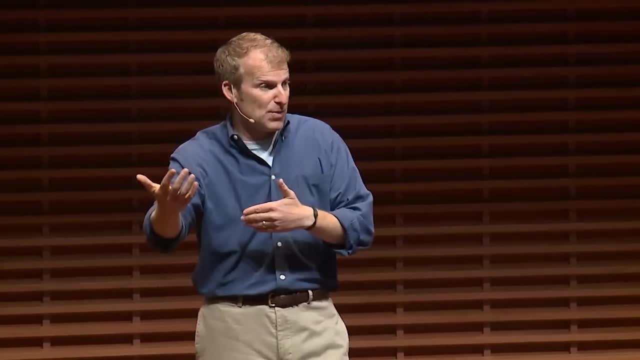 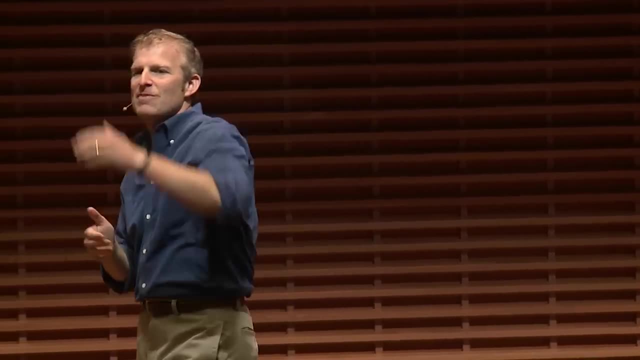 And not hear what the person's asking. I see it as an opportunity to reframe and explain. Okay, so again, you have to practice, But that's how I think you address it. Are there other questions? I see a question back here. 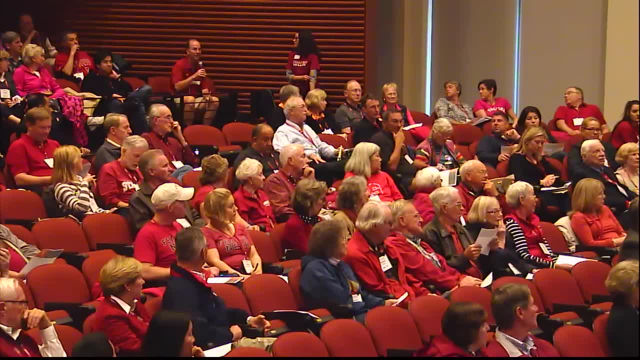 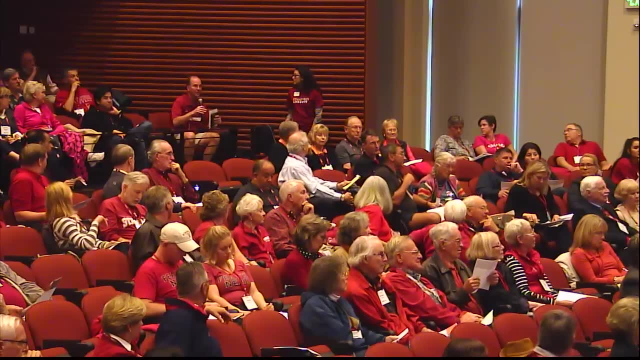 Yes, please Yes. first of all, thank you very much. Great, great presentation. Thank you For a lot of the speaking I do. I have remote audiences, Audiences distributed all over the country with telecom. Any tips for those kinds of audiences? 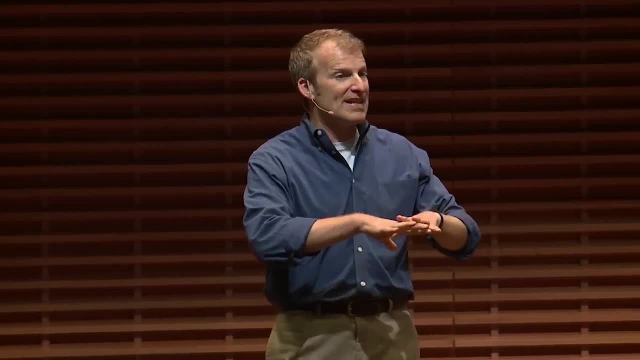 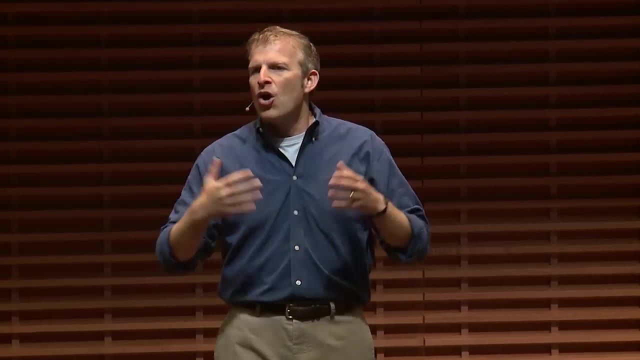 So when you are speaking in a situation where not everybody is co-located- in fact, right at this very moment, there are people watching this presentation remotely- What you need to do is be mindful of it. Second, try to include engagement techniques. 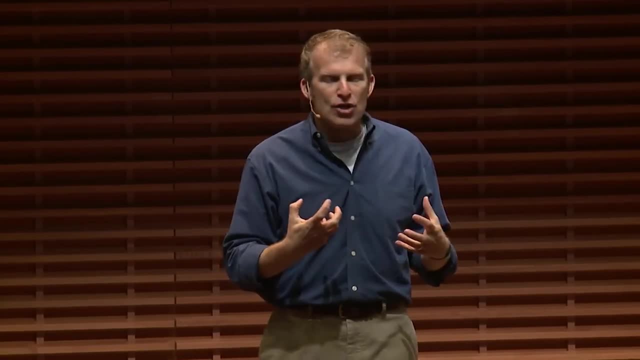 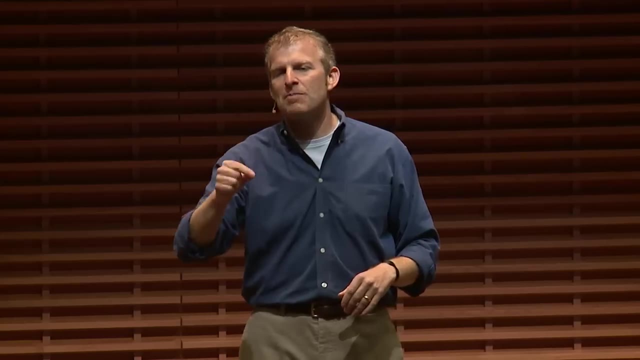 where the audience actually has to do something. So physical participation is what we did here. through the games, You can ask your audience to imagine something. Imagine what it would be like if, when we tried to achieve a goal, rather than say here's the goal we're trying to achieve, say: imagine what. 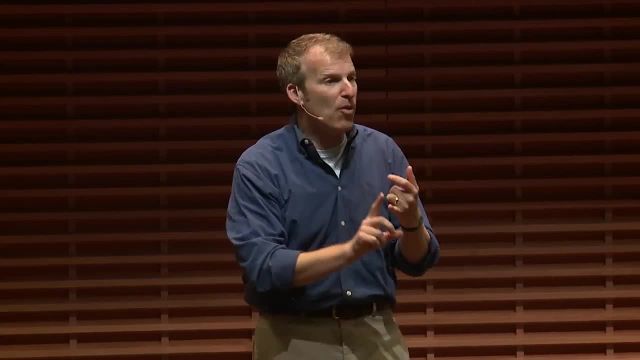 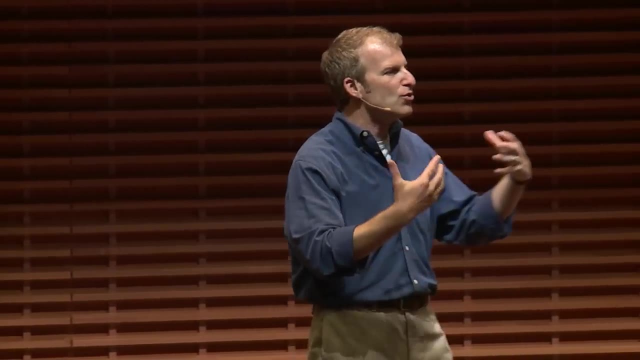 it would be like if See what that does to you, It pulls you in. I can take polling questions. Most of the technology that you're referring to has some kind of polling feature. You can open up some kind of Wiki or Google Doc or some collaborative tool where people 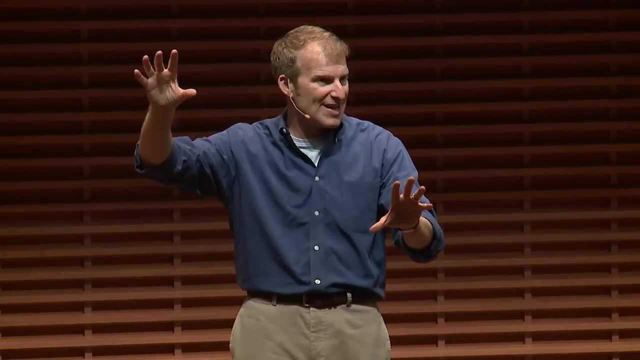 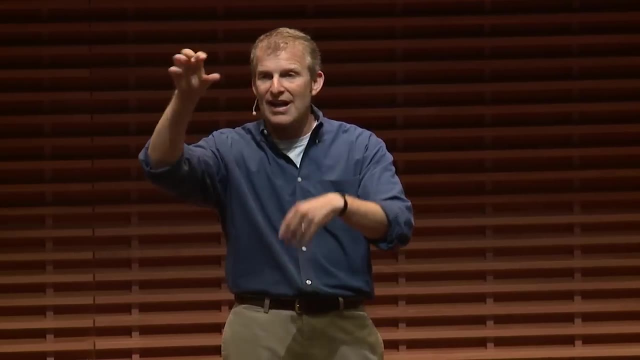 can be doing things and you can be monitoring that while you're presenting. So I might take some breaks. I talk for 10, 15 minutes and say, okay, let's apply this and let's go into this Google Doc I've created and I see what people are doing. 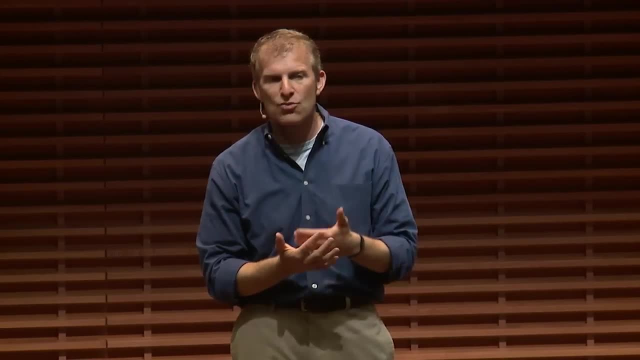 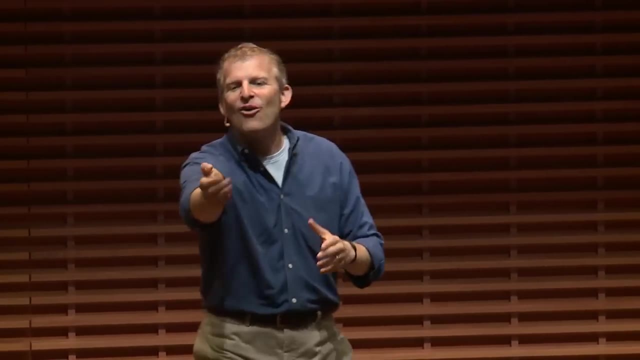 So it's about variety And it's about engagement. Those are the ways that you really connect to people who are remote from you. Other questions You're pointing? Oh, I've got to look for where the mic is. Yes, please. 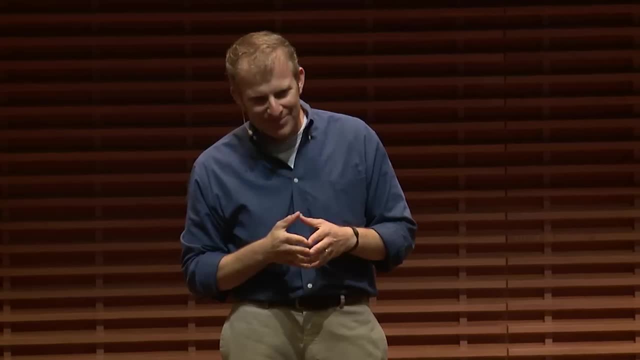 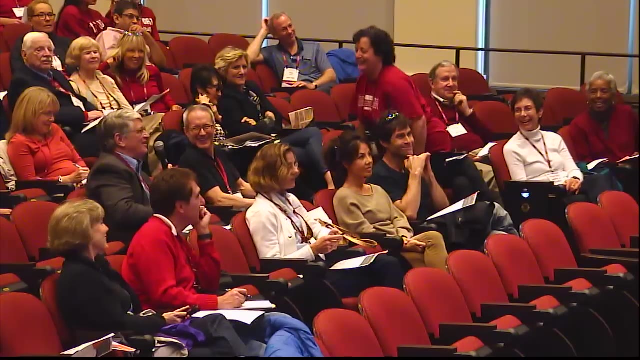 This might be similar to the first question, but I do a lot of expert witness testimony. What's your recommendation for handling cross-examination specifically, Specifically a hostile? I feel like I'm being cross-examined Right. That's very hostile. 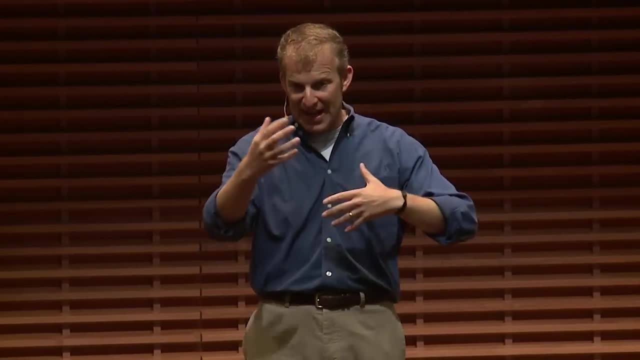 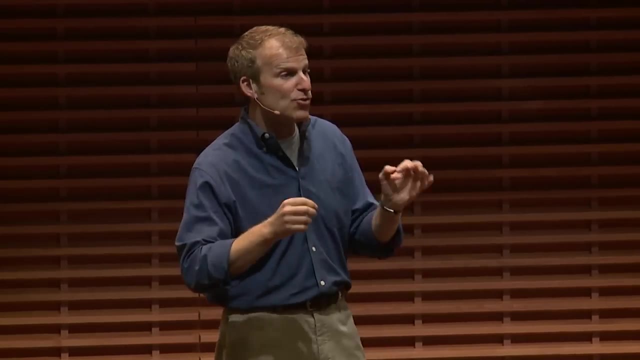 So in any speaking situation that you go into that has some planned element to it, I recommend identifying certain themes that you think are important or believe need to come out, And then, with each one of those themes, have some examples and concrete evidence that you 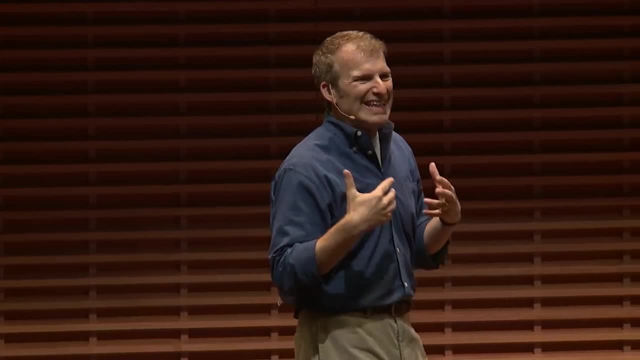 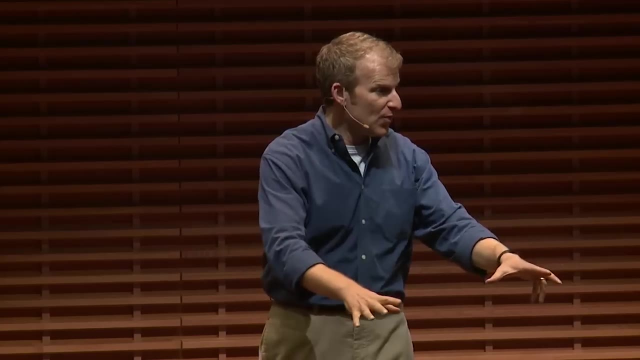 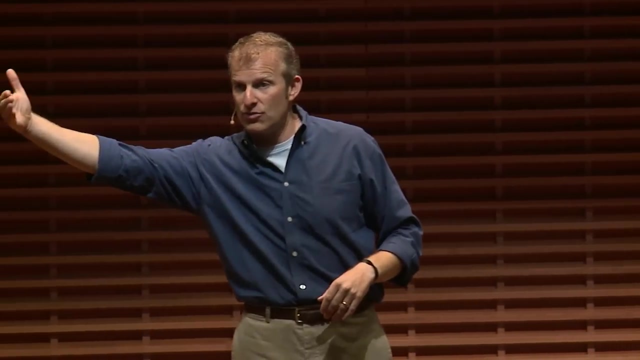 Second, try to include engagement techniques where the audience actually has to do something. So physical participation is what we did here. through the games, You can ask your audience to imagine something. Imagine what it would be like if, when we try to achieve a goal, 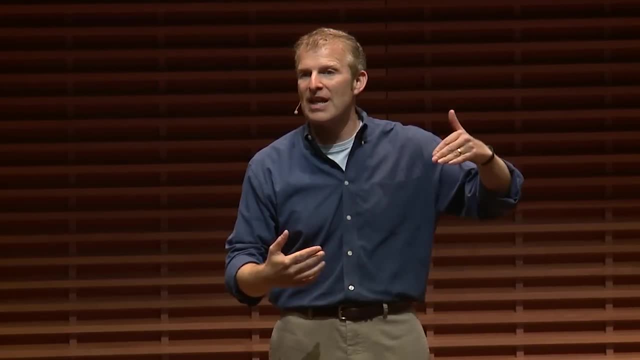 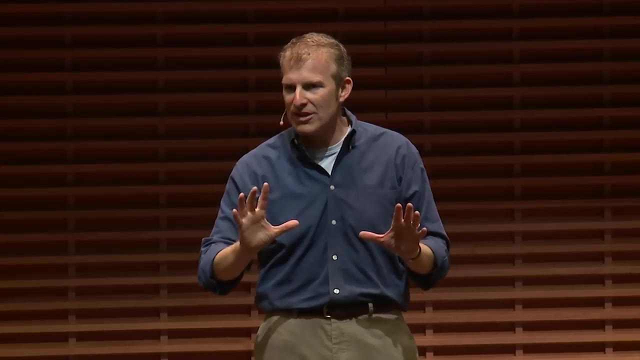 Rather than say here's the goal we're trying to achieve, say: imagine what it would be like if See what that does to you. It pulls you in. I can take polling questions. Most of the technology that you're referring to has some kind of polling feature. 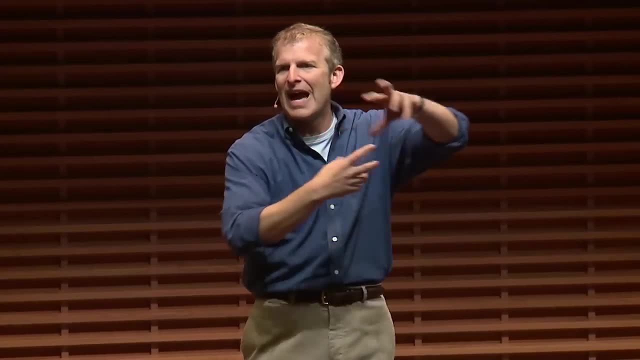 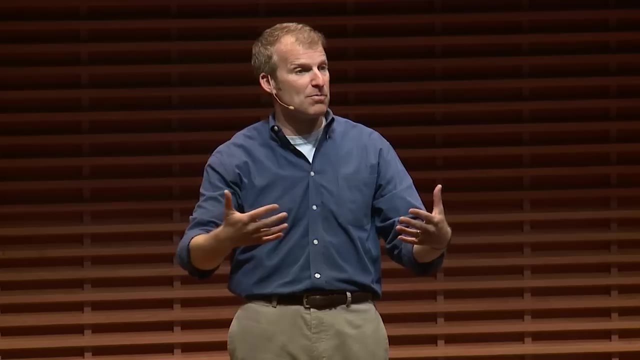 You can open up some kind of Wiki or Google Doc or some collaborative tool where people can be doing things and you can be monitoring that while you're presenting. So I might take some breaks. I talk for 10, 15 minutes and say: okay, let's apply this and let's go into this Google Doc. 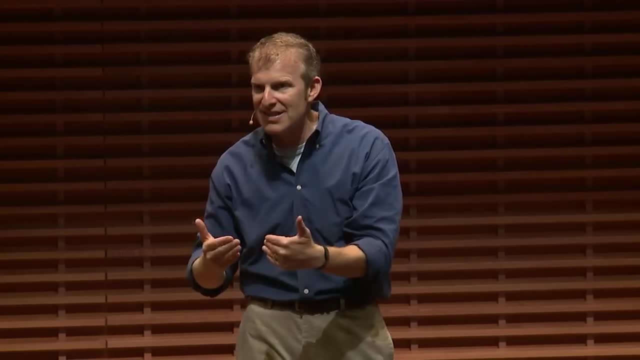 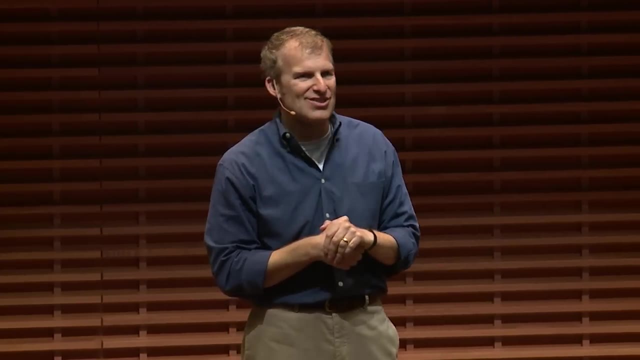 I've created and I see what people are doing. So it's about variety and it's about engagement. Those are the ways that you really connect to people who are remote from you. Okay, Other questions You're pointing? Oh, I've got to look for where the mic is. 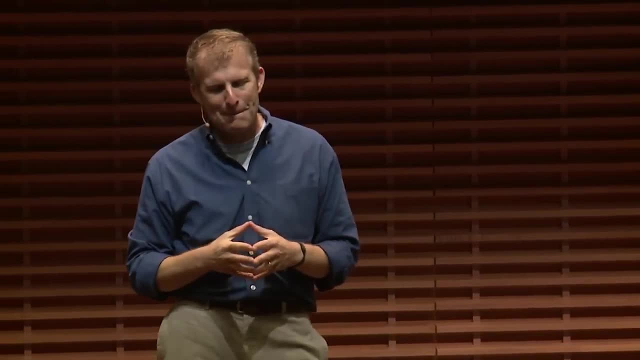 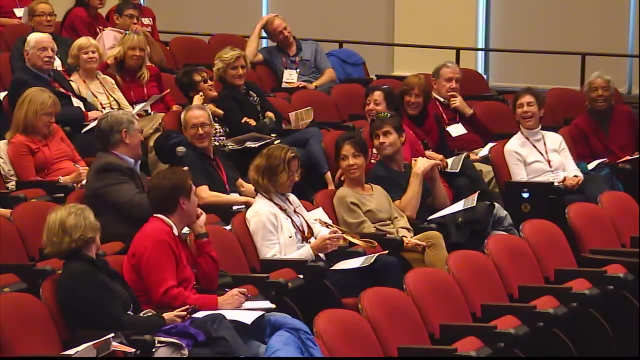 Yes, please. This might be a similar to the first question, but I do a lot of expert witness testimony. What's your recommendation for handling cross-examination specifically? Specifically, I feel like I'm being cross-examined Right. That's very hostile. 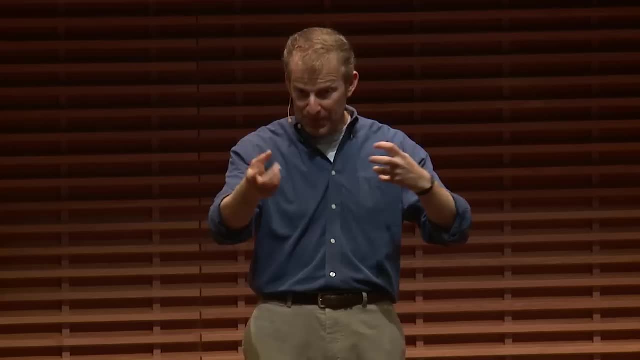 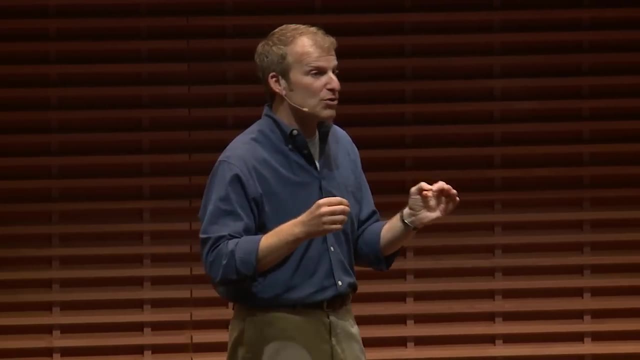 So in any speaking situation that you go into that has some planned element to it, I recommend identifying certain themes that you think are important or believe need to come out, And then, with each one of those themes, have some examples and concrete evidence that you 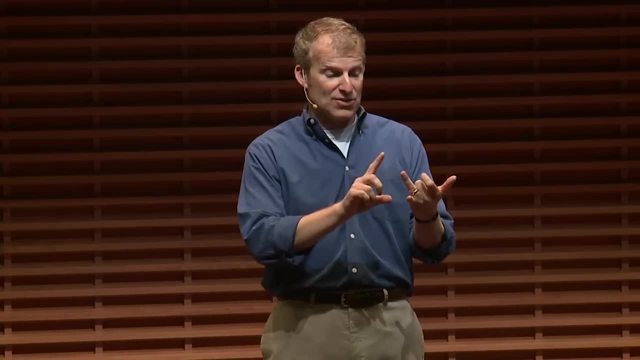 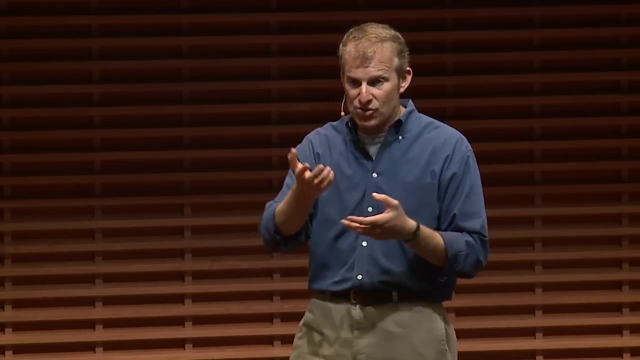 can use to support it. You don't go in with memorized terms or ways of saying it. You just have ideas and themes and then you put them together as necessary. So when I'm in a situation where people are interrogating me, I have certain themes that 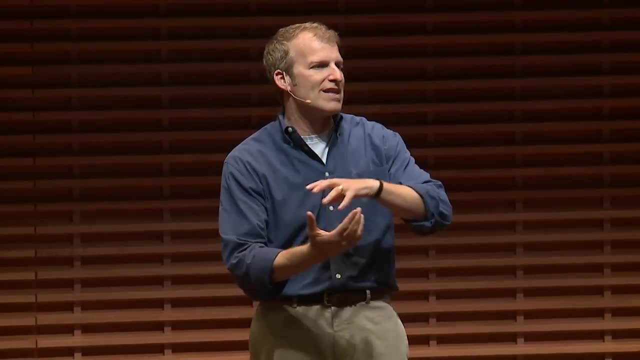 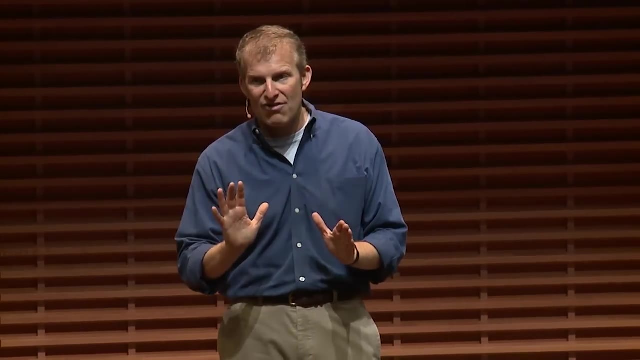 I want to get across and make sure that I can do that in a way that fits the needs in the moment. If it's hostile again, the single best tool you have to buy yourself time and to help you answer a question efficiently is paraphrasing. 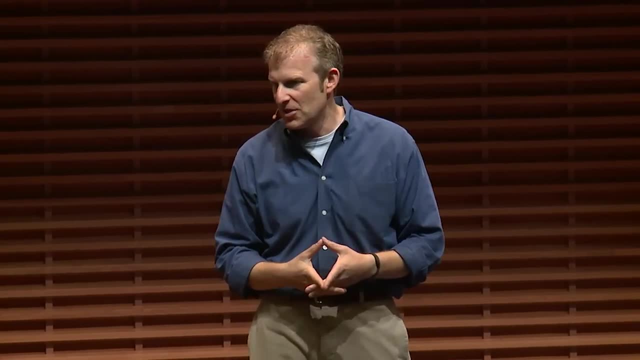 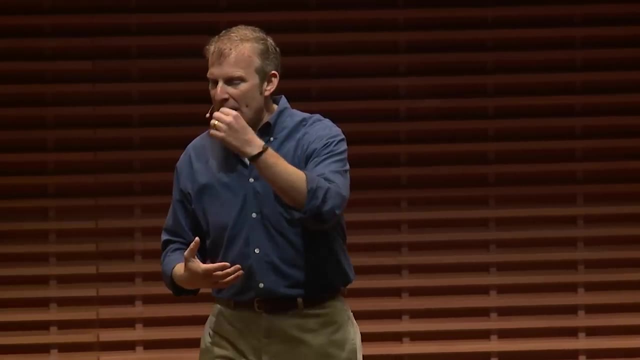 Okay, Paraphrase is like the Swiss army knife of communication. If you remember the show MacGyver, it's your MacGyver tool, Right? So when a question comes in the way you paraphrase, it allows you the opportunity to reframe it. 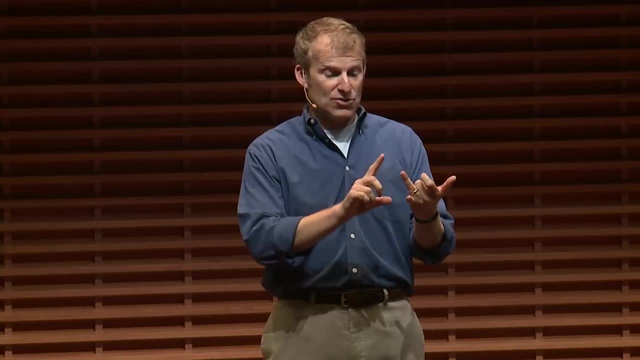 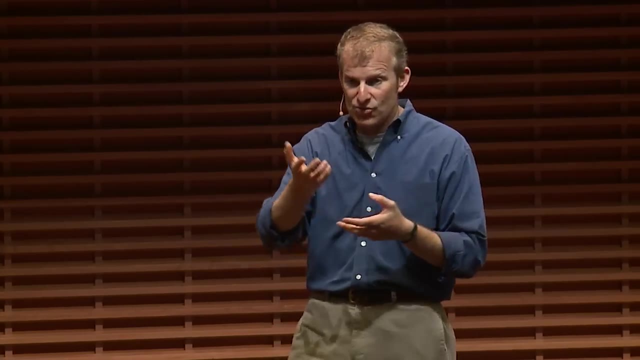 can use to support it. You don't go in with memorized terms or ways of saying it. You just have ideas and themes and then you put them together as necessary. So when I'm in a situation where people are interrogating me, I have certain themes that 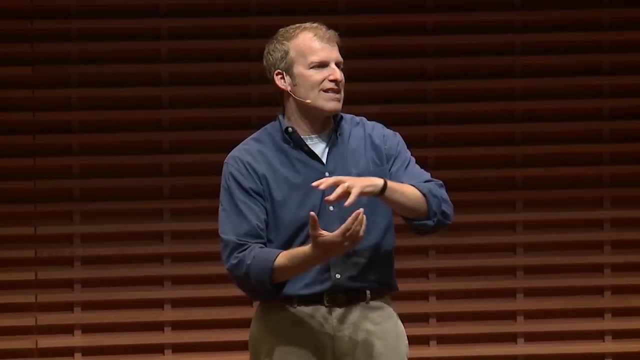 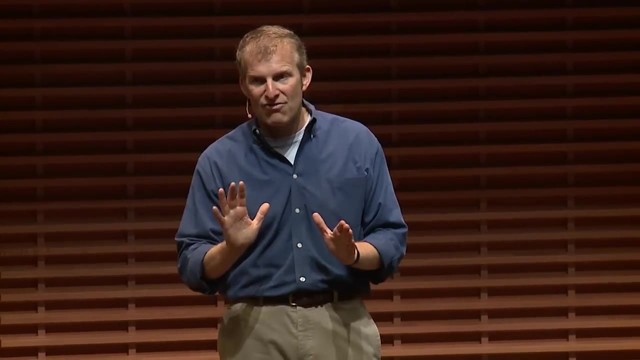 I want to get across and make sure that I can do that in a way that fits the needs in the moment And if it's hostile again, the single best tool you have to buy yourself time and to help you answer a question efficiently is paraphrasing. 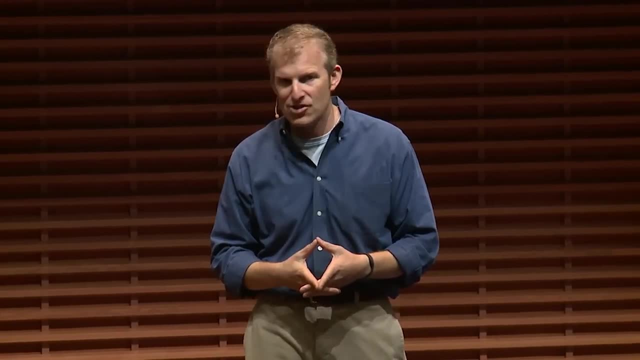 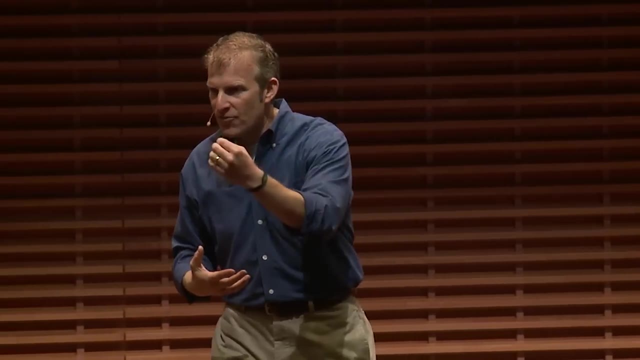 The paraphrase is like the Swiss Army knife of communication. If you remember the show MacGyver, it's your MacGyver tool. So when a question comes in the way you paraphrase, it allows you the opportunity to reframe it. 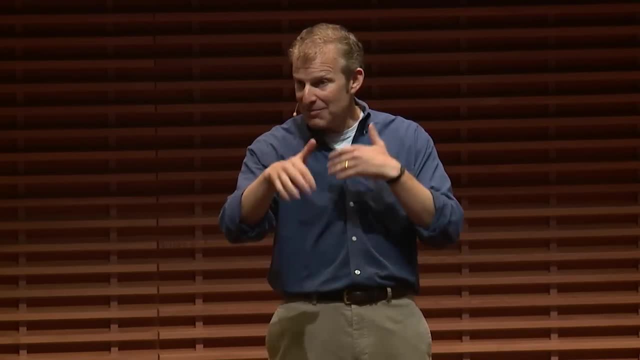 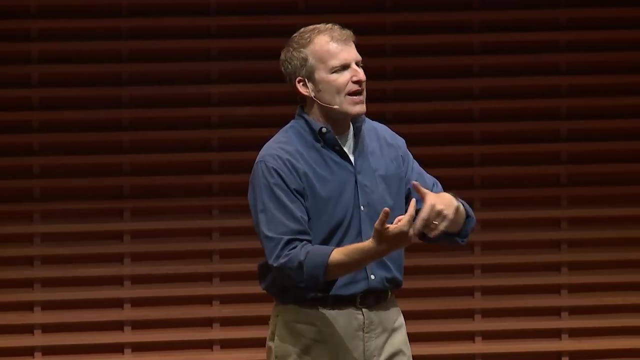 to think about your answer and to pause and make sure you got it right. So when you're under those situations, if you have the opportunity to paraphrase, say so. what you're really asking about is X, Y and Z. that gives you the opportunity to. 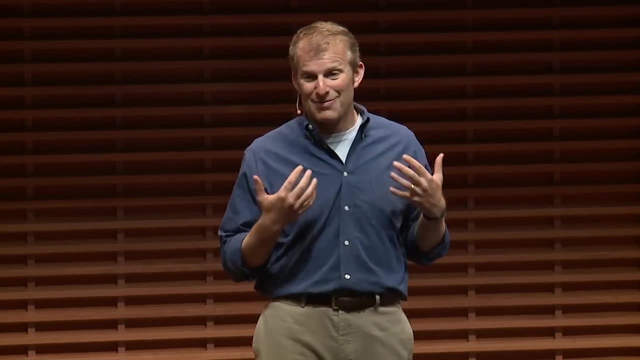 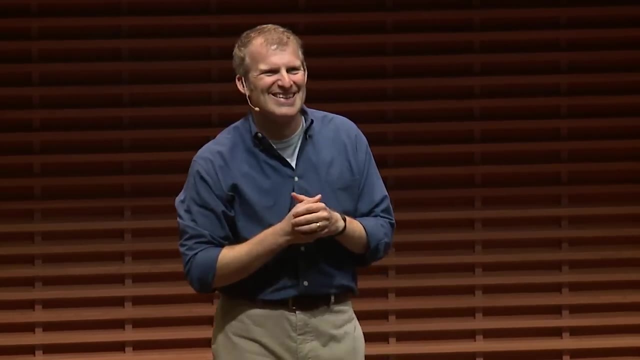 employ one of these techniques Now. I've never been an expert witness because I'm not an expert on anything but those tools I believe could be helpful. The microphone is back there, Thank you. Thank you so much. This has been so helpful and enjoyable this morning. 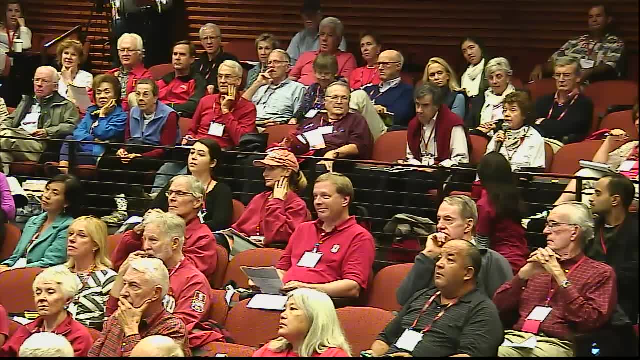 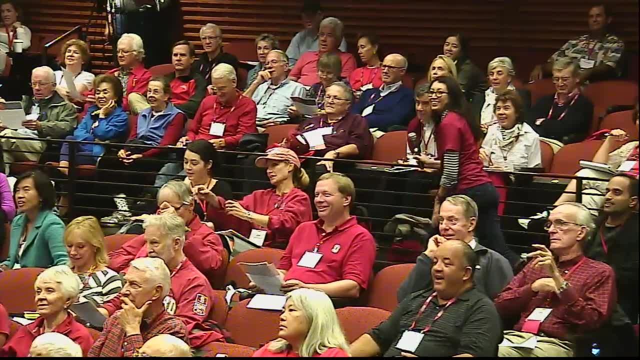 Oh, good, Thank you. Would you please show the last screen so we can get down the name of the book that you've written and the information? Absolutely Thank you. I think they actually. You might even have an opportunity to: Oh, it's on the. 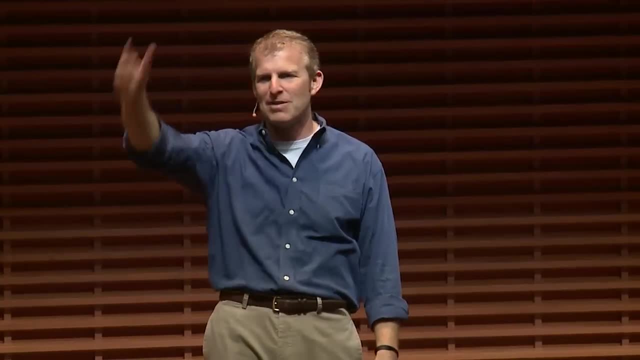 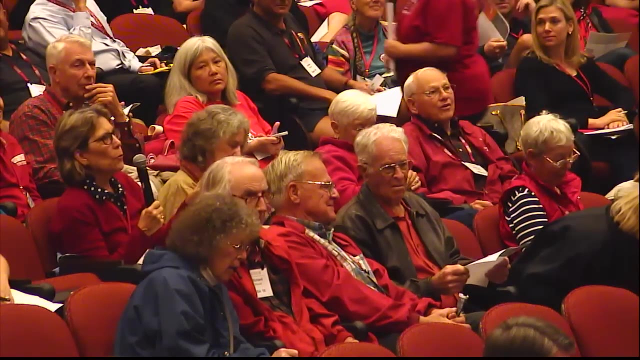 sheet too. Everything I said is on the back of that sheet, but I'm happy to have this behind me while I talk. Other questions: Yes, please. Yes. I work with groups that represent many different cultural backgrounds, so are there any caveats? 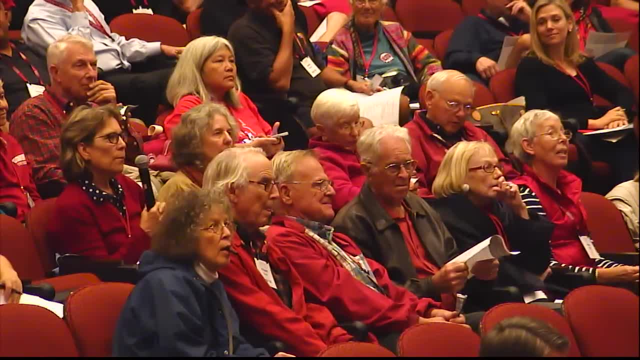 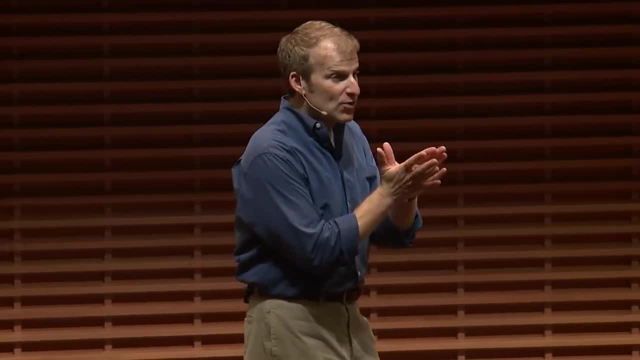 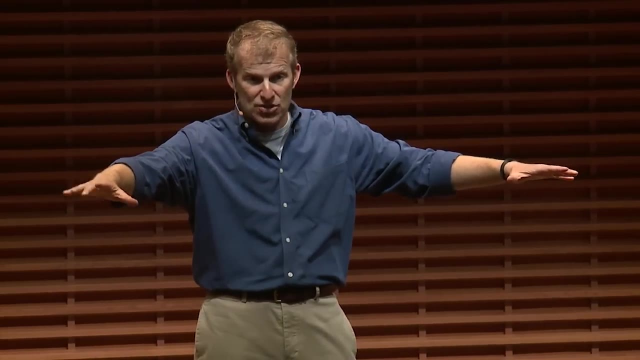 or is this a universal strategy? So, in terms of From your perspective as the speaker, I believe this applies, but whenever you communicate, part of the listening aspect is also thinking about is who is my audience and what are their expectations. So what are the cultural expectations of the audience that I'm presenting to? 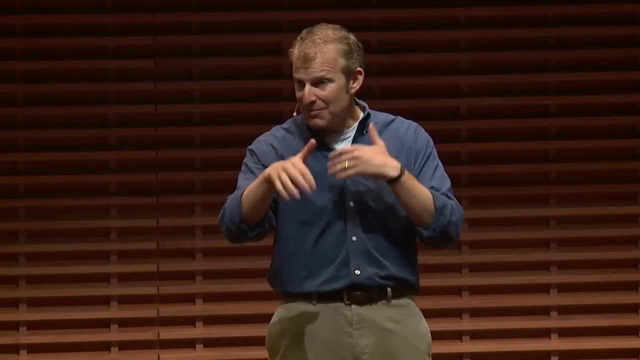 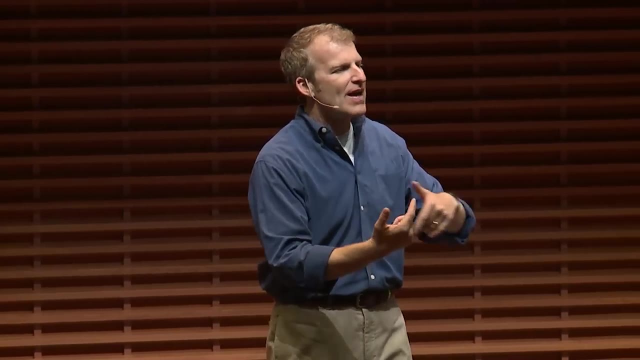 to think about your answer and to pause and make sure you got it right. So, when you're under those situations, if you have the opportunity to paraphrase, say so. what you're really asking about is X, Y and Z. that gives you the opportunity to employ. 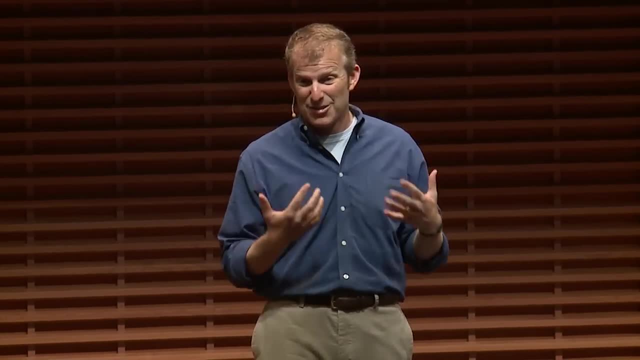 one of these techniques. Now, I've never been an expert witness because I'm not an expert witness. I'm not an expert witness. I'm not an expert on anything But those tools I believe could be helpful. The microphone is back there. 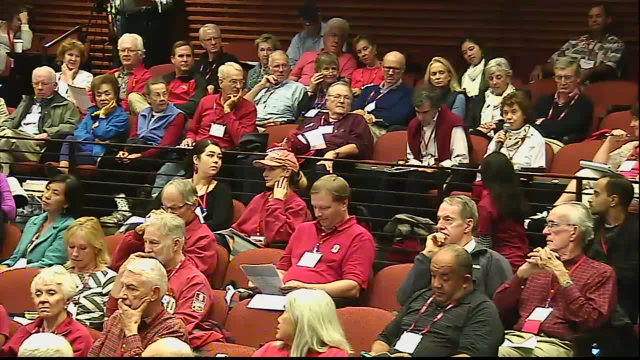 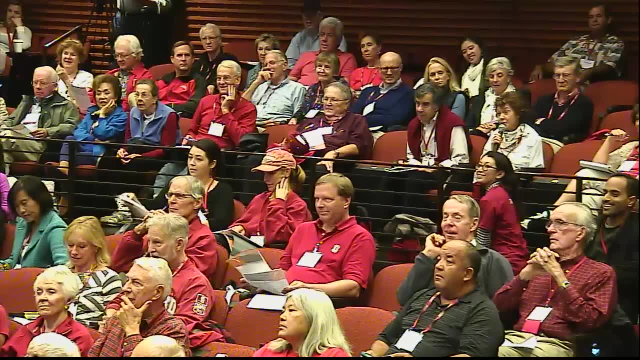 Thank you. Thank you so much. This has been so helpful and enjoyable this morning. Oh good, Thank you. Would you please show the last screen so we can get down the name of the book that you've written and the information: Absolutely. 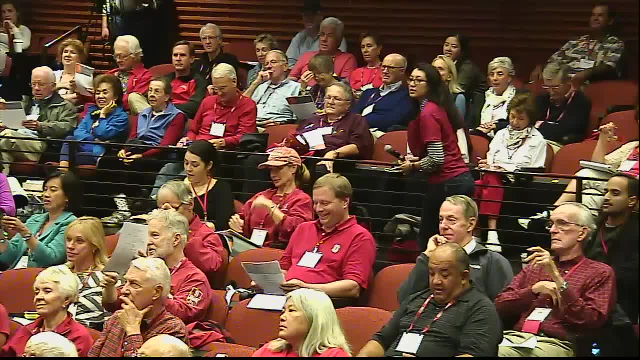 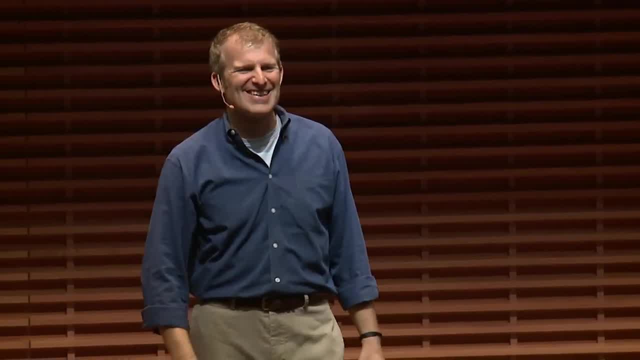 Thank you. I think they actually. You might even have an opportunity to. It's on the sheet too. Everything I said is on the back of that sheet, but I'm happy to have this behind me while I talk. Other questions. 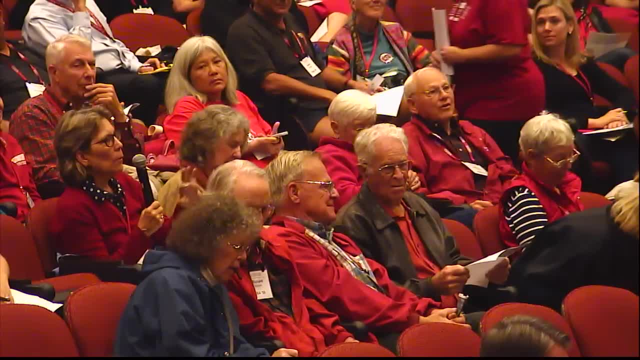 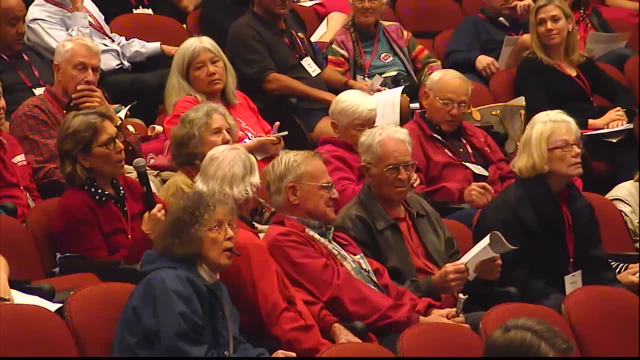 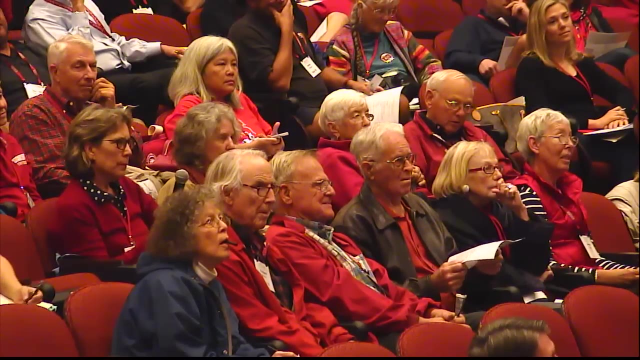 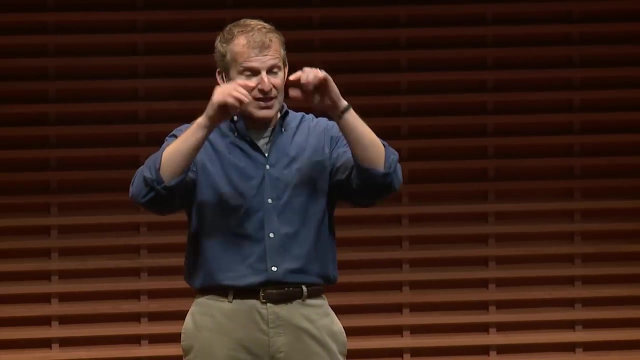 Yes, please. Yes, I work with groups that represent many different cultural backgrounds, so are there any caveats or is this a universal strategy? From your perspective as the speaker, I believe this applies, But whenever you communicate, part of the listening aspect is also thinking about is 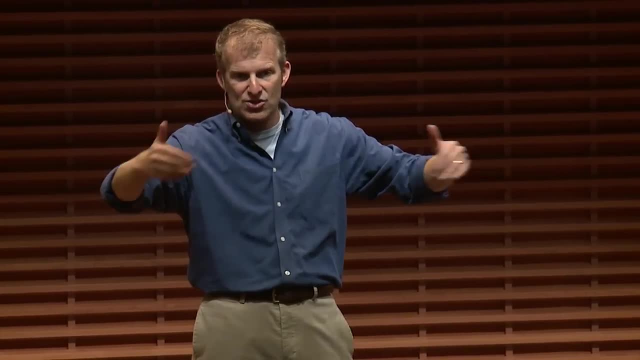 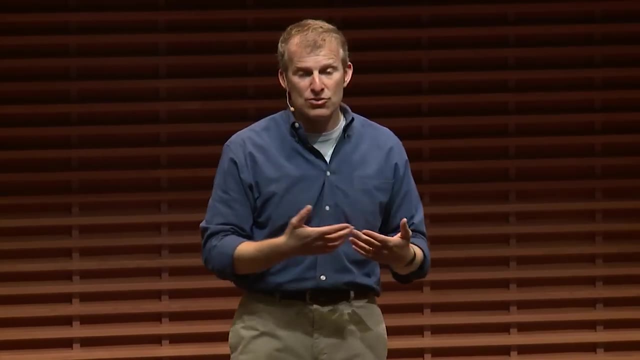 who is my audience and what are their expectations? What are the cultural expectations of the audience? What are their expectations of the audience that I'm presenting to? There might be certain norms and rules that are expected. When I travel and do talks. I have to take into account where I'm doing the presentation. 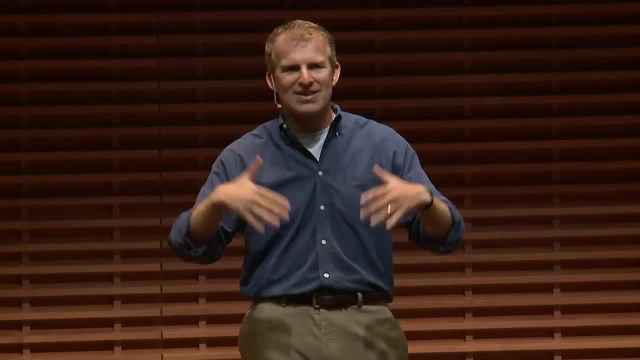 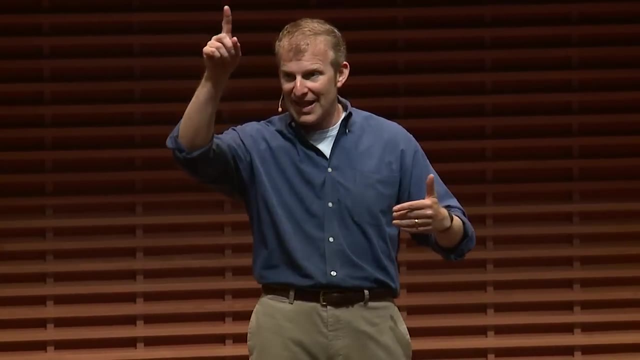 I help present in the IGNITE program. If you have not heard about the IGNITE program here at the GSB, it's fantastic. I just did a presentation standing in one of these awesome classrooms that have all these cameras and I just taught 35 people in Santiago, Chile. 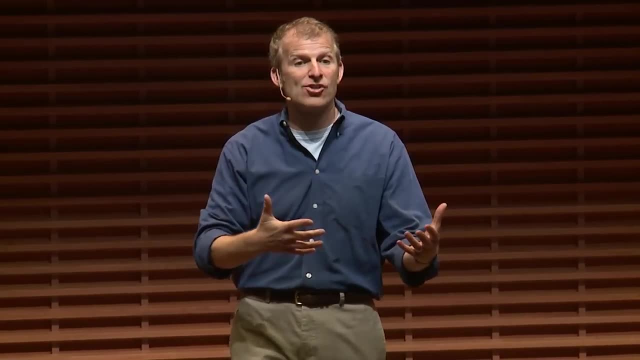 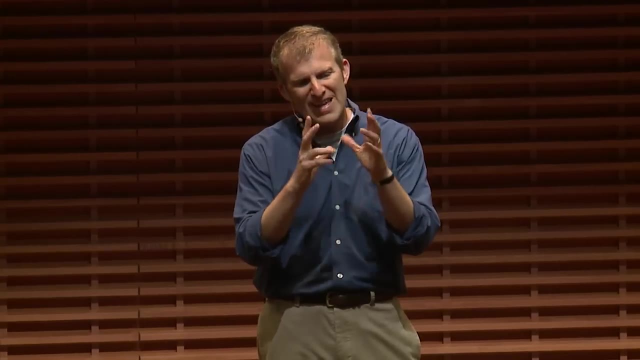 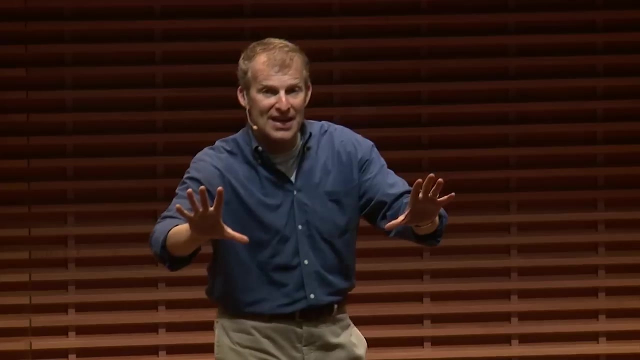 Right. I needed to understand the cultural expectations of that area and what they expect and what they're willing to do when I ask them to participate. It's part of that listening step where you reflect on what are the expectations of the audience. I think we have time for two more questions and then I'm going to hang around afterwards. 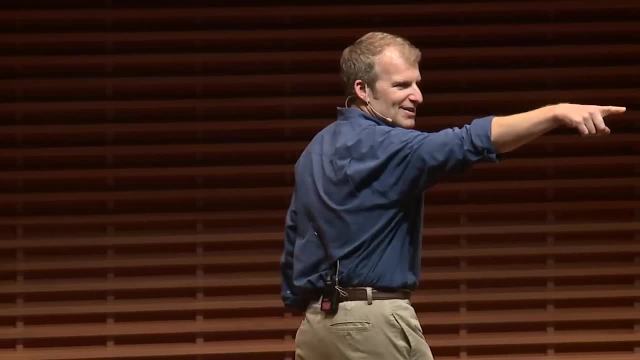 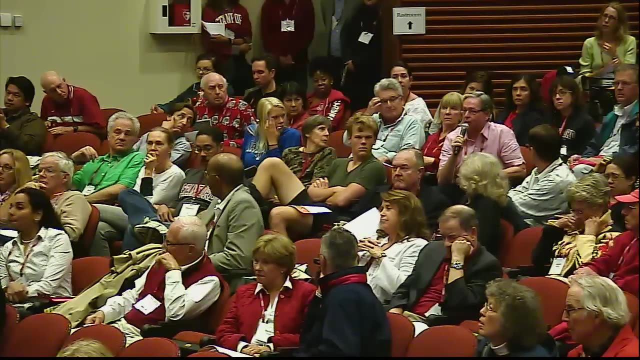 if anybody has individual questions, but some of these folks really want me to keep on schedule. Yes, please. I wanted to ask a question. One of the things that you've done effectively in your talking, and I've seen other effective speakers do, is interject humor in their talk. 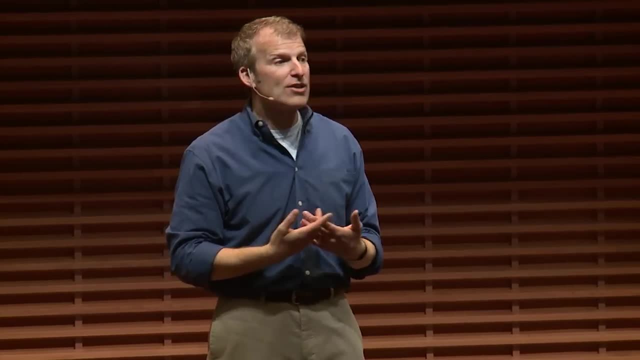 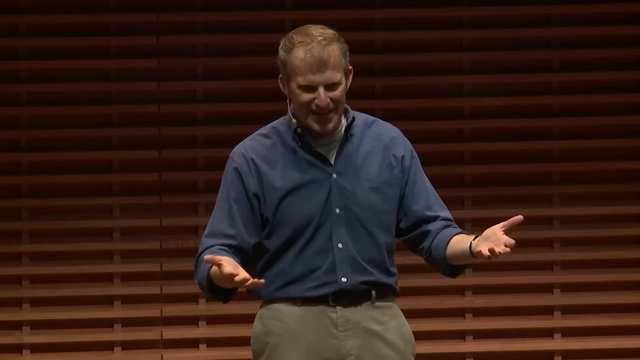 So there might be certain norms and rules that are expected. So when I travel and do talks I have to take into account where I'm doing the presentation. So I help present in the Ignite program and if you have not heard about the Ignite program, 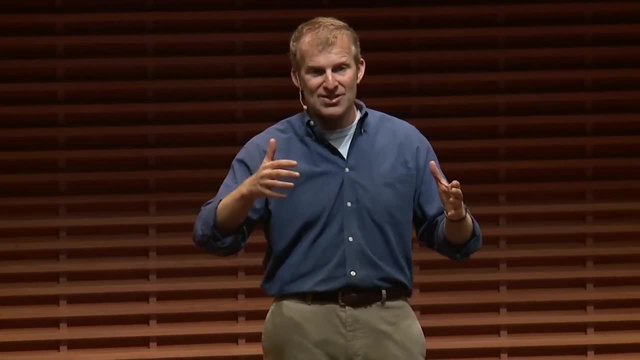 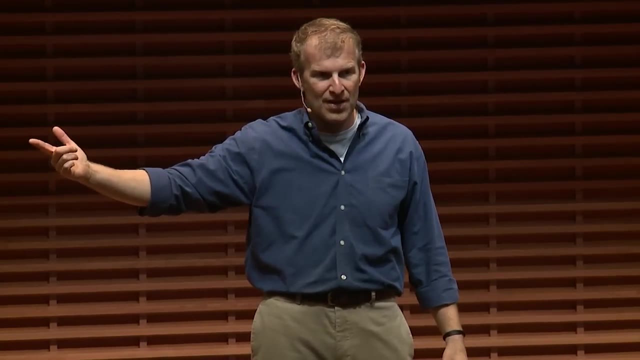 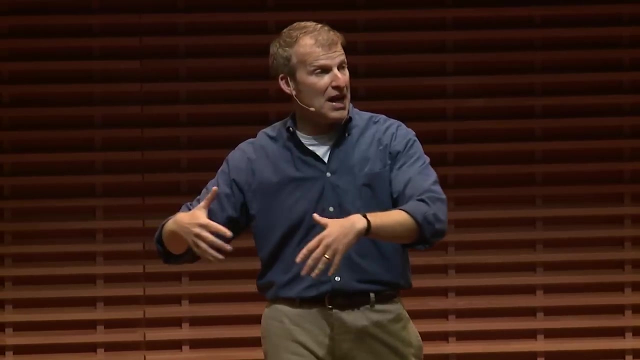 here at the GSB. it's fantastic. It's fantastic. I just did a presentation standing in one of these awesome classrooms that have all these cameras and I just taught 35 people in Santiago, Chile, And I needed to understand the cultural expectations of that area and what they expect and what. 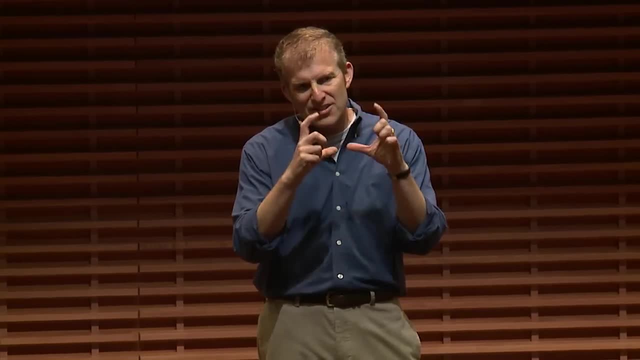 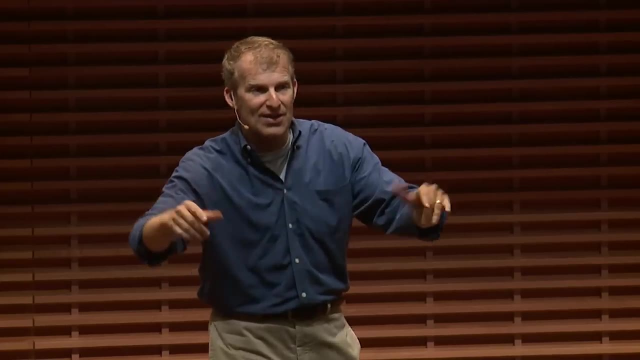 they're willing to do when I ask them to participate. So it's part of that listening step where you reflect on what are the expectations of the audience. I think we have time for two more questions and then I'm going to hang around afterwards. 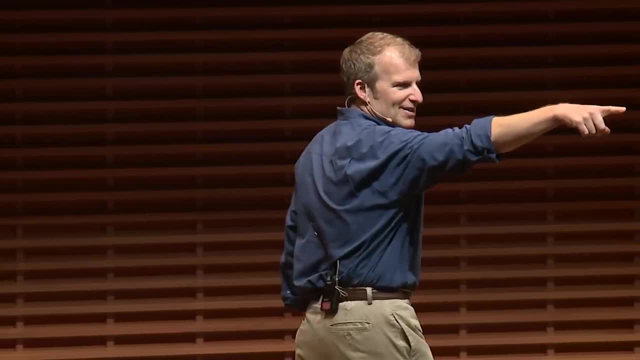 if anybody has individual questions, But some of these folks really, These folks really want me to keep on schedule. Yes, please. I wanted to ask a question, One of the things that you've done effectively in your talking- and I've seen other effective. 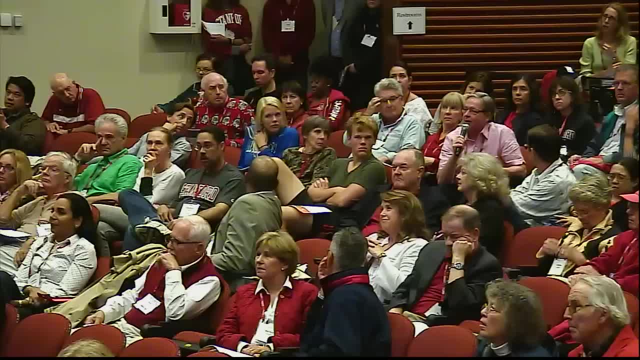 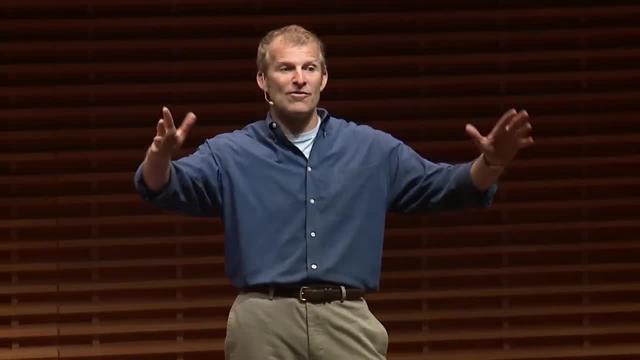 speakers do is interject humor in their talk. What are the risks and rewards of trying to do that? Well, first, thank you, and I appreciate all of you laughing. Those are, That's the sum total of all my jokes. 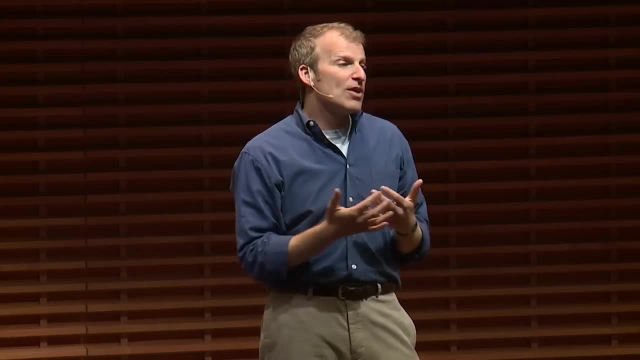 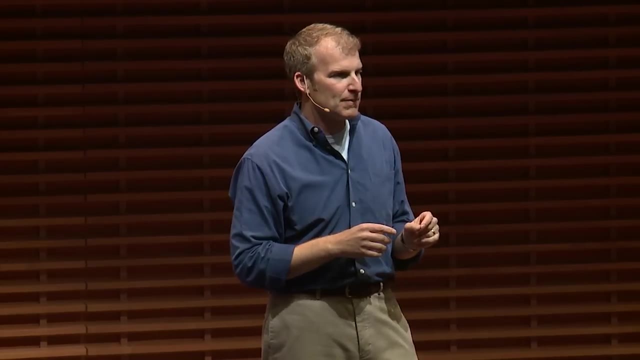 You've heard them. I am not funny beyond those jokes. So humor is wonderfully connecting. It's wonderfully connecting, It's a great tool for connection. It is very, very risky. Cultural reasons get in the way Sometimes. what you think is funny isn't funny to other people. 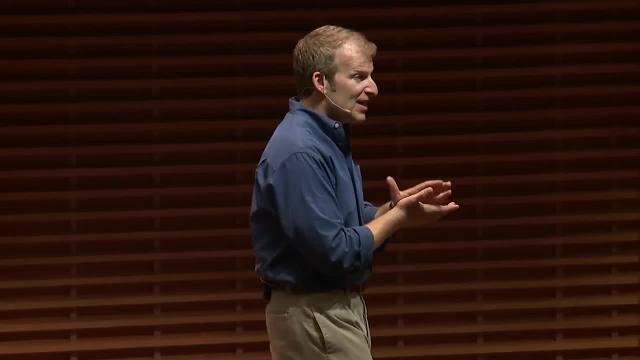 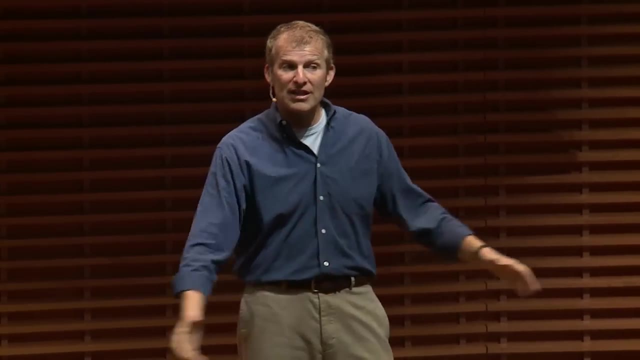 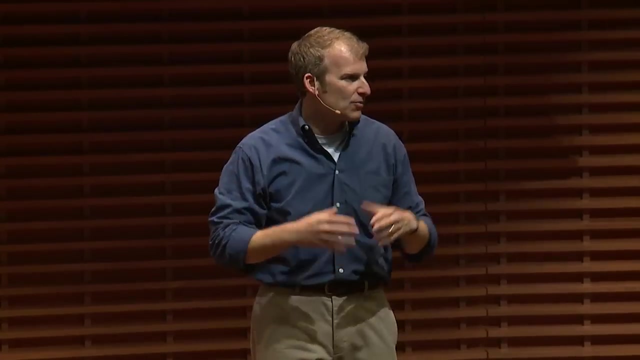 What research tells us is that if you're going to try to be funny, self-deprecating humor is your best bet, because it is the least risky. There is nothing worse than putting out a joke and having no response. It actually sets you back farther than if you would have gotten Where you would. 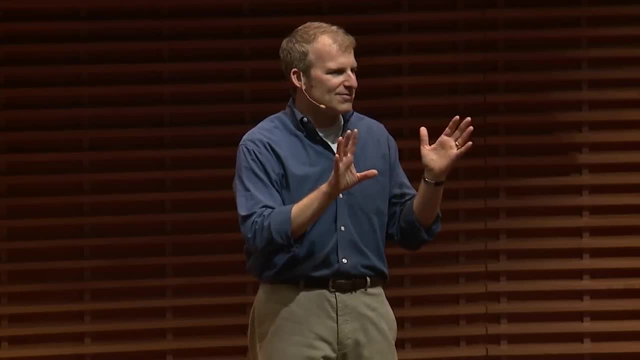 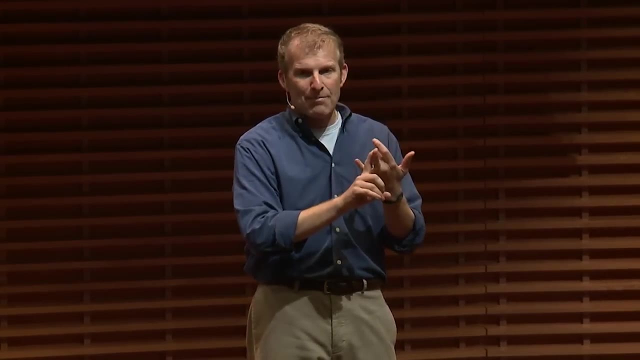 have gotten if the joke would have hit So basic fundamentals you need to think about with humor. One: is it funny? How do I know? How do I ask other people first? Second: what happens if it doesn't work? Have a backup plan. 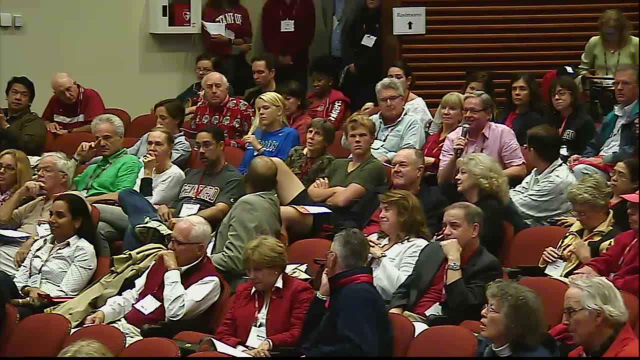 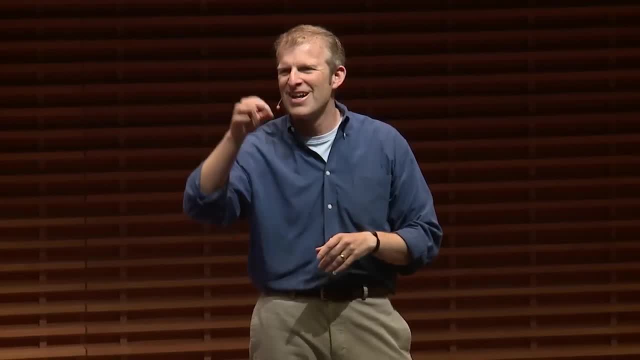 How? What are the risks and rewards of trying to do that? Well, first, thank you, and I appreciate all of you laughing. That's the sum total of all my jokes. You've heard them. I am not funny beyond those jokes. 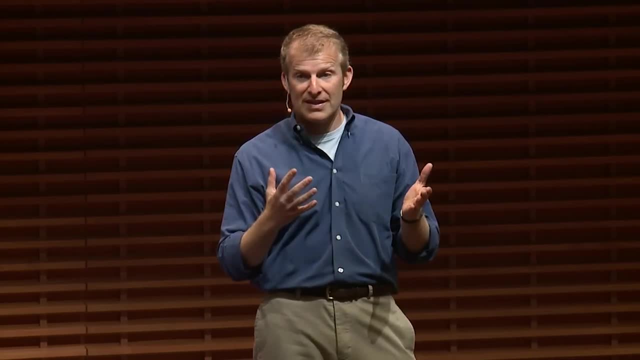 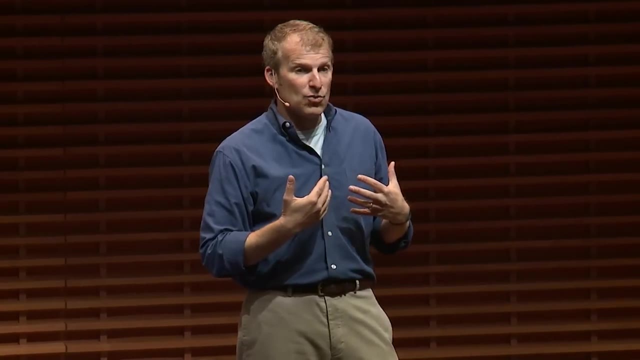 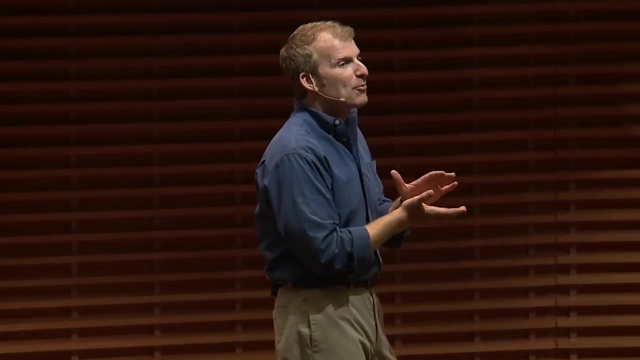 Humor is wonderfully connecting. It's wonderfully connecting. It's a great tool for connection. It is very, very risky. Cultural reasons get in the way Sometimes. what you think is funny isn't funny to other people. What research tells us is that if you're going to try to be funny, self-deprecating humor. 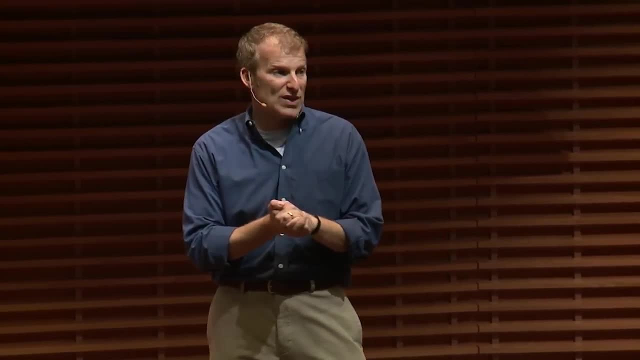 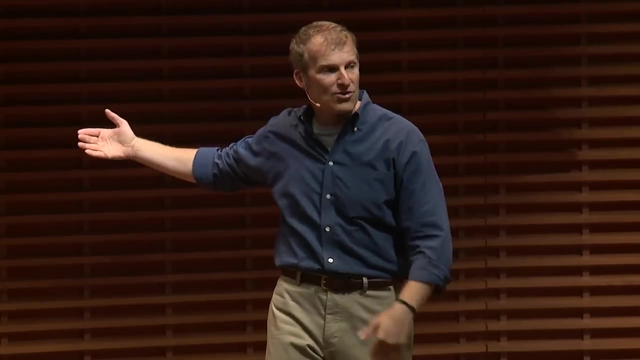 is your best bet? Okay, Because it is the least risky. There is nothing worse than putting out a joke and having no response. It actually sets you back farther than if you would have gotten where you would have gotten if the joke would have hit. 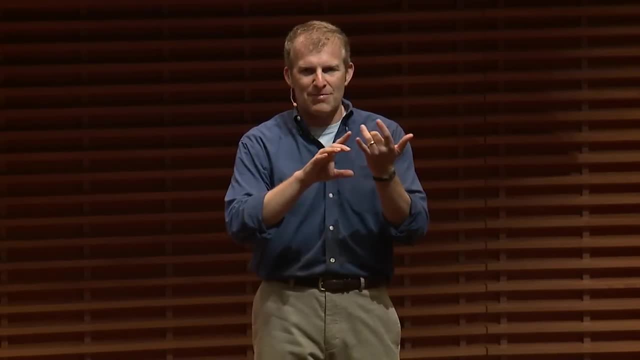 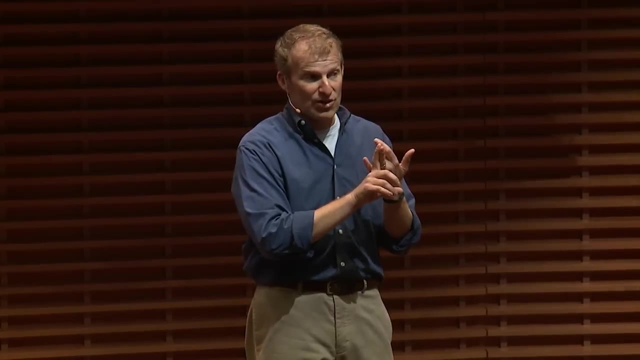 So basic fundamentals you need to think about with humor. One: is it funny? How do I know? I ask other people first. Second, what happens if it doesn't work. Have a backup plan Right. And then, third, if you're worried about the answers to those first two, don't do it. 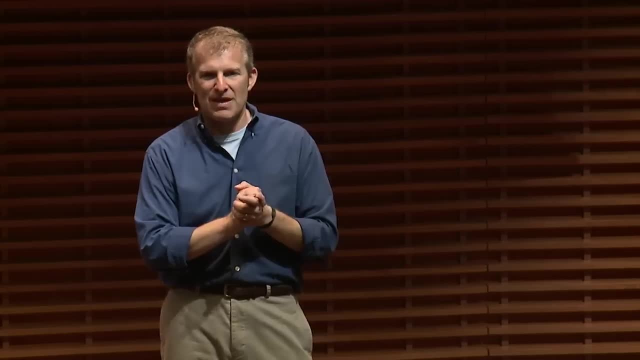 Right. One last question, please. The microphone is right here And then, like I said, I will hang around afterwards. Yes, please. I'm sort of on the opposite side of this, since I am a journalist and I frequently have to ask spontaneous questions of people who have been through media training. 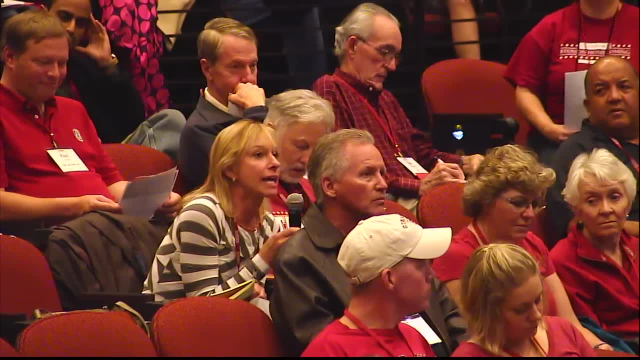 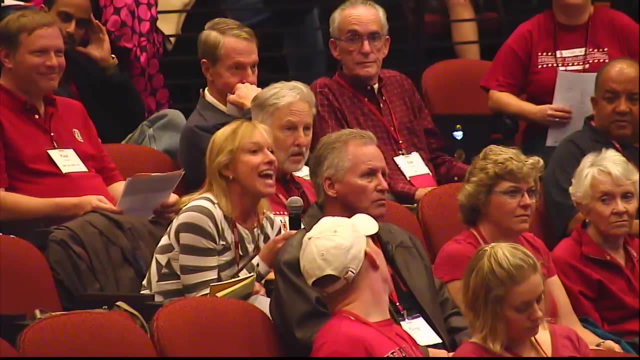 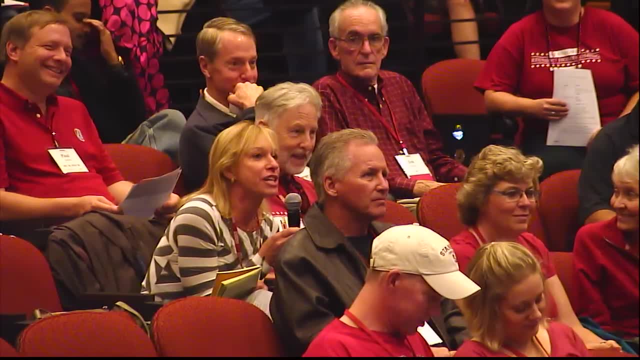 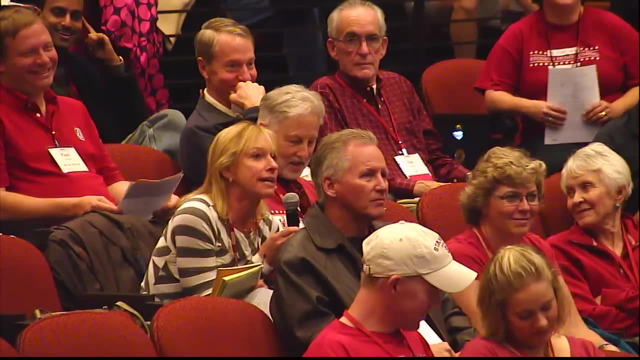 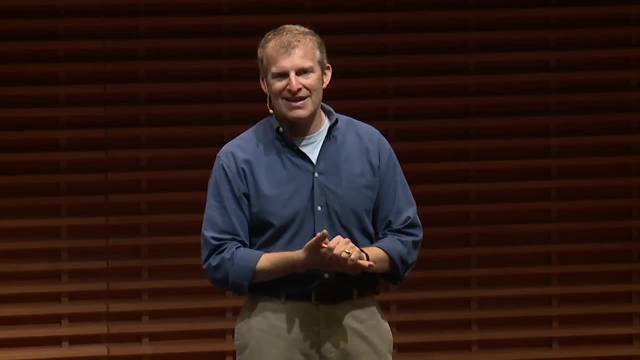 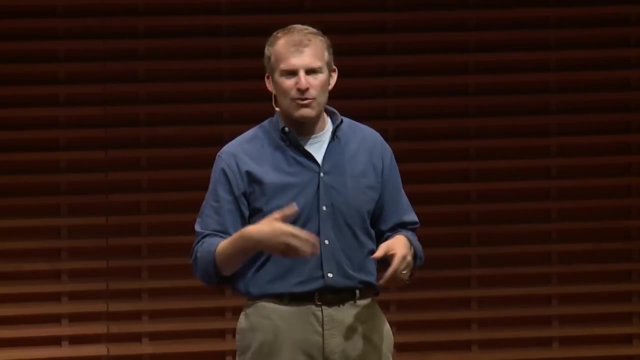 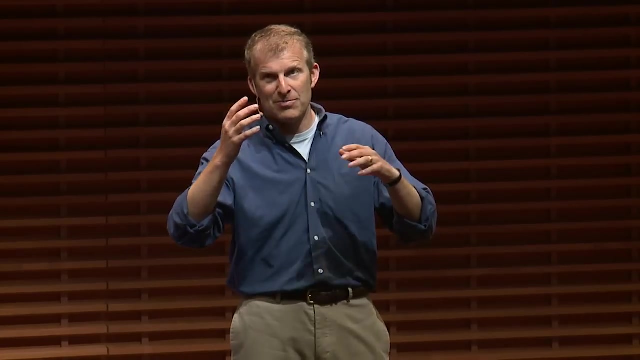 One is: I have young boys and the power of the. why is great? Just ask why. a couple of times and you can get through that. first two layers of training. Why do you say that? How do you feel about that? The second bit is to what I have found successful in getting people to. I do this to get. 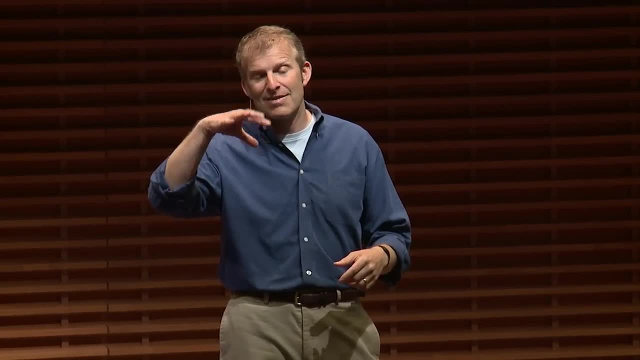 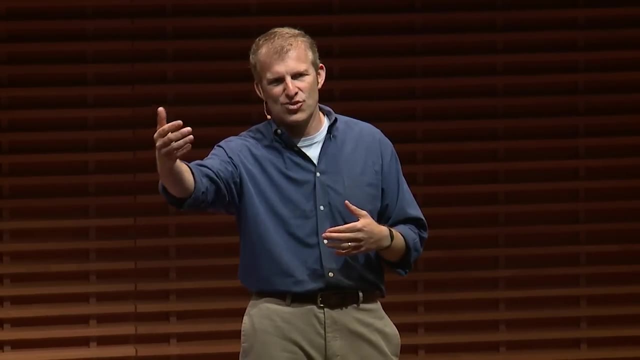 people to answer in a more authentic way. What I'll do is I'll ask them to give advice. So what advice would you give somebody? what advice would you give somebody who's So what advice would you give somebody who's challenged with this? Or what advice would you give to somebody in this situation? And